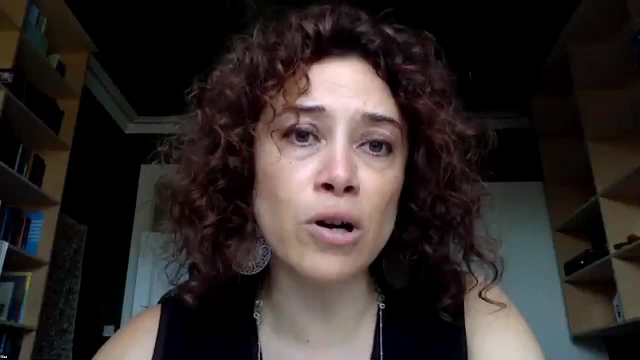 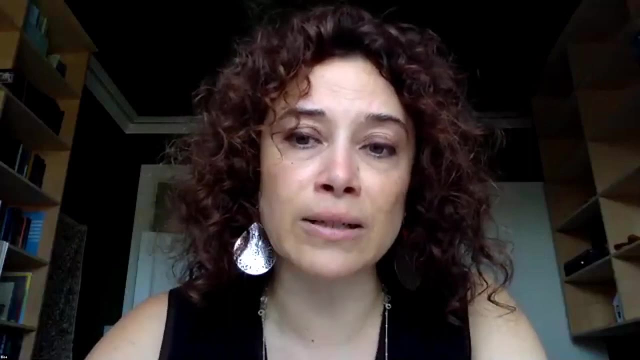 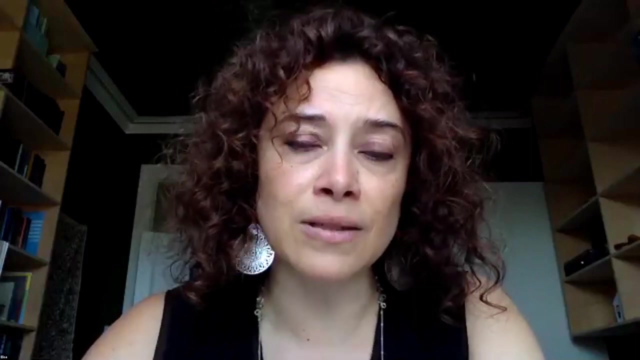 able to address multiple threats to the ocean and work across scales, from the international level to the local level, with everything else in between, and how we can really connect discussions at the UN level or at government level with the reality on the ground and the experiences and lessons learned on the. 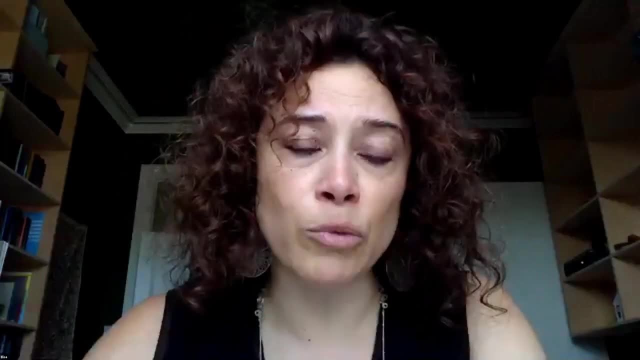 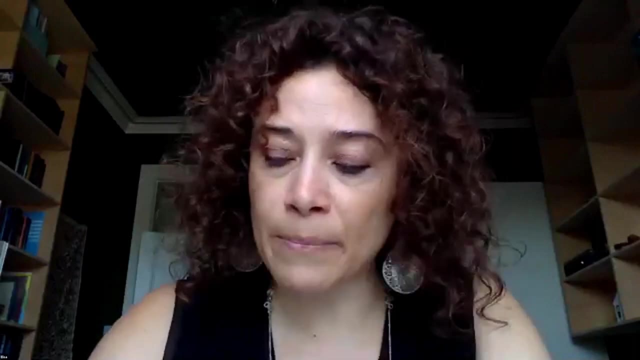 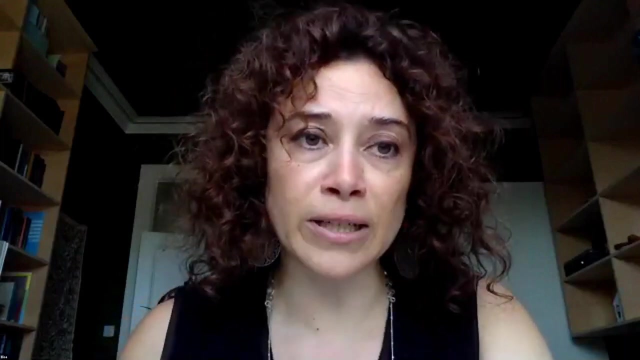 coast on the sea, of the people that are most closely dependent on the ocean. so, without further ado, I will briefly introduce the three colleagues who will be chairing and being discussants for today's session, and then our colleague Kira, who will be chairing, will introduce our incredible speaker for today. so one 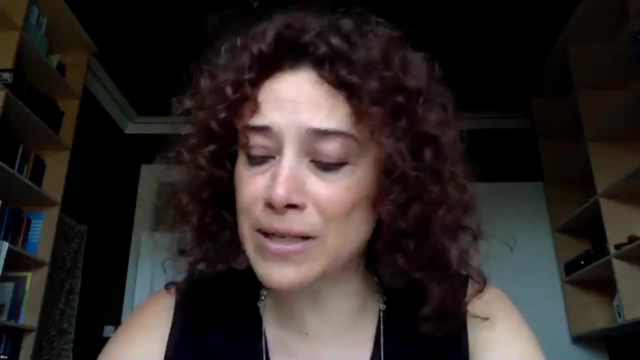 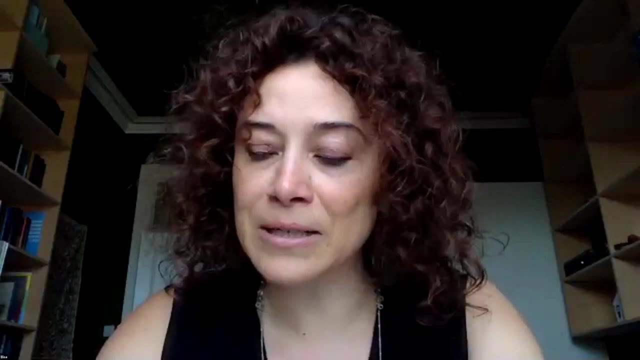 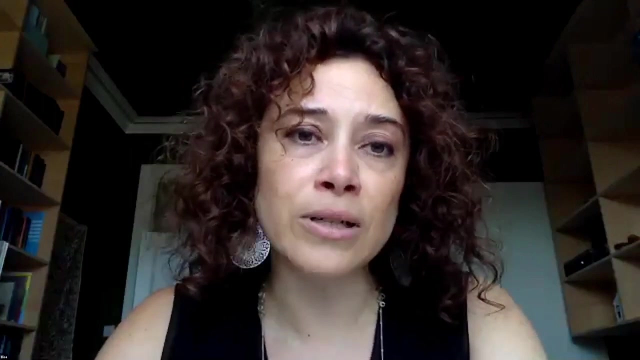 of our colleagues. well, Kira, who just appeared. Kira Erwin is senior researcher at the Urban Future Center of Durban University of Technology in South Africa. she's a sociologist and she will be chairing today's session and also contribute her own reflections on how the marine science expertise and 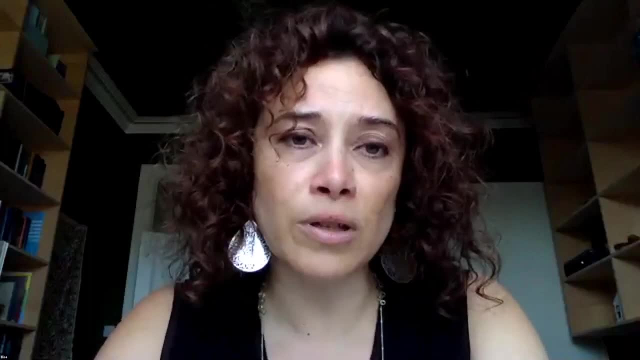 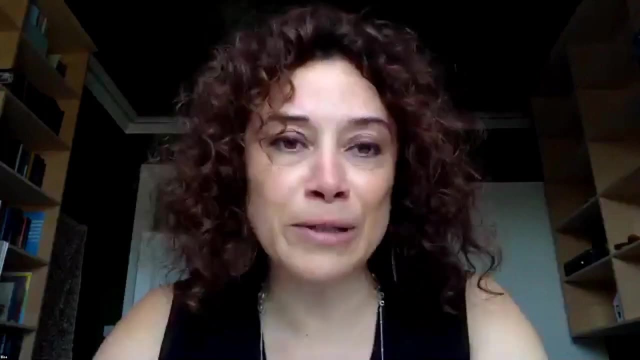 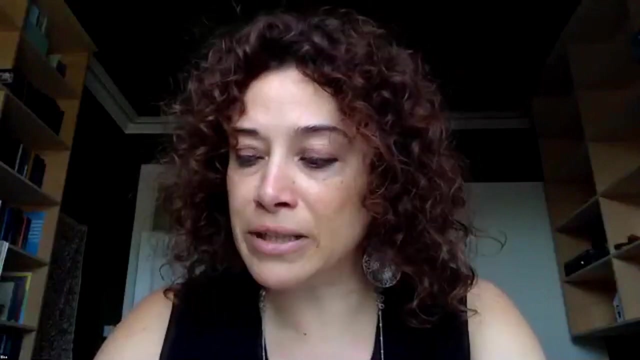 experience that Kari Sink will share with us speaks to the themes and the issues that she's been working on for quite a long while now. the other colleague that will be with us is Sean Rees. Sean is a senior research fellow at the School of Biological and Marine Sciences at Plymouth University in the 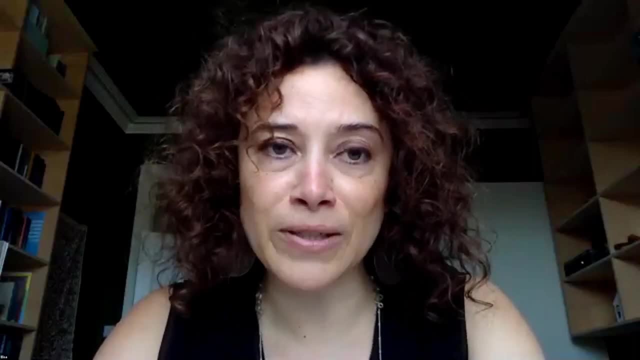 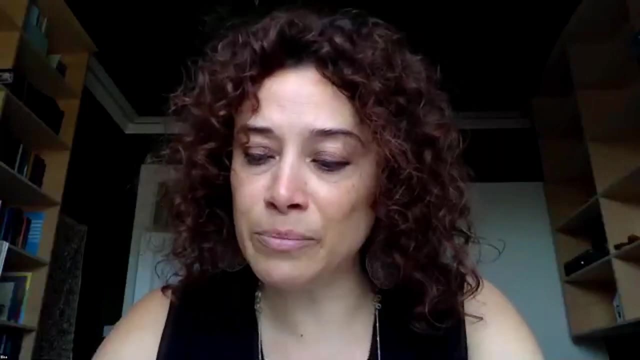 UK. she's done quite a lot of work at the Science Policy Interactive Association and also the research at the University of Canada in the United States, and she's also an expert in ecosystem services. and the third colleague that we're really privileged to have with us is Dr Dilan Meghari. he's 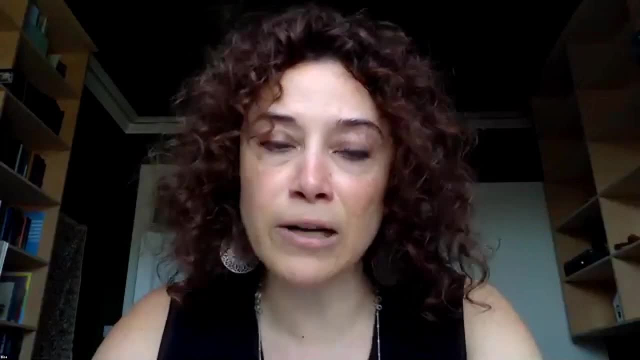 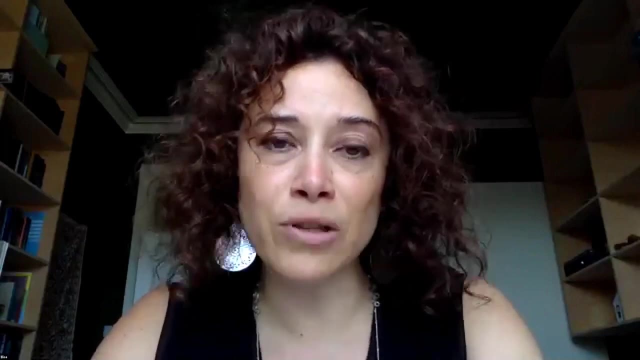 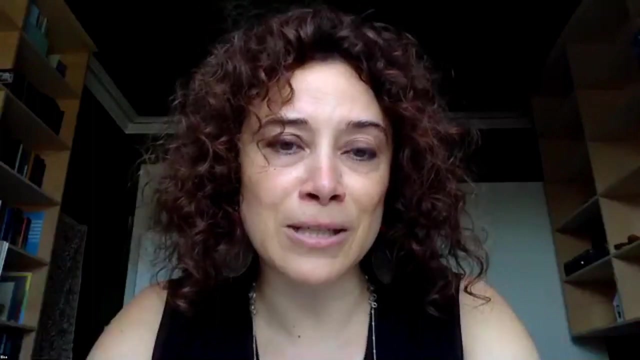 a senior researcher at the Environmental Learning Research Center at the University currently known as Rhodes University in South Africa. he's the director of the Institute of Uncanny Justice and one of the co-directors of the One Ocean Hub. so, without further ado, I'll leave the floor to Kira to. 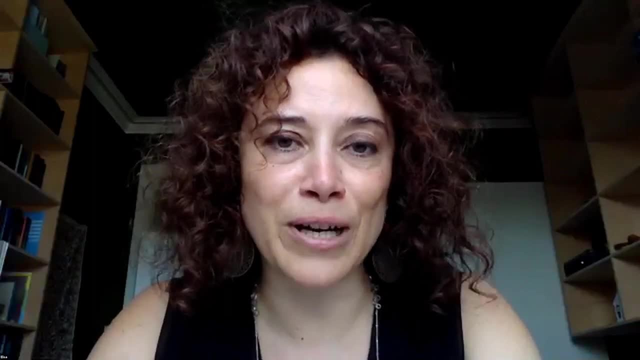 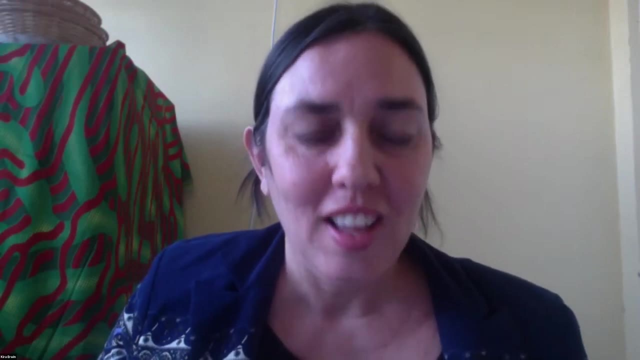 talk about her work today, and I'm very, very excited for her to take the floor very soon. hi everyone, so lovely to be here with you all, and I've got the honor of introducing Kari, and I'm gonna read it, because there's a lot to say about. 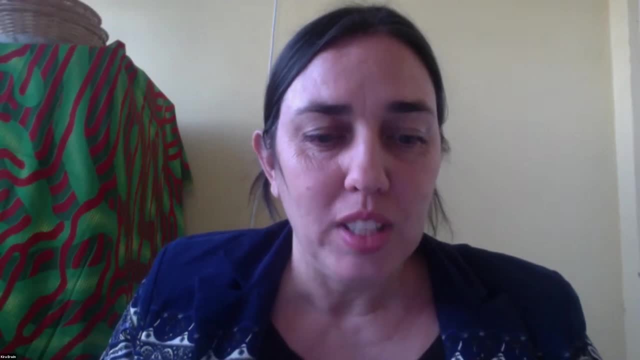 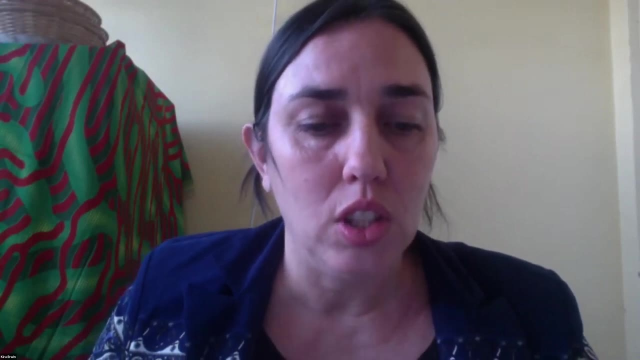 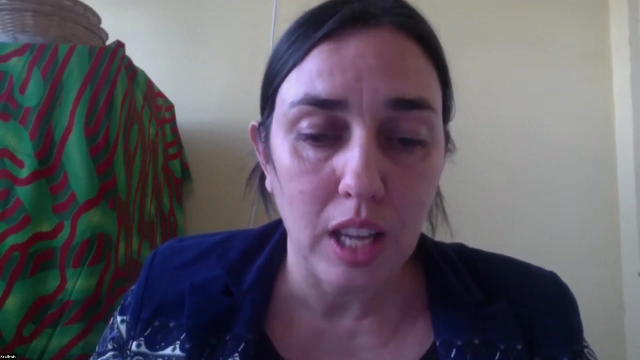 Kari Sink, and we're very privileged to have her with us today. Professor Kari Sink is a principal scientist at the South African National Biodiversity Institute and a research associate at Nelson Mandela University. she leads the national biodiversity assessment with a long term investment in the classification, description and mapping of marine. 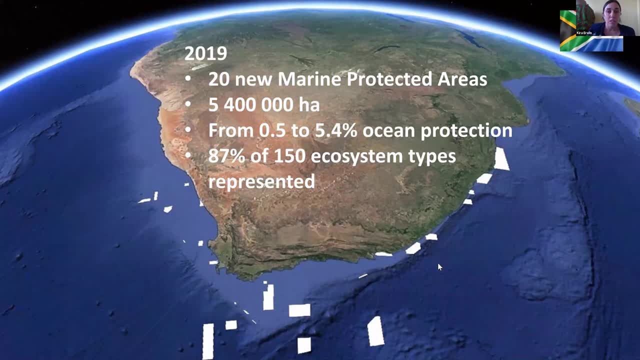 ecosystems. Kari's greatest investment- and you'll see the slide up on the screen- has been in supporting the establishment of a new network of marine protected areas in South Africa. she began this work in 2006 and 13 years later, in 2019, 20 new MPA's were declared, representing a tenfold increase. 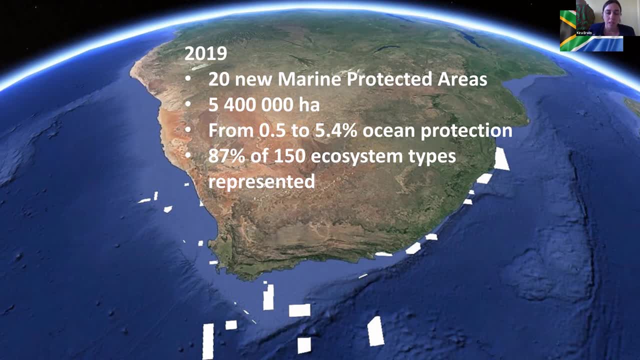 in South Africa's ocean space in a single step. Kerry was supported by the Pew Fellowship in Marine Conservation, and her work in this area has received a Distinguished Service Award from the Society for Conservation Biology. Kerry is very passionate about capacity building and development in marine science and management, both in South Africa and beyond. 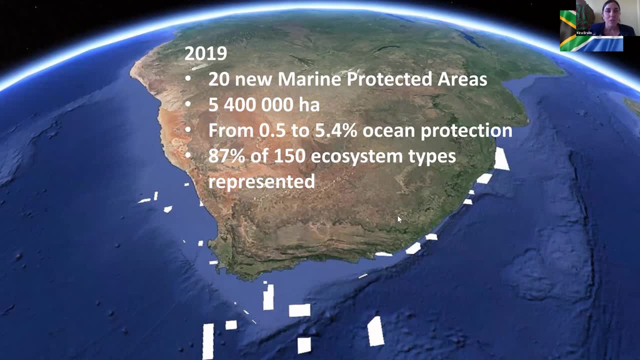 and we are very happy to have her with us today. I'm going to speak to you briefly after Kerry's presentation and then let the panellists give some reflection, and we will have time for questions and answers as well. So today, Kerry will take us on a journey. 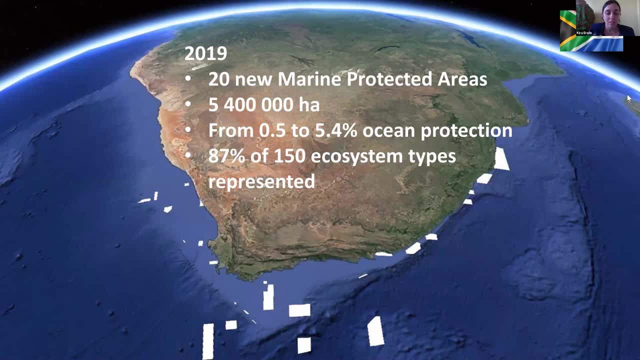 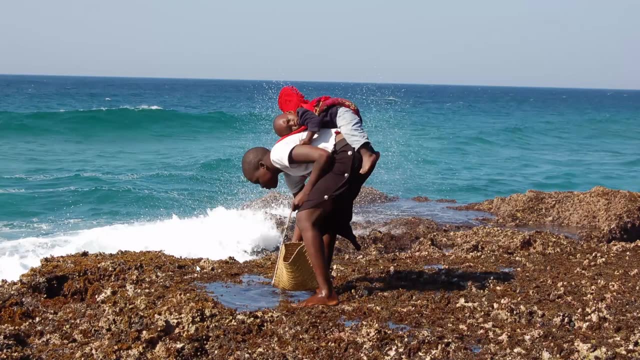 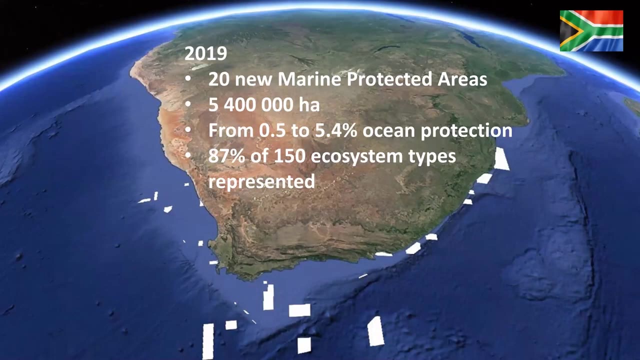 exploring some of the turning points in her personal and professional experience, a journey I'm very much looking forward to. So, Kerry, I'm handing over to you. Hi everyone, Apologies for the technical challenge. Thank you so much for inviting me to share my experiences today. 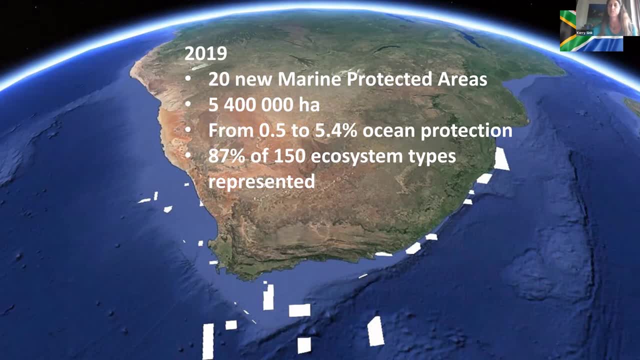 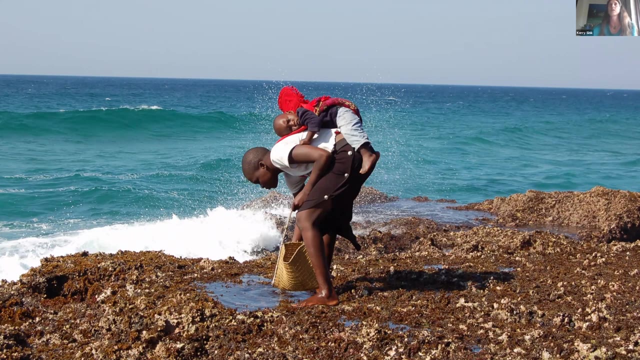 and the opportunity to reflect My personal journey has been a journey of increasing depth. I started my career on the rocky shores of northern KwaZulu-Natal and this is a really accessible ecosystem, and I got to study the patterns and dynamics between the different species, the different communities. 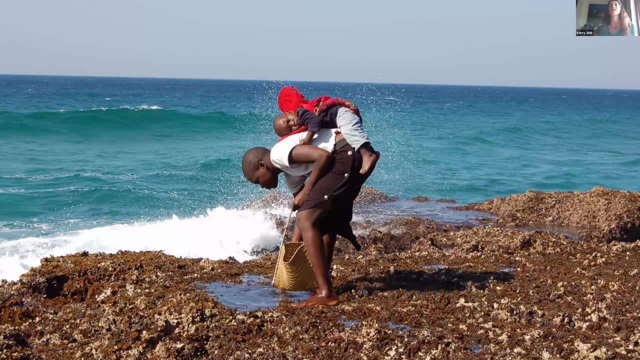 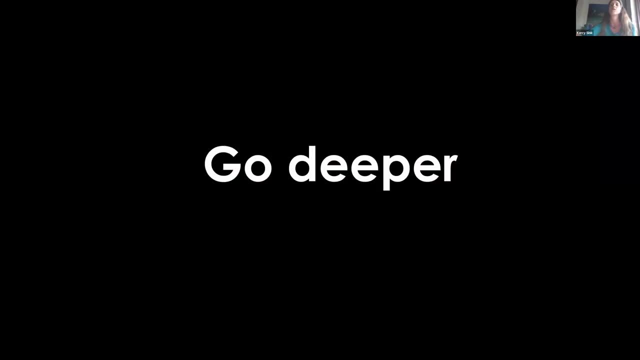 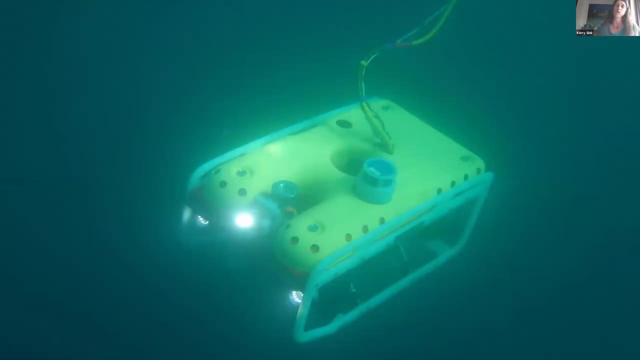 and also the human dependencies on these systems, laying a great environment, a great groundwork, before moving into a far more inaccessible environment. And it was really the discovery of a fish, and that fish is the coelacanth, a living population of coelacanths, many, many years later. 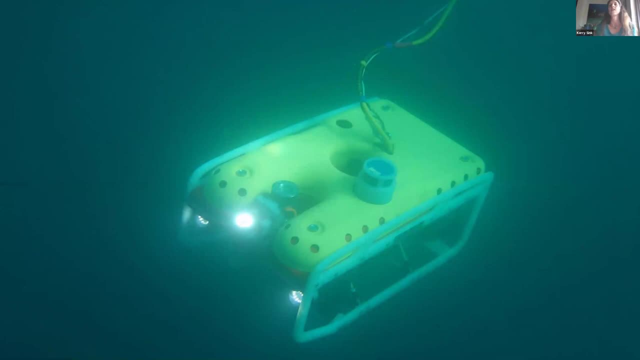 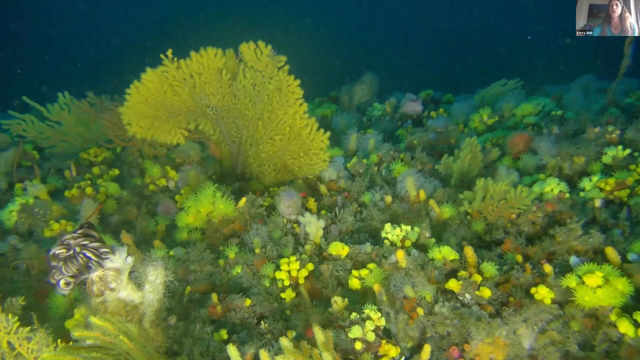 later, after they first became known to science. that enabled South Africa to move into deeper water, And we were able to hire a remotely operated vehicle like this, which allows you to take a walk on the sea floor, And it's an incredible privilege to experience these. 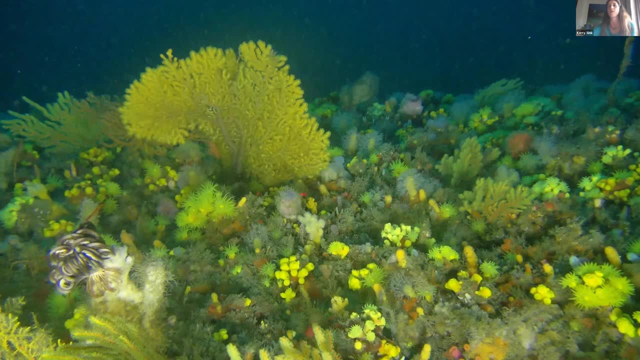 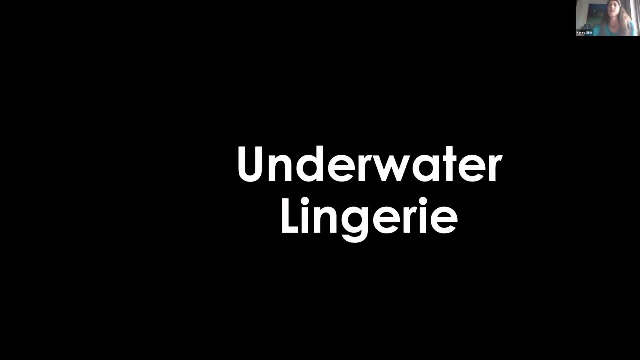 ecosystems. It's a unique opportunity to have these colors and shapes and this diversity revealed before your eyes. There's a lot of anticipation when you're going to go and explore an area for the very first time. In my case, I'd done years of work using computers and 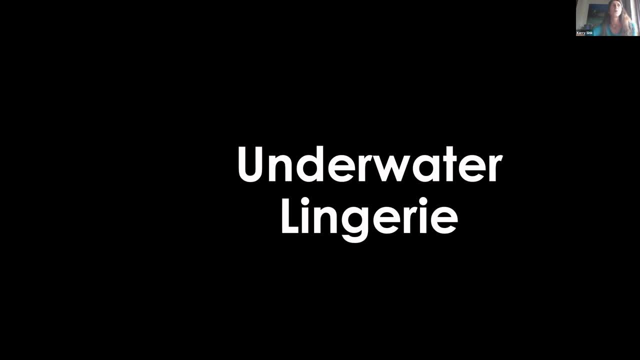 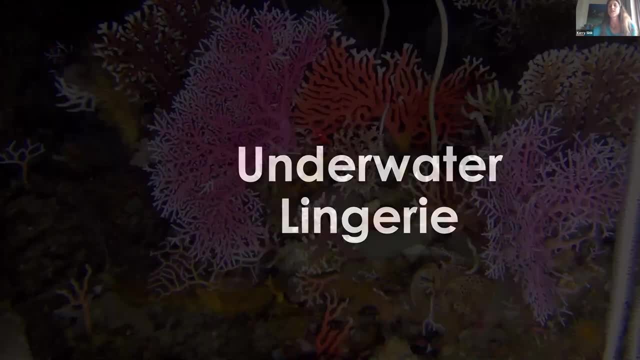 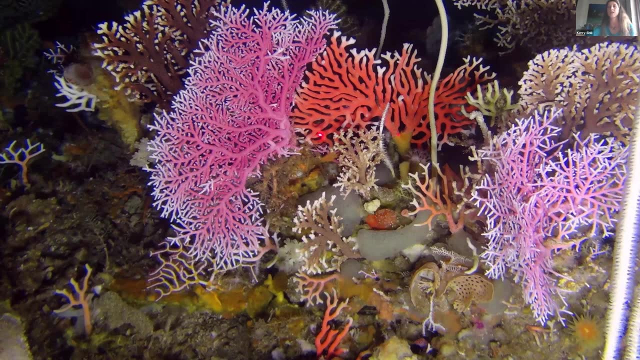 sent down this underwater trail And we sent down this underwater trail And we sent down this underwater robot. It's kind of like an underwater drone And the lights just lit up this entire forest of lace corals. And these lace corals are really very, very fragile And the beauty and fragility 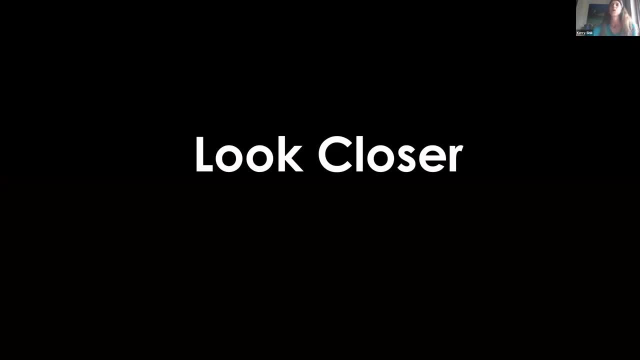 just blew me away. One of the special experiences I've had is to work with marine biologist Lisa Levin, And Lisa took the time and effort to come to sea with us in South Africa and work off shore and help us learn, And one of the things she did was to teach us to look more closely, And so 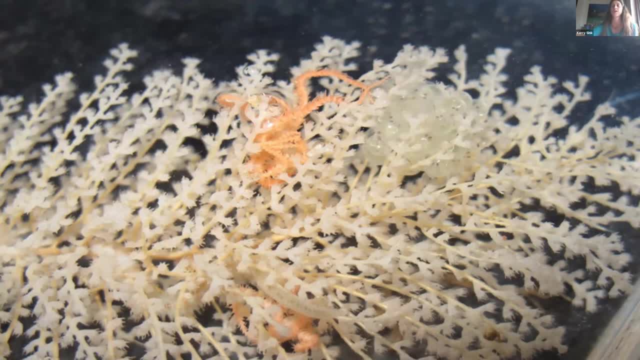 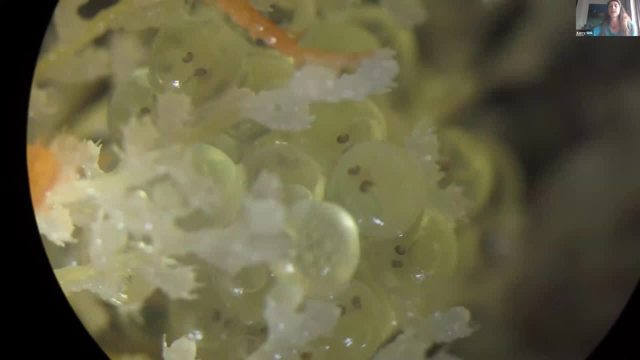 she showed us by collecting soft corals in our deep water, not just the brittle stars and the worms in them, but the eyes of future fish. It's one thing to read a scientific paper about the role of coral habitats as nursery areas, but it's another thing to really experience that by looking down a microscope and seeing the 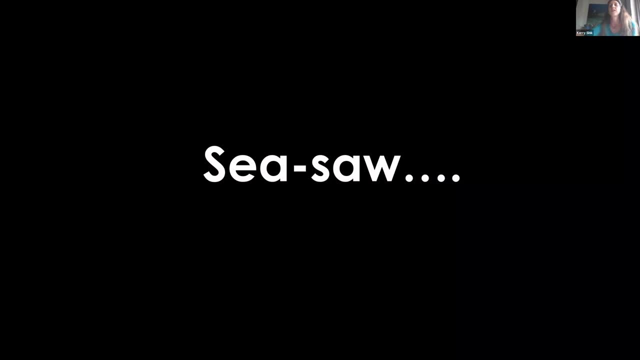 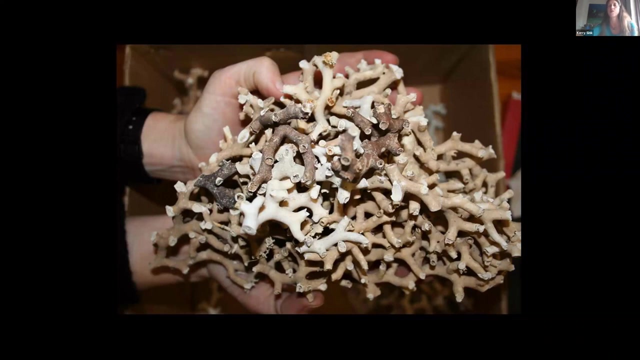 eggs in the arms of a soft coral. Offshore work has its high points and low points, And one of the greatest kind of seesaw moments I had was going from first discovering, very accidentally, cold water corals in South Africa's museum Walking through the worm section of the museum. these corals caught my eye because I used to work on shallow corals. 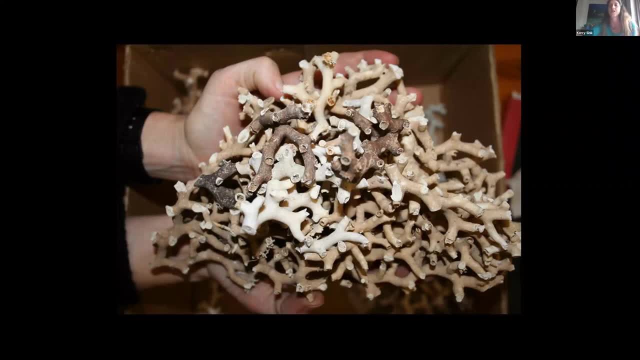 And I picked them up and on the label they had come from 970 meters And I had read a lot about deep cold water coral communities in the in the northern hemisphere, but I didn't imagine that we had these complex three dimensional structures inside South Africa's waters. 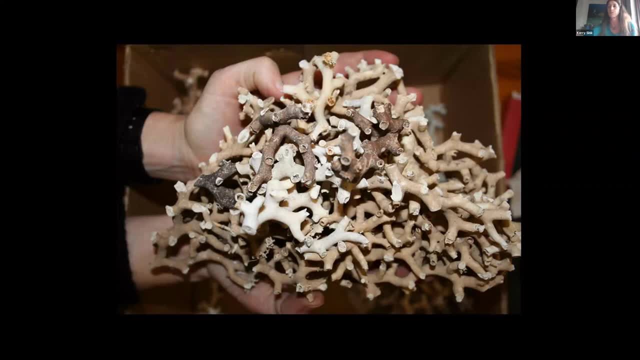 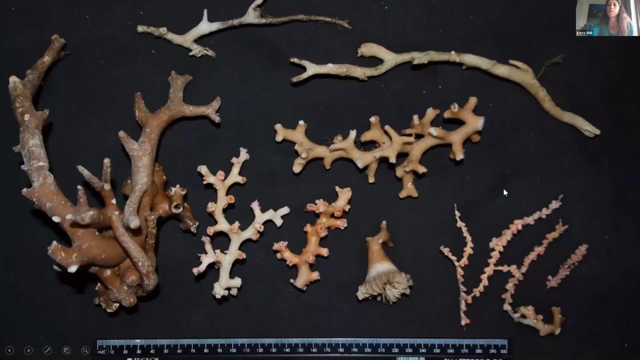 So I was really excited to go and learn more. We sampled these habitats. Sorry, We sampled these habitats. Let me just admit all I dredge from 900 meters, but South Africa doesn't yet have the capacity to work below 700 meters with visual work. 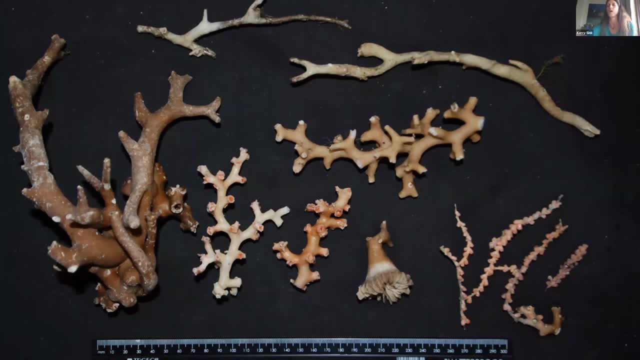 But in 2016, I got the opportunity to work in one of our first proposed coral reserves at a museum in South Africa- at a museum in South Africa, And I had a depth of 300 meters and I was so excited for that experience. 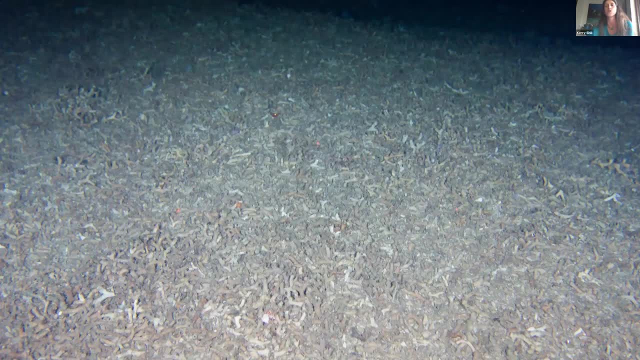 Like what am I going to see? But what we found was that this complex three dimensional structure of the corals had been broken down into a field of coral rubble. Now, the most likely reason for this is trolling, but we can't rule out climate change, because cold water corals are very sensitive to ocean warming, deoxygenation and ocean acidification. But what we found was that this complex three dimensional structure of the corals had been broken down into a field of coral rubble. Now, the most likely reason for this is trolling, but we can't rule out climate change, because cold water corals are very sensitive to ocean warming, deoxygenation and ocean acidification. 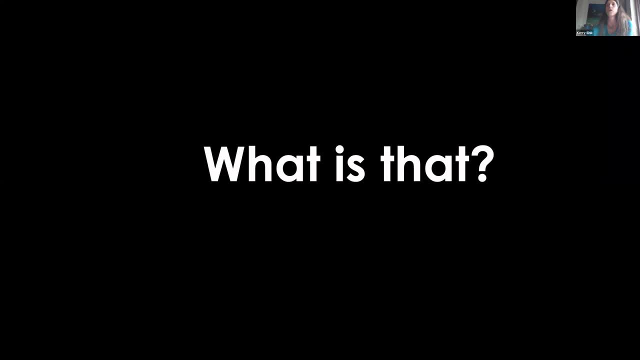 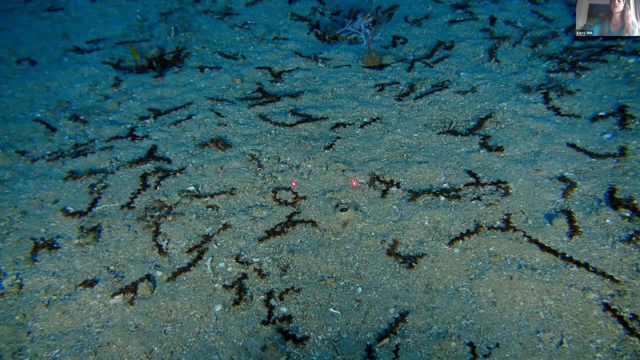 So you know, just like I said, we don't know what killed the coral, And we we always encounter new mysteries. One of my favorite ones was this species. So this is a species of what we call foraminiferans, And it's basically like an armored amoeba, a very simple, single-celled animal that can secrete a shell. 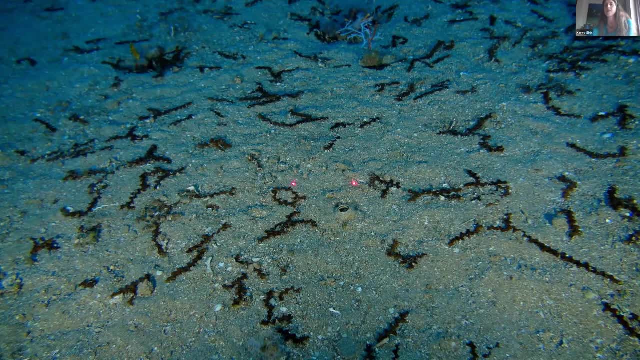 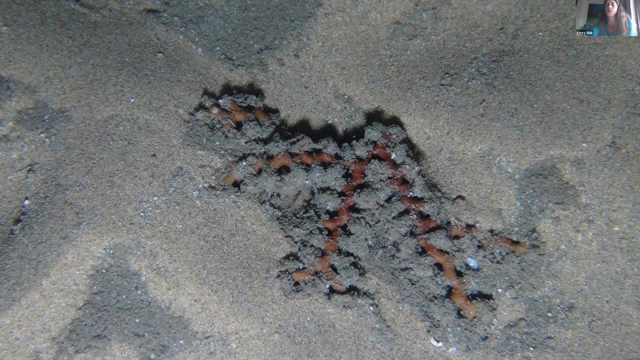 These are some of the largest ones in the world, And imagine this, Amazingly. when I worked to identify this species, I had help from a guy who works on seashells, and this species is actually recorded as extinct. but what you can see here, it's very much actively processing the sediment and particulate organic matter and indeed these species have shown to be important in cycling nutrients on the seafloor. 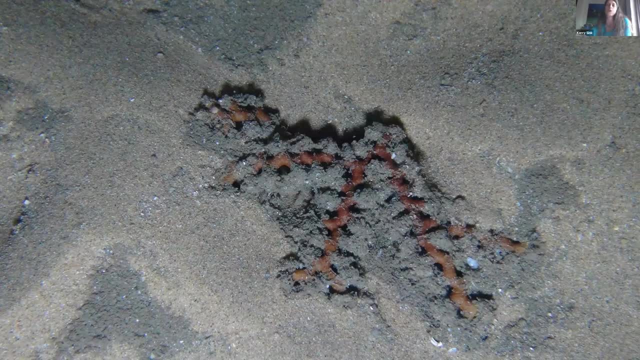 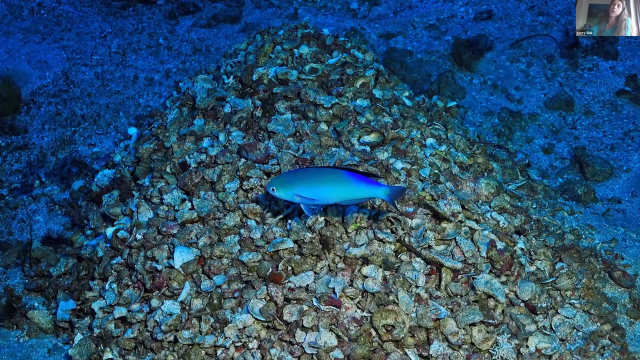 They play a key role in the carbon cycle. Another mystery was these mounds of shell, grits and coral that I was seeing on the shelf edge in the Isamangaliso Marine Protected Area. I was so excited about our coelacanth discovery that I took up mixed gas diving and in our explorations we'd see these mounds and all the divers would ask me, the marine biologists in the group, what makes the mounds? 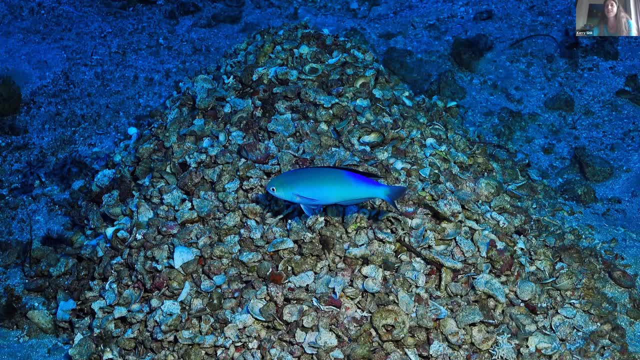 And it took us nine years to find out that this little fish, it's a tilefish. it actually goes and fetches each little piece of coral rubble and builds a home and then normally, especially if you approach with an ROV or a submarine or something noisy, it ducks into its home. 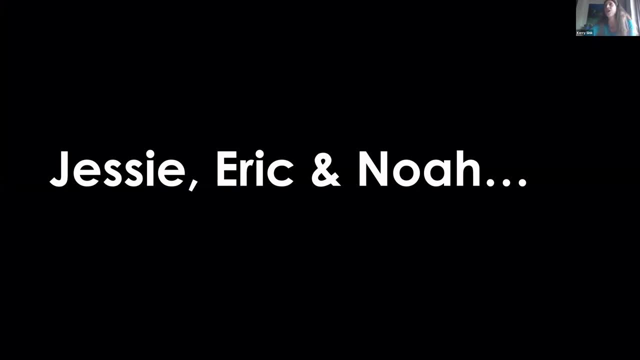 I find the biology of fish is completely fascinating. It's a couple of fish, a couple of individuals. These are individual fish that I've actually had the privilege of studying for a long time that have given me the deepest insights. Jessie is the first coelacanth that was known to divers from Sedwana Bay. 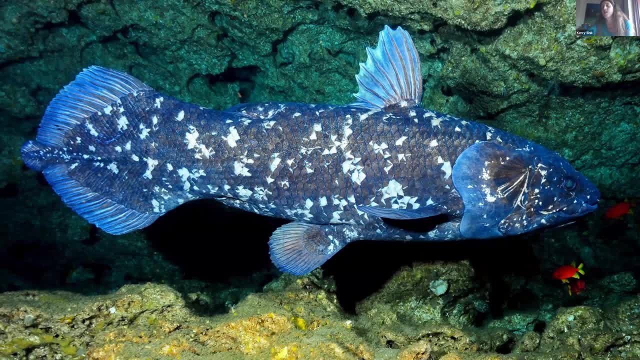 She was discovered in the year 2000,. and for these 20 years I've tracked these individual fish. We have 34 individuals. This one here is actually Noah, recognized by the arc on his side. I try to give them names so that when I see them I'll recognize them immediately. 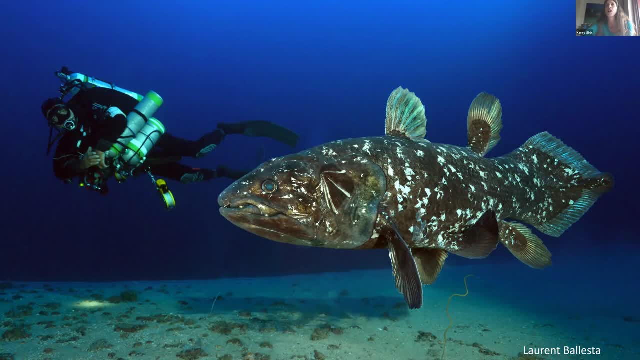 This is Eric Eyelashes, and Eric Eyelashes gave me an incredible peek into his life because we managed to tag this fish. The brave divers put a tag on this fish that stayed for nine months, attached to Eric popping up nine months later, and then, by satellite, we got minute-by-minute log of the depth of Eric Eyelashes. 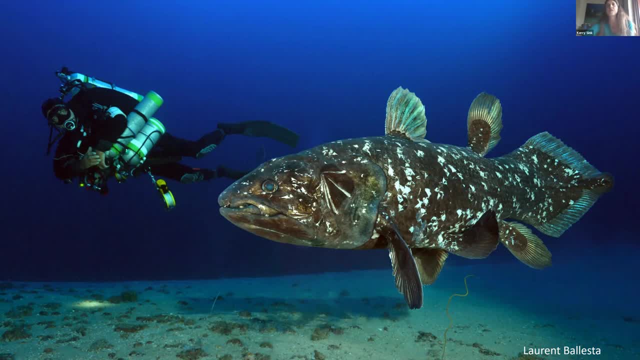 And I got to know that pretty regularly he comes out of his cave. we think, Yeah, We can't see what he's doing, but we think it's a cave because it's at a depth where we know there's a cave where he spends a lot of time. 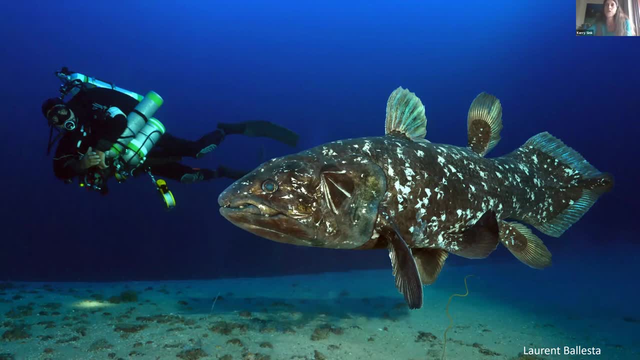 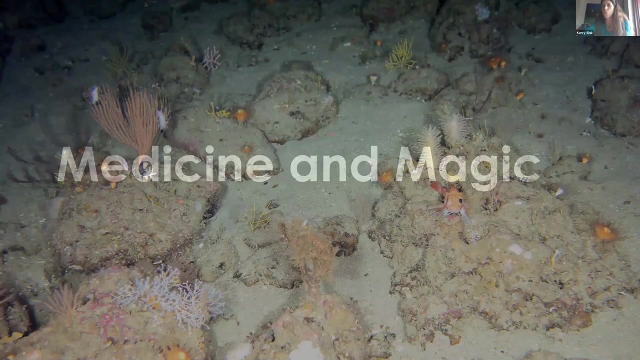 Out of the cave and then travels up and down as shallow as 70 meters and as deep as 400 meters, returning at dawn to have a steady time and then every evening, going about his business. One of the animals that was even harder to find than a coelacanth was this gelatinous necromancer. 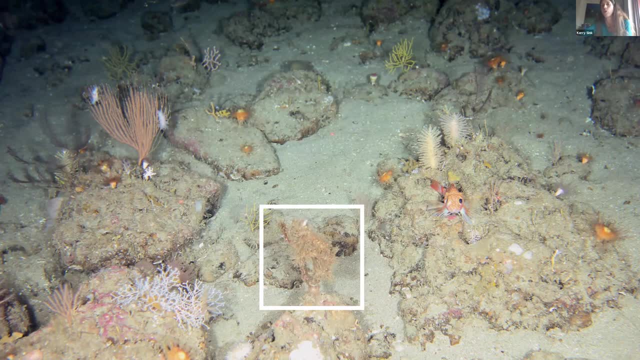 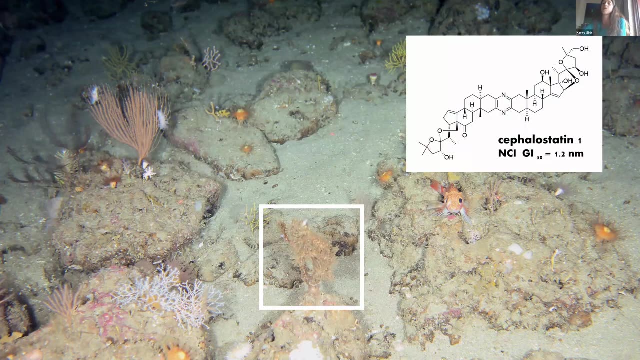 This is an acorn worm or hemichordate, and it's famous because it's been found to have a compound that's amongst the most potent compounds ever tested against cancer. The thing is that when this animal made it into publications by chemists, they reported that they had collected it by scuba diving. 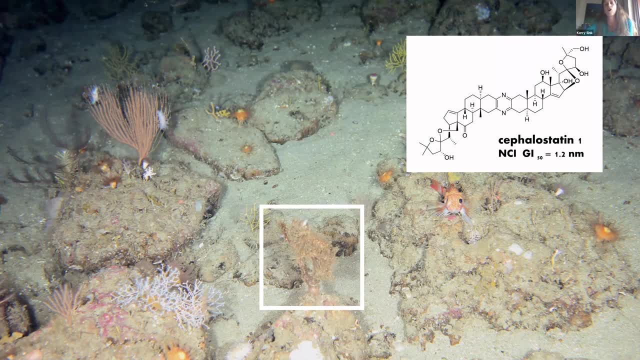 So for years and years, we had been looking in the wrong place to find this animal, And it's only recently been revealed that this species lives only in the South African deep sea, as far as we know, And it's our sole responsibility to look after it. 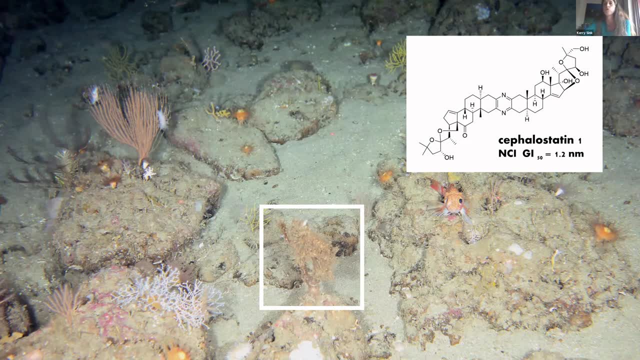 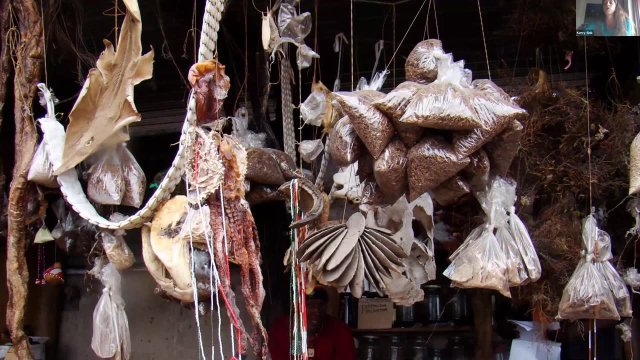 And we're really excited about this discovery now because we can move forward with drug discovery. One of the more interesting surprises I had was actually made on the shore, And that's when I was walking through what we call a mooty market. That's a market where plants and animals are sold for use in traditional medicine and ritual. 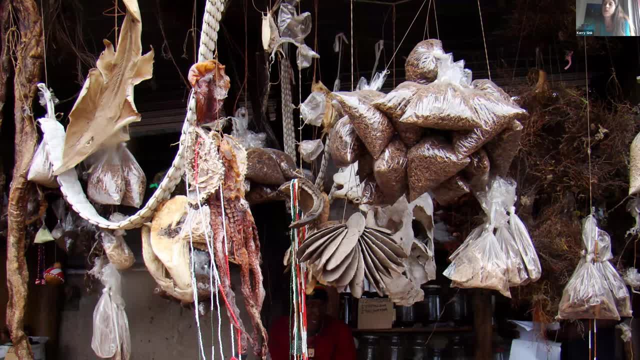 And I was amazed to find that the eye patch species from our prawn trawl fishery were being collected by deckhands and sold for use in traditional medicine and magic. This was certainly not a group of stakeholders who I had consulted in deciding and working towards marine protected areas. 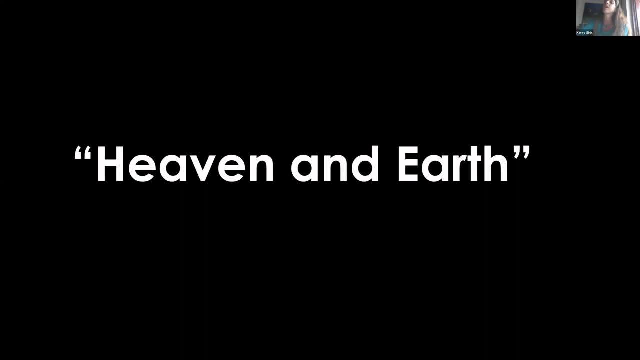 This was certainly not a group of stakeholders who I had consulted in deciding and working towards marine protected areas. One of the groups of stakeholders who took the most time from me, and indeed taught me the most lessons, were the offshore oil and gas industry. 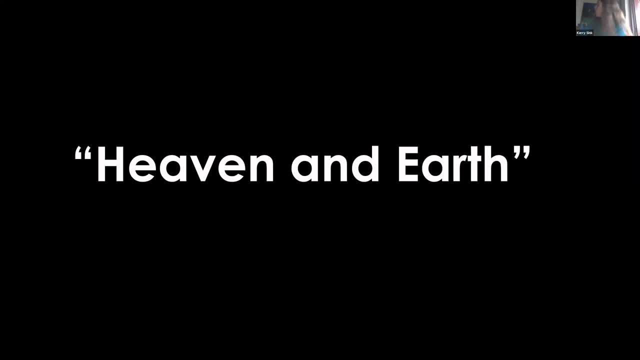 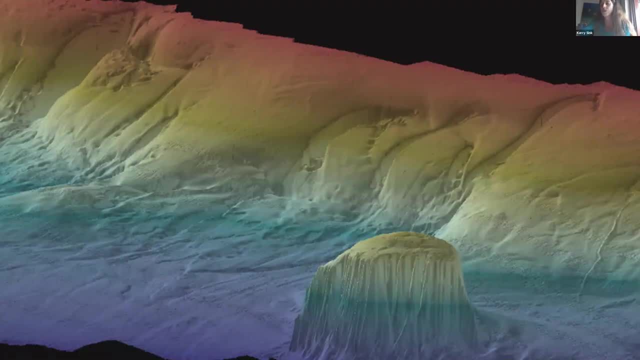 One of the groups of stakeholders who took the most time from me, and indeed taught me the most lessons, were the offshore oil and gas industry. This picture was made possible by a data set collected by one of the petroleum companies. it's called Mount Merrick. 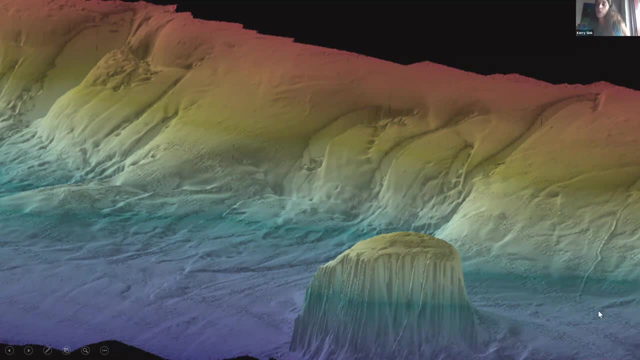 And we're hoping to visit this feature for the first time, But I do really want to thank you all for your patience. Thank you time. So this is a future moment that I'm really looking forward to on the One Ocean Hub cruise. 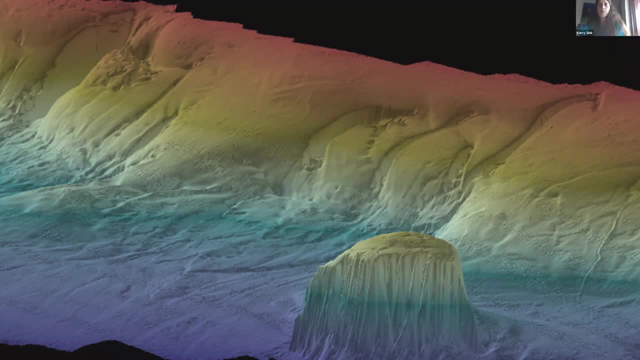 So you can see the seamount and you can see these incredible submarine canyons that can slide into our western margin. And the relationships with oil and gas are important because a scientist like myself and the geoscientists of the country can only dream of the resources. 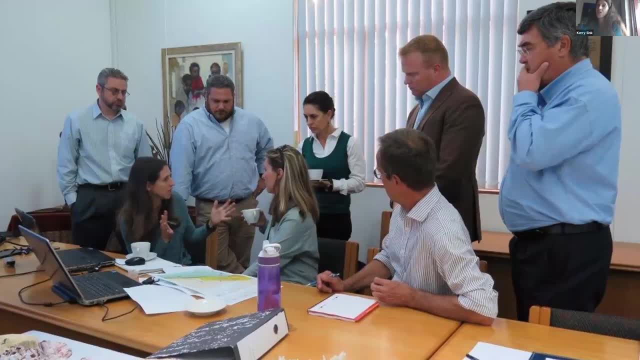 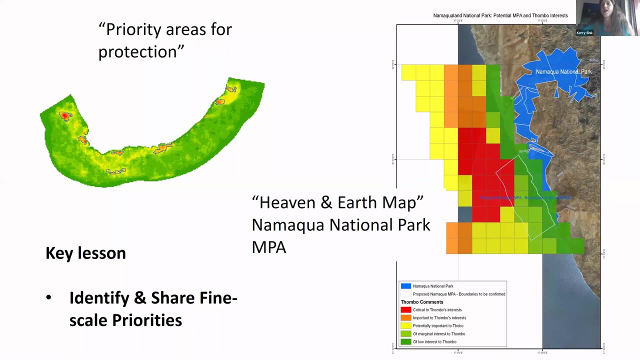 to collect such a data set. These negotiations, however, are not easy. All the women in this group are from the Marine Protected Area team, and the men are from three different petroleum companies. The particular moment that stands out for me was a moment when I was visited by a team. 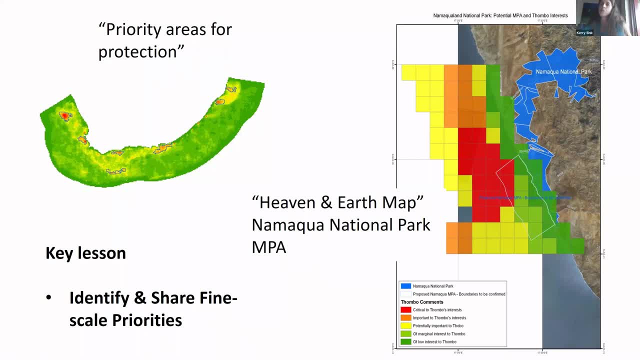 of petroleum executives discussing the proposed Namakwa Land Marine Protected Area, first identified for protection in South Africa. when I was four years old, The executive walked into the room and unfurled his map And he started his sentence with the words right. And I knew that something was going to happen. And he said to me: you've. 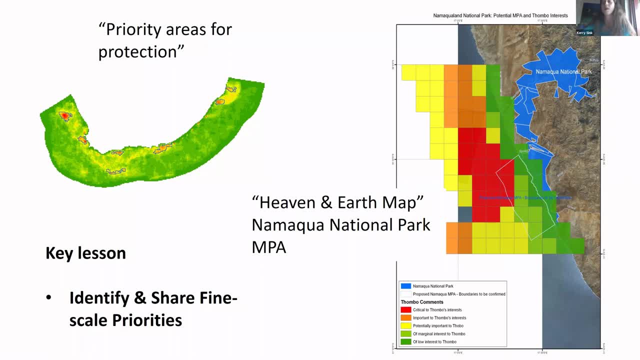 got your biodiversity area map and now we have our map And he said: I'm calling this the heaven and earth map And basically the green area, we don't care if you try to put a protected area there, But the red area will move heaven and earth. to stop you Discussing this with my husband, 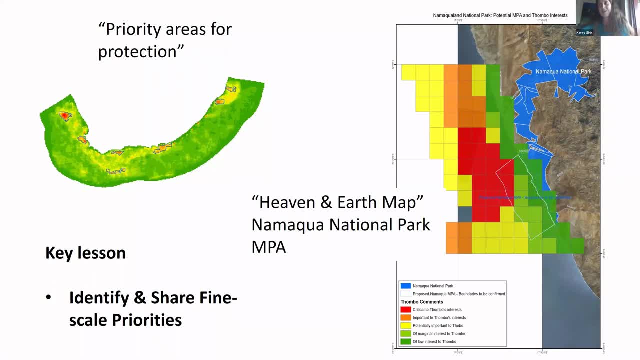 over dinner that evening we agreed that this was a little bit intimidating, But I explained to him that the critical thing was that we had finally reached the point where we had the fine scale sharing of priorities, And this unlocked four decades of negotiation for protected area establishment. The day that, I think, I really felt the full. 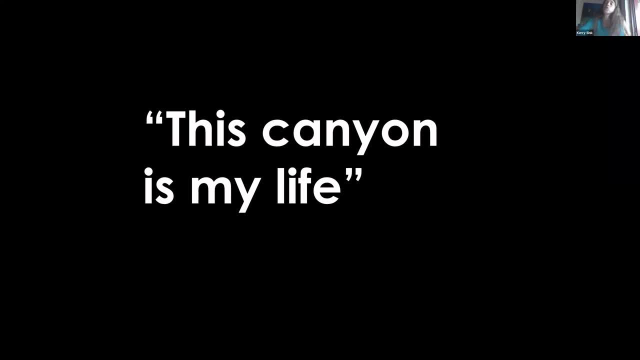 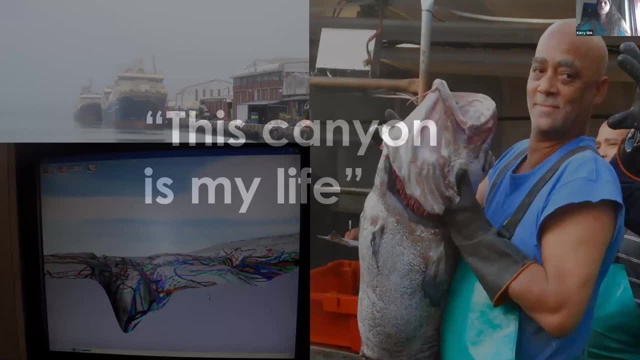 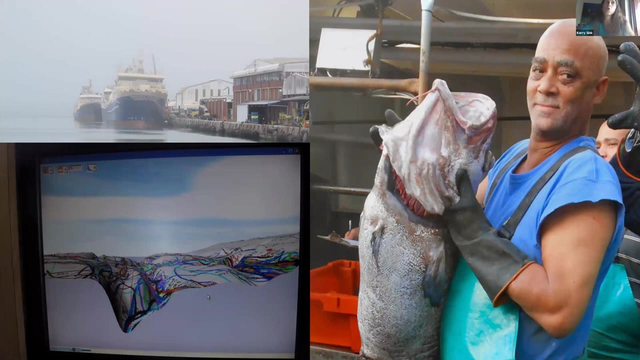 weight of the implications of some of the work that we do in terms of impacts on fishermen was a very misty morning in Saldana Bay on our west coast, And there I went aboard a vessel, very large trawler, that does a lot of fishing in the Cape Canyon area. I was 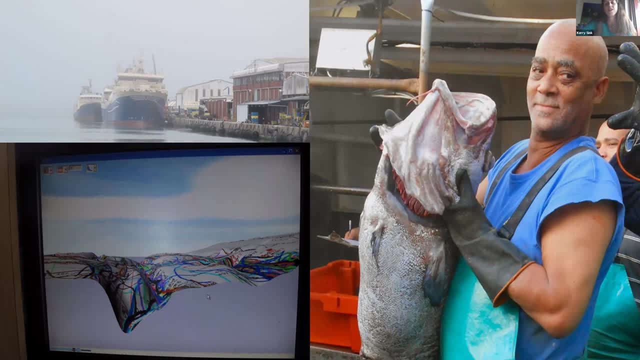 trying to work out how do we protect the most sensitive part of the canyon head while having the least impact on the environment. And I got into a dilemma, which is: well, what does it mean to be protected? Well, that's a tough question, The reason being that I was 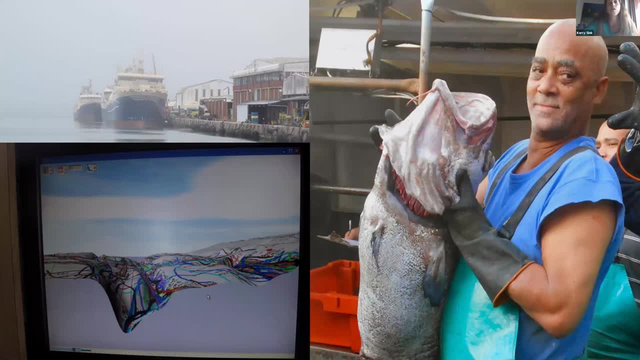 on the fishermen who depend on that productive area, and so we were sharing tracks. but there was just this moment of quiet when, when the captain of this vessel turned to me and he had these piercing blue green eyes and he said to me, Kerry, this canyon is my life. 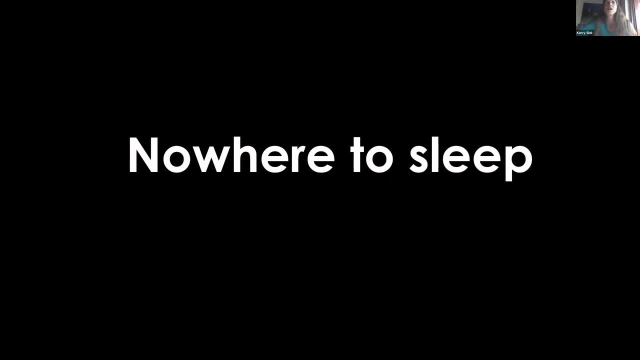 sometimes, in the difficult moments, we turn to our children for inspiration. and when I first had to leave my son to go to sea, he was just three years old. I explained to him that I wouldn't be there to tuck him in that night and for many nights to come, and why and what I was doing, and with the wisdom 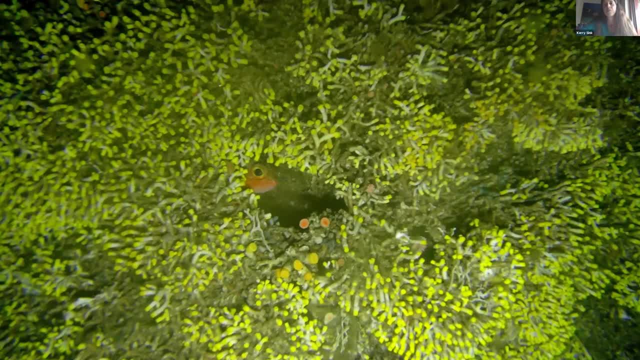 of three-year-olds. he looked at me and he said to me, Kerry, what's the one thing you want me to do? and I said, Okay, I want to go to sea. and I said, Ok, bye. And he said, mommy, that's good, because if you don't look after the seabed, the fish will have nowhere to sleep. 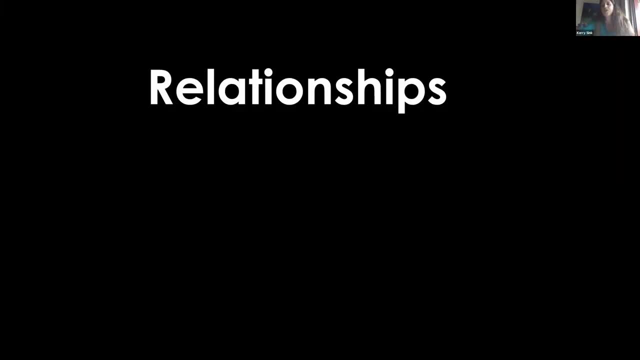 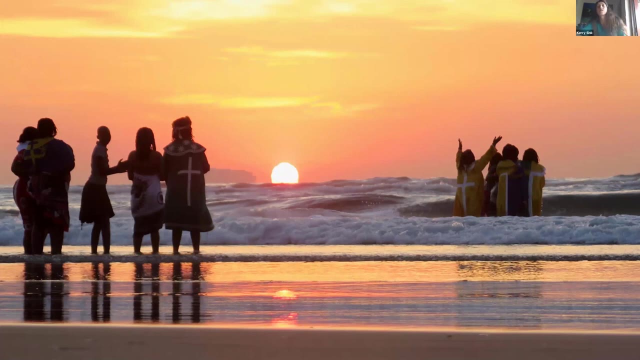 So I'd really like to thank you for the reflections and the reflective opportunity that putting this talk together has given me over the last 13 years, And I think that one of my key reflections is really that we need more than science. We need to have a deep appreciation of human dependencies and of all the connections, including the spiritual and emotional connections, that we have with the ocean. 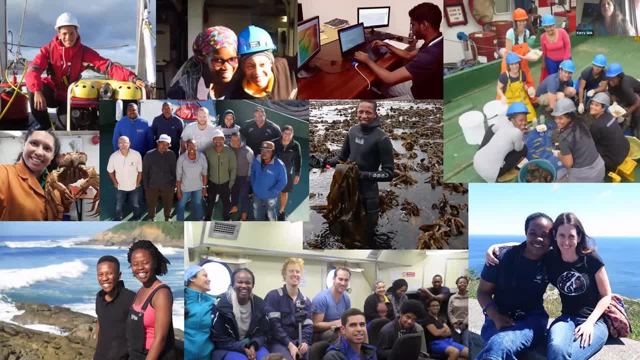 But we also need more science. And, in closing, I'd really like to thank all of my collaborators and all of my staff, Students, And also all of my stakeholders for sharing this journey with me and for the lessons. Thank you, Kerry. thank you so much. 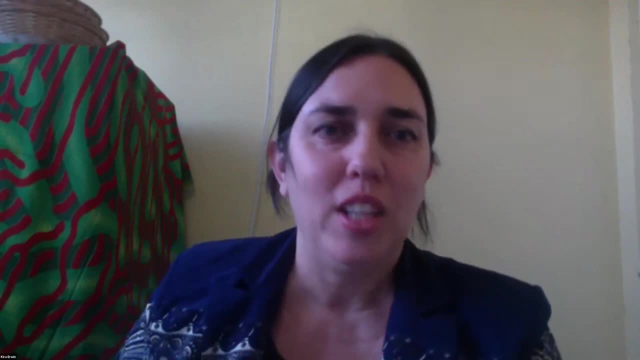 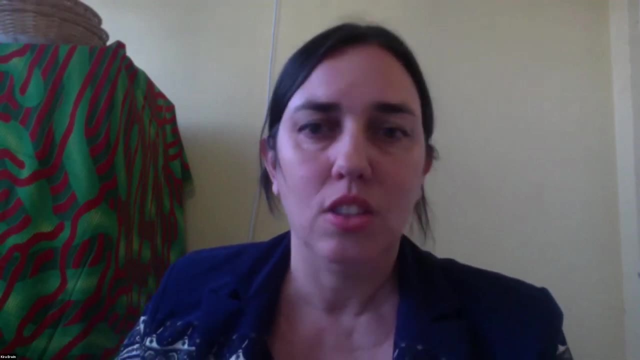 Sure, Incredible. We need more science and we need more than science. I'm going to ask everyone, if you don't mind, just to take 30 seconds, so just half a minute, just to reflect on the images, the stories that Kerry shared. 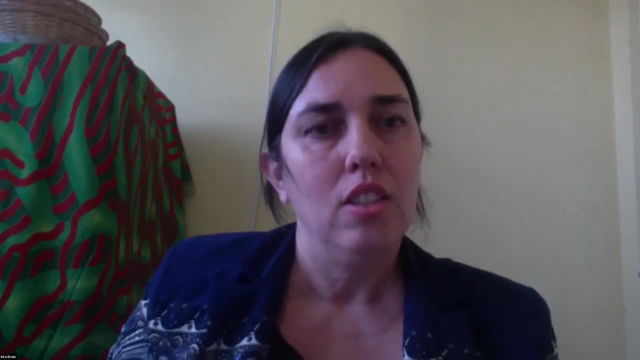 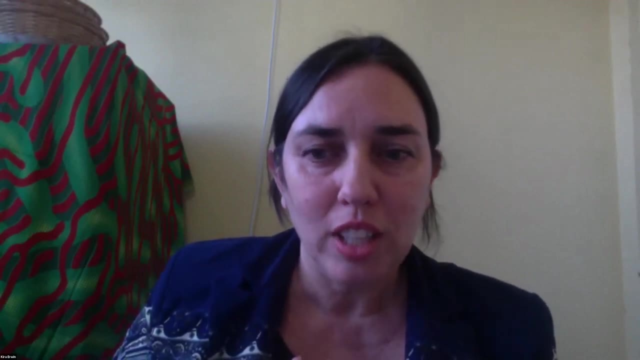 And if you could, in the chat, just type a few words that immediately come to mind, If I could ask you not to send it straight away, if you don't mind, but to hold it, And in 30 seconds I'm going to ask us all to share. 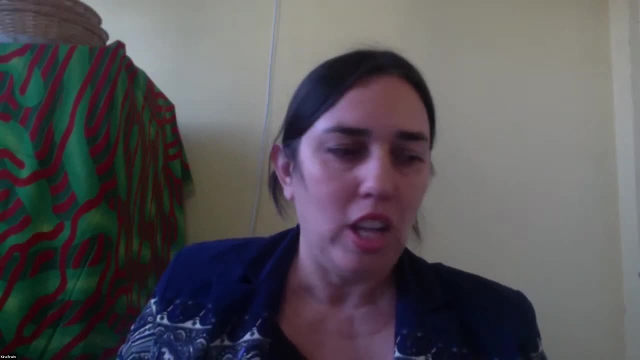 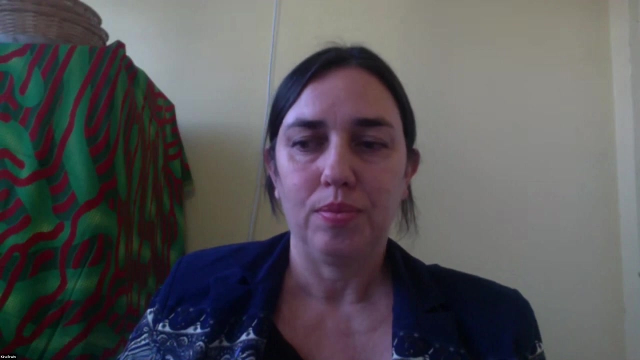 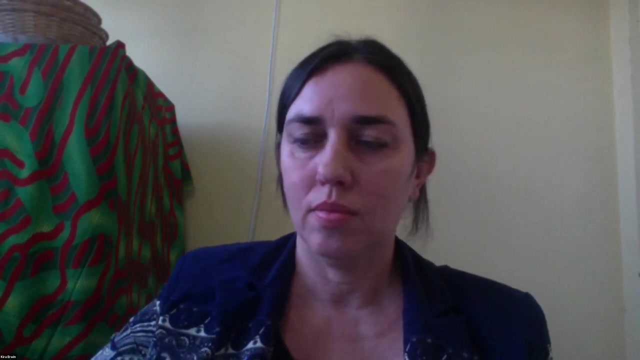 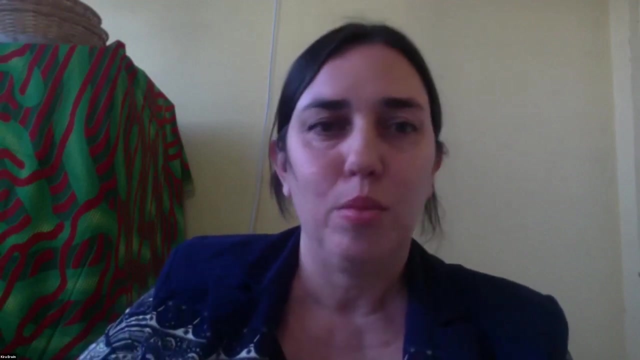 So take a moment to reflect And then, in the chat, just a few words on your immediate reactions to the talk, please. And if you've got your responses, please do so in the chat. If you've got your responses ready, if you could press send. we'd love to see what they are in the chat please. 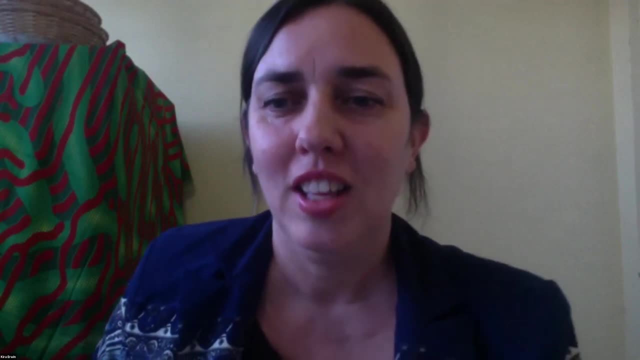 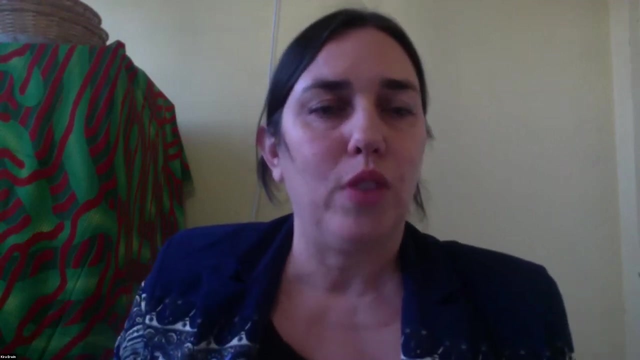 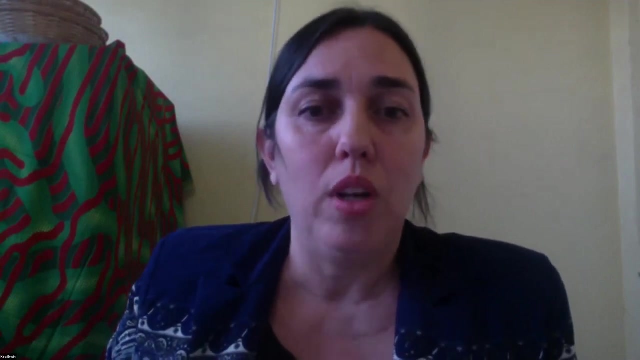 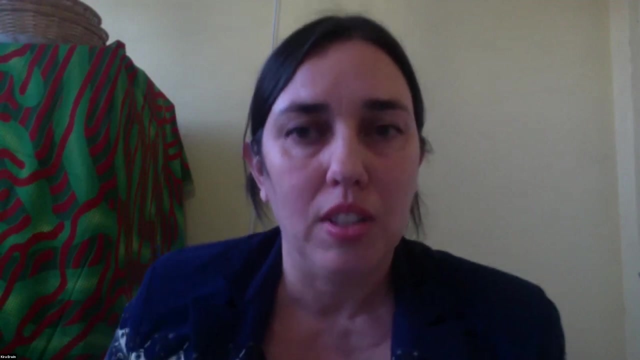 Oh, fantastic. There's some lovely responses coming through And I think, Kerry, that the power of storytelling using both photos and experience is really important to think about when we think about ocean governance and what it means to work in this area, And I just wanted to share with you one of the moments when I've seen your presentation around how powerful maps are and the mapping of our ocean, and what an incredible tool it is to help us both negotiate for protection. 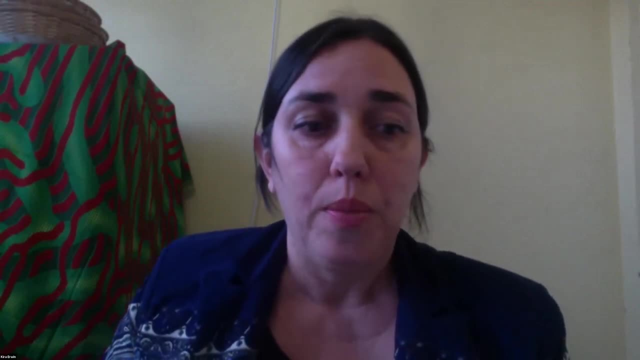 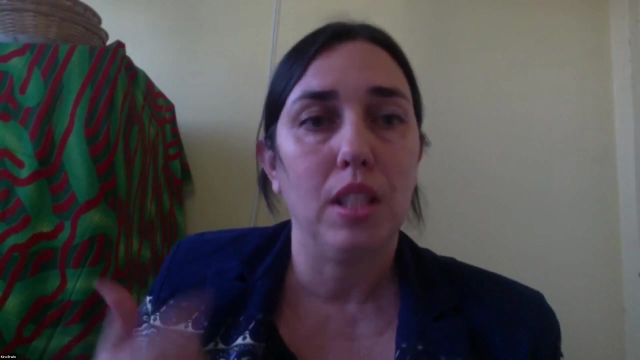 And also for resources. But your point too, about who are the people around the table who either have the resources to create these sorts of maps and the technology to create these maps, and which people are not sitting around the table and which kind of meanings of the ocean are not mapped. 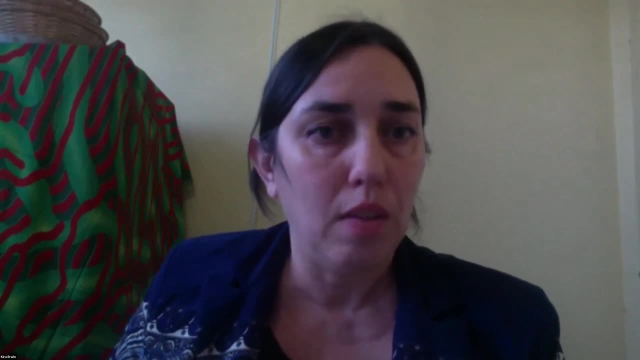 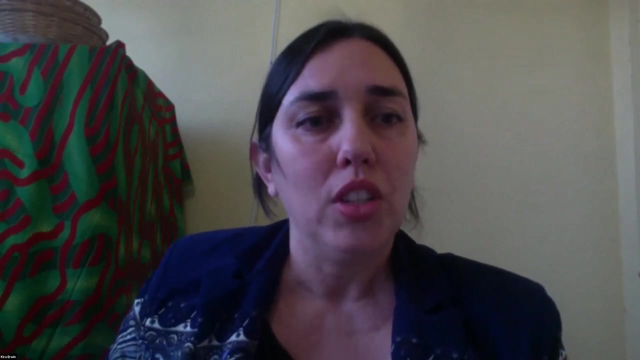 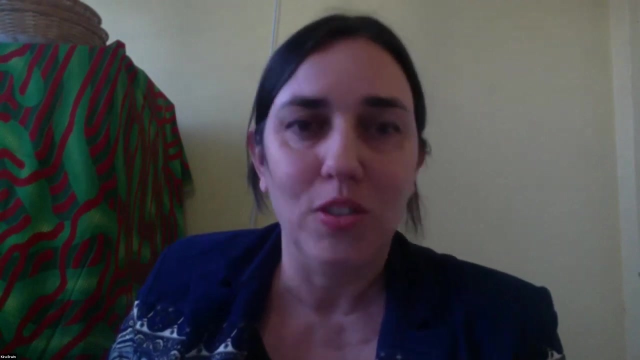 So how do cultural and social and economic livelihood meanings get mapped into these spaces as well is really really important. I'm going to hand over. I'm going to hand over briefly and thank you, keep your comments coming. they really useful to see. I'm going to hand over to Sean and just to get her reflections on what it's like to listen to Kerry's stories. Sean over to you. 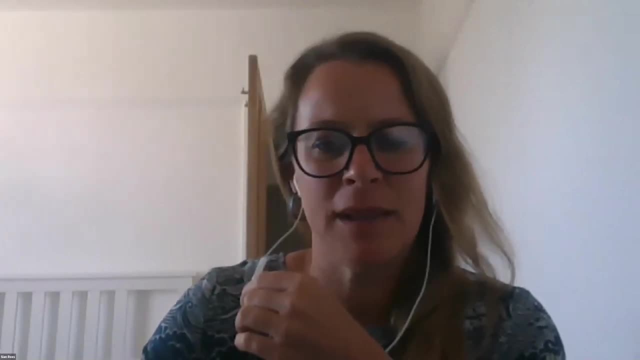 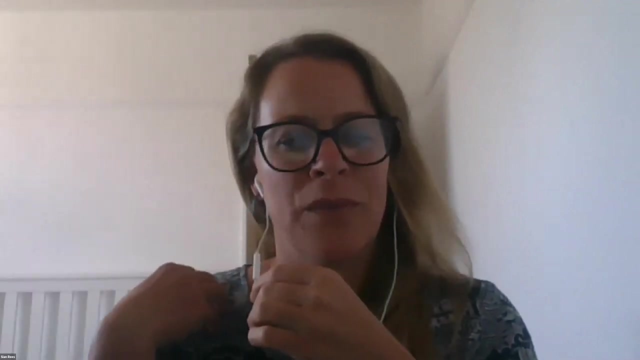 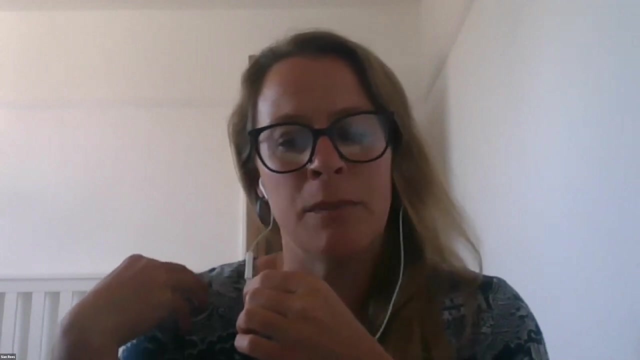 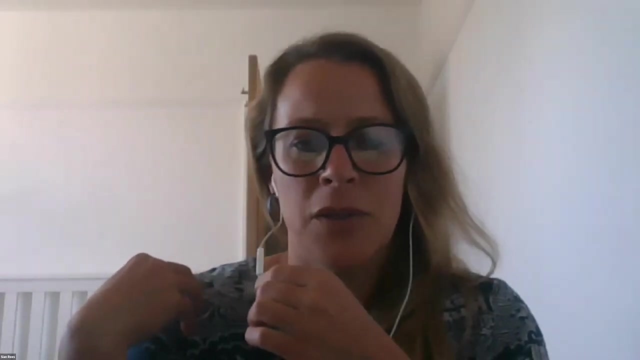 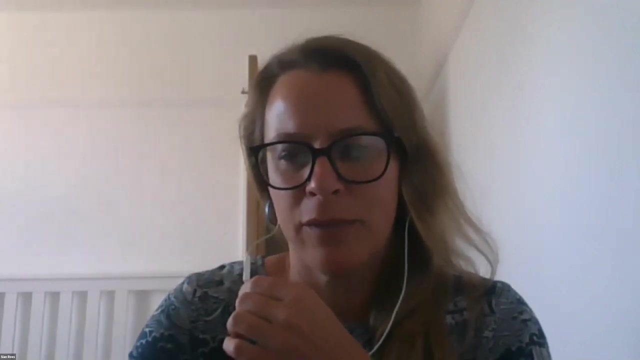 Great, thank you. Well it's been. it's been fascinating learning about Kerry's story And my first reflection is that for natural scientists- and many of the natural scientists I work with- I work with I work in a biology department at the university- is that much of science is linked to discovery and wonder and the majesty. and for me, as a social scientist and economist, I too I'm really amazed by these discoveries. and then, from my perspective, when I look more closely- as Kerry describes this need to look more closely into your own science, I start to wonder what they do. 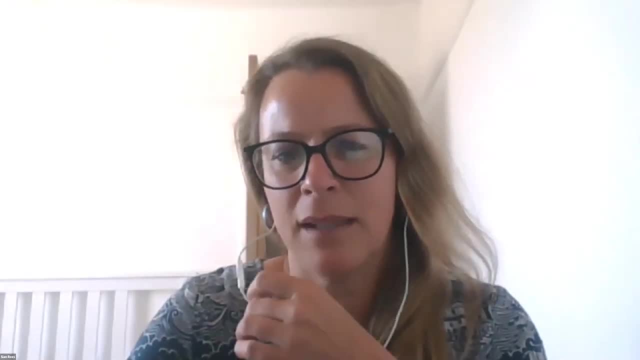 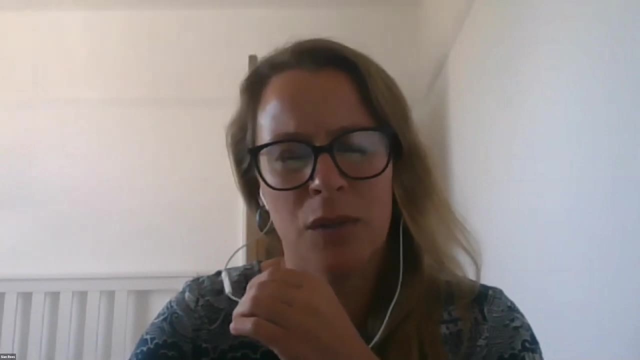 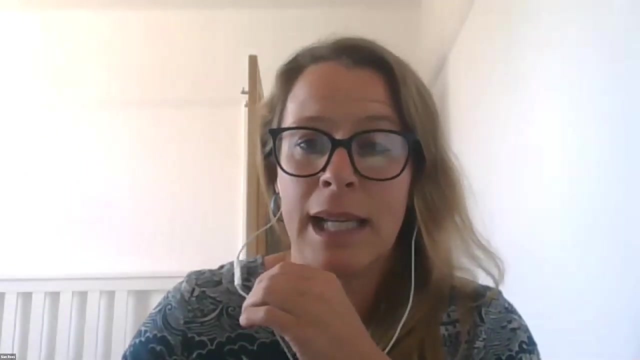 And then I think about how do these ecosystems then cross over with the humans Product, Mhm, and then why do they matter? And quite often when I look around the room of stakeholders I think to myself: What's that funk that's going to make those people feel that a notion ecosystem actually matters to them? why should they care? 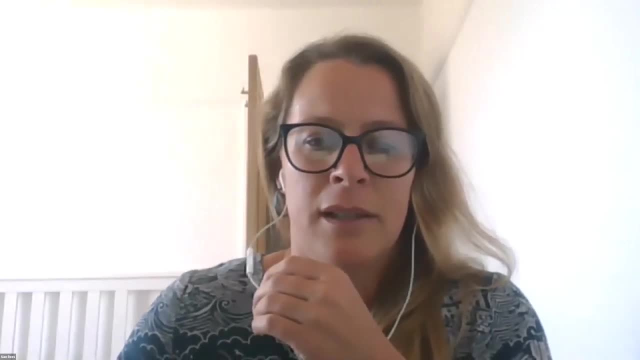 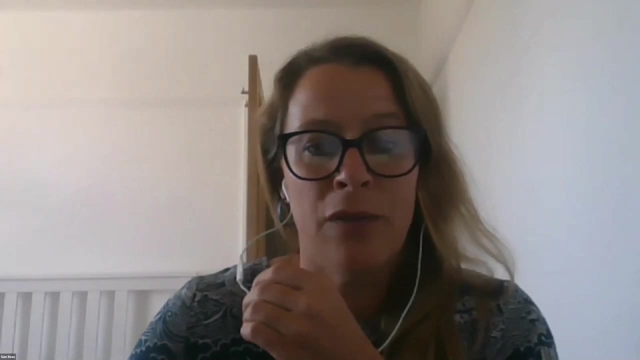 So Kerry showed us the the mosaic interaction between the living and the non living components of the ecosystem, That they function to support these flows of ecosystem services. There's l yapting of them livelihoods, and by ecosystem services I mean those benefits that humans derive. 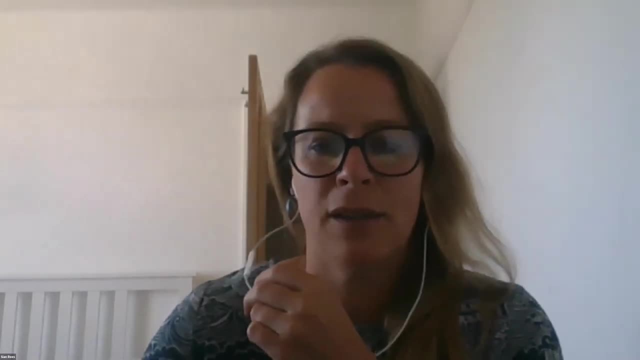 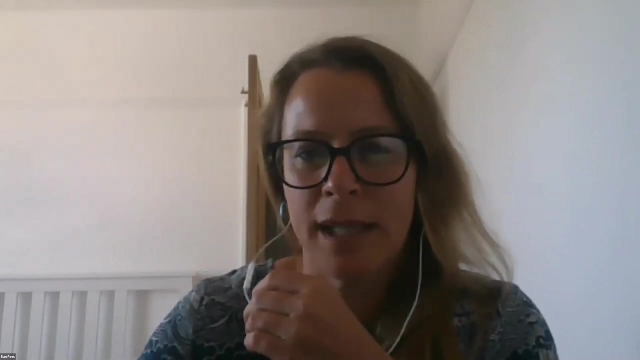 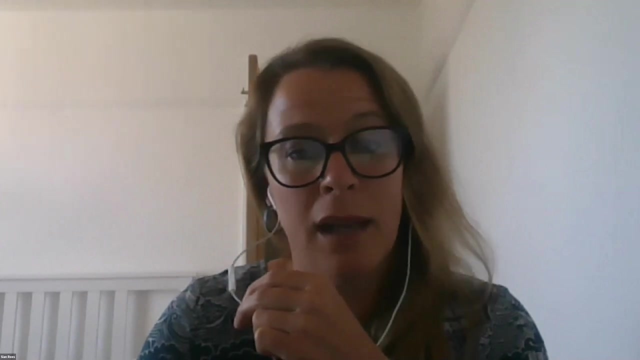 from ecological systems is how we make a living. it's the food that we eat and it's the air that we breathe, and in the deep sea, just like in coastal systems, we can discover those complex places that provide nursery habitat, refuge areas for marine life, including commercial fish species, things that enable the food. 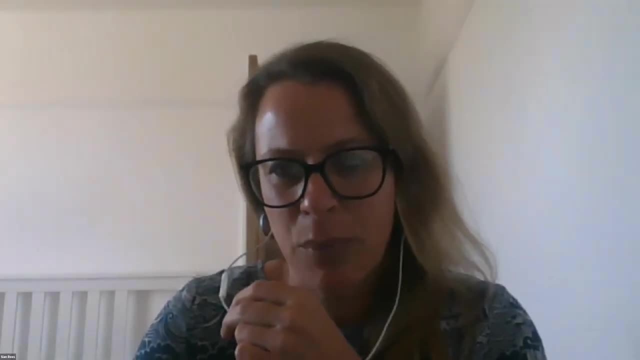 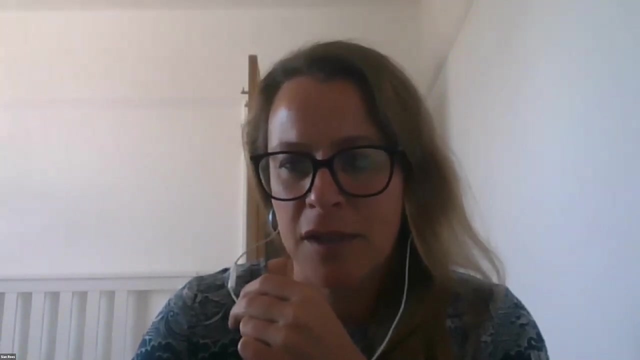 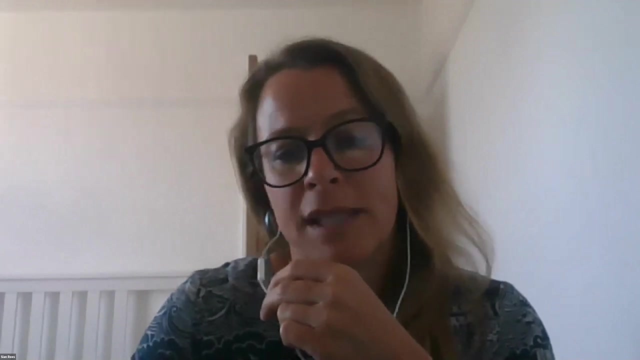 chain. but more hidden in the muds and the sands, perhaps, the less what we could describe as the, the less charismatic places are those ecosystem functions that support global processes through shifting, storing bioturbating carbon, for example, and when we think about precautionary protection of deep-sea. 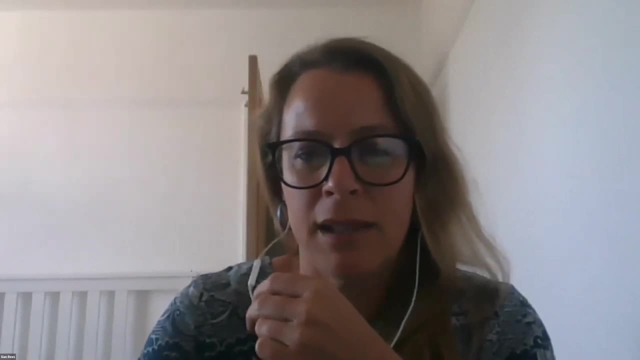 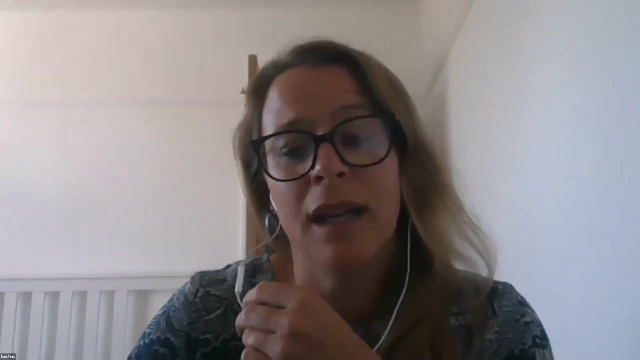 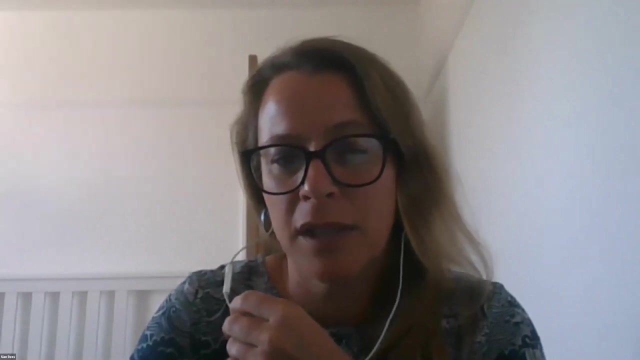 habitats. we have to think about the pockets of rare and the scarce and unique, but also the common and the functionalities of the ecosystem, and perhaps even the boring, the muds and the sediments, because global processes such as carbon and the nutrient cycle are supported by ocean ecosystems and 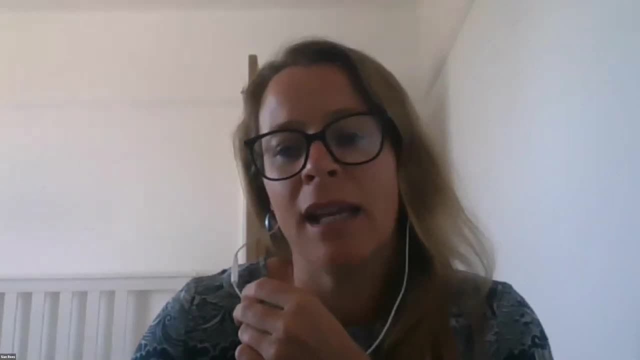 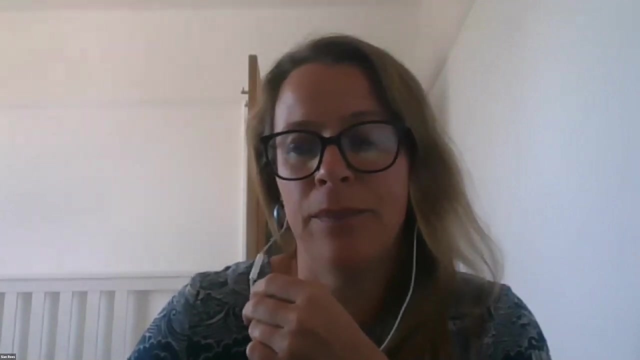 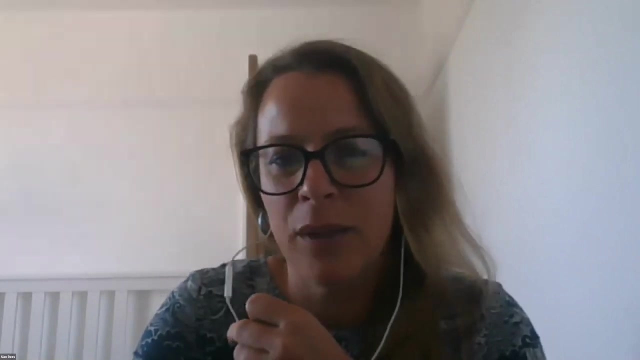 they're connected across vast scales, a scale at which current governance and management frameworks may not be fit for a global community. as an economist, I reflect on Kerry's presentation in terms of value, how we value and what we value of those benefits from nature, those ecosystem services. it's important to the 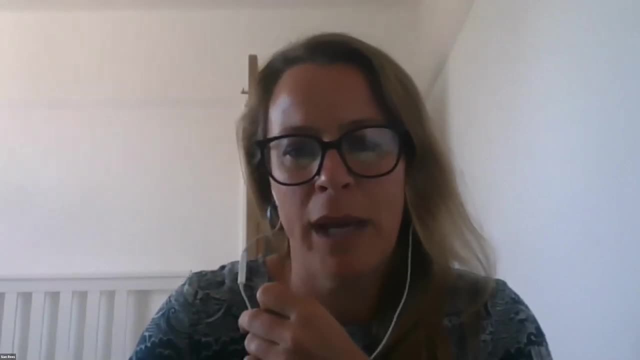 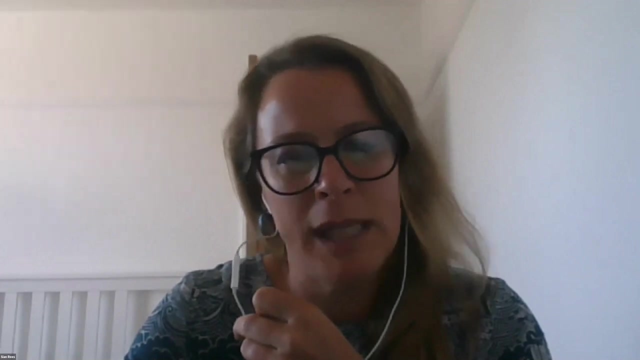 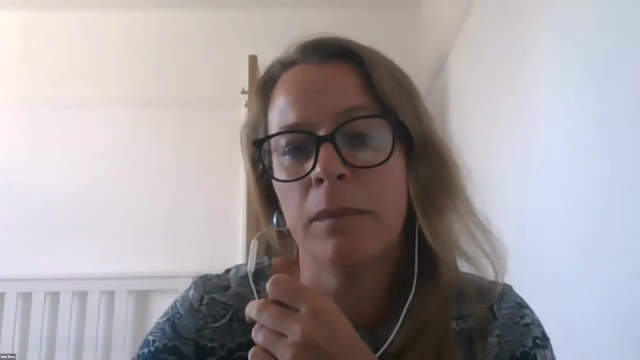 process of how decisions are made, of how we use or benefit or exploit different ecosystems, and it's really just too easy to see value in meeting economic needs such as jobs or GDP, and it's extremely challenging to create a decision-making forum where all values and value sets can be considered on an equal footing. 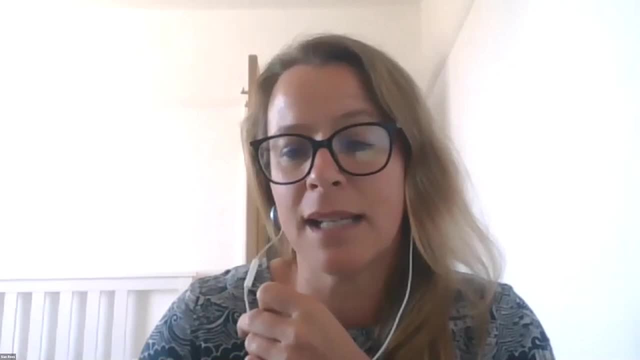 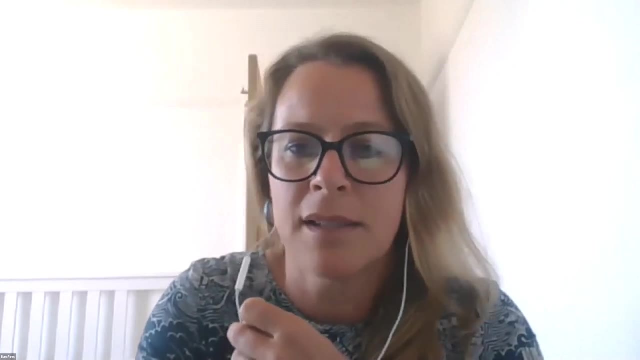 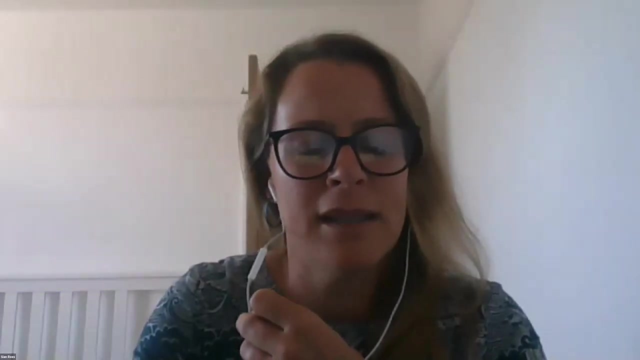 and also to consider if the sharing of those benefits is actually fair and Kerry demonstrated in her talk, I think, the much more complex strands to value the huge deep-sea fish, which is, which is the value of existence, of time spent, and how old are these fish, the 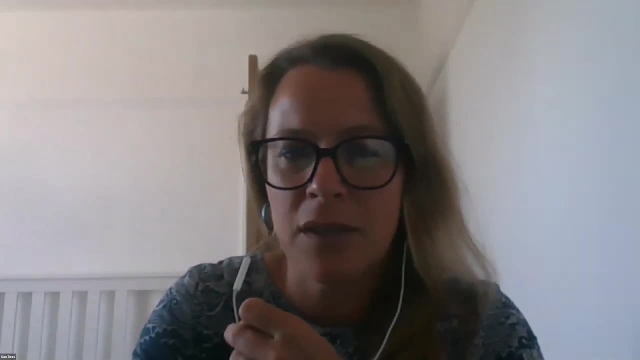 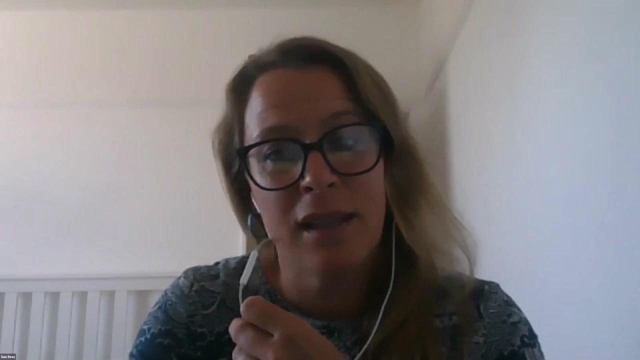 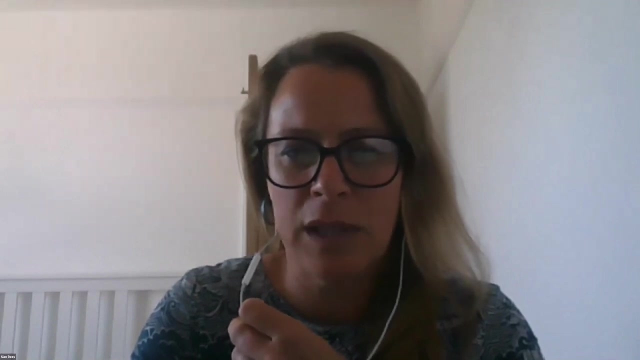 value of knowledge through developing partnerships with fishermen and industry. a drug compound even to treat cancer, and we have colleagues in the one ocean hub who are discovering ocean value in the antibiotic properties of deep-sea sponges, for example. and there are untapped reserves of knowledge and value that perhaps should be known or should definitely be. 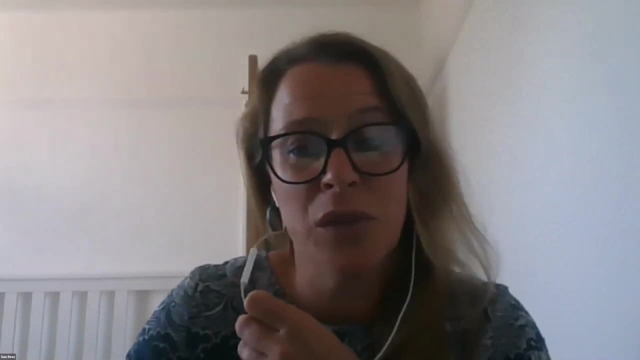 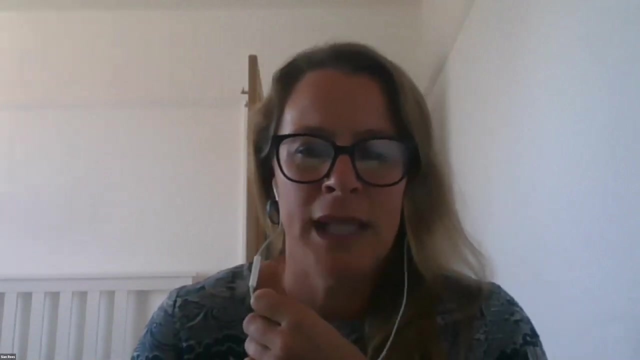 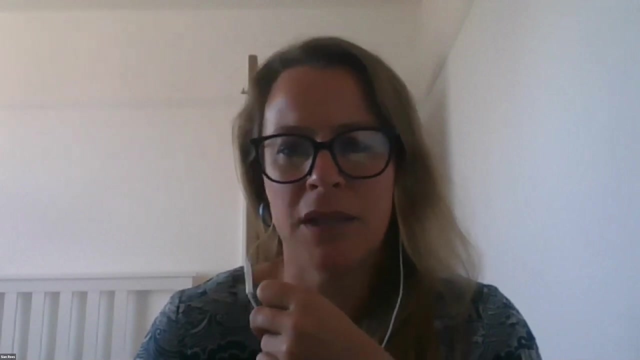 known before they are altered or destroyed. even so, my final reflection on Kerry's beautiful story is that we need to bring the social and the economic sciences much more closely into play, and Kerry describes us perfectly with her map- and Kira mentioned this as well- that the heaven and earth map shows the 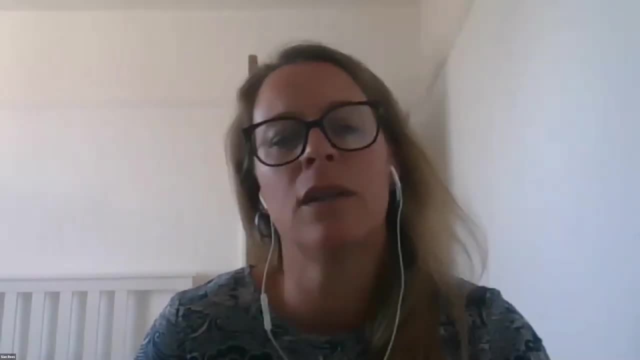 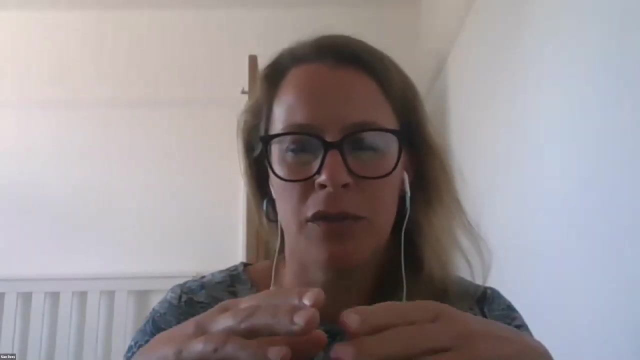 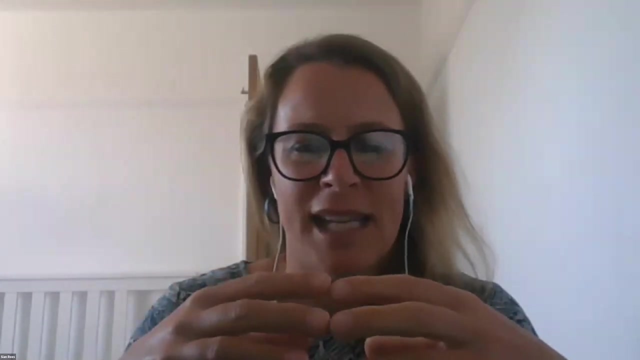 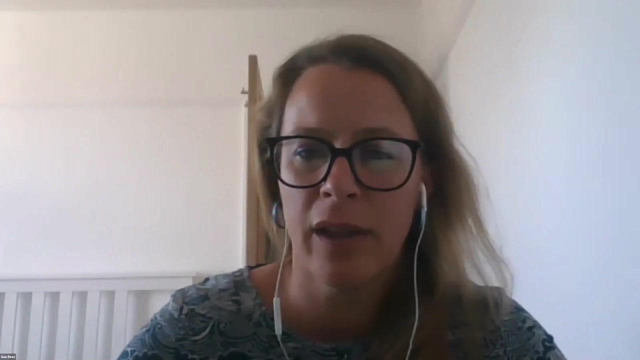 immense power of Maps and fine-scale trade-offs and negotiations. essentially, someone is mapping or annexing their economic value attributed to an ecosystem, but without another means at present to map things, it is. we could also consider that it's a critical starting point in developing shared values, but we do need to go further. 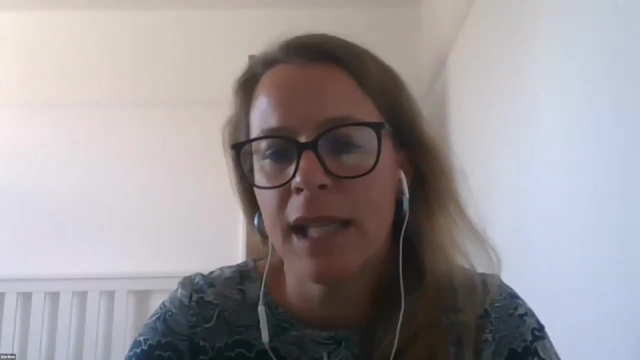 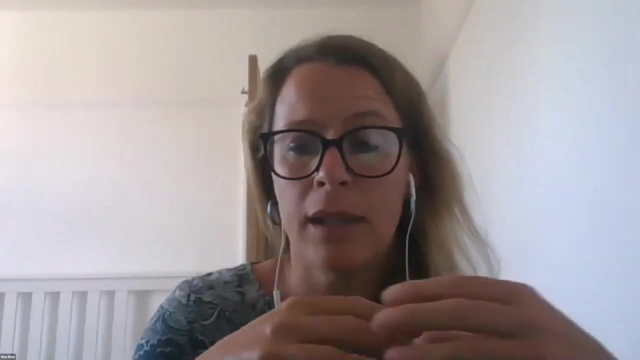 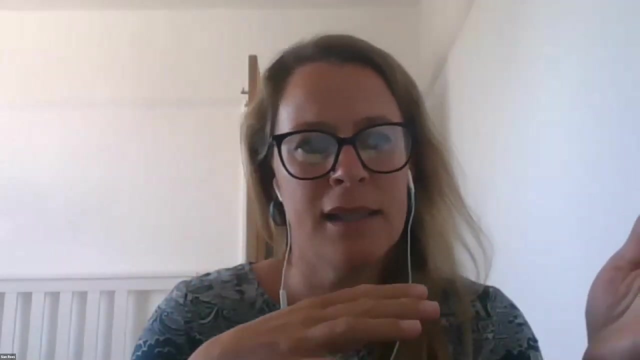 through bridging ecology into the social in the economic sciences, we can can derive perhaps a much more richer understanding of how ecosystems are linked to planetary health and human well-being, and then perhaps our conversations cannot be so binary between monetary economic values on one hand and conservation on the other, but much more nuanced. 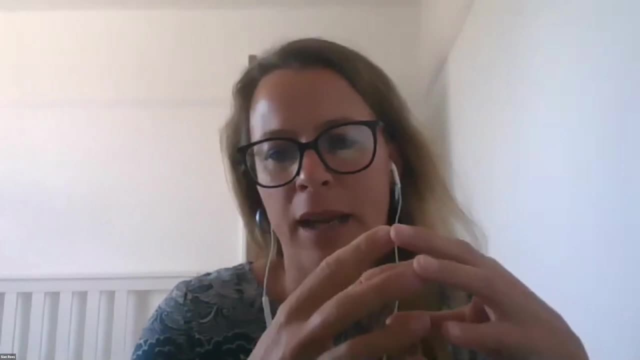 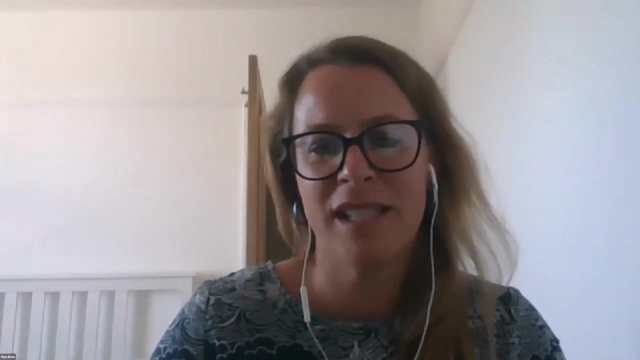 in terms of how they are linked and how we place the health and the condition of our natural environment, and all its diversity in terms of the services and the benefits it provides, at the absolute heart of our decision making. So I'd like to thank Kerry for her talk. 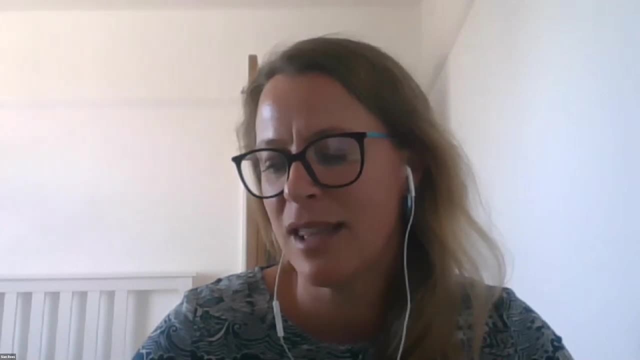 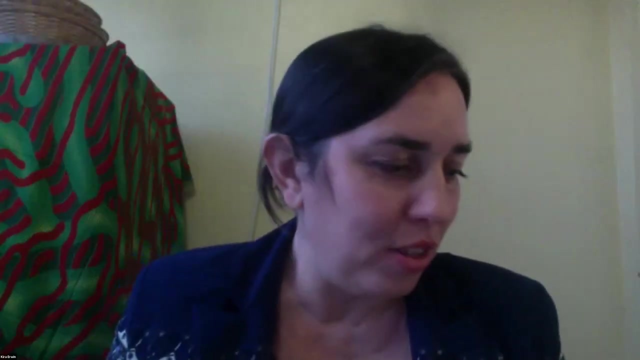 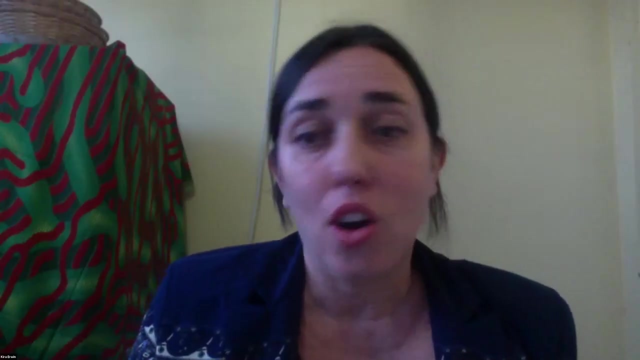 and also the opportunity to have a good think about my perspective on it. Thank you, Sean. thank you so much and absolutely as you're talking, I'm wondering how, in thinking about value, how do we also incorporate some of the comments that are coming up on the 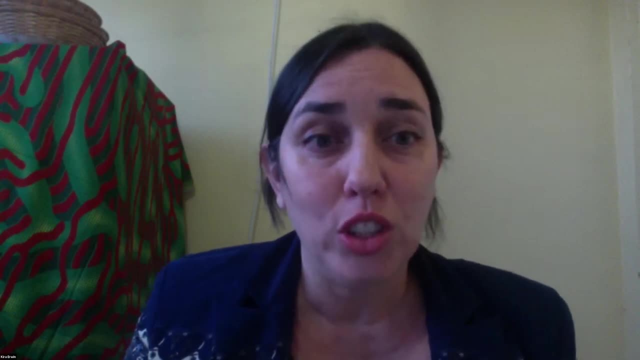 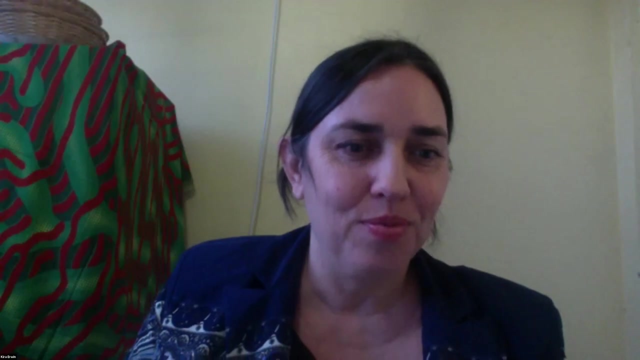 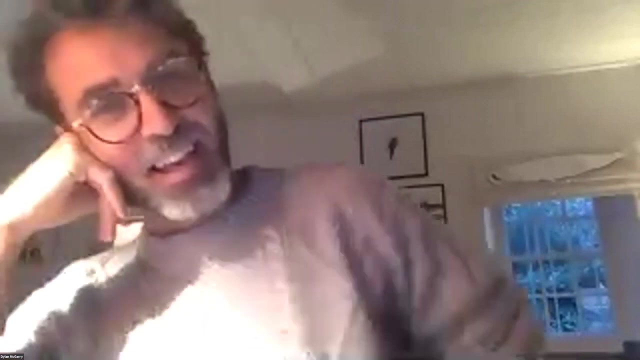 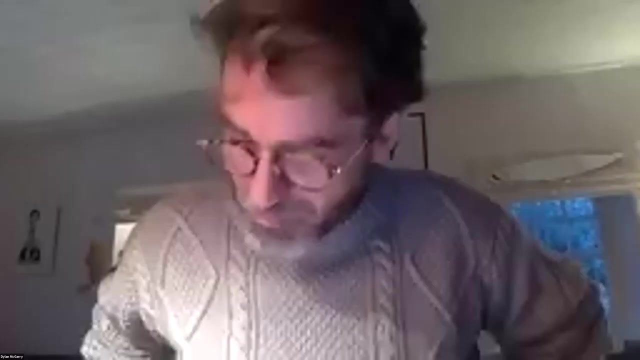 chat. So Anas from Jordan wrote: ocean love: how do we value environment? ocean love, Dil, I'm going to hand over to you. Thanks so much. For me as well, nice to have a segue with ocean love, because I think that's the thing. 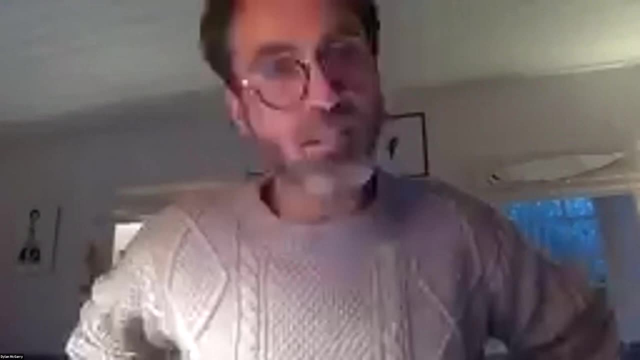 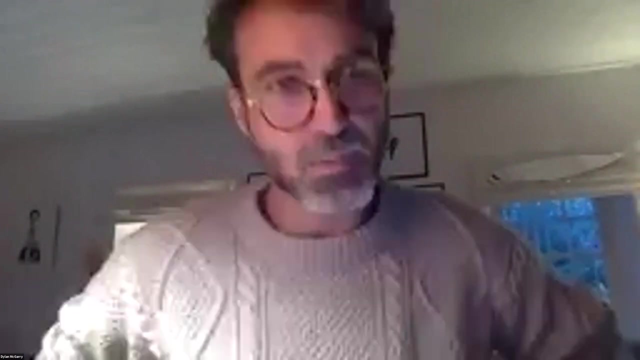 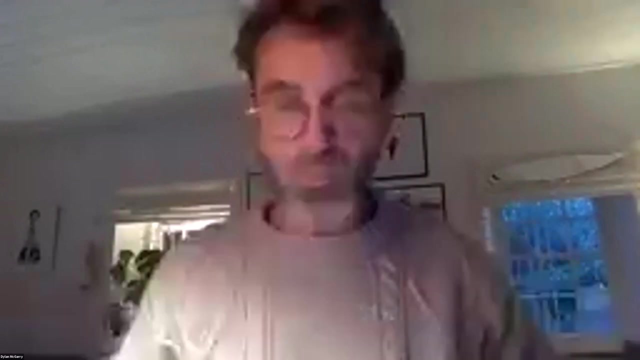 that really stood out for me was your love for an wonderful sea And also your capacity, not just as a scientist, to observe and reflect and try answer questions, but your capacity also to build relationships and the relational qualities that are needed in this kind of work. So there's these relationships with individuals. So I mean what really stuck? 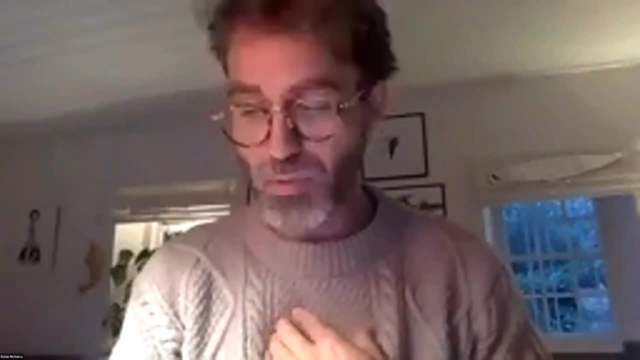 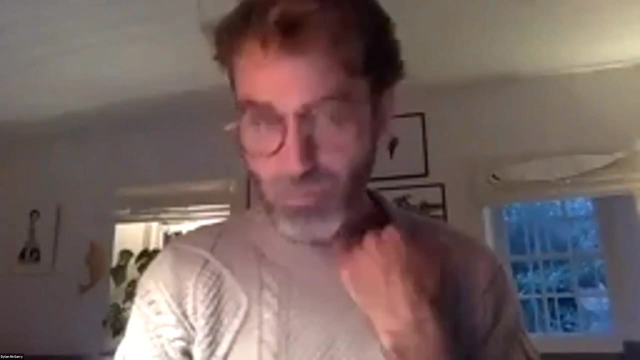 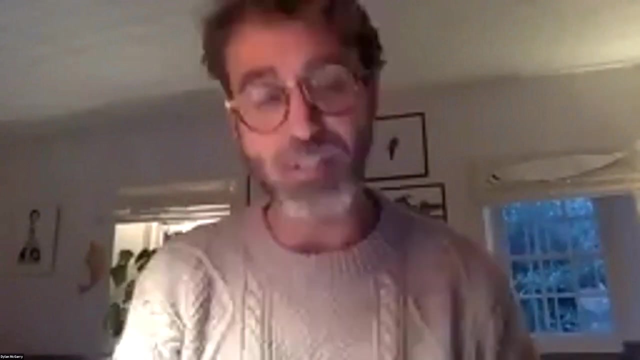 out was the individual relationships with the more than human, So with the coelacanths themselves as individuals, Bindings, Bindings, And their very personal character, their eyelashes or the markings that they have, And being able to follow an individual fish for 20 years is remarkable. 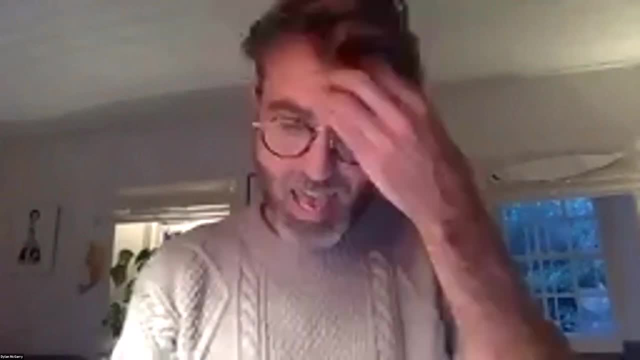 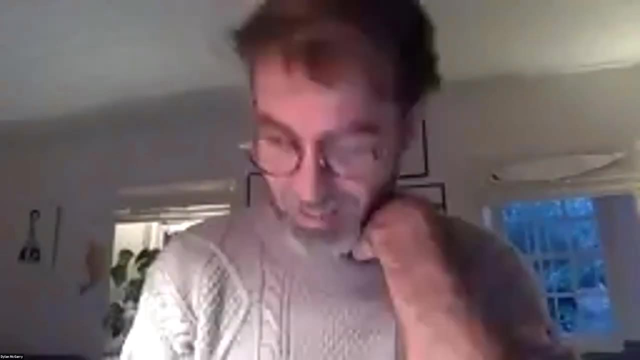 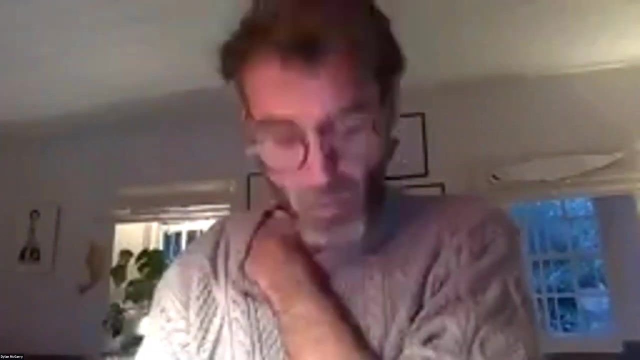 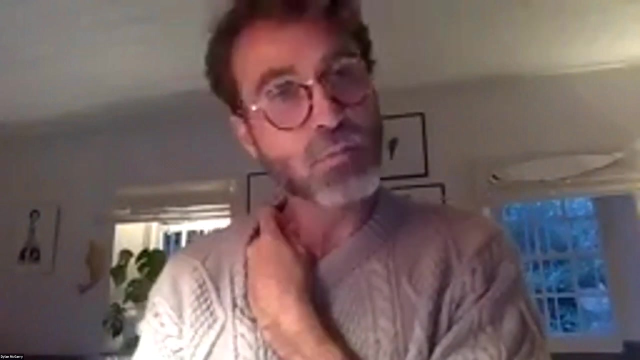 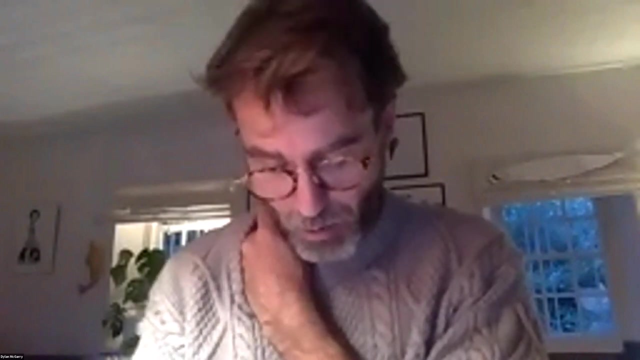 I mean especially a fish so strange and mysterious as that, And also this line you said is that you said there are many mysteries at sea, And I think that's part of the beauty of working in this realm, And the mystery that you discover on shore when seeing the mooty market that's used for ritual and magic and different forms of tangible and intangible heritage, really opened up some thoughts for me around how there are these other dependencies. 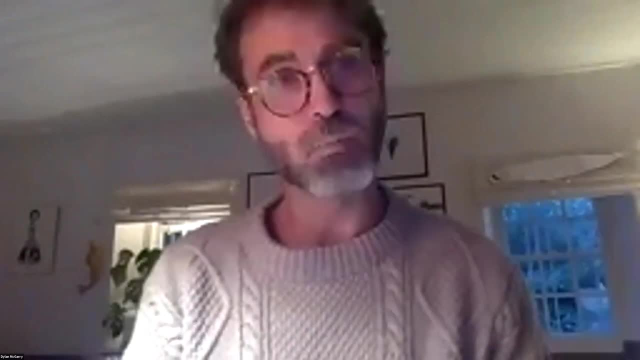 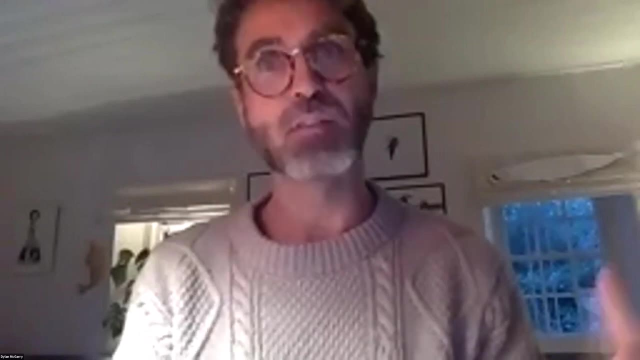 You said you know, you wondered, you know these were a group of people you hadn't consulted yet when building some of the parks, And how You know it opened up a whole new place for you to explore The worldviews and questions in which a whole other demographic has. 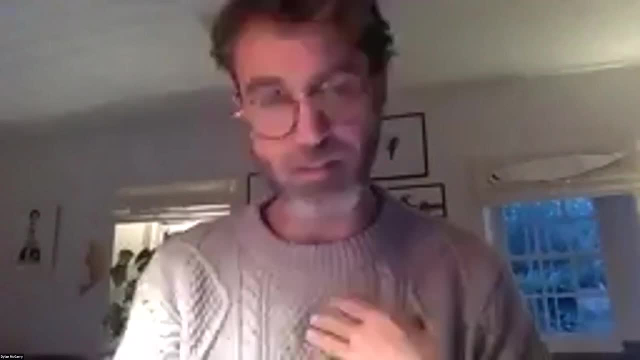 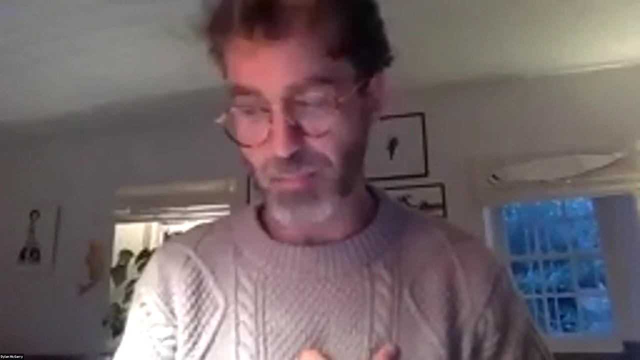 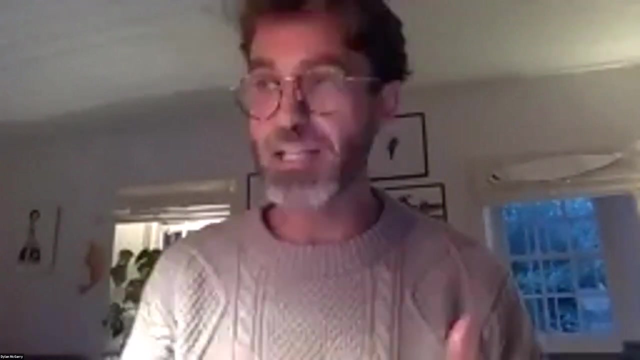 It is important to the Xhosa and Amazulu culture, with mooty and magic, is that the deep sea is a place that is equivalent to heaven. You're answering my experience of Africa, the ocean. It's a place where traditional healers go after the, when they go to gain wisdom from their ancestors. 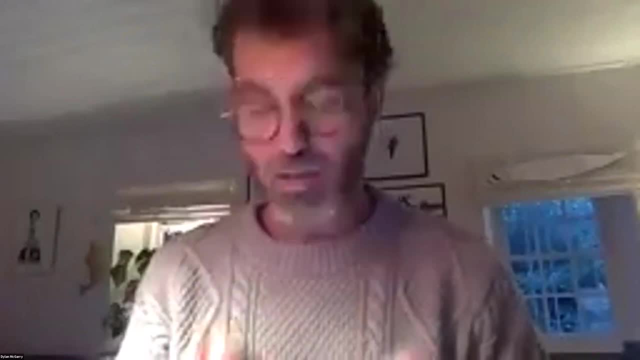 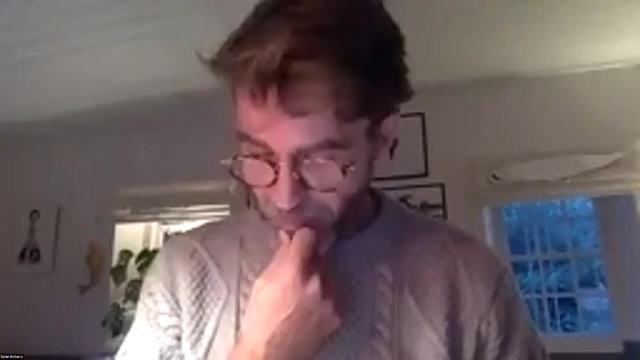 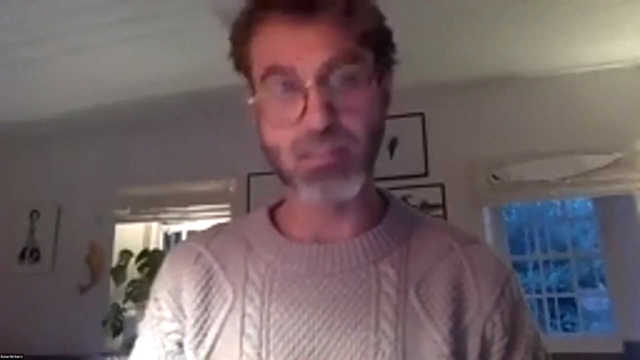 It's said that they go under the sea and the sea itself. the water itself has all these qualities and healing properties, and the species that come out of them are considered sacred. So just a scientist recognizing and thinking carefully about what this means when building these maps is so important and something we should all be considering. 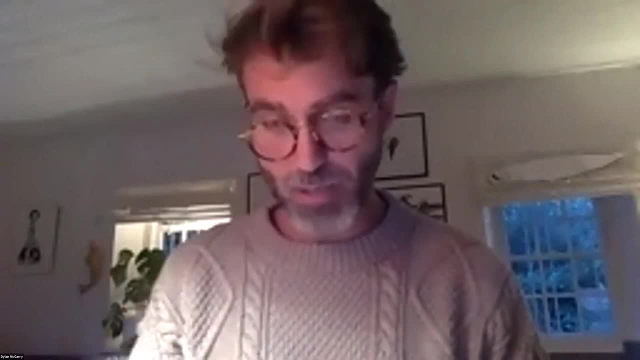 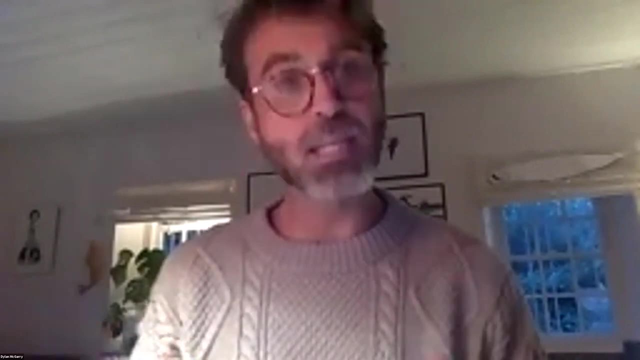 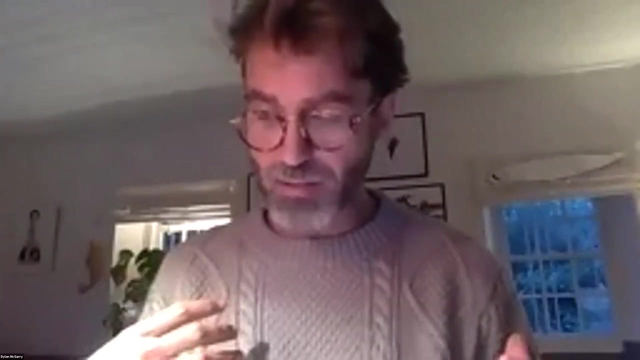 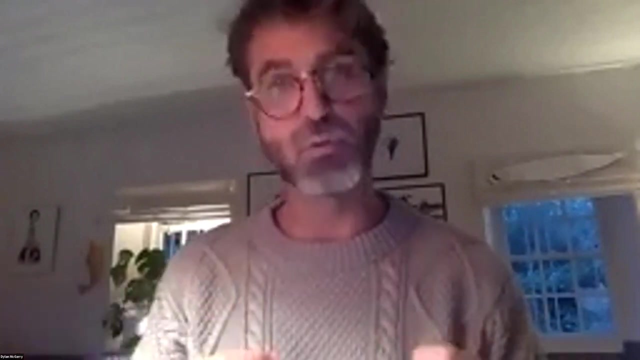 Around the world we're now thinking through trying to create marine protected areas and And who are the different publics That make meaning through the sea? And this relational quality And, and what also struck for me kind of echoing here and Sean, is this the power play of who isn't in the room and who is able to express the knowledge. 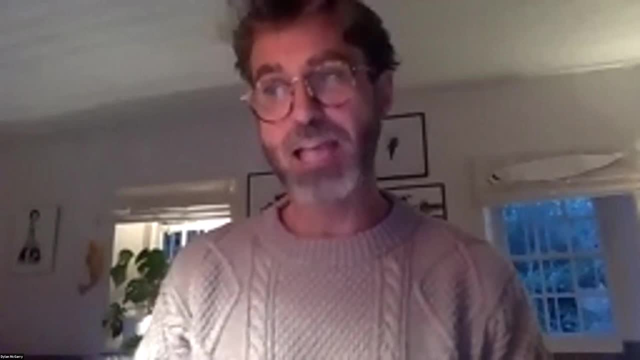 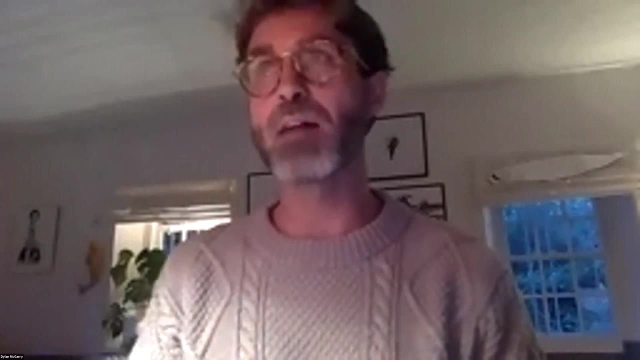 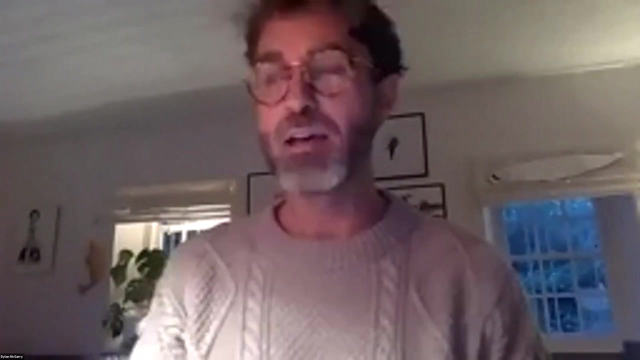 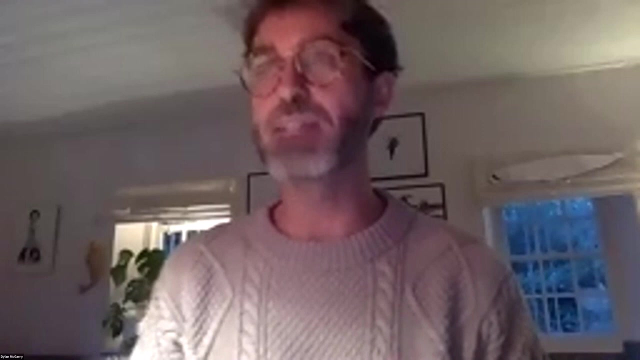 And will the perspectives and meaning, meaning making of the CB as valuable or as not as valuable, will be listened to in the same way a petrochemical director would be listened to. So how, how? my big question now is: how do we create groups that allows for a multi-market seller and a 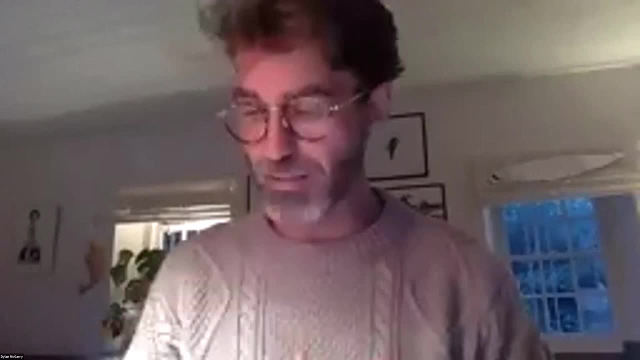 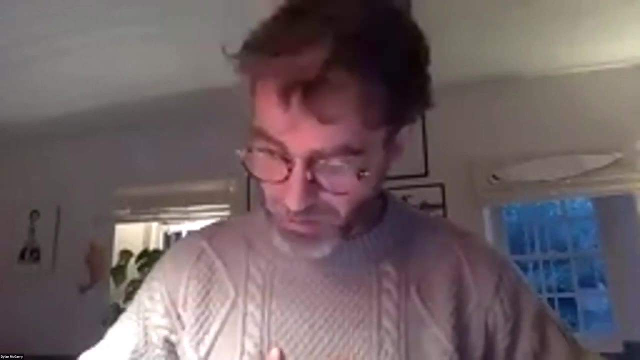 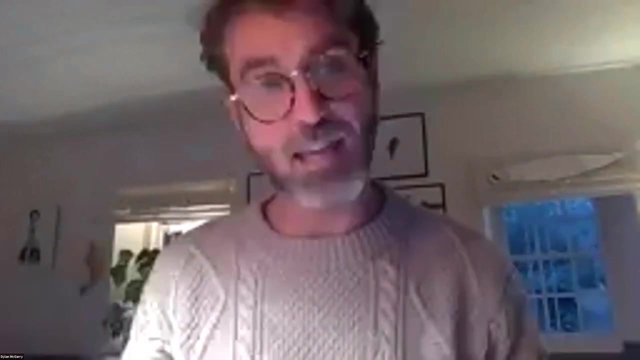 traditional healer, to have as much say in in that map as a as a petrochemical representative. So and then I also just thought that something that stood out for me is also knowing that your son was able to understand the importance of this work in 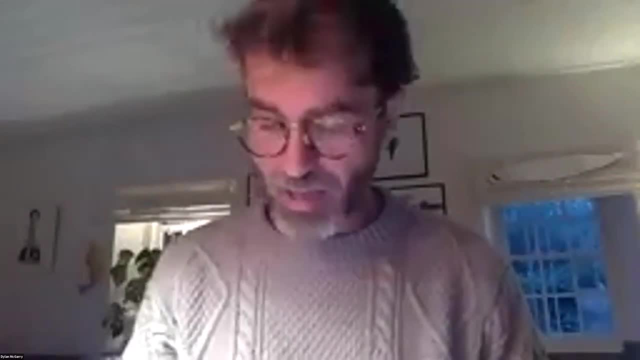 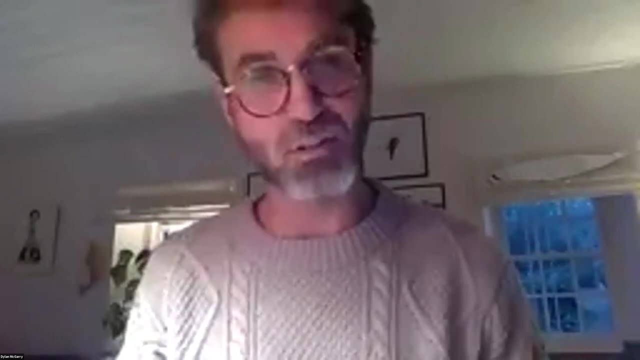 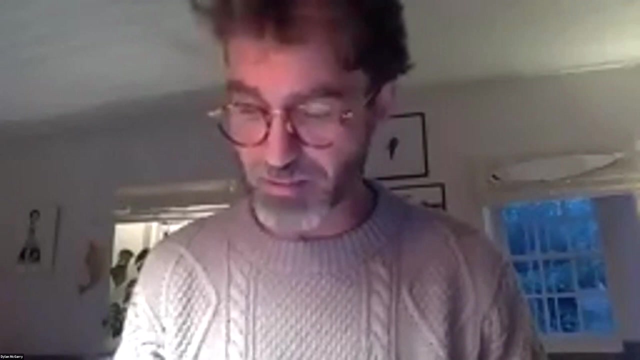 such an embodied and true way in himself, And that the difference between scientists and children is not not that different. And my engagement with getting to know you as a researcher, but also with other scientists I've met in this field, is that there's a 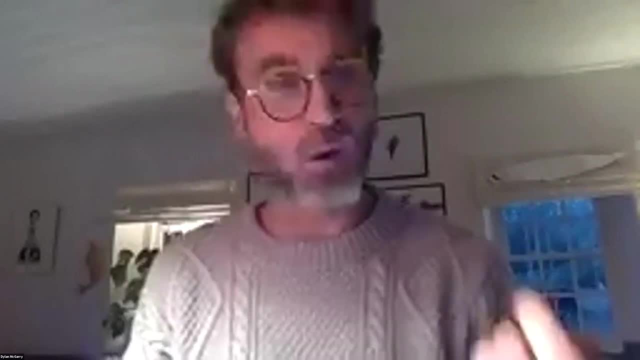 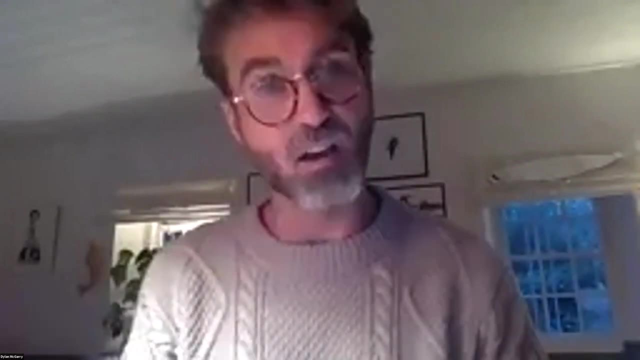 genuine awe and wonder and like, and often just being asking: what's that? I don't know. We're so excited, We can't wait to find out. I find that incredibly inspiring and exciting that there are still so many mysteries that we we don't have answers to. 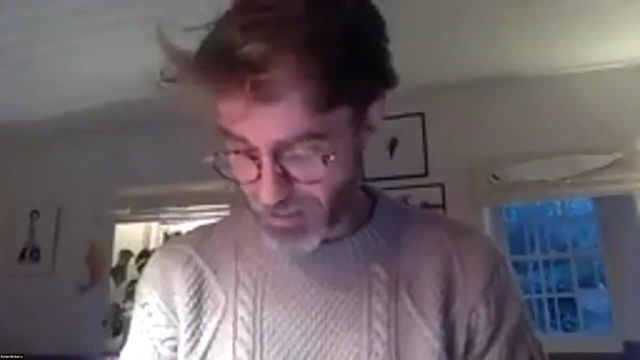 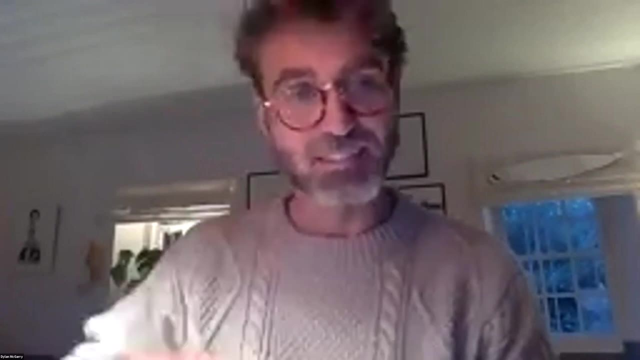 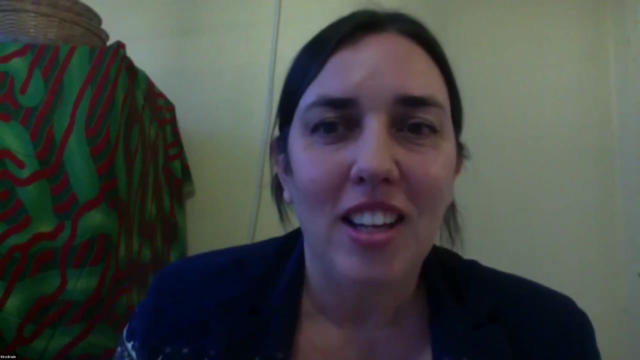 So, yeah, thank you so much for that Beautiful presentation and and also an example of scientists being incredible storytellers as well. Thank you so much, Dylan Kerry. I'd love to let you have a quick response to Sean and Dylan. 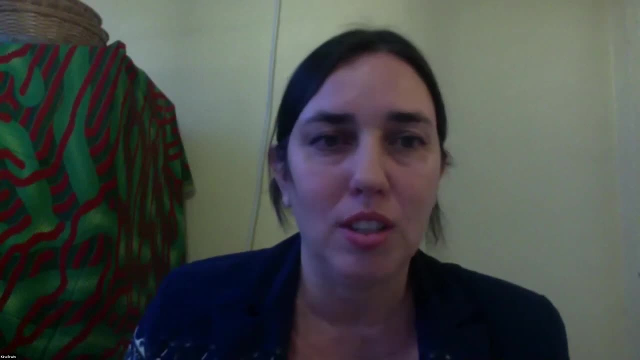 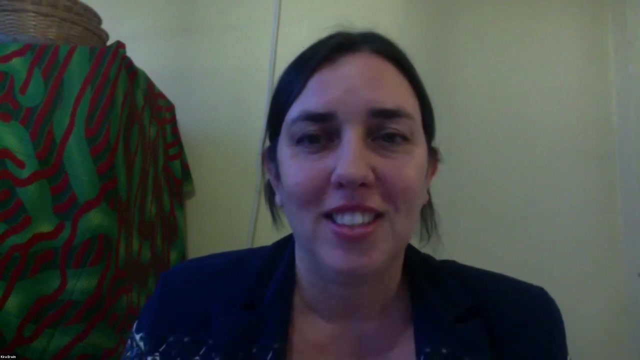 and then we're going to open it up to everyone to ask some more direct questions of yourself and possibly, if they'd like, some of the other panelists. but yeah, Kerry, perhaps you can respond and tell us what it was like to tell the stories and 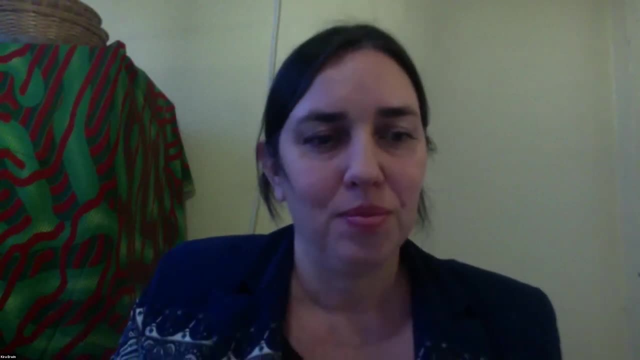 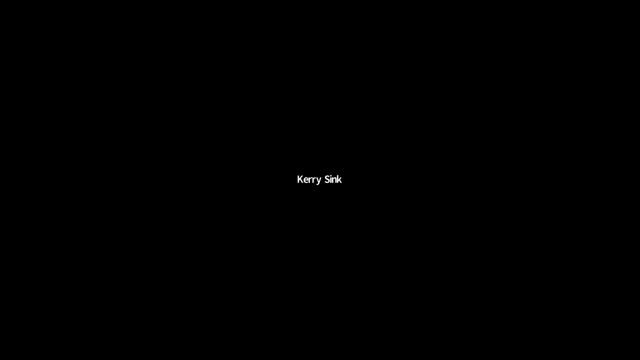 then to listen to people reflecting on them. Um, thanks Kerry. Yeah, It just really brought up more stories and memories for me of of different examples. Um, and to really reflect on this balancing act, it made me think about the part of the ocean. 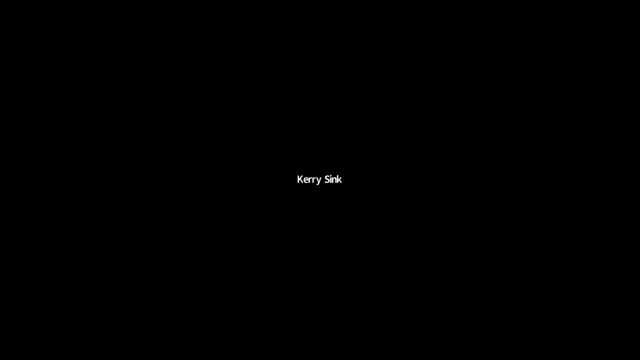 the 50% of the planet that belongs to everyone. And how do you make decisions for something that belongs to everyone? And that's something I still wrestle with, but I'd love to hear from the audience. No thanks, Kerry. 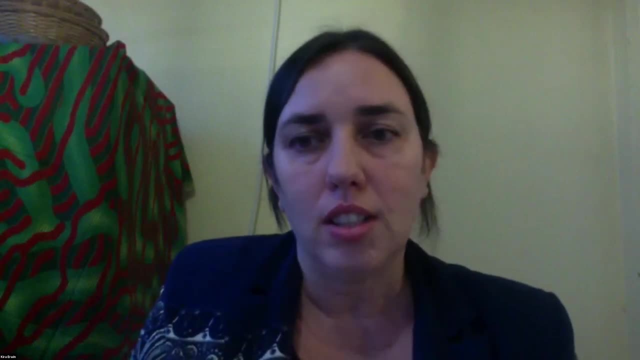 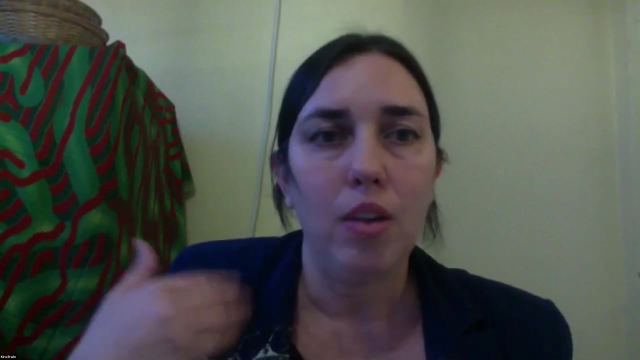 Let's do that. We're going to open up for questions and answers. Um, could I ask if you can raise your hand if you have a question, um, and when I ask you to, to please, uh, introduce yourself. 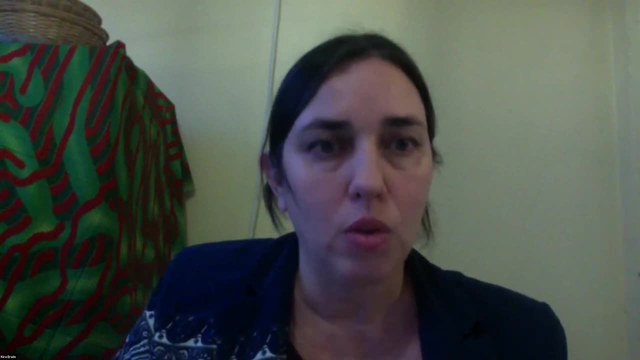 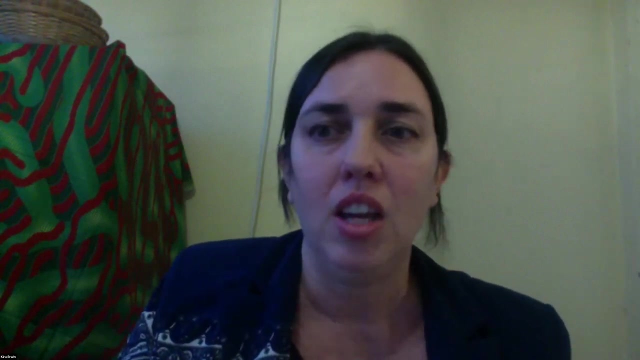 and turn your video on, if possible, just whilst you're asking the question. be lovely to see faces, And I'm going to take two questions at a time and then let Kerry or anyone else you'd like to hear from respond. Please do note that this is being recorded. 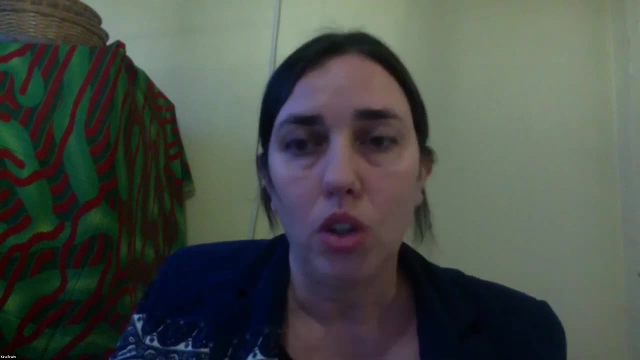 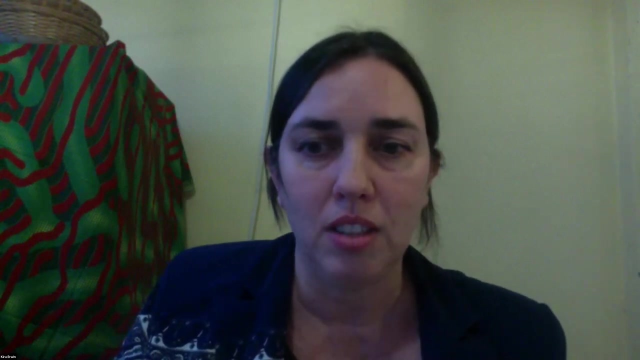 I just want to call your attention to that. Um, Joe is recording for the One Ocean Hub and I'm sure we'd be happy to share this afterwards if anyone would like the recording as well. So if you have a question, please do raise your hand and I will open the floor up to. 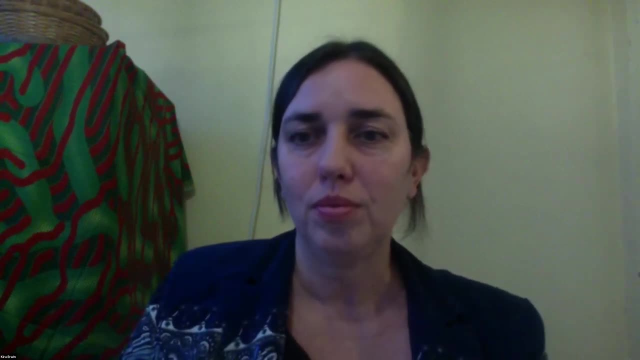 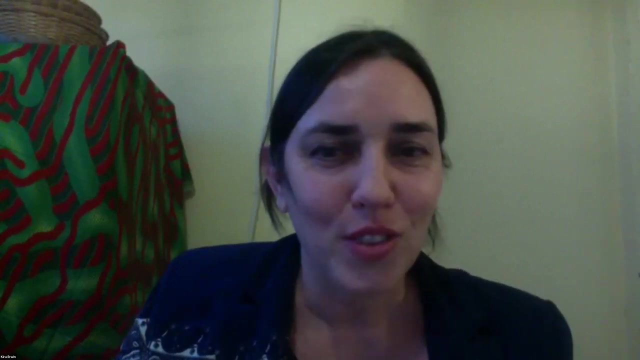 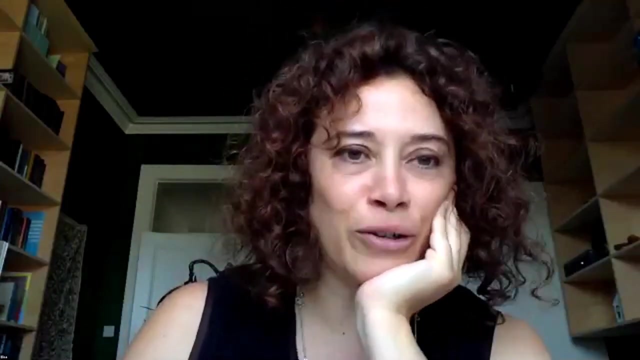 you? No questions so far, unless I'm missing some. Ah, Elisa, Yes, go ahead. I thought I'd break the ice and see if others will follow. Uh, I think Kerry was. I mean, I've I've heard your story before. 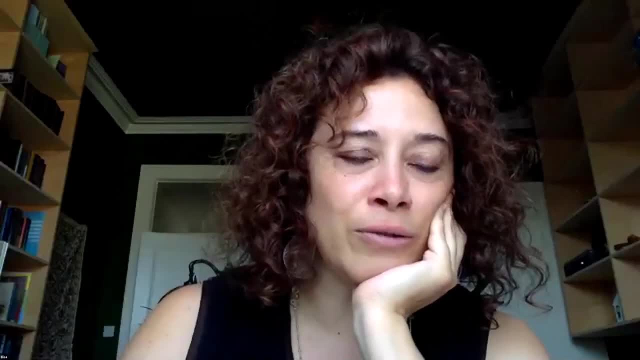 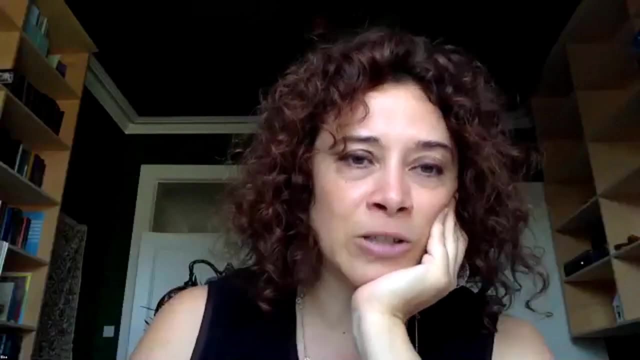 but each time, new thoughts, I think, come to mind. Uh, one thing that I thought was very interesting- maybe you could expand a bit more uh, for the benefit of our colleagues on the call- is what your experience in collaborating with them? 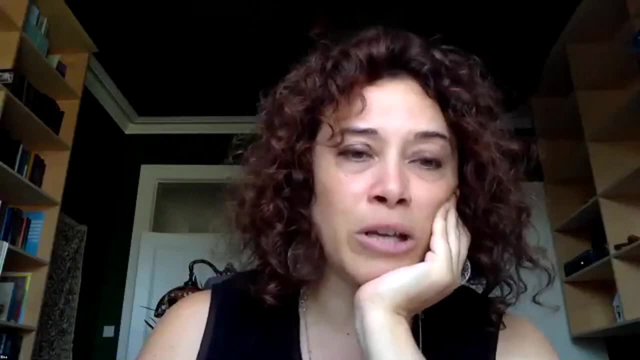 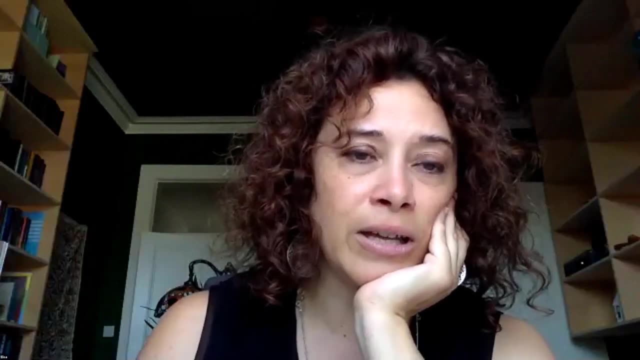 scientists from the U? S and Europe. I know you mentioned in your story how significant it was for your colleague, I think from the U? S, who came to South Africa to work with you. And you know, teach and learn from you, And I 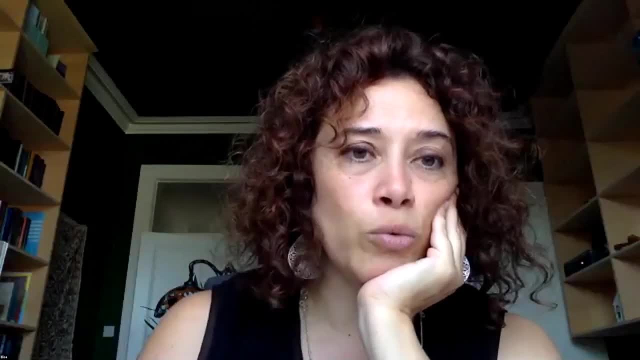 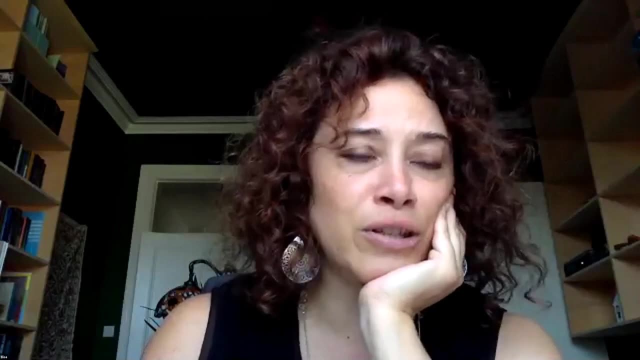 and I was wondering if you have more stories about what it means to work with colleagues from other countries that may have more means and um uh, capacity to, or have been, deeper than you in the oceans. what has worked and what has not worked? 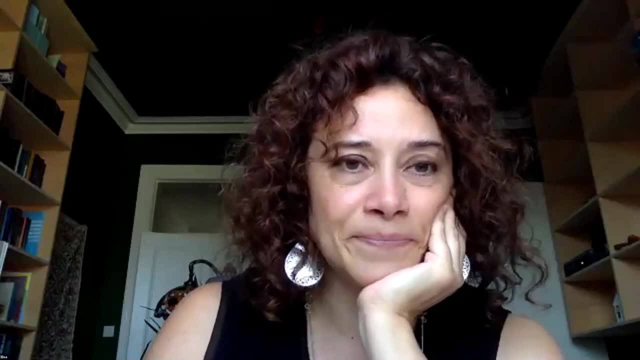 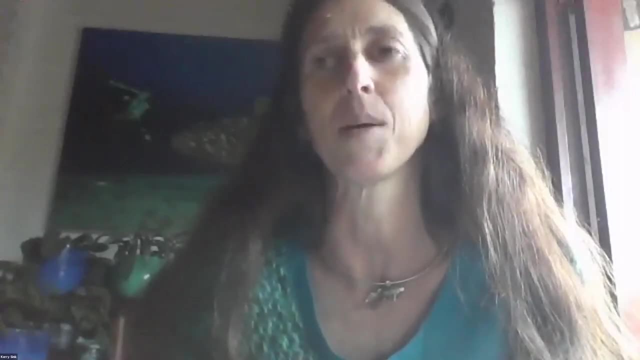 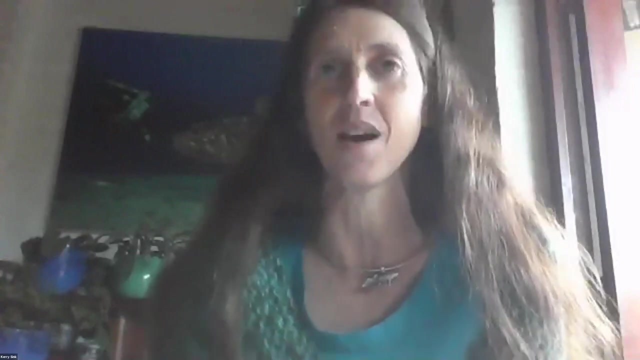 um, for you and for your own research in South Africa. Thanks, Elisa. Yes, Um, so it's always something that, um, we were often a little bit jealous when we get to see the kind of technology that many deep sea scientists from other countries have. 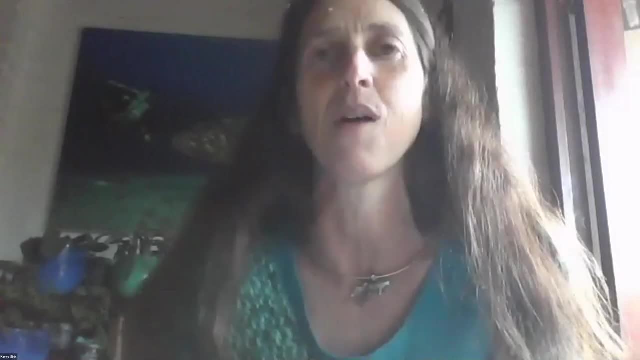 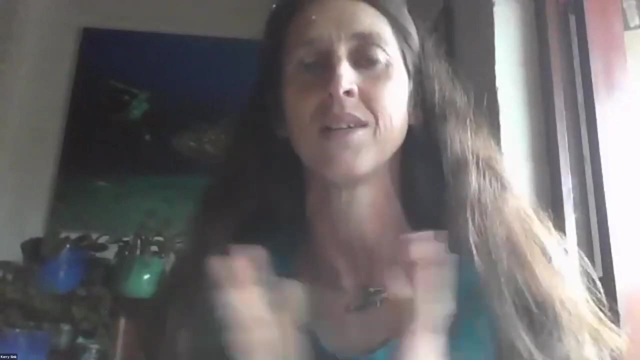 And indeed when I first went to the deep sea conference, I felt a bit like a fraud, because the deep sea is generally defined as 200 meters And so much of my work has been in kind of the twilight zone between a hundred and 200 meters. 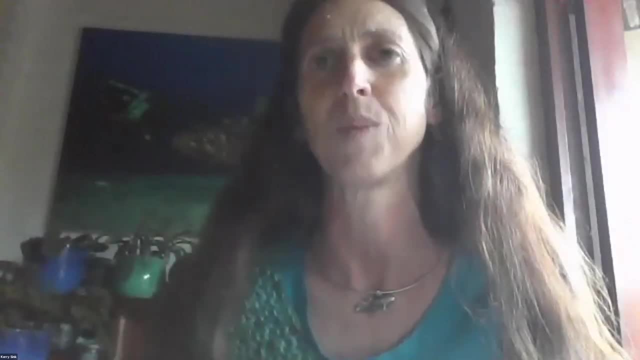 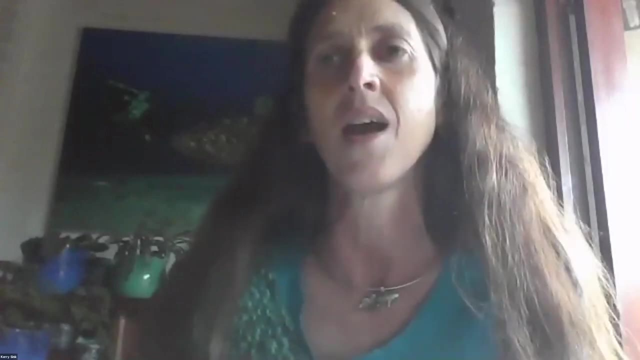 not often making it into that really deep area, So so that always was a bit of a discomfort for me, but the the community is often very welcoming, And the person that I was talking about, Lisa Levin, is someone who came out to. 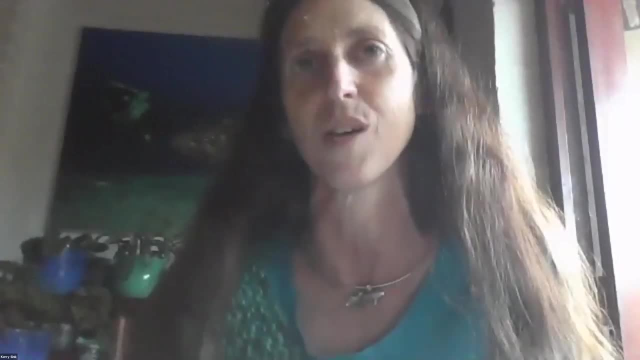 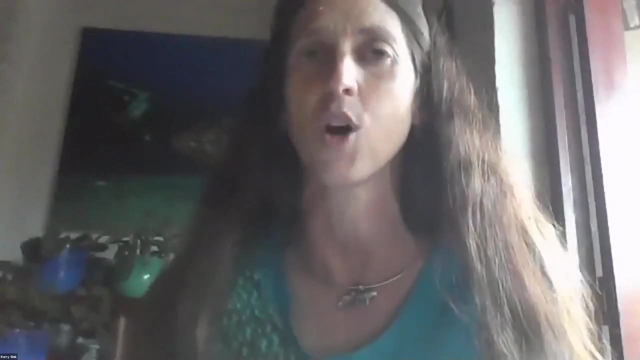 to South Africa and gave a guest, gave guest lectures, several guest lectures, And there were very few people who seem to be interested from South Africa, but myself and and the one ocean hub colleague, Laura Atkinson, were in the audience And um. 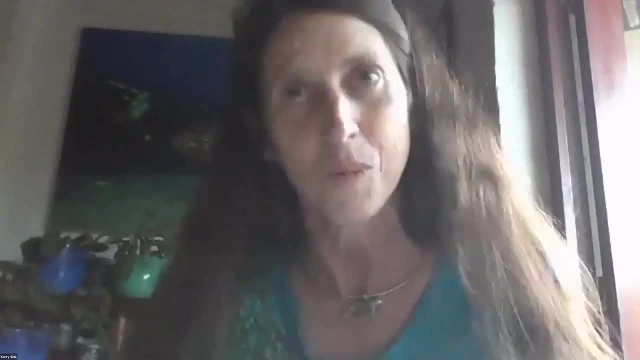 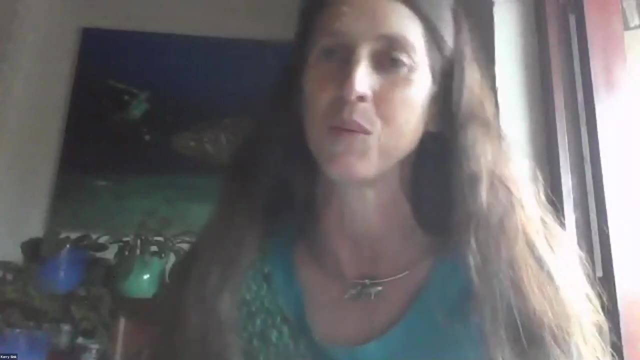 Lisa really gave us the confidence to say she was like no, you should be giving these lectures, You should be talking About the deep sea in your country. And we were like no, we don't really know enough and we haven't sampled. 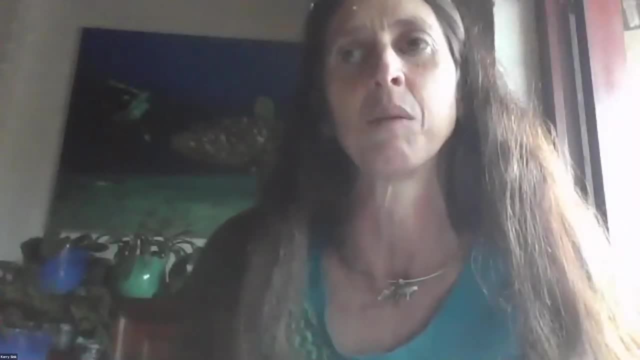 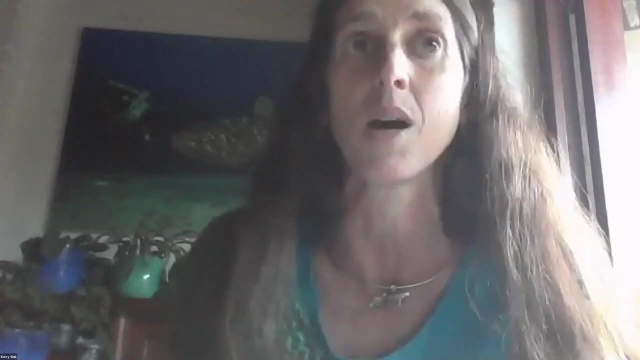 And we don't know what the things we are seeing on. She was so encouraging but, um, but really the the kind of game changing experience for us was when Lisa was willing to come across to South Africa and come to see with us. 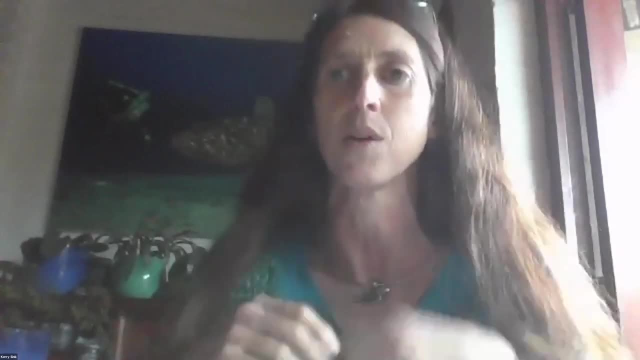 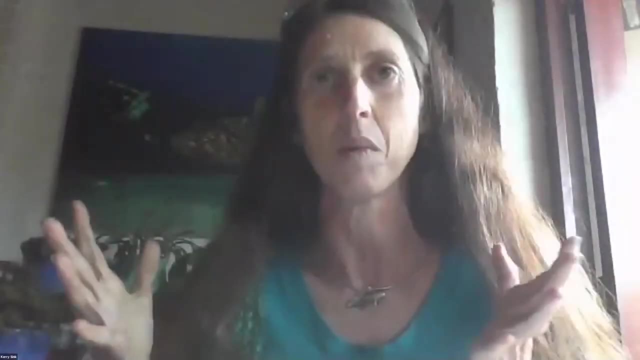 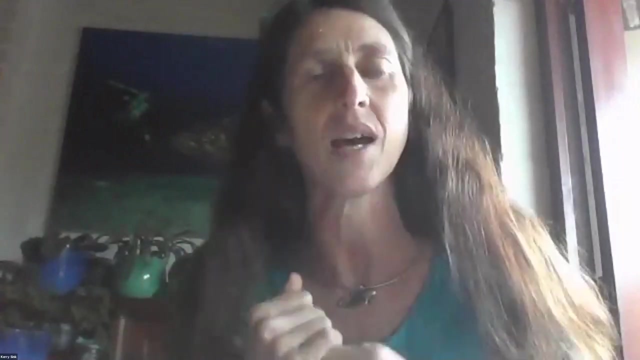 And what was so important about that and so different from the experience of a of a developing country scientist going and participating on a cruise where you get to have amazing experiences but that technology is so out of your reach. So so Lisa came to us and then, within the constraints of our 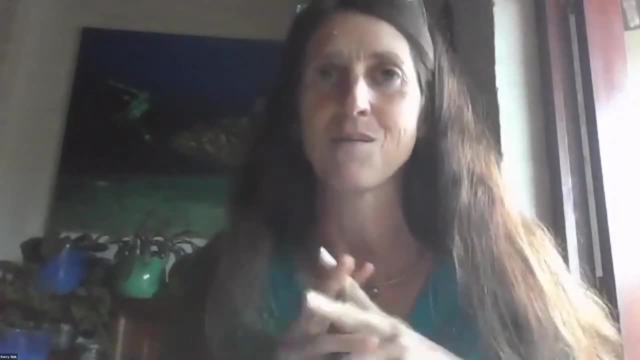 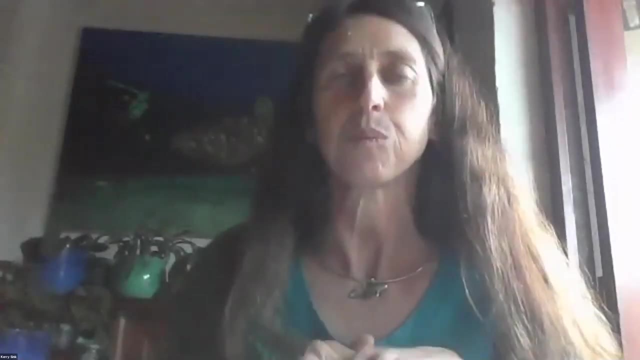 uh, our kind of, uh, our ship that we have and the equipment that we have which is like a drop camera that we have. she really taught us to strengthen the science and, uh, our own conditions and our own limitations And we have the Agalus current in South Africa. 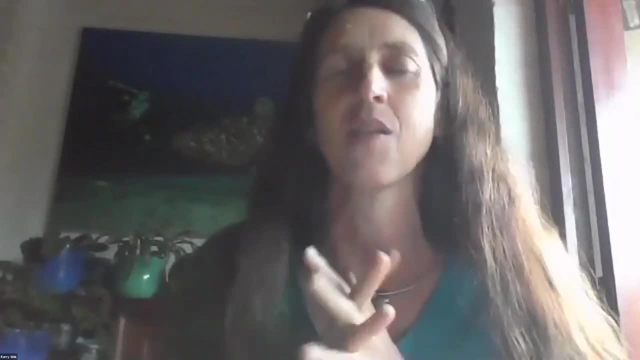 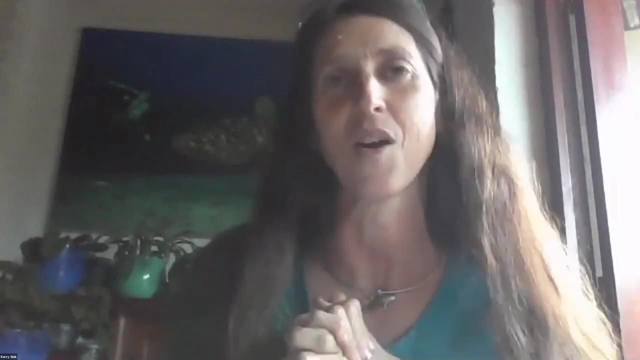 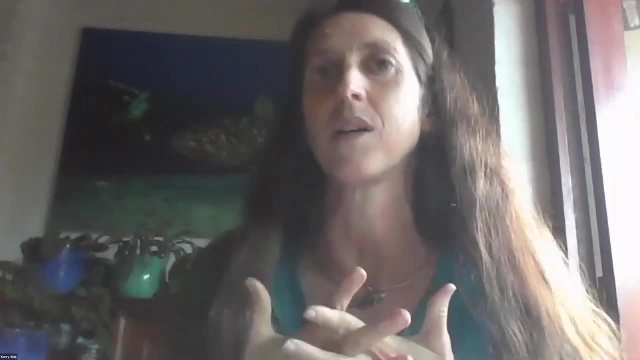 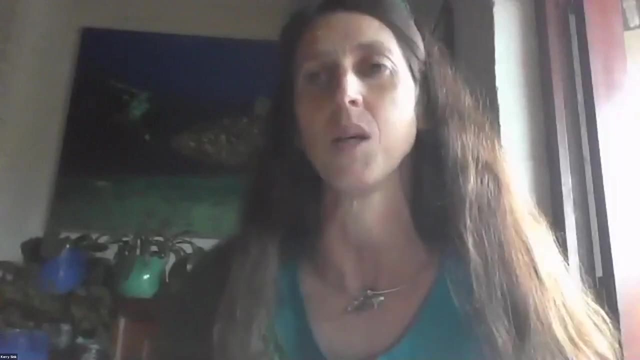 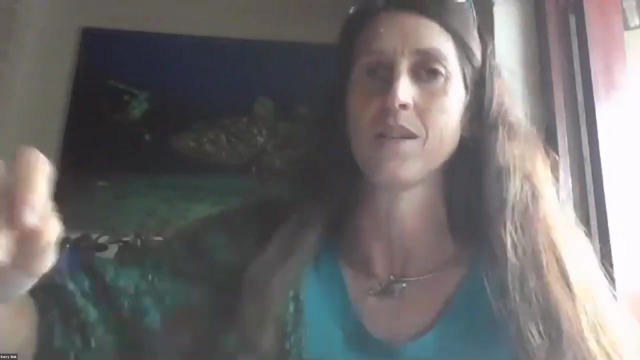 our equipment down Um, and Lisa was able to share some of her more practical experience, but also to show us what different deep sea ecosystems look like, teach us to recognize SEEP systems. So it's not a common capacity development model, but really one that I think is very important. 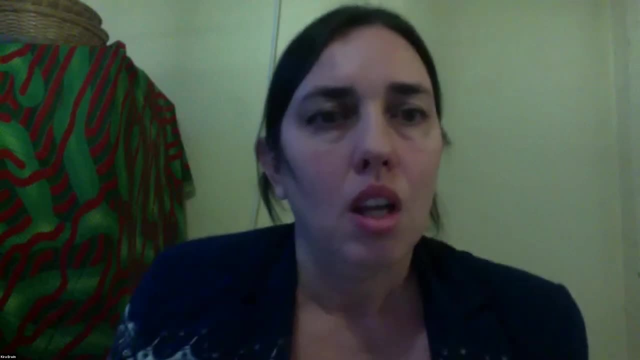 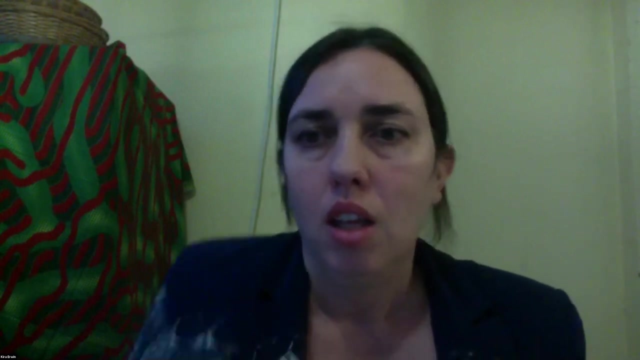 Thanks Kerry. Thanks Lisa, for the first question. Anyone else have questions you'd like to ask of Kerry, or perhaps you have something you'd like to share? Kerry's stories are frequently about relationships, and that can those can- be very tricky. 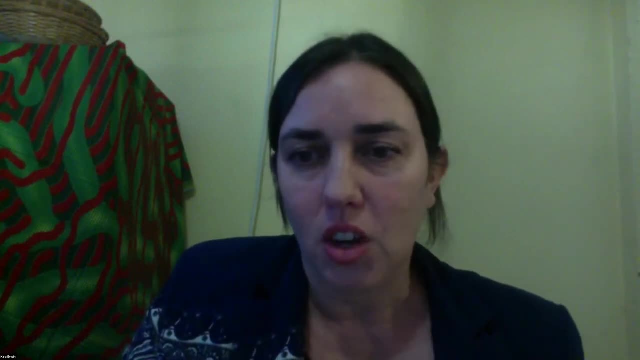 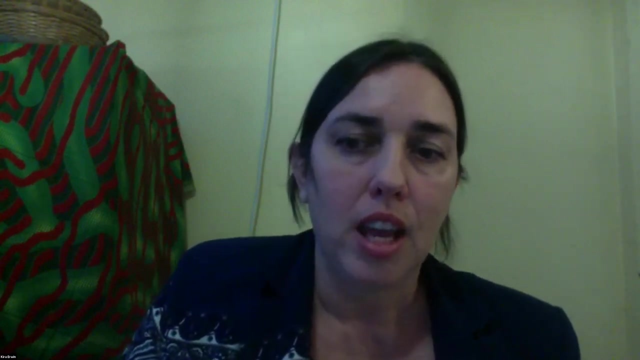 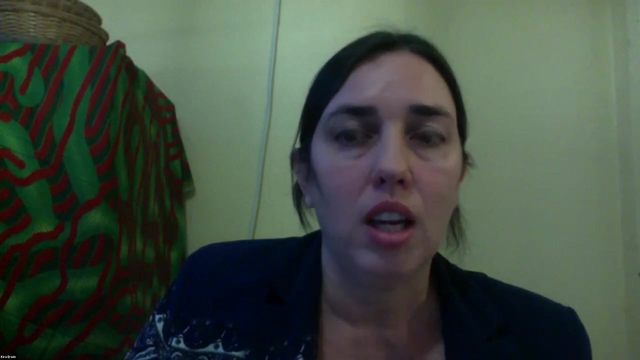 uh, in negotiations as well. Okay, So Holly has a question for all panelists. What do you think are the barriers for people embracing the less tangible benefits of the deep sea? Thanks, Holly. I note that I'm going to let Andrea. 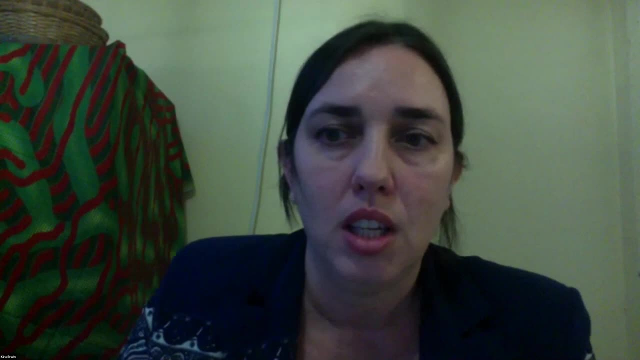 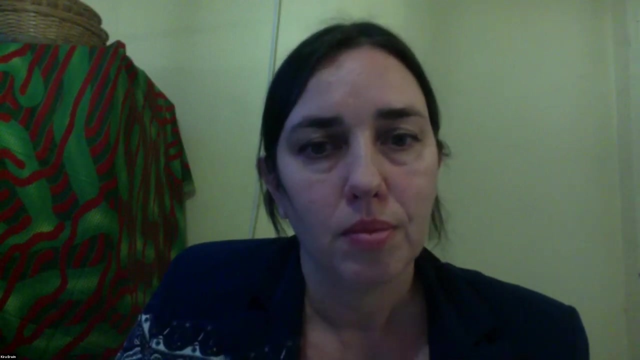 have a question as well, and then we'll come back to both of those. Andrea, I see your hand up if you'd like to give us your question, please. Yeah, thank you, Can you hear me? Oh, good, Kerry. 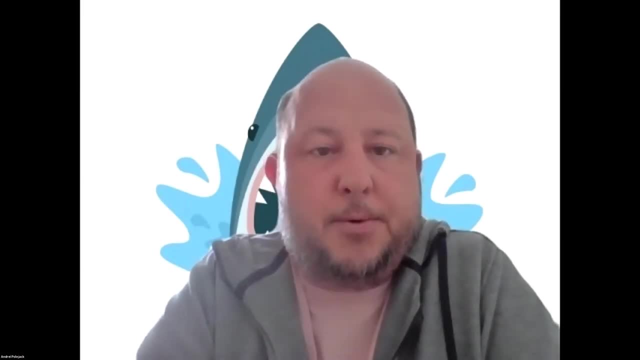 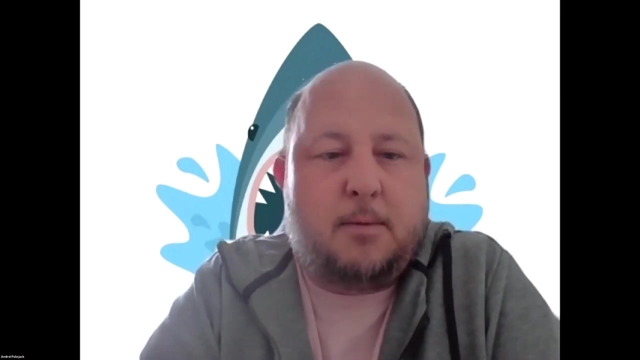 thank you very much. First, I just wanted to ask you, uh, if you are aware of, uh, the balance statement that was signed between Brazil, South Africa and the European Union on a research collaboration and deep sea, certainly one of the areas that we are looking into. 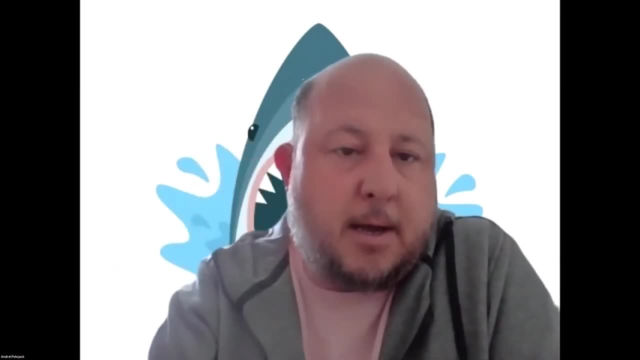 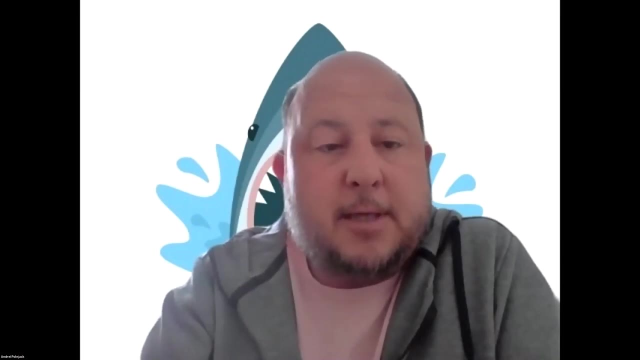 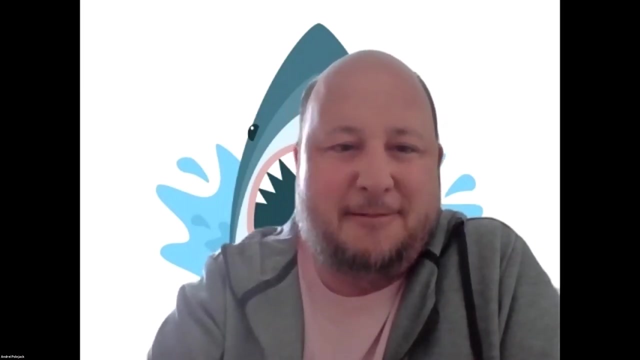 And then can uh, that is a framework that can uh really help you uh to develop further uh collaborations into that. Uh, the other question that I have to you is: I'm a national from Brazil and we are in the same capacity as scientific. 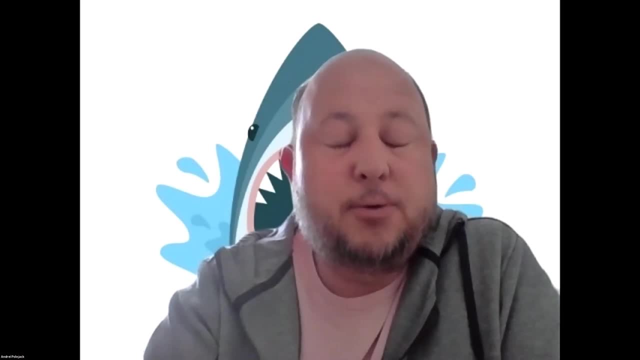 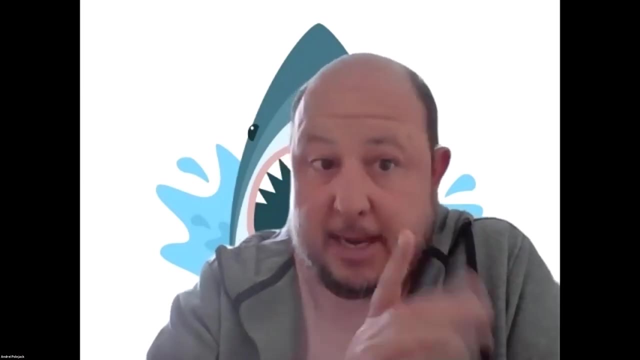 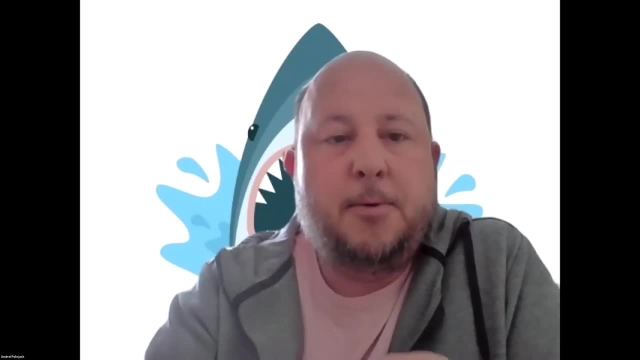 uh, the reasons that you're sure you shared. So one of the issues that we always had is that usually oil and gas companies, they have all the data that we would die for, uh, to get our hands on, And it's very hard to get them. 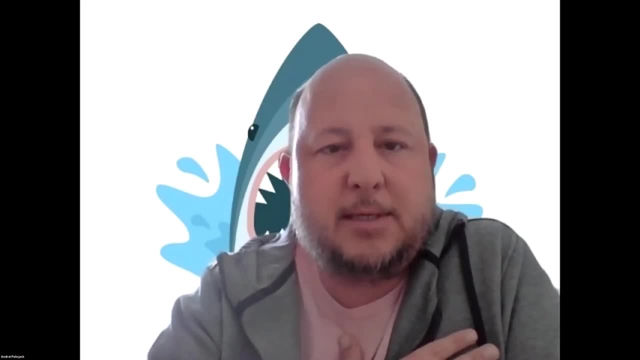 uh to release the data or to work together with the scientific community? And by you nodding, I understand that you have uh the same issue in South Africa. So I thought, uh, but uh, don't you think that the power of 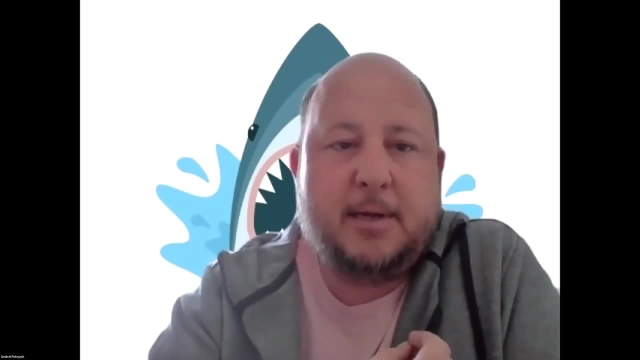 uh, I've been learning a lot from social sciences and now on, uh, how to develop better science to policy interface, in a sense that the even pressures can be given into the companies in the private sector, uh, towards more collaboration. What? 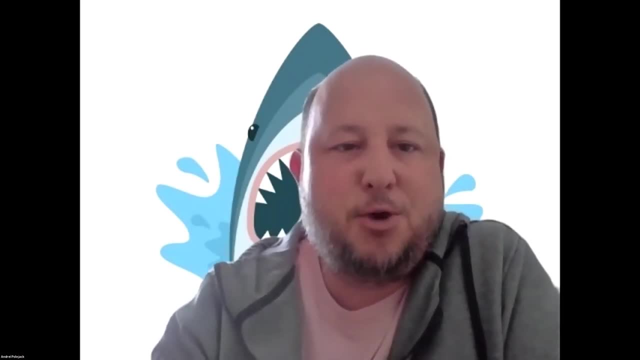 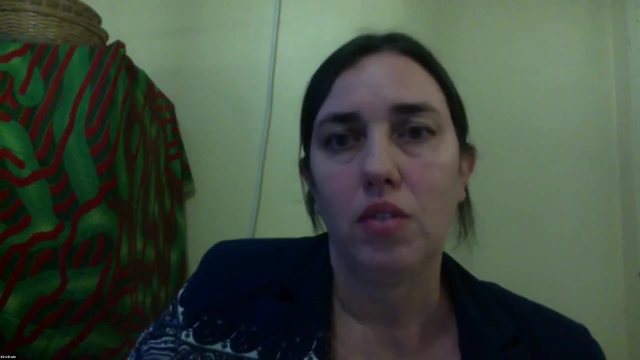 what are the lessons that you could share with us from that regard, Thank you. Thanks so much, Andrea Kerry. I'll let you answer that question first, if you'd like, and then if you've got anything to add for Holly's question. 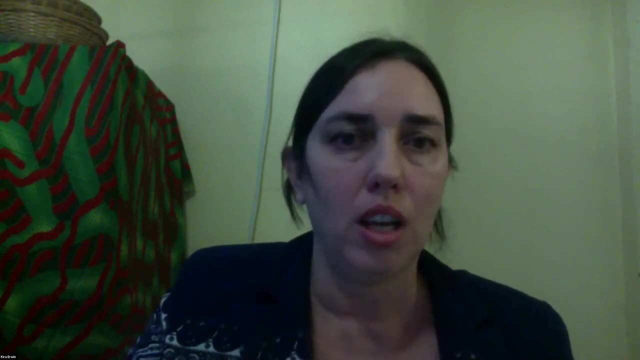 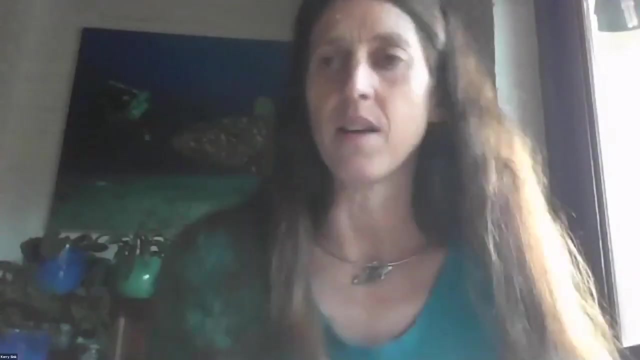 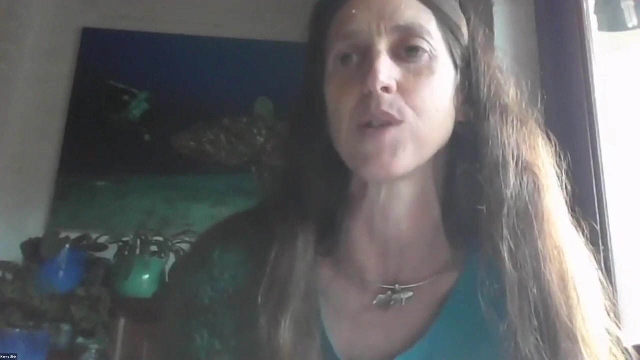 um, and then I think certainly I'd like to respond to Holly, and possibly Dylan would like to, and Sean as well. Thank you, Uh, thanks, Andrea. Yeah, I'm aware of the um statement and actually there are some good collaborations between South Africa and Brazil. 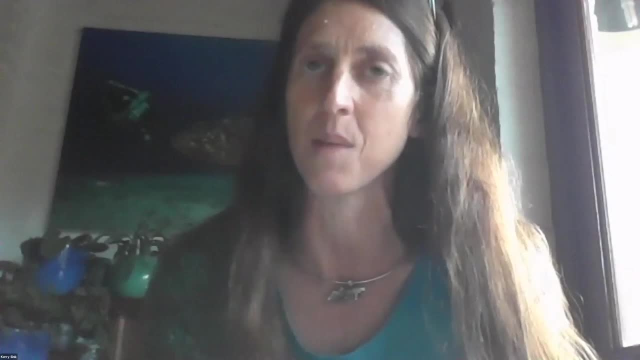 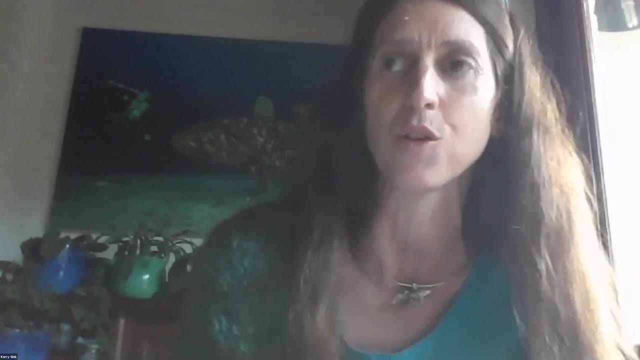 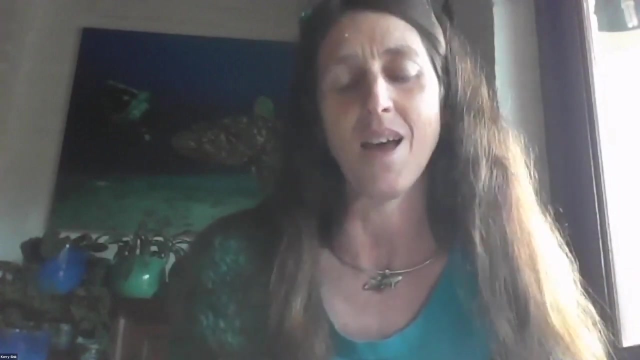 In particular, I have a PhD student shared with them, with someone in Brazil who's helping to develop capacity in taxonomy of our deep water coral species, but also through some of the regional projects in terms of the oil and gas. I was nodding and I was smiling and I was thinking about. 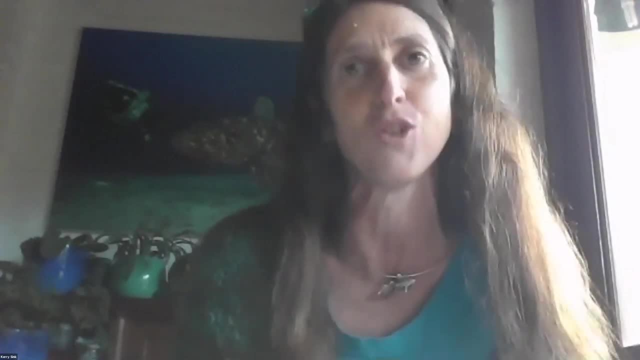 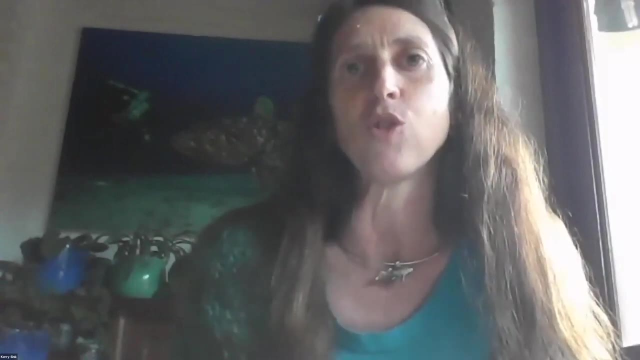 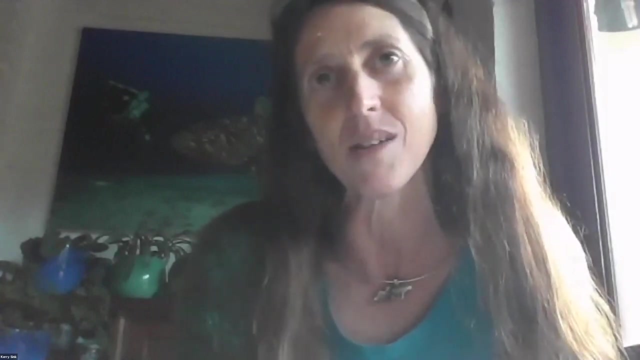 um, some of the more innovative, innovative measures I had to use to build relationships with the oil and gas industry, Um, but really it comes down to those individuals, and the one, the one particular person who I kind of nicknamed our seamounts after, was just someone that kind of understood. 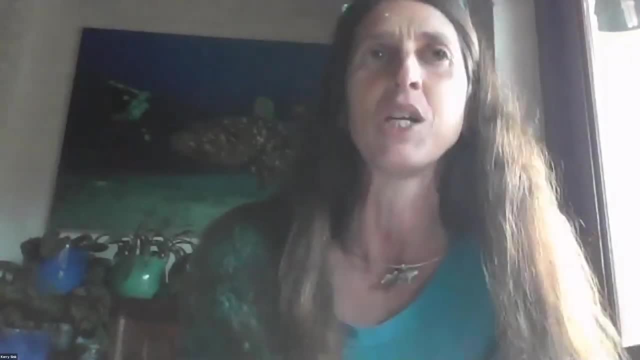 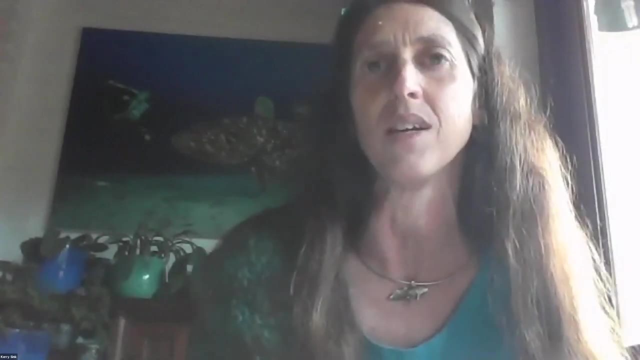 He used to spend a lot of his off time, even though he's an oil executive, spent his off time in nature and in game reserves like the Kruger national park, And so he he said to me: I get what you're trying to do. 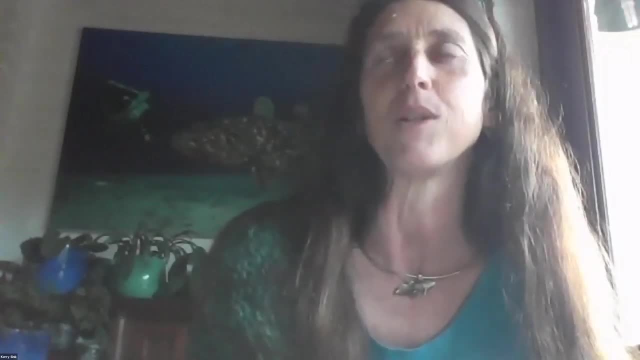 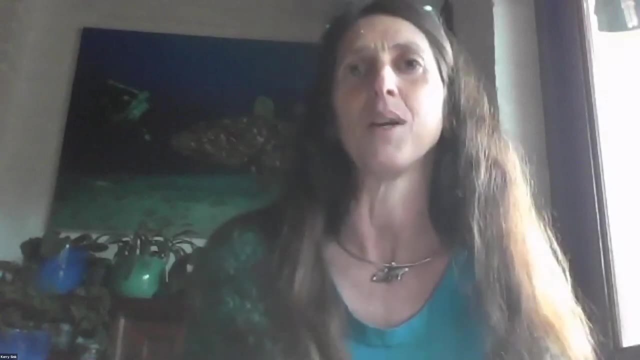 And um, yeah, it was by slowly, slowly building projects. I was telling some of the the one ocean hub team members I even did things like helping oil executives kids with school projects on shells. So I would say, you don't have to die. 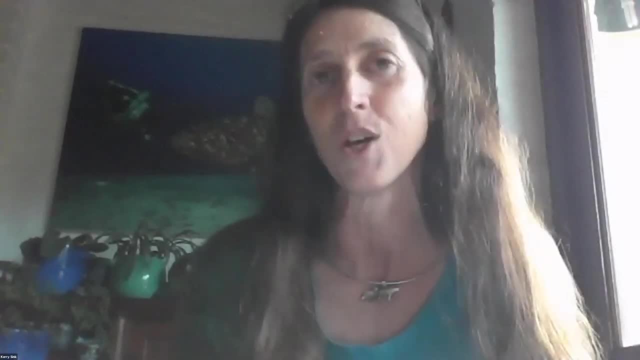 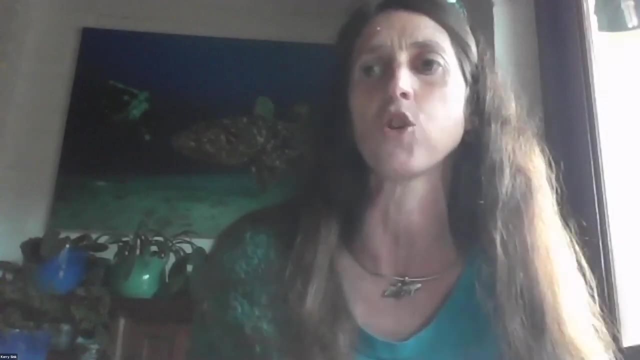 but you do have to step out of your, your comfort zone to sometimes get that data. Um. but I also think that we need to work across government government departments to make sure that the right permits are in place and the procedures in place. 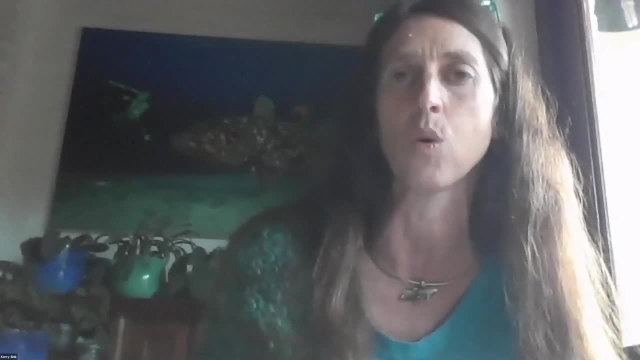 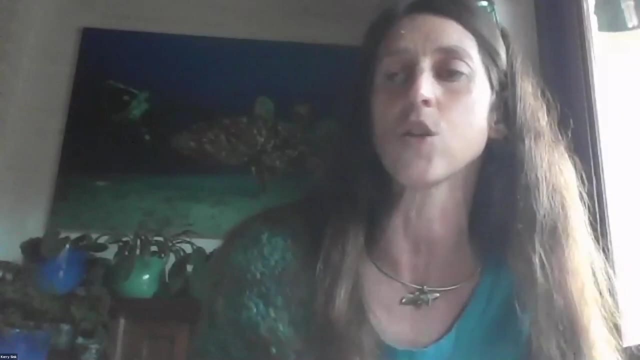 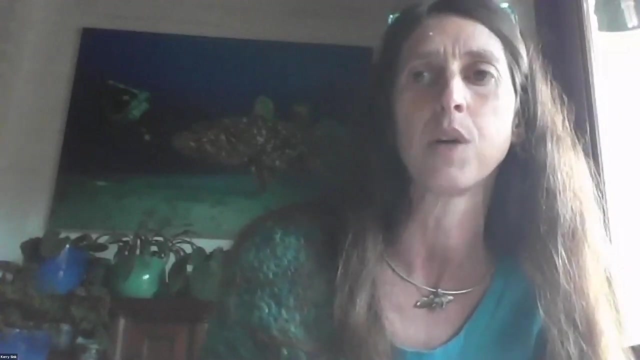 And we have been making some progress in in acquiring shared information through collaborations. We've also done some cooperative research projects and I think that's a really important model for strengthening knowledge and capacity in South Africa to to maybe make use of the vessels and work with industry. 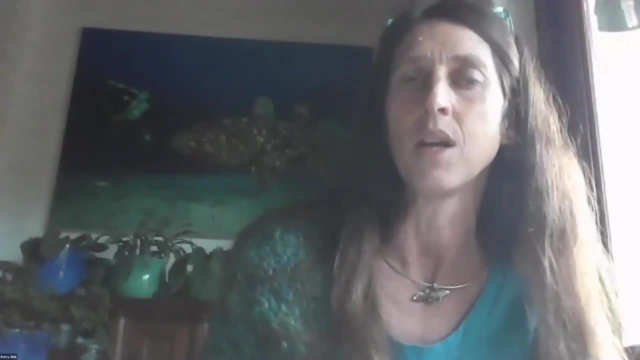 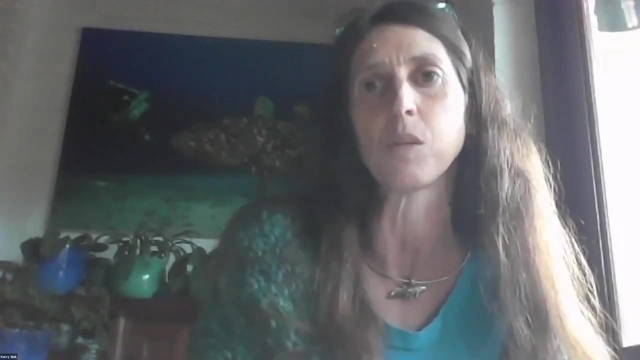 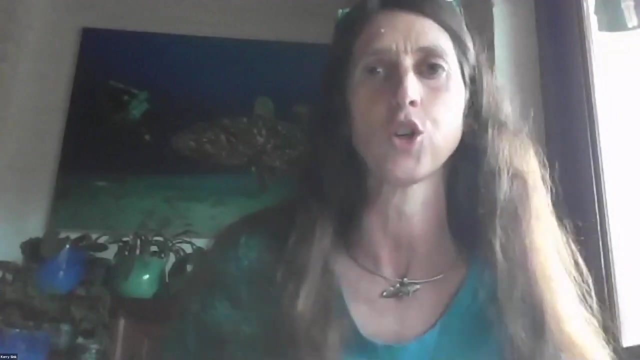 It saves costs for industry too, because they can have someone experienced out there instead of necessarily hiring someone or bringing someone from another country. they can draw from local expertise And, for example, deep water corals or identifying sensitive ecosystems and and that kind of approach. 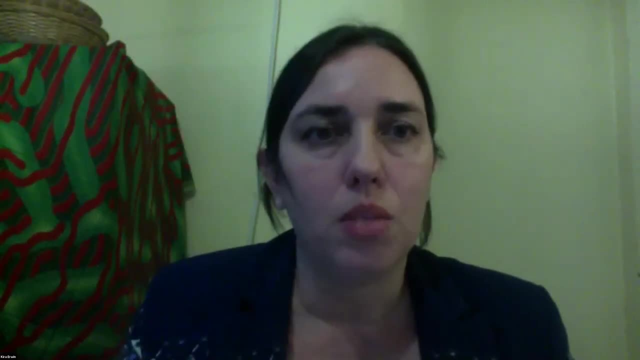 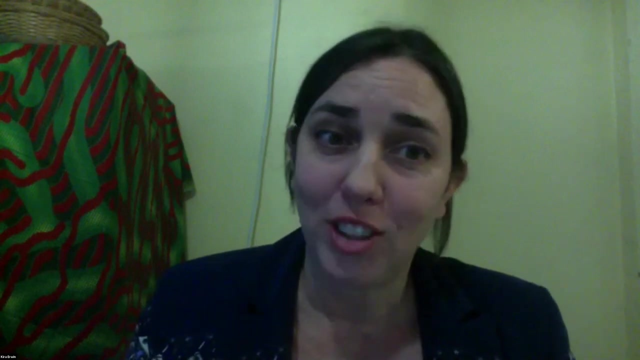 Thanks, Kerry And um Holly. maybe just to pick up on this idea of the less tangible and Kerry's just given an example of how the sort of intangible relationship building that happens even amongst these negotiations. So I think that this really is a critical area at the moment in ocean governance. 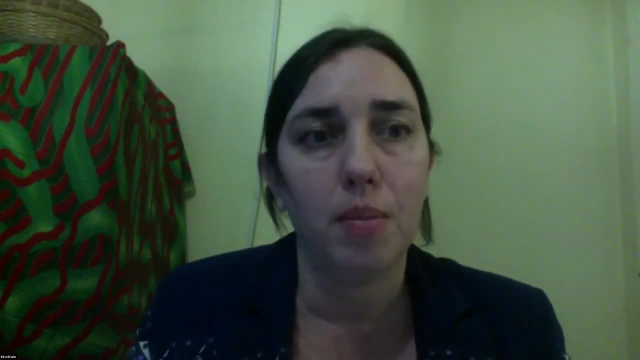 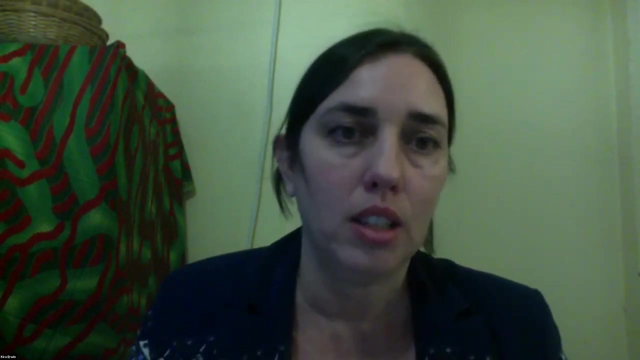 and I'm going to ask Dylan to speak a little bit more about this, And perhaps Elisa also wants to come in, because the one area that is attempting to make some headway here is around the idea of customary law and how you take intangible heritage into account in policy. 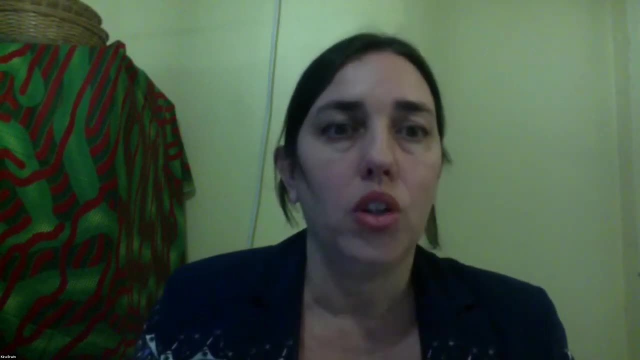 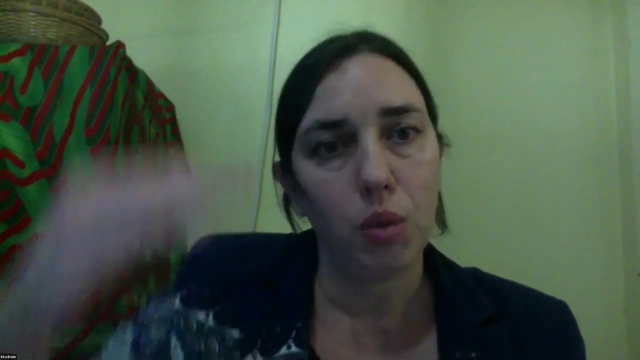 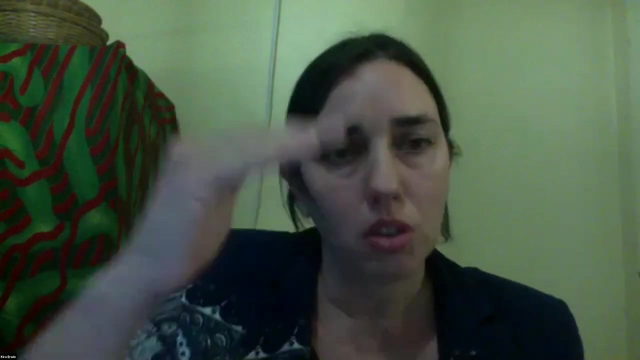 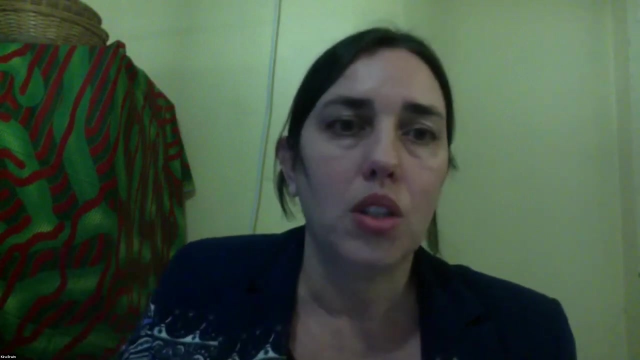 Some of the work that we've been doing in South Africa as a one ocean hub is is thinking quite seriously about how you attempt to make kind of a translation devices between science and sort of the canons of how policy is made and in terms of how spiritual and cultural ideas of the ocean can at least find a way in which they can start to have a conversation, because currently that's not happening. 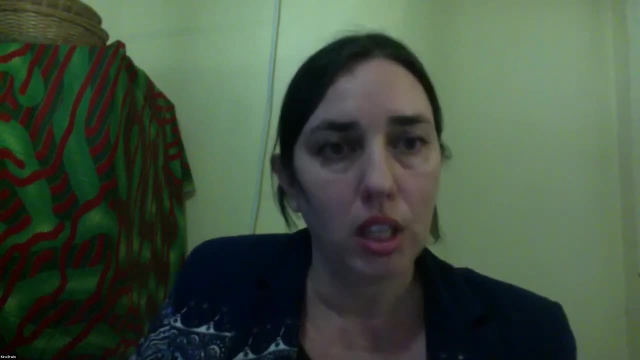 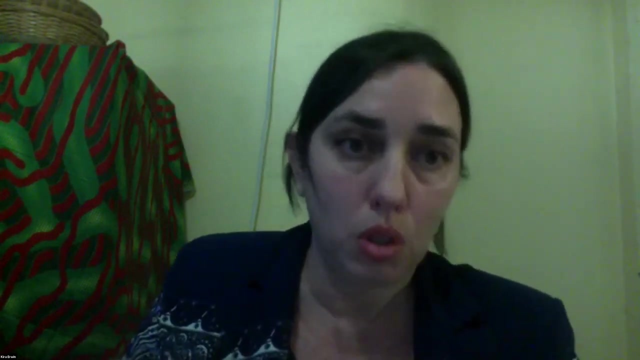 So in most of the policies, especially when there's applications for oil and gas drilling. the one of the reasons for them to not be allowed to explore or to stop the drilling would be if they found marine heritage, which are all based on sort of material artifacts. 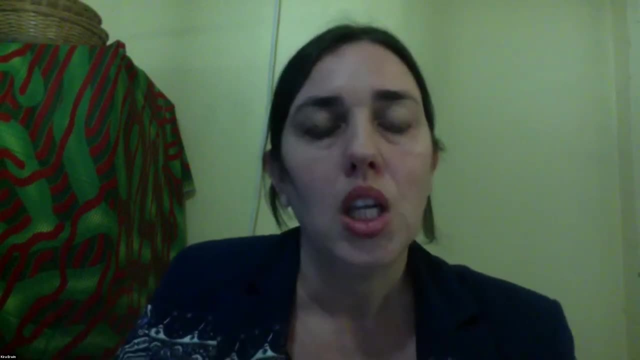 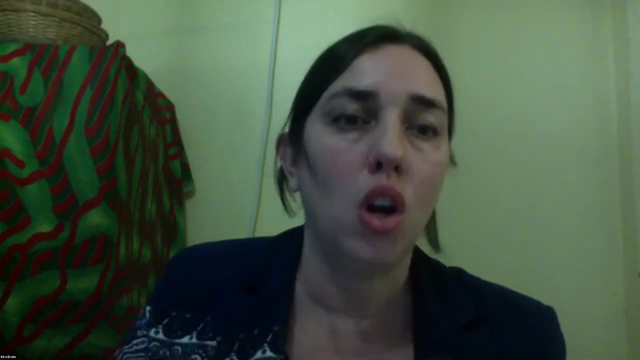 But certainly in our country and in many around the world, there are intangible beliefs and cultural heritage, living heritage around the oceans and the coasts, which are also being damaged and harmed from some of this activity. So it's a critical question about how those interests are listened to. how do they, as Dylan said, 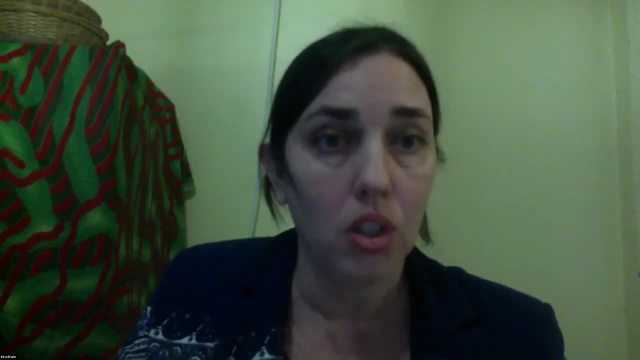 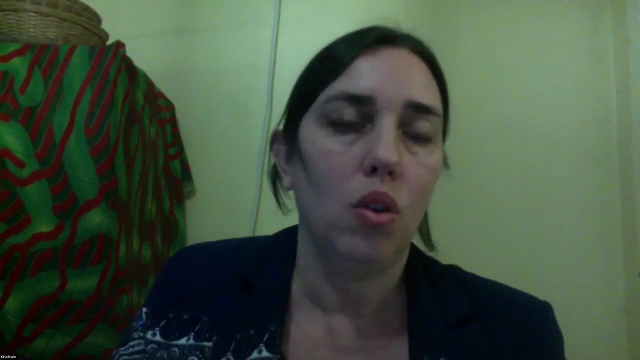 start to be taken as seriously as a concern- and a competing concern, actually compared to just economic livelihood or or looking for resources in the oceans. So, Dylan and Alisa, I don't know if you'd like to add to that point. 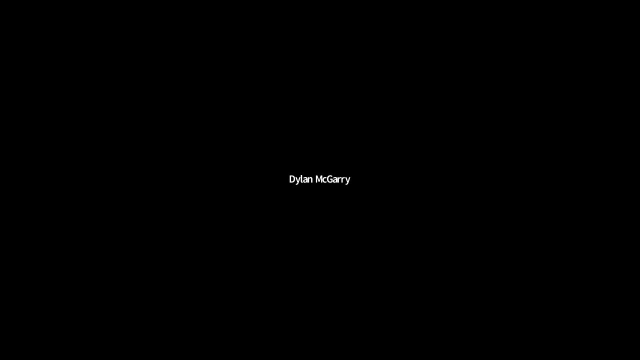 I would love, love to Thanks, Kira. I'm going to keep my video off because my internet's a bit shaky. Can you hear me? Um, I hope so. Uh, so I just wanted to say that, um, I thought of some of the barriers, Holly, like just off off the cuff, because there's quite a few, but one was, um, the lack of, like, legitimate, legitimate spaces for people to share their meanings and values of the ocean We have. we don't have many spaces in which these can be negotiated. 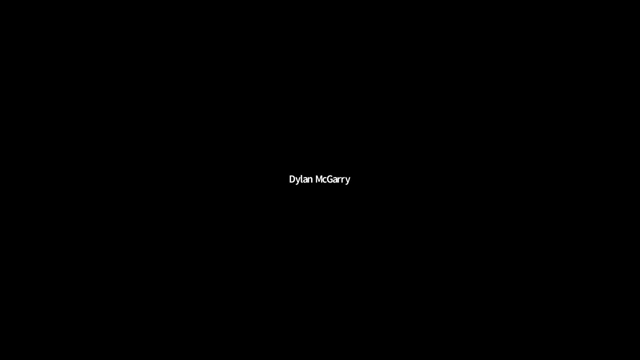 So one is actually just creating and not relying on the old, the old ones, Um, or the, the current established systems for these, these um questions to be negotiated. So what's needed is kind of a meaningful dialogical process. 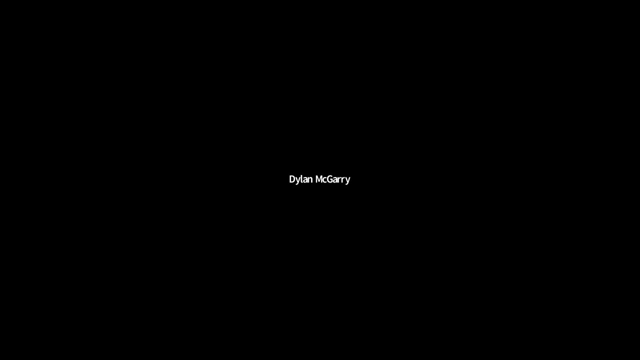 And I think one of the responses is any practices that can engage empathy um between different groups, and empathy being a very powerful tool in this Um. so one of the one of the ways in which you can create these translations is one of the best allies we can have in this work. 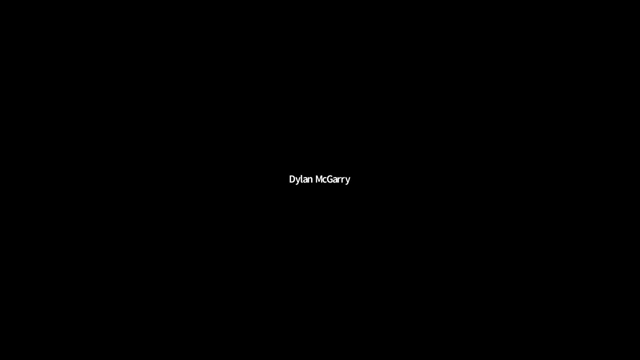 So actually this is a big part of the work, but I think the most important thing is is is to have these works and there's there's a very strong commitment around ocean governance and intangible heritage, is working with artists and cultural practitioners and how 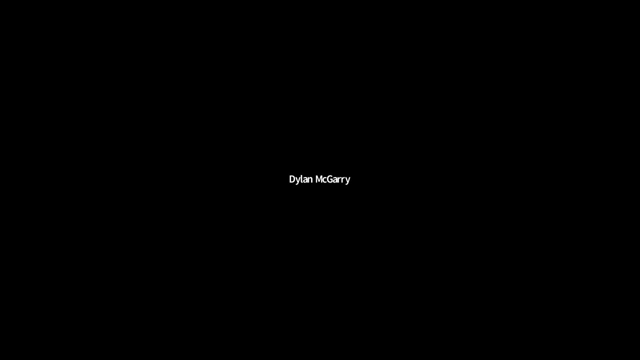 We have. Oh, Can you get a program to support artists in helping in this negotiation of making the intangible at least somewhat tangible through storytelling, through music and dance and um other forms of embodied practices? Um, we've been experimenting for some time. 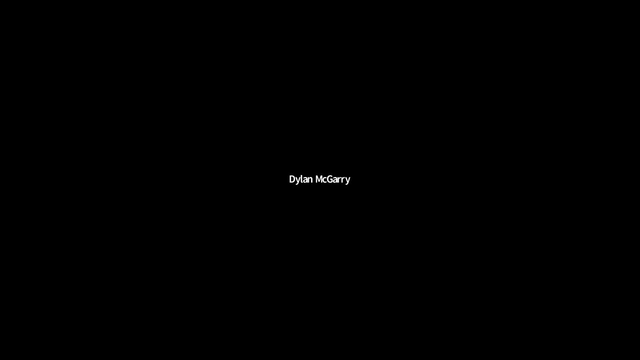 Um time with theater, we developed a methodology called empathy theater, as well as um, we're moving into film and animation as a way to make these invisible uh meanings of the ocean visible to policymakers, scientists and other knowledge practitioners and um, and i think one of the 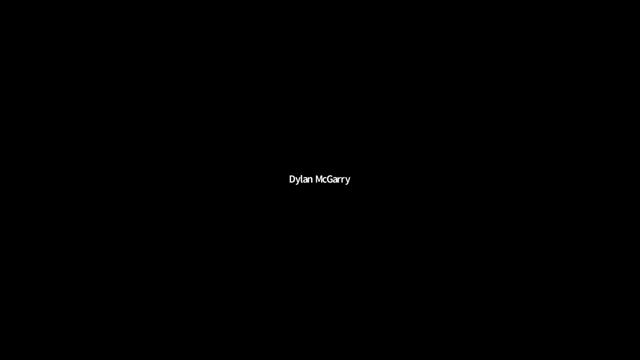 is the idea of universe, especially in legal processes and governance, is this idea that there's um like a universal truth and but we're moving more and more into understanding that there's multiple truths and a plural, resonant world and that there's these really interesting relationships, and it's about um kind of creating entrances and exits between these different 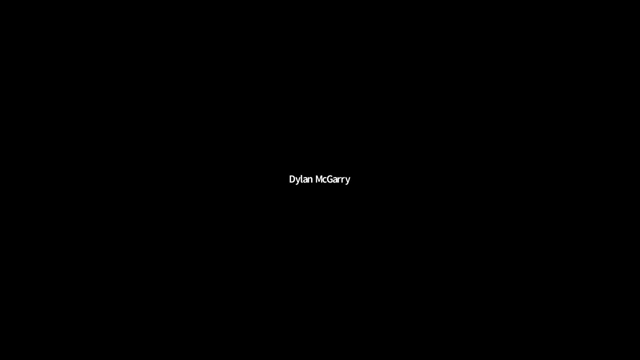 worldviews through um, working in in solidarity with artists and storytellers and other creative practitioners and the cultural practitioners themselves, who who carry this knowledge, um, and so i suppose one of the ways we respond is, rather than trying to make policies that are often kind of, if we imagine the responses, to create something for a solo. 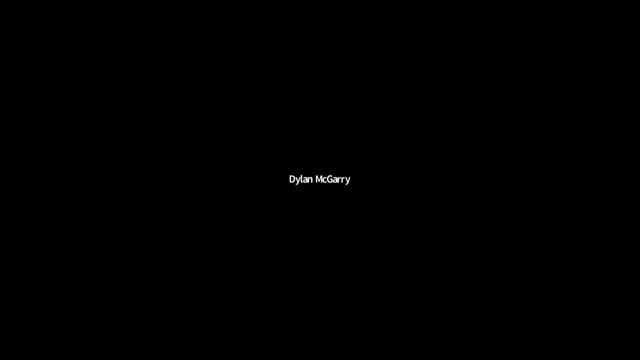 pianist. we're actually wanting to create policies that are writing music for orchestras, for many different instruments to be able to, to play this response or this plan or this policy. not just a solo soloist and not just a single beneficiary, but many. um, but yeah, i would, i would. 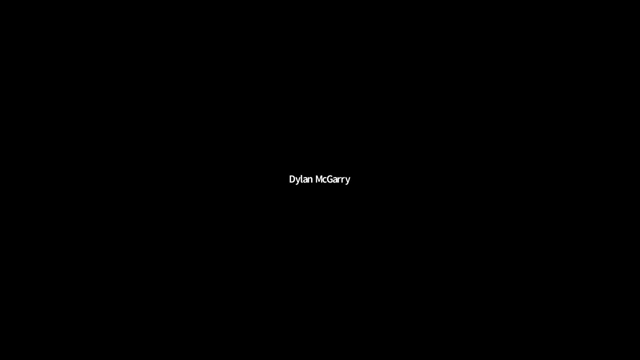 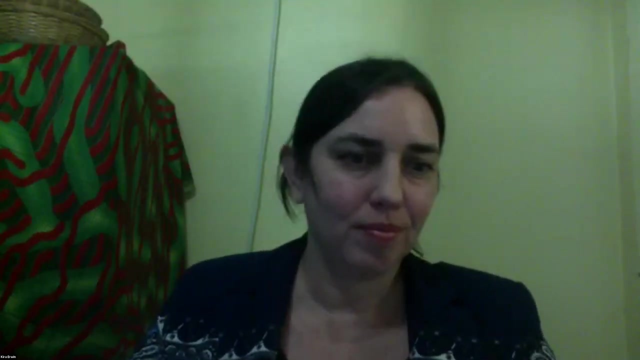 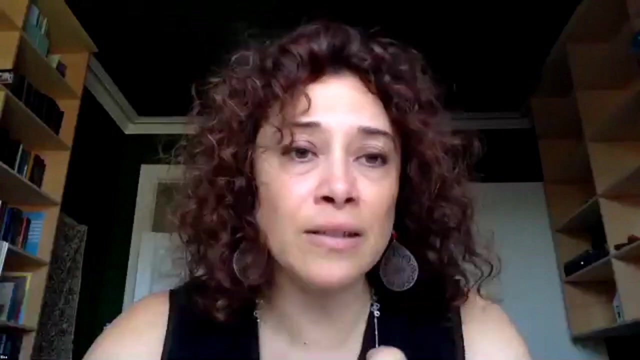 love to follow up on it, on that question even more, but i'll leave it there. it's a wonderful question. thanks, holly. thanks, though, elisa. yeah, just to compliment and say i think you know there are legal barriers as well to having this um different values recognized, and i think for 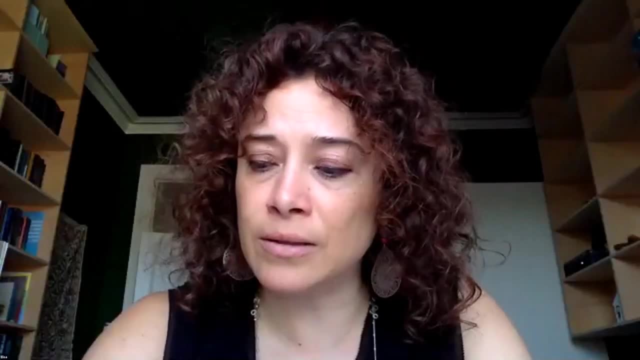 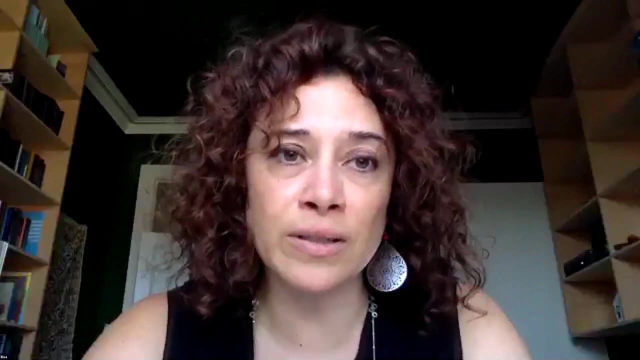 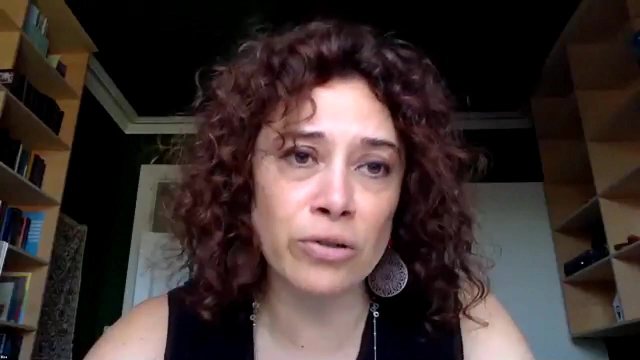 for the, for those holding those values to feel that, um, they have actually legal entitlements to have their concerns, um, voiced and heard in decision making around the conservation and use of the ocean. i mean those of you who, on this call, are familiar with the convention on the law of the sea and you know the wilder's recognition of multiple values there are. 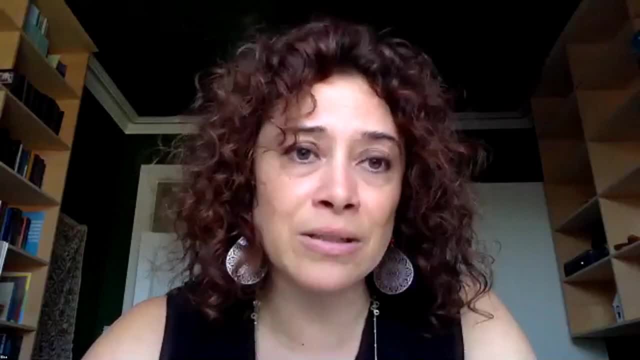 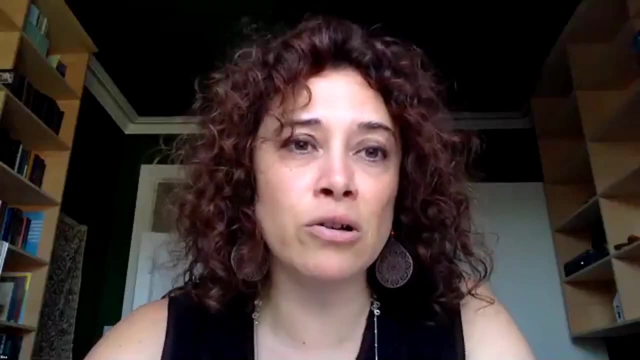 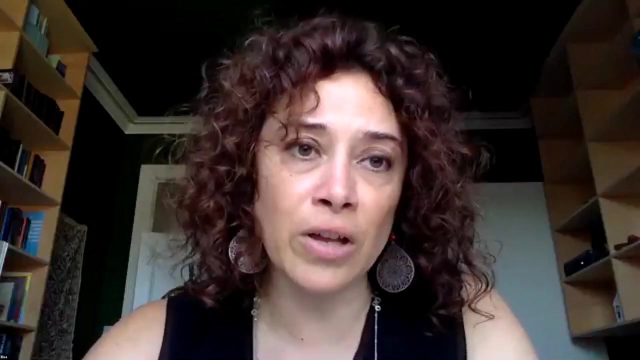 some aspects that maybe are not as addressed in as much detail as others, and i think the questions about intangible heritage, customary laws, traditional knowledge- those are not necessarily themes that we find explicitly addressed under the convention on the law of the sea. however, many of you may also be familiar with the convention on biological diversity. 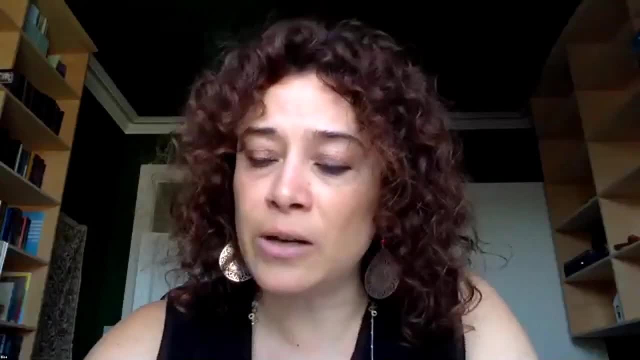 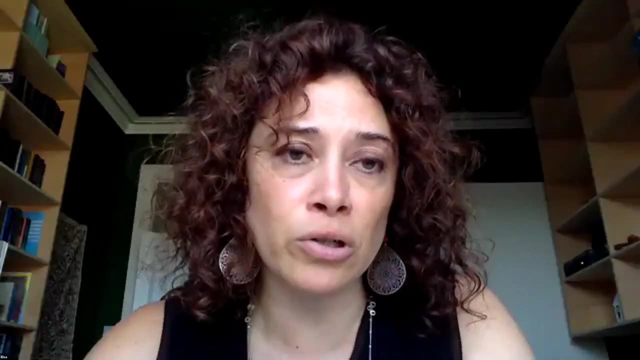 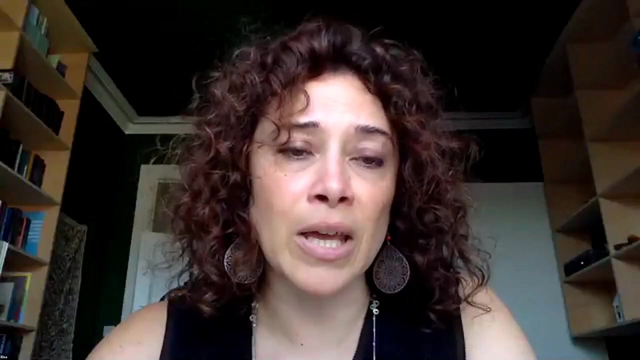 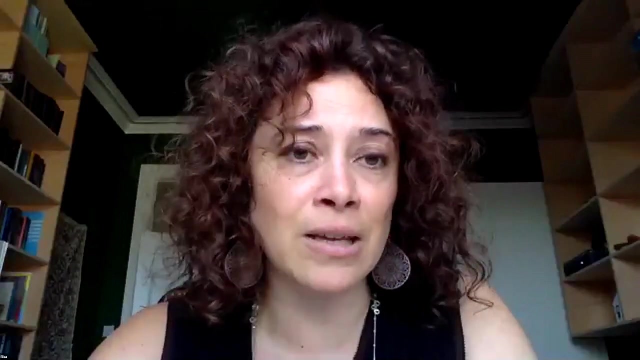 which has done a lot of work on marine biodiversity and, of course, has done a lot of work also in terms of understanding the contributions and the need for protection of the traditional knowledge and sustainable customary practices of indigenous peoples and local communities. um, and we, we know as international lawyers that all those parties to the cbd are also parties to anklos and they are 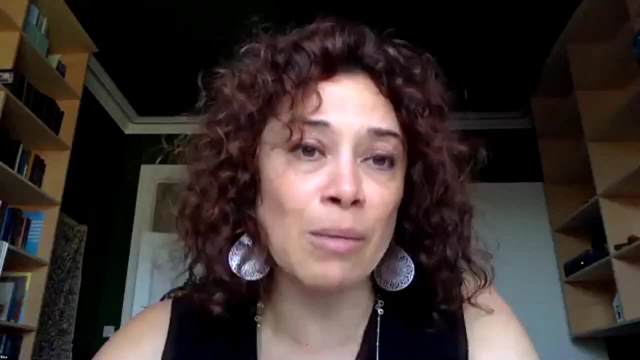 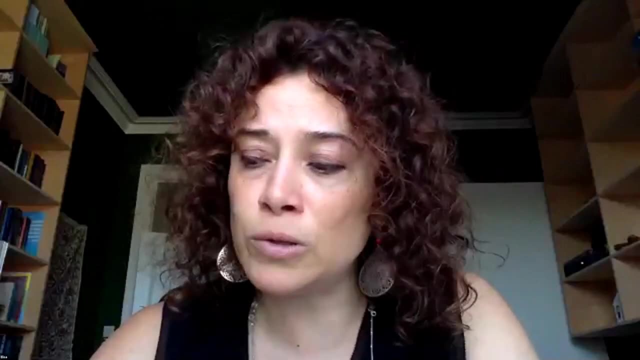 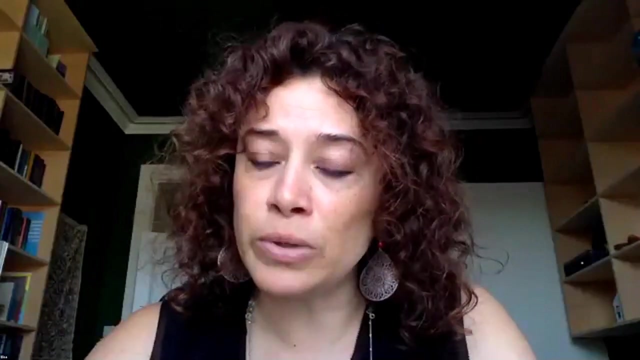 expected to implement their international obligation in a mutually supportive manner. so one way, one. one thing: the ocean hub is exploring, but also other lawyers around the world is understanding what that means, what governments and other actors at the national level need to do to really ensure both the conservation of the ocean and sustainable use of the ocean, including 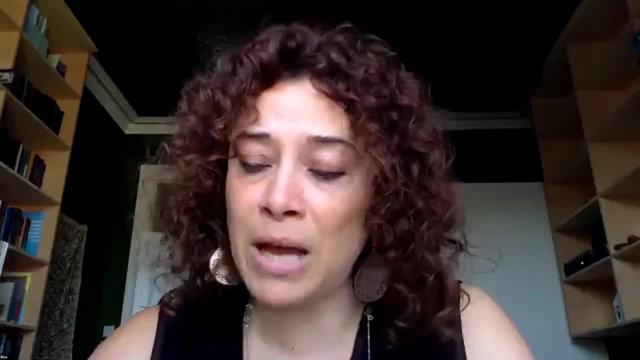 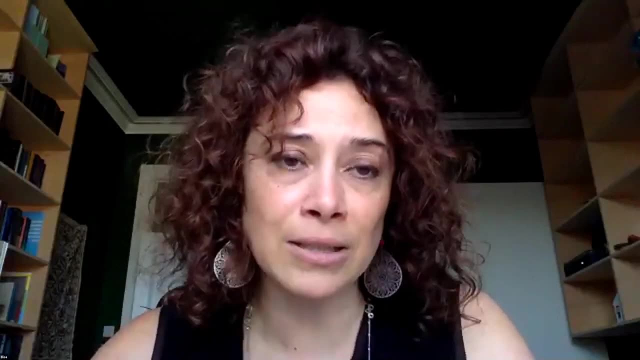 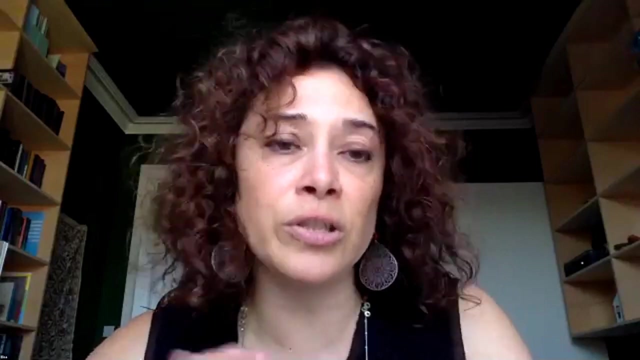 marine biodiversity, but also respecting and and maximizing the opportunities to learn for the benefit of conservation and sustainability and the use of the ocean as a source of sustainable use from traditional practices, traditional beliefs um and traditional knowledge, and more and more we see how that traditional knowledge internationally. 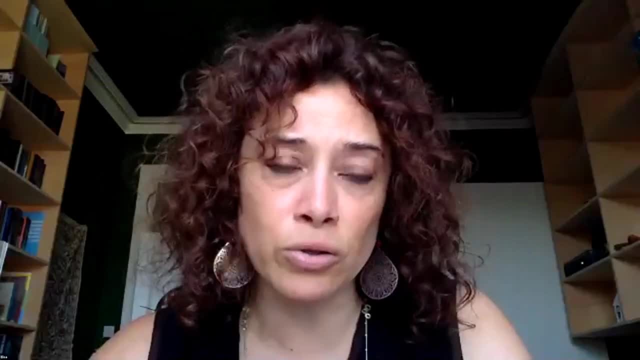 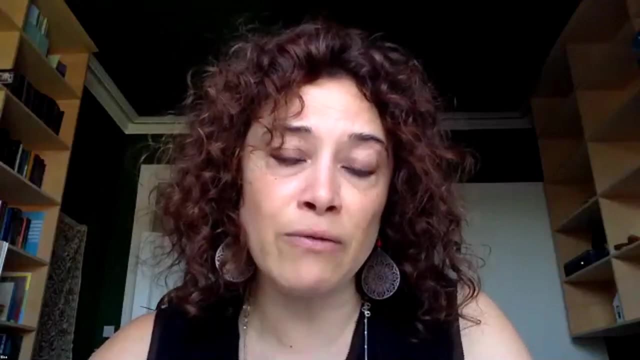 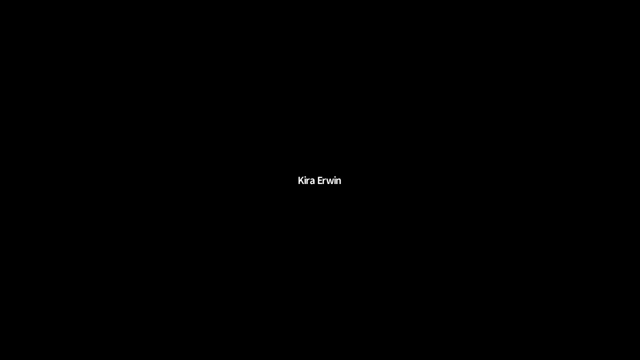 although maybe in different ways nationally, is recognized as an equal source of knowledge in in decision-making processes, um, and i think the other thing that that i would like to contribute from, from a legal perspective, what dylan was saying about, what are the spaces for the different international regimes um to be implemented at the national level and for 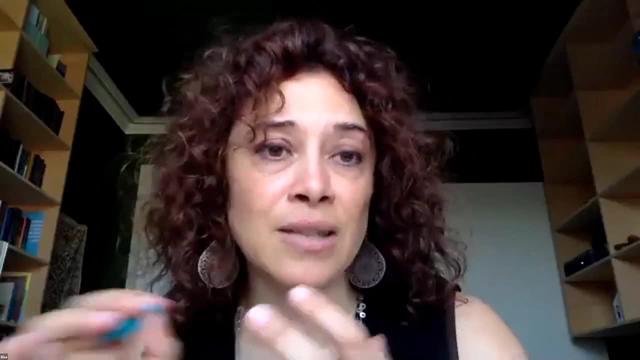 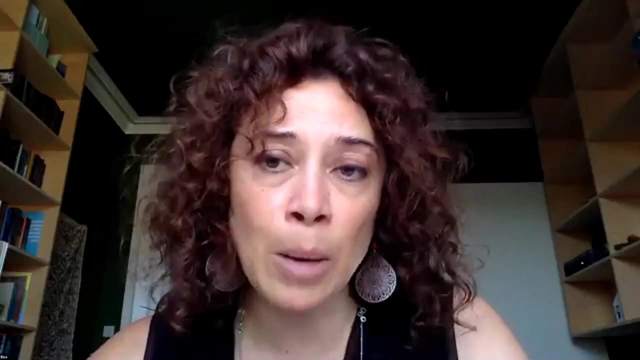 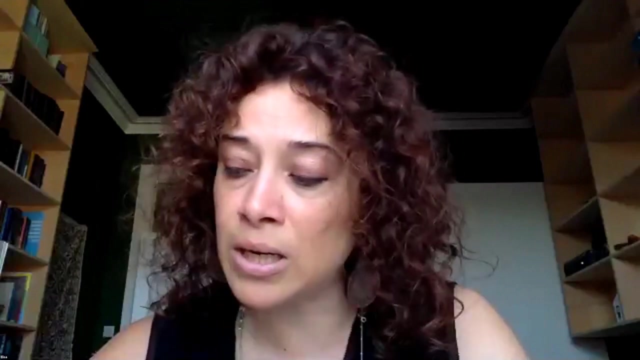 different groups. they have maybe different stakes in some of the elements that are protected internationally. to have a dialogue, and one of the things we're looking into at the one ocean hub- but many of you may be very familiar with- is how environmental impact assessments may be processes. 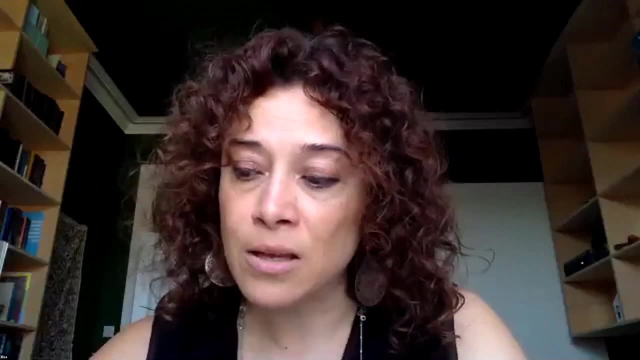 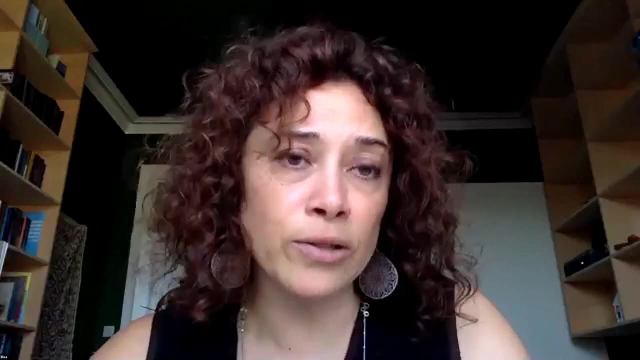 where we could have a dialogue about different- um, tangible and intangible- values of the oceans. the environmental impact assessments may be processes that are easily monetized, one that may have to do with, uh, well-known uses of the ocean, be that, you know, offshore oil and gas, or mining or fishing. 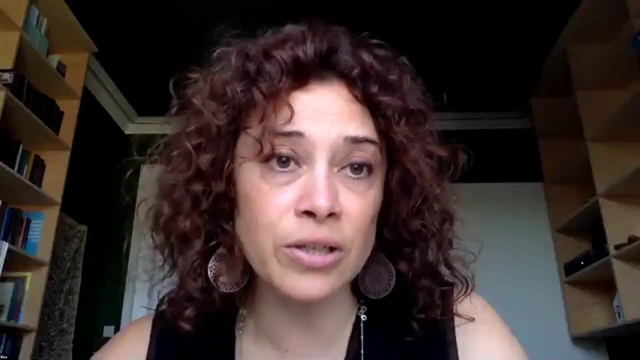 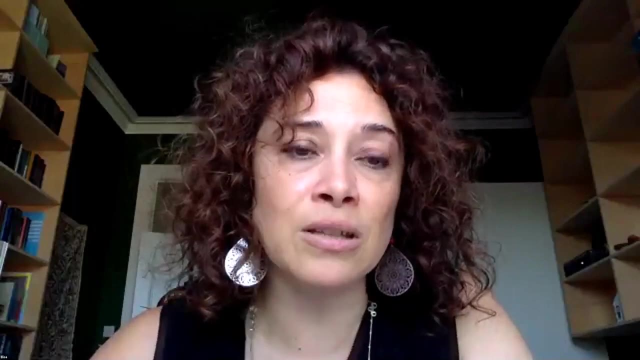 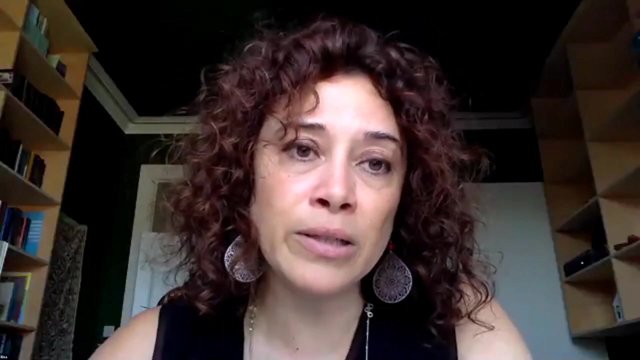 but also the other values- cultural, spiritual values, small-scale fishing uses, and how those environmental impact assessments can move from a process that's often very driven by damage limitation and damage control to a process where instead we can, we can try and all put our heads together and think about. 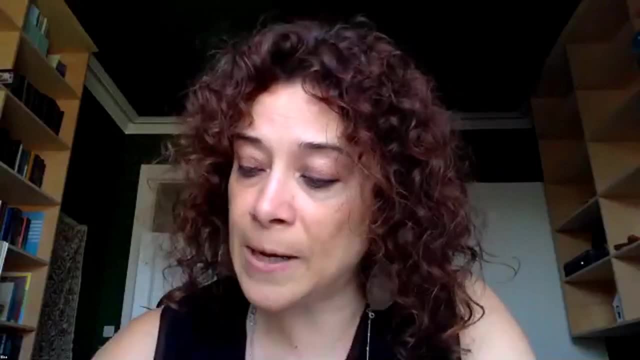 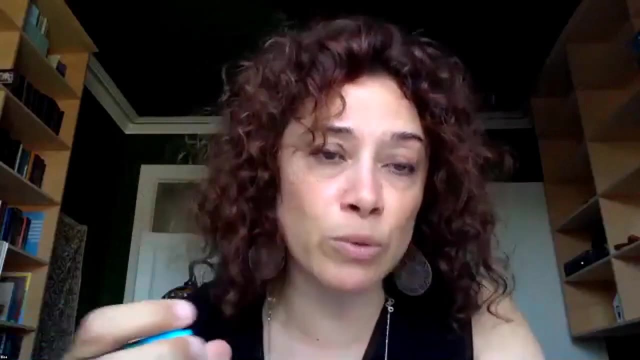 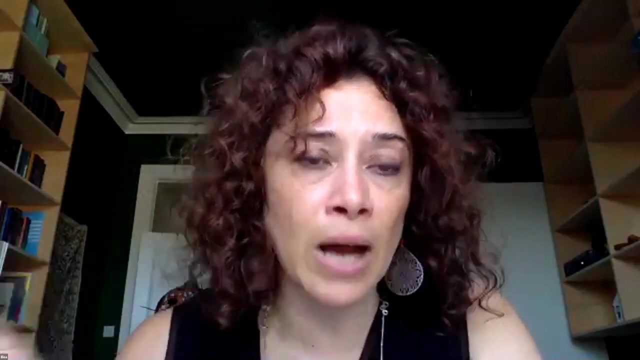 maximizing benefits for different groups, um, and and really understanding, in the balancing that carrie mentioned, how, in what ways different groups that come to the table with their own agenda and are there to push that agenda forward, how, through the process, they can learn better where other people are coming from and how there may be opportunities to to cooperate and identify. 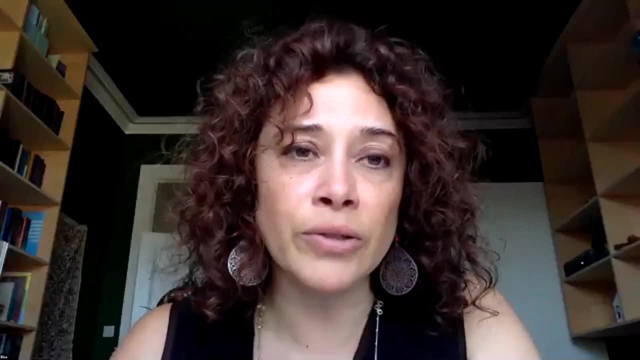 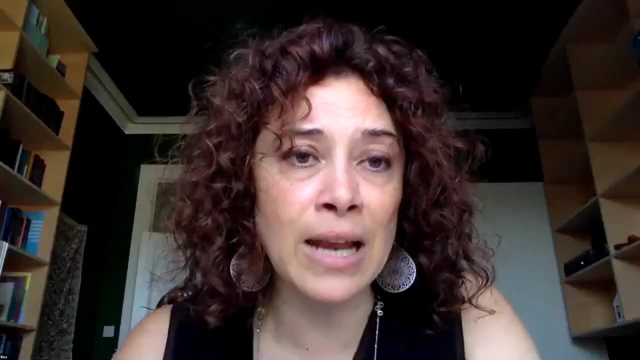 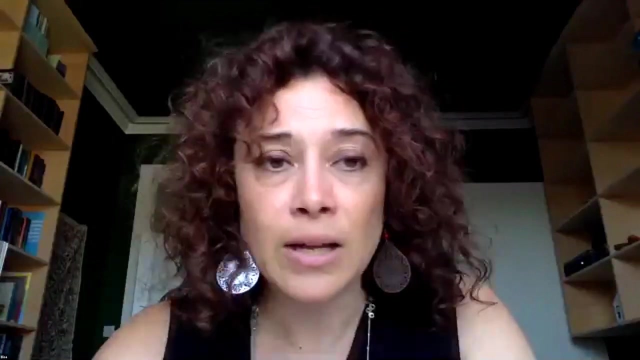 common grounds and i think what carrie shared earlier around understanding fine-grained priorities with oil and gas through that engagement, also getting, as andre was highlighting, into a place where you can collaborate and share data because you finally find a common agenda to work towards and, ideally, 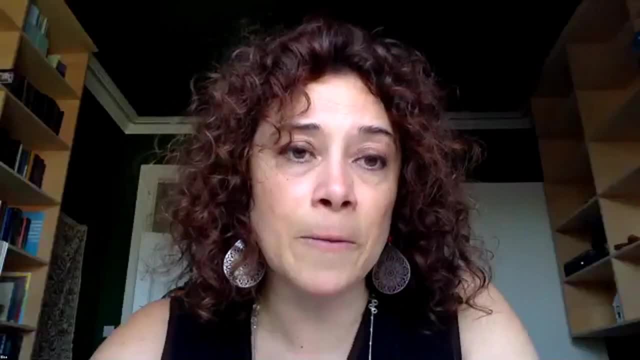 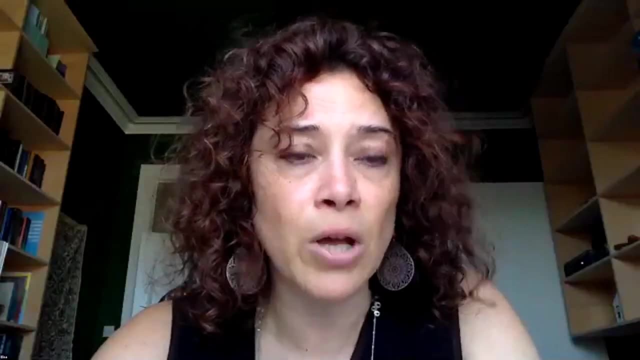 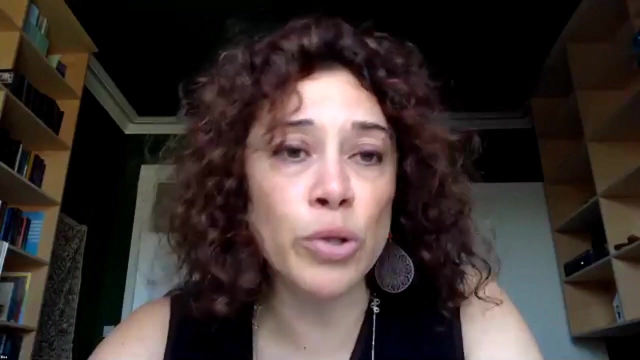 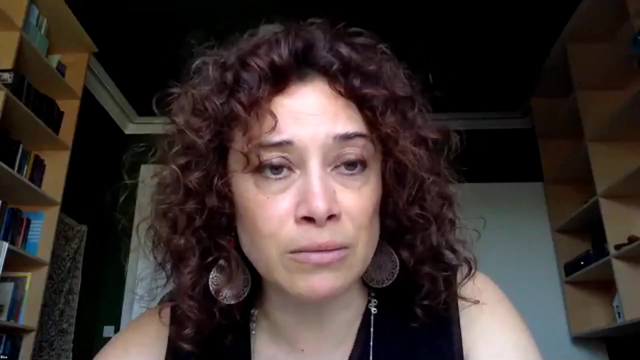 going even forward, but making through the process, um giving voice to those that usually are not sitting at that table. we saw the picture from carrie's presentation of oil industry represented and marine scientists, but we didn't see many other community representatives who would have felt equally vested in whatever the decision would have been either regarding creating a marine 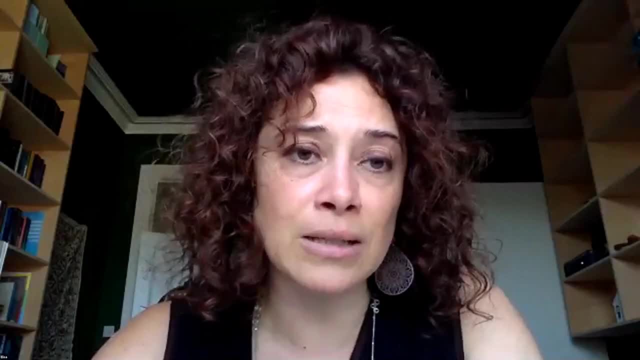 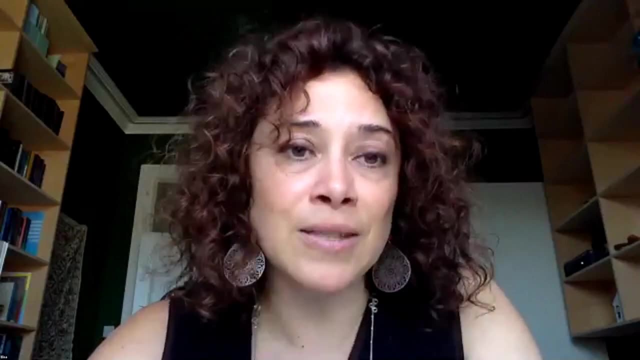 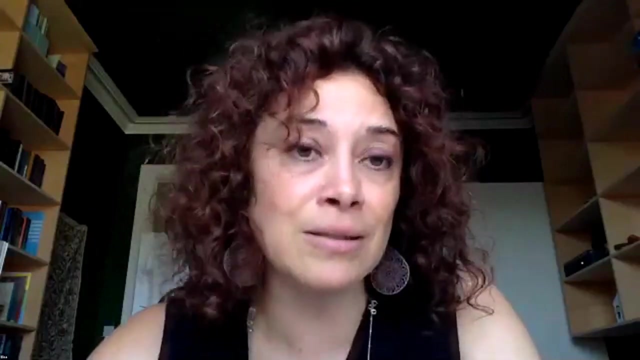 protected area or going ahead with an oil and gas offshore project. so eias could provide that opportunity, but they do require, i think, some additional work, be that in how legislation at the national level is implemented or is framed and the practices that are being implemented around it, and how, for instance, eia consultants see their role and may facilitate dialogue and 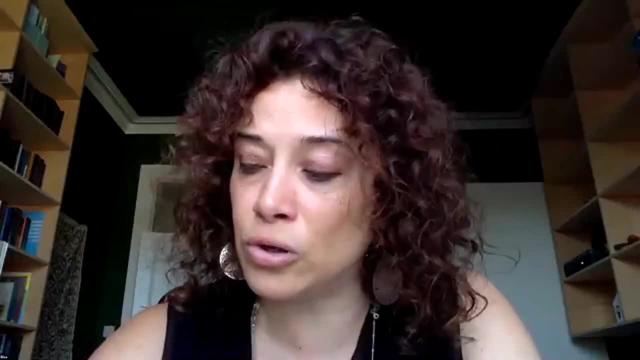 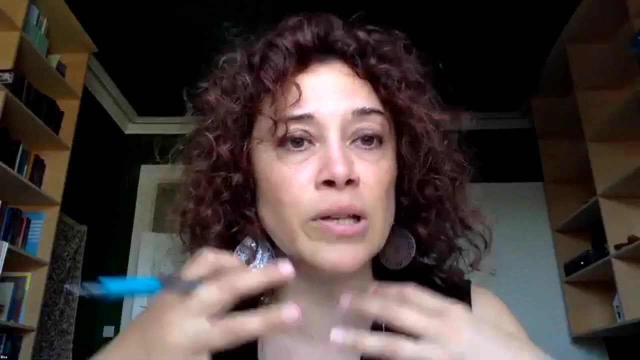 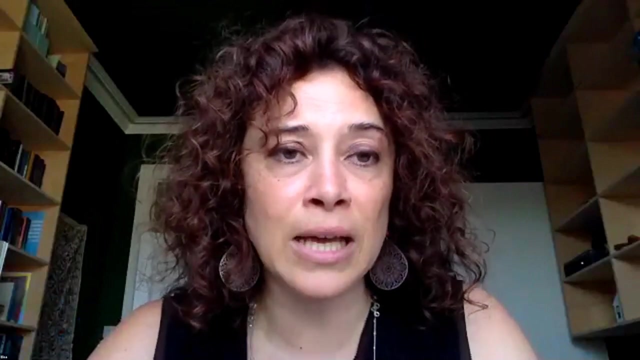 you know, including information and knowledge from different sources or not, to including that point that dylan made about involving artists and ways in which people can not only engage in these negotiations in a very, um, kind of rational and maximizing outputs way, but in a in a more empathic way to learn from others and and understand their position. 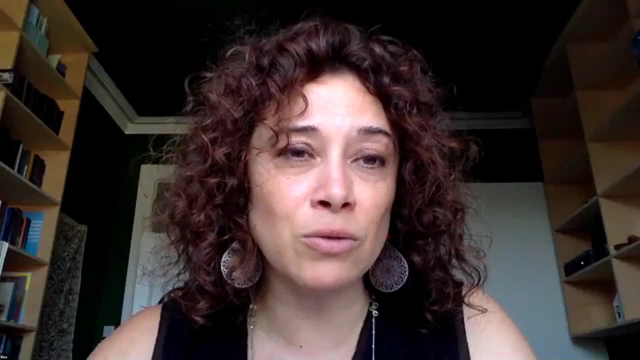 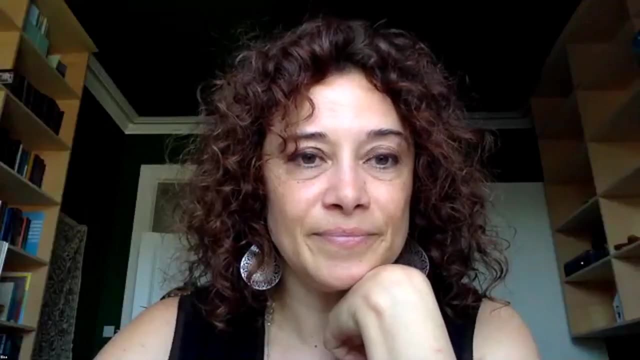 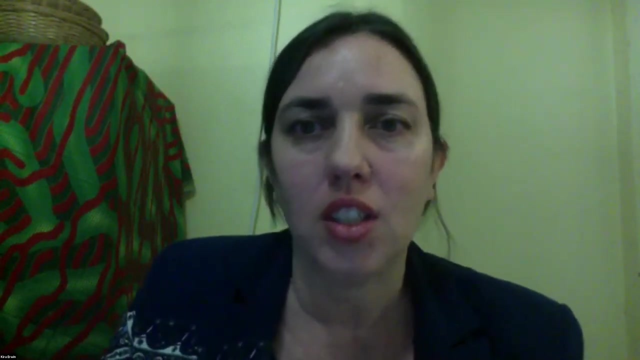 and through that move maybe in a space when they can be more open to co-develop solutions together. thanks so much, elisa. we've got two more questions. um, aditya has asked in the chat and kirsty i will hand over to uh in a minute to ask a question of kerry, but the one question 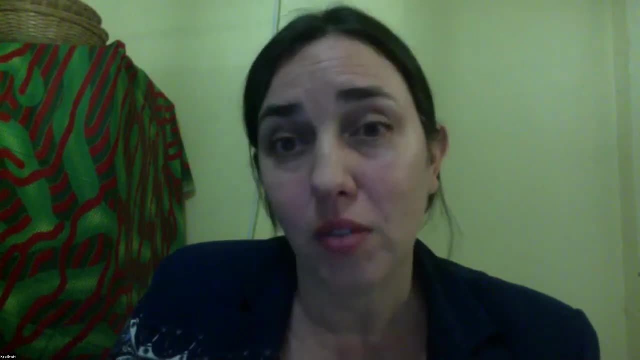 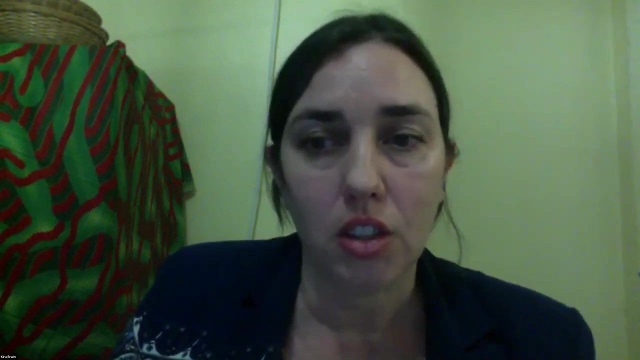 kerry, coming from aditya, is: how responsive is the government of south africa to scientific papers and what are the challenges besides the sort of bureaucratic issue? and then if we can just give kirsty a chance to ask her question, because you may want to answer it together. so, kirsty, can i hand 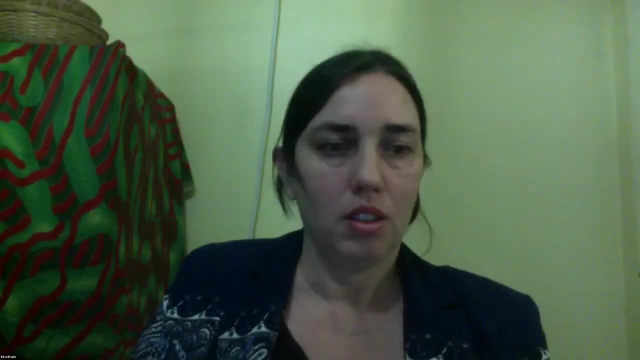 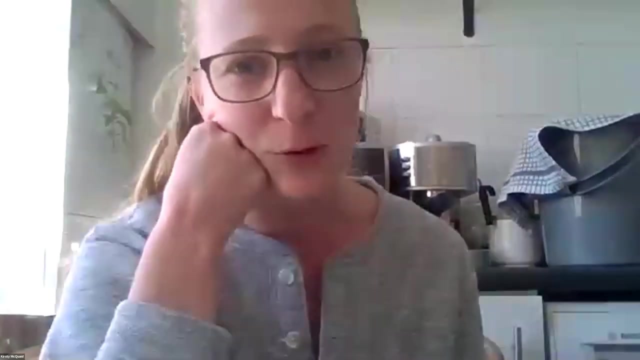 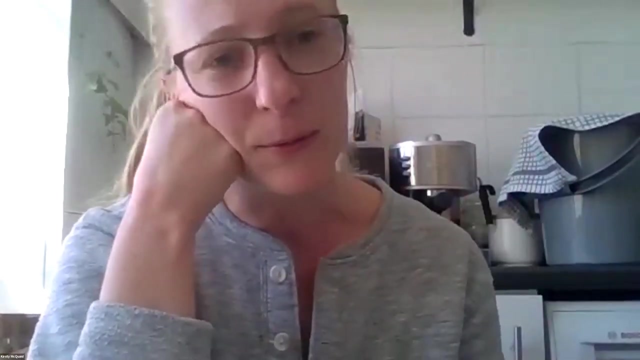 over to you. hi, yes, sorry, um, i just wanted to ask- it's a much simpler question, but i guess what are the key kind of um bits of advice, if you have to distill it all down. um, if someone wanted to engage in policy like a scientist or a social scientist or whatever, 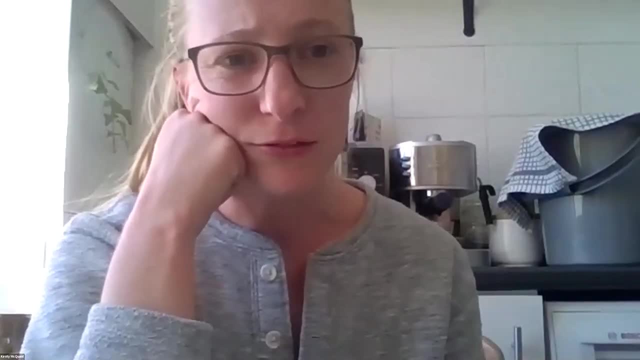 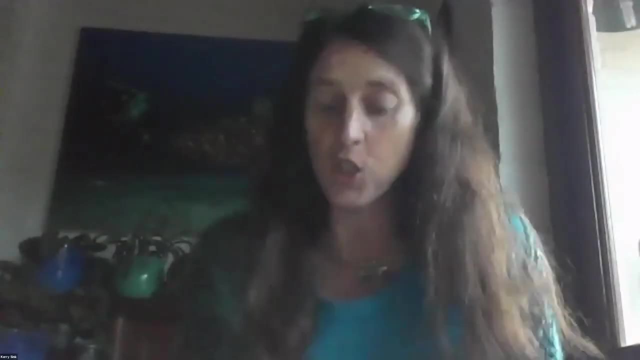 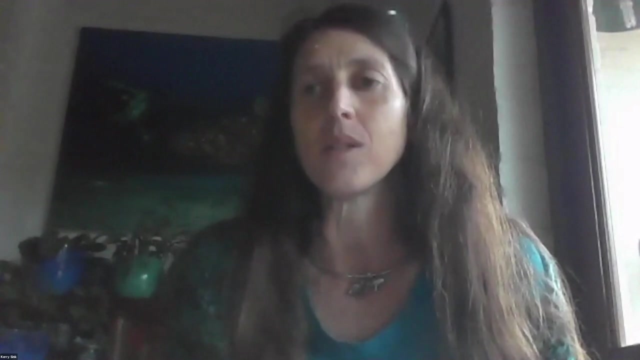 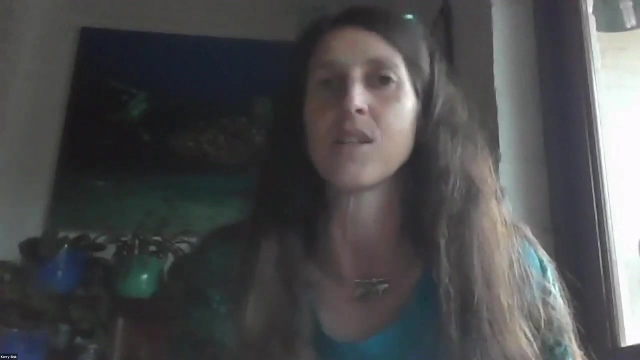 what would be the key pieces of advice that you would give? Thanks, Thanks both. So the first question. that's quite complicated Overall. I mean, the South African government is respectful of science. Science receives a substantial portion of funding and scientists are often listened to. 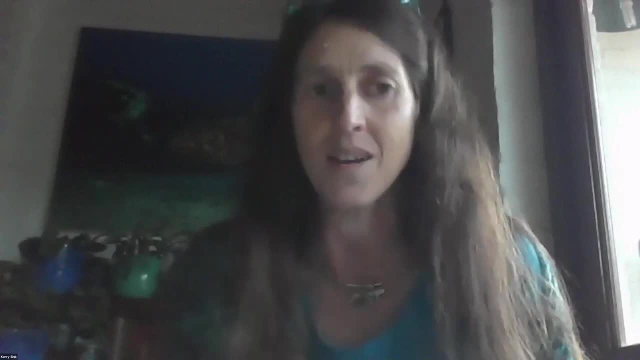 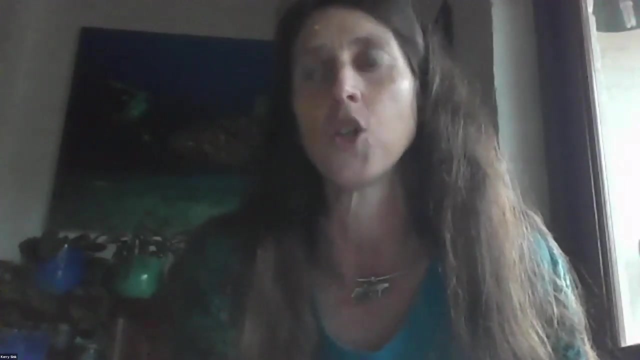 but they're not usually the loudest voice. That's what I can say. I think, in the work to take this forward, one of the key lessons- if I can blend the responses together- for me was we really needed to invest earlier in communication And in shepherding this network. 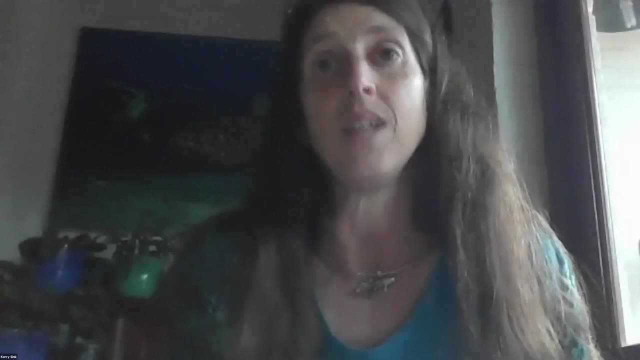 of protected areas through cabinets. we really needed a strong science base, So that was critical, And I had a very strong network of scientists- probably more than 30 scientists that contributed into this work. So there was a strong science foundation, But what we didn't do 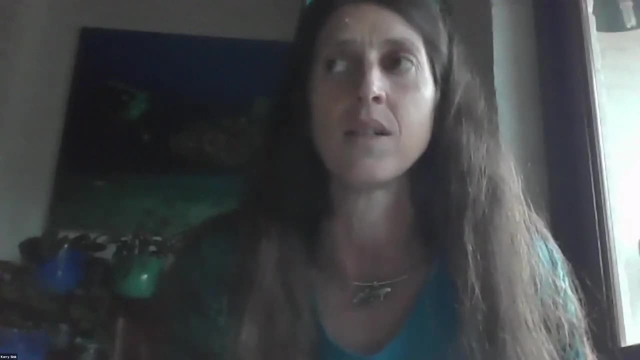 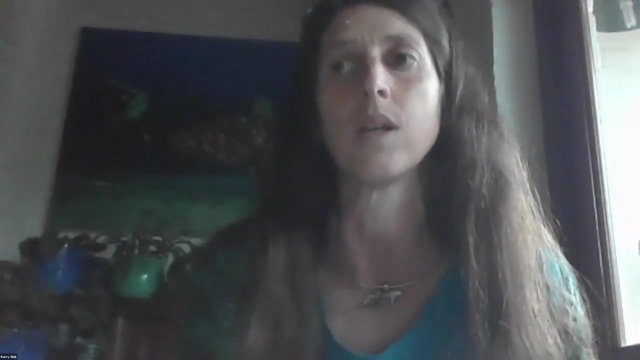 well was to articulate the need for protected areas and maybe the benefits, well, until quite late in the process, And I think that was one of the key things that we, I think, sealed our discourse, And what I want to say to anyone is that Moli игры. 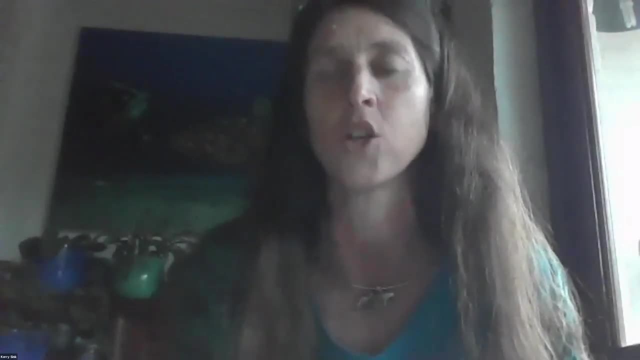 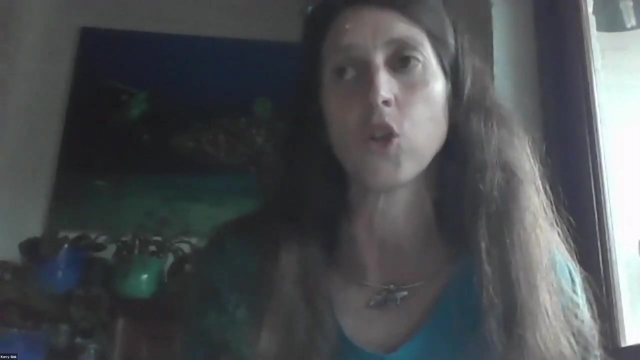 I believe has a lot to do with the have not really locked things in cabinets, So no talking to policymakers. You need to be very brief And it's good- the opposite of what you would normally do when you give a scientific explanation- and- and I think that the power of like the 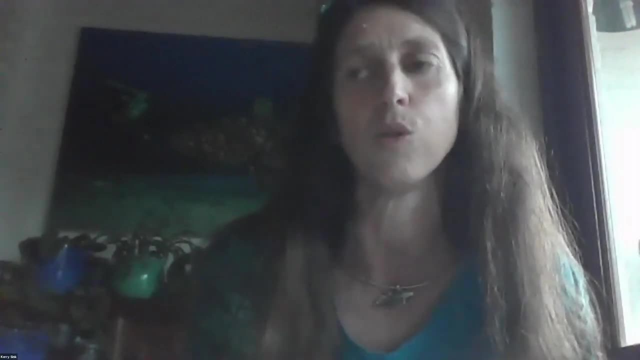 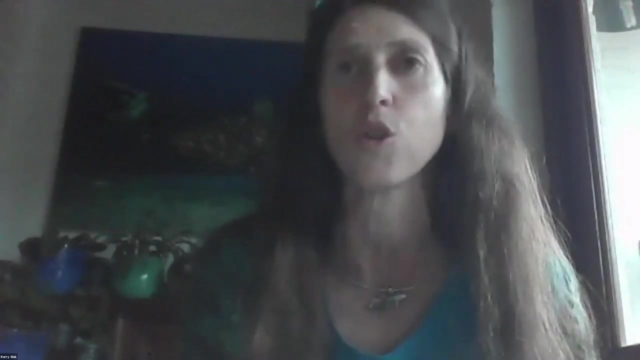 imagery and showing people has been very, very important and Minister Melewa, a environment minister forward. she ended understood what sean was saying, that it's not only the exciting things, it's also the boring things. and and the one day i was amazed when she had a meeting with x and mobile and she 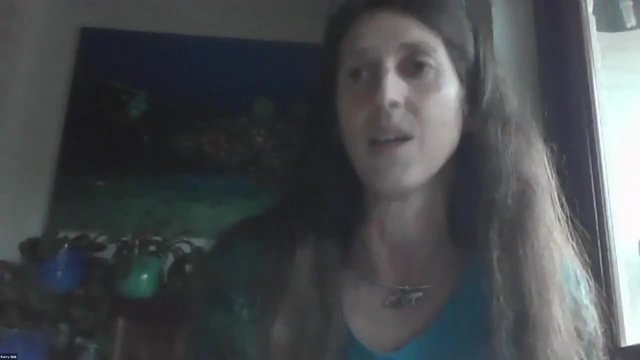 was talking to them about the myths and, um, i had given her slideshows about the various areas and she actually brought up slideshows and she also had that sense of wonder and was showing people the giant spider crabs in the mud and- and she was talking about this in her response to to the oil. 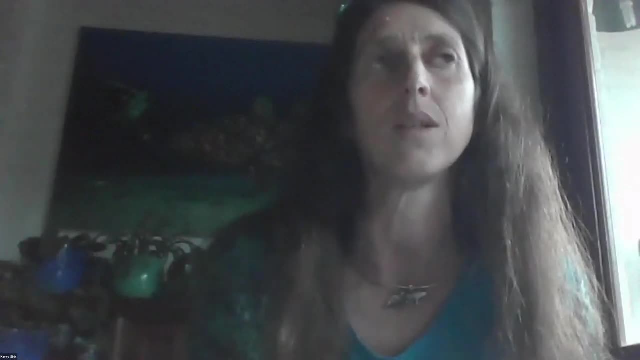 and gas industry. so i think that's a critical element. um and we we faced serious communication challenges. um, in terms of other lessons, is when you want to make a change like this or achieve something difficult. you need to remember that this kind of work is is really. i like to use the 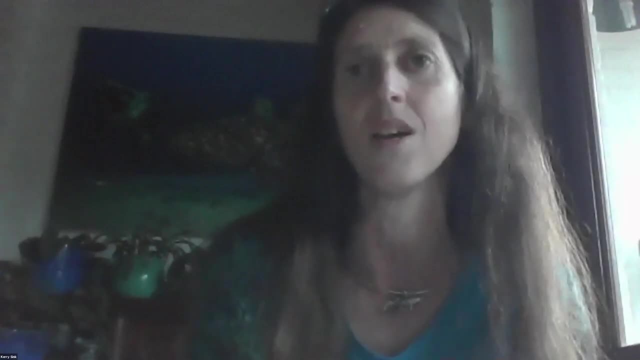 analogy of an ocean crossing. it's not a harbor race. it's really a long game. so you need to to work at it for a long time and you need to slow down and prepare for that. you need to understand more deeply and and then you need to be willing to compromise. it is a compromise. you know i didn't get everything. 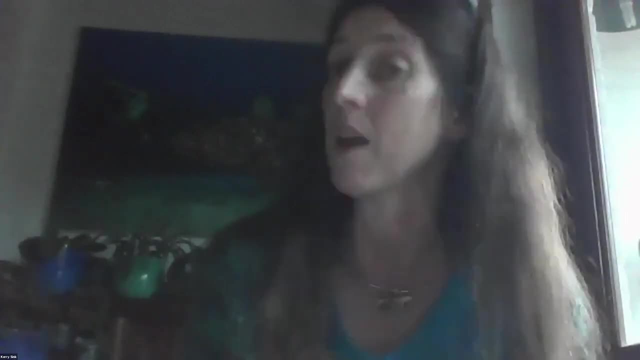 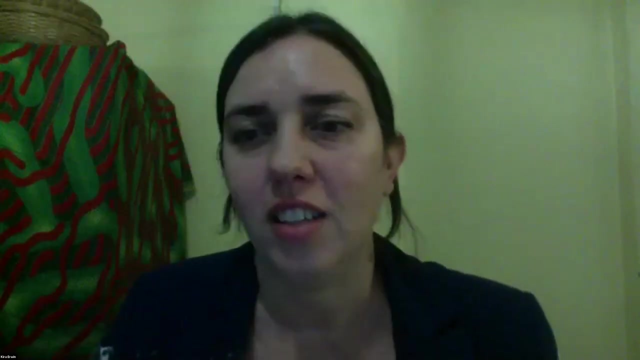 that i set out to to get um and we had to make many balanced compromises and then and then working with principles in that balancing act was was really important. thanks so much, kerry, and i see holly has also picked up on the point of the eia's talking about. 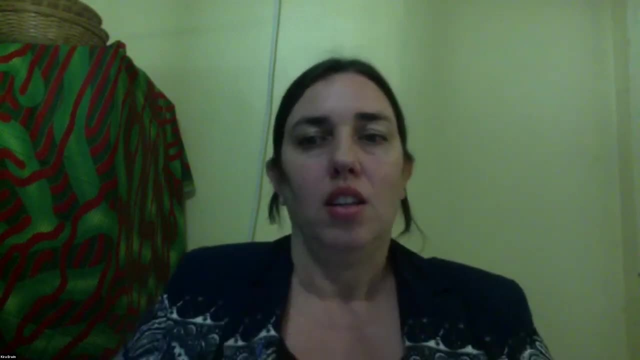 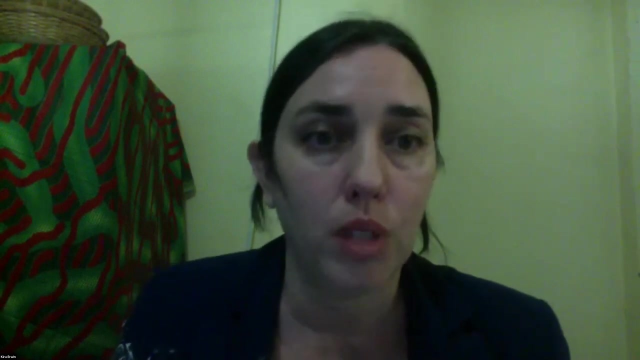 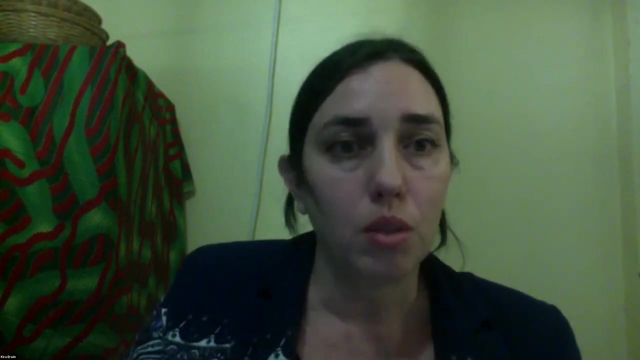 how do we move towards more innovative methods that have holistic and realistic representations of ocean values and impacts? so again, sean's question about how do we start to to value other ways of experiencing and having relationships with the ocean um dylan has also put in the chat. if you would like a link to the eia's website and i'll put the link in the chat box as well. so if you would like a link to the eia's website and i'll put the link in the chat box as well. so if you would like a link to the eia's website and i'll put the link in the chat box as well. 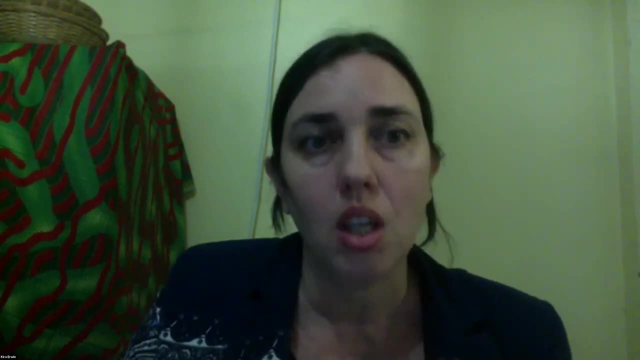 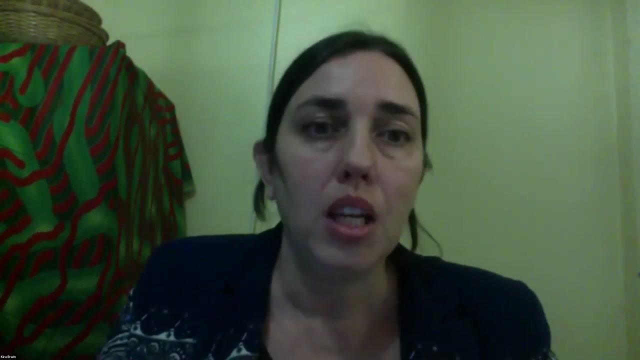 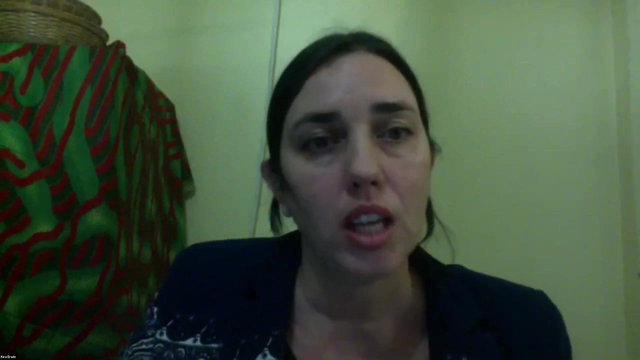 one of the projects in south africa that the one ocean hub has been working on that used a form of theater as storytelling, collecting stories of coastal people and the meanings that they attach to the oceans, and from scientists, from sangomas, from marine educators and to fishers as well. so if you're interested, you're welcome to have a look. 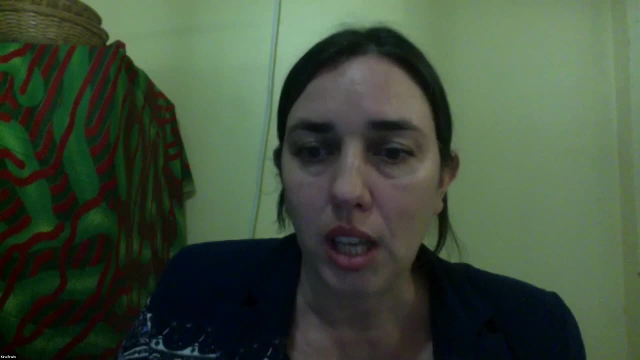 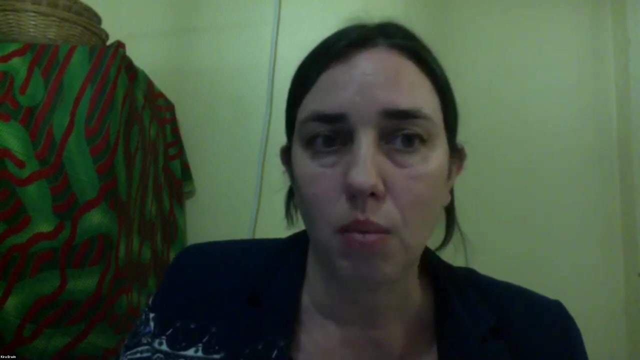 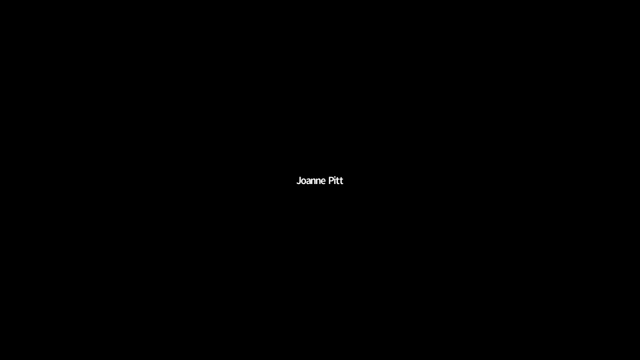 um, joe, i wonder if i could just call attention. in the chat there's also one of the fellow who's trying to get in but can't connect. i don't know if you can see them waiting in the waiting room. thanks, kira. um, there isn't anybody showing in the waiting room just now. okay, i just admitted. 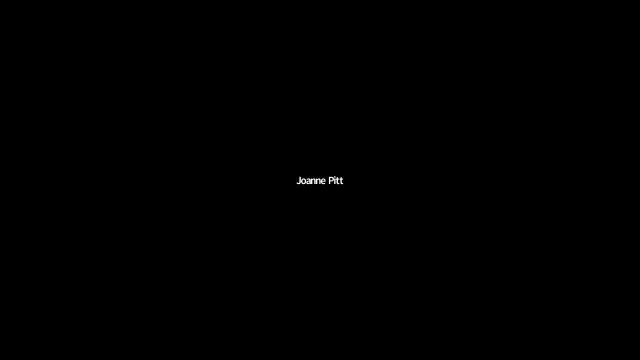 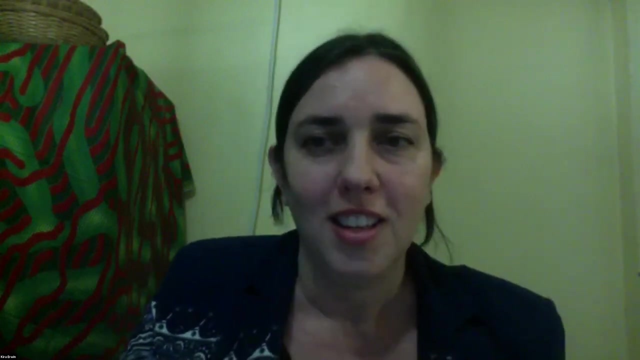 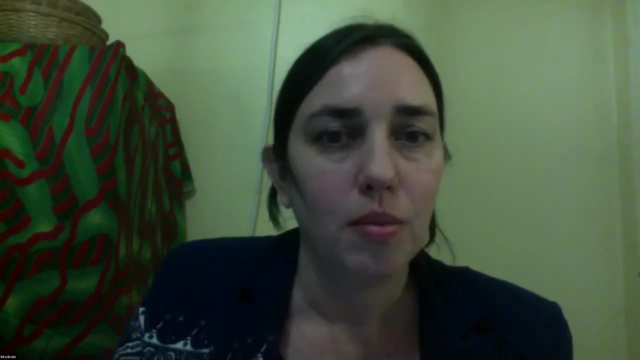 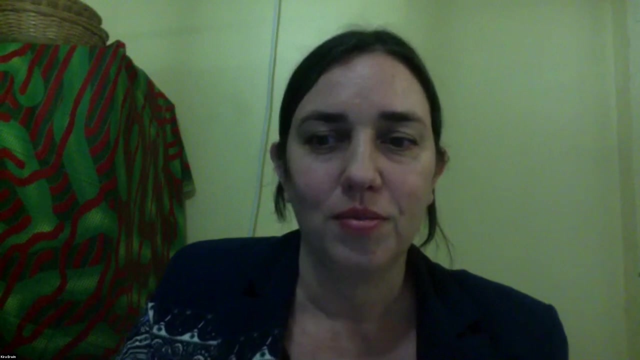 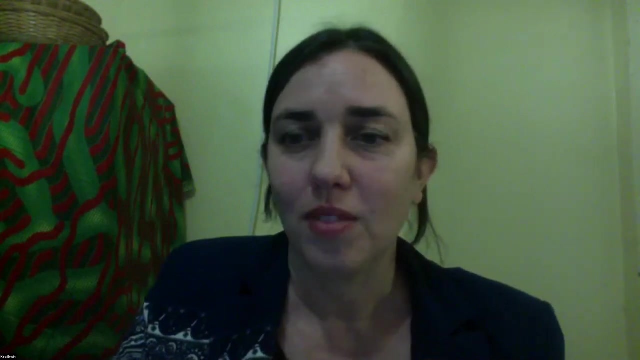 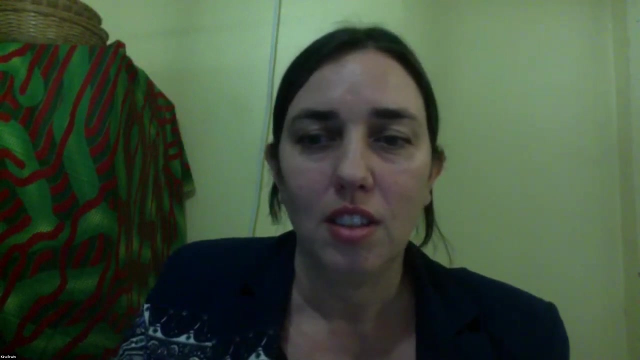 somebody, maybe two or three minutes ago. okay, no problem, thanks, maybe. uh, maybe they'll try again in a bit. any other questions or comments somewhere? or perhaps there's also something you'd like to share from your own experiences that you think would enrich the discussion? nothing yet. 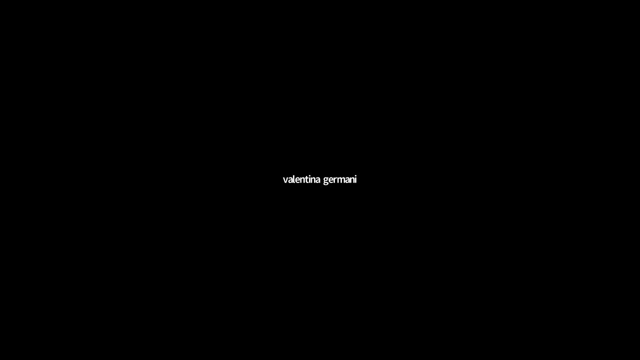 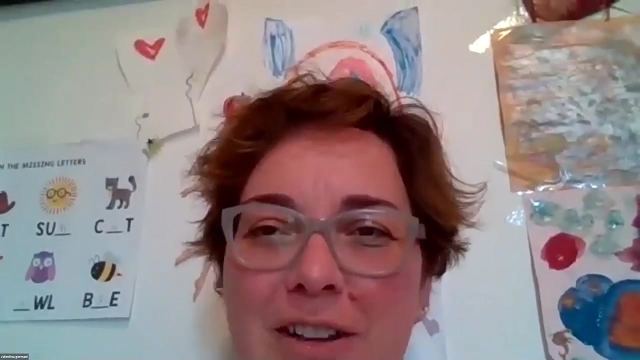 yeah, this is valentina and i apologize because i haven't been able to identify how to raise my hand. see the technological barriers that we have to face and, if it, if it's uh, uh, apologies for butting in like this. um, and let me put my video on. um. see, i'm surrounded by my? um. children's art. 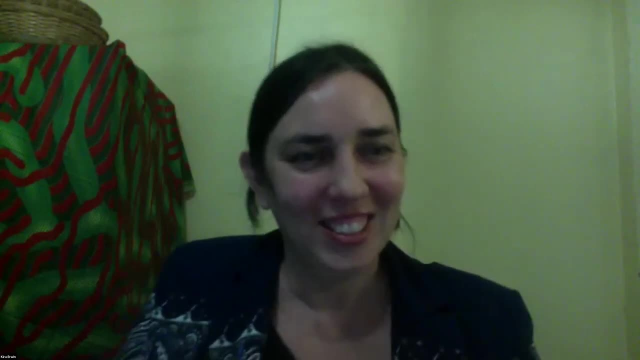 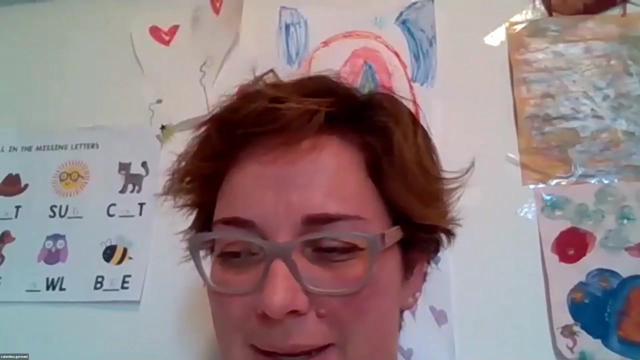 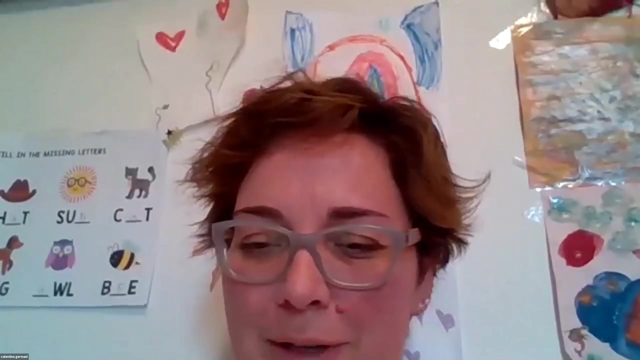 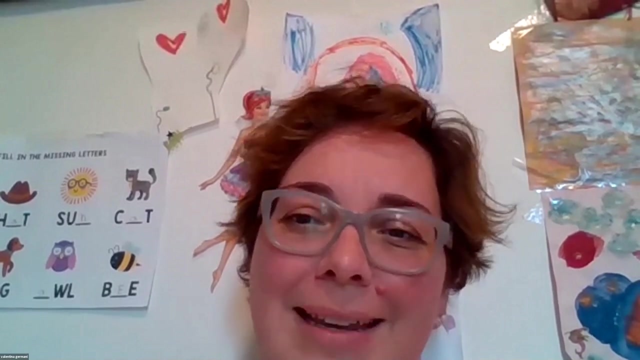 here. that's wonderful. um, here, and this is valentina, i work for the division for ocean affairs and law of the sea and, uh, i am the project manager the un nippon foundation fellowship programs and the alumni network. um, so maybe, while other people might think about some of their additional questions, i i'll take 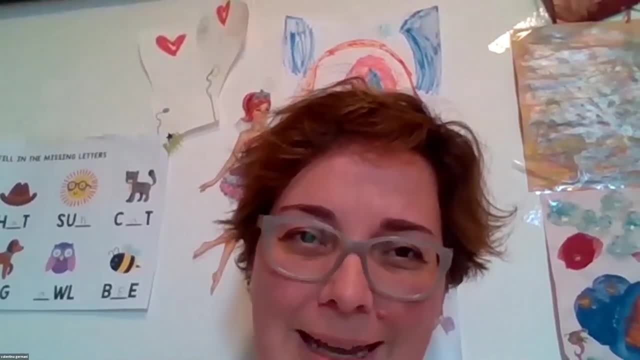 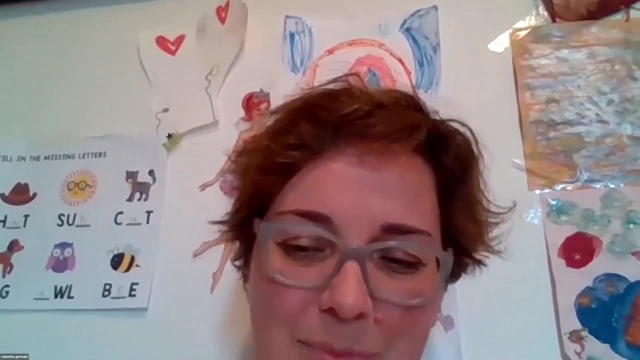 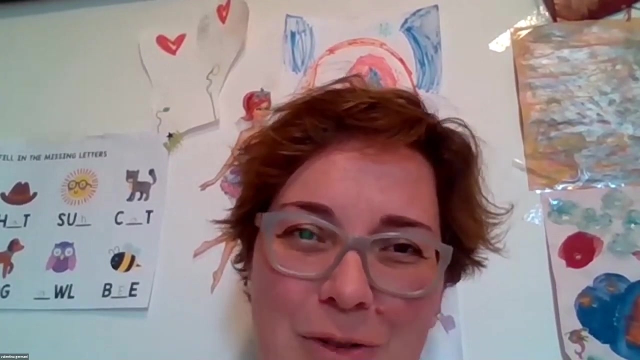 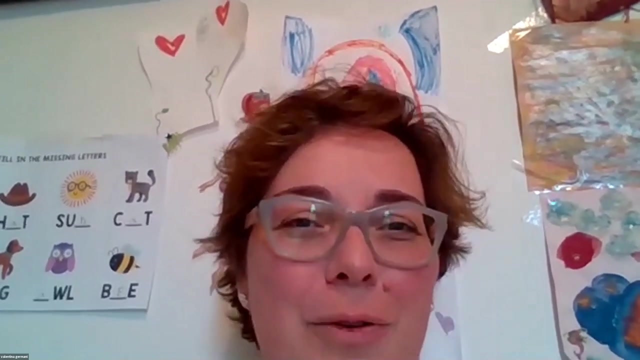 advantage of this pause to first of all thank elisa and one ocean hub and all the vast number of collaborators that they have across the world, and today's presenters in particular, for sharing this wonderful set of images and stories and expertise with us. and we are here, or i am here, in new york in a lockdown for about 10 weeks. 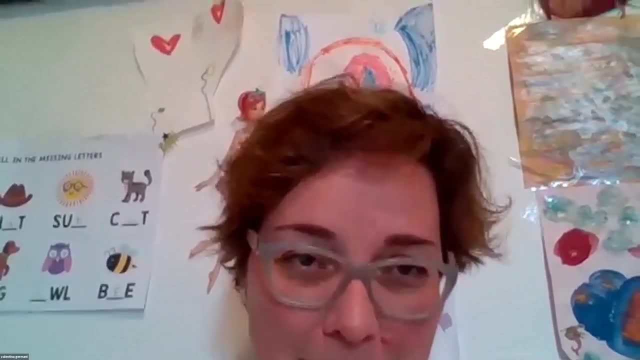 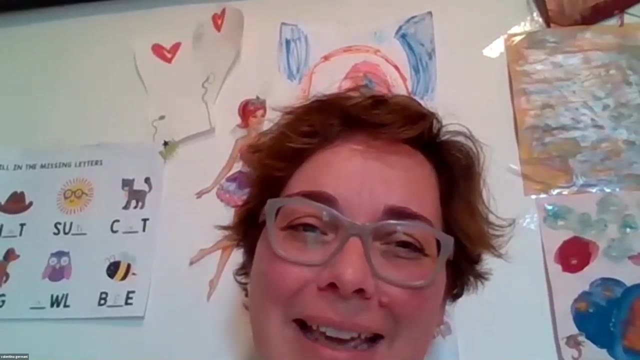 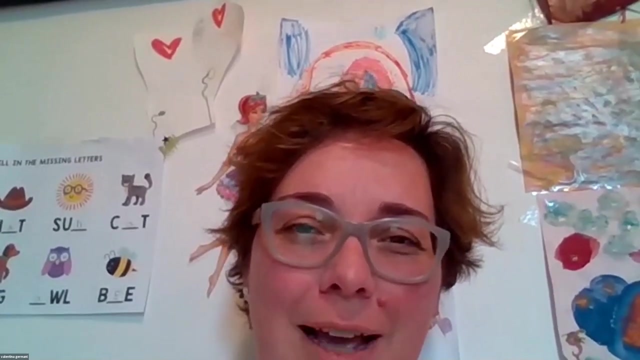 and seeing you know, locked in a small new york apartment surrounded by my children's art. that's why it's not really the usual office environment and i want to really thank carrie for bringing us back to the ocean and allowing us after such a long time, right now, exactly locked. 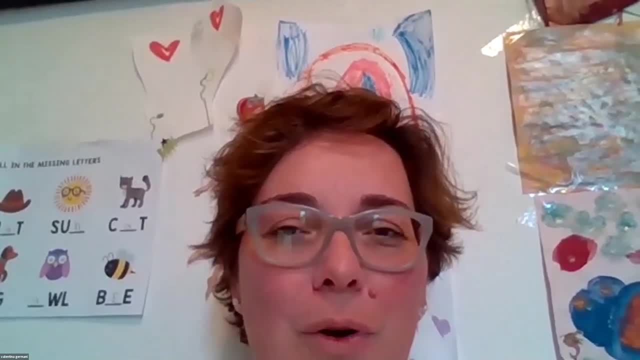 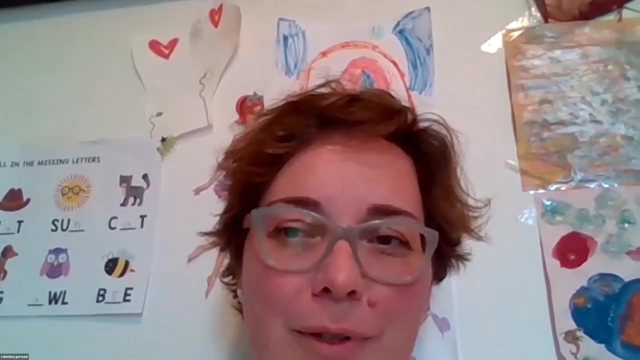 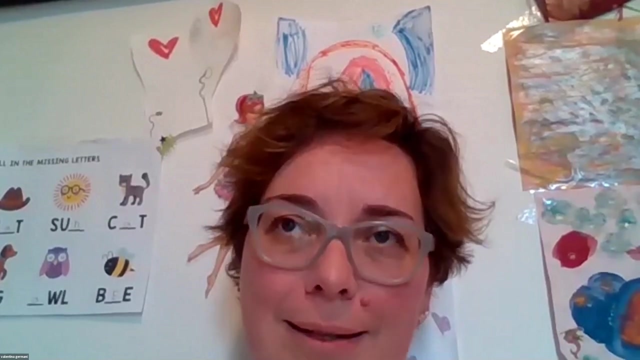 up in these uh small spaces to go with our imagination to the uh, to the ocean. so, first of all, that very uh personal thing and and then again, thank you to elisa and uh and the hub for uh organizing these activities for our alumni. i know that also many of them are in similar uh long-term. 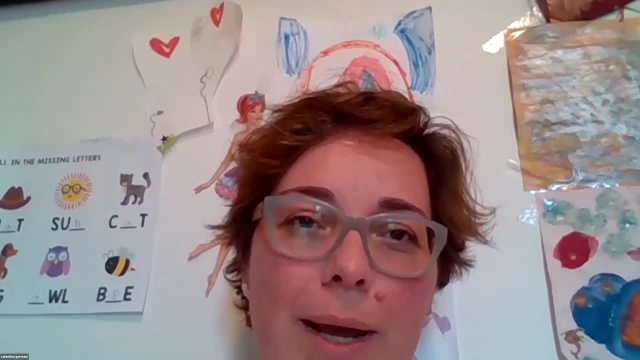 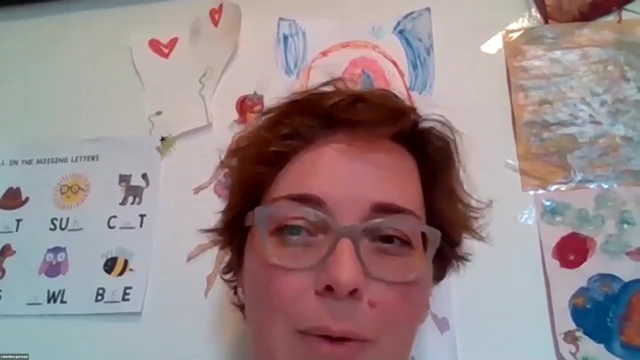 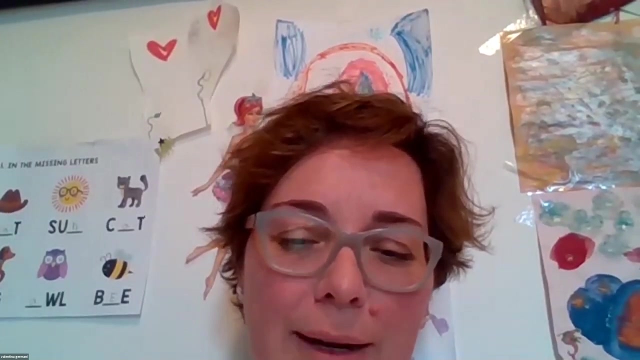 lockdowns, and we have tried to imagine ways to continue our activities with them and continue to build their awareness and our awareness and their capacity. so, um, exactly just a moment to say thank you to all of you and for sharing uh these um innovative ways of thinking of science and uh. 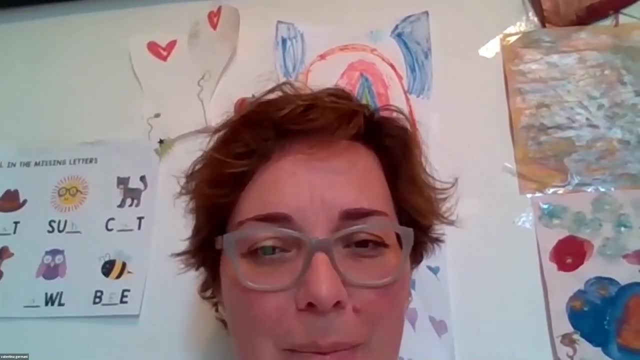 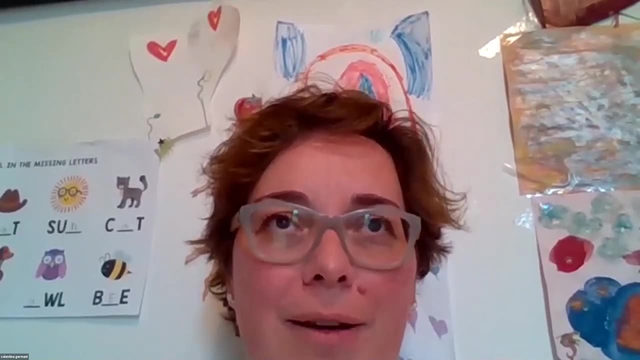 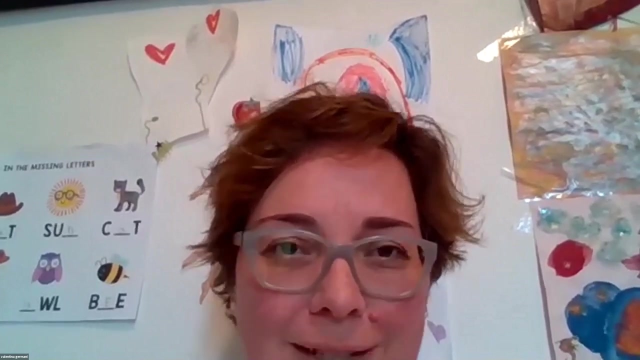 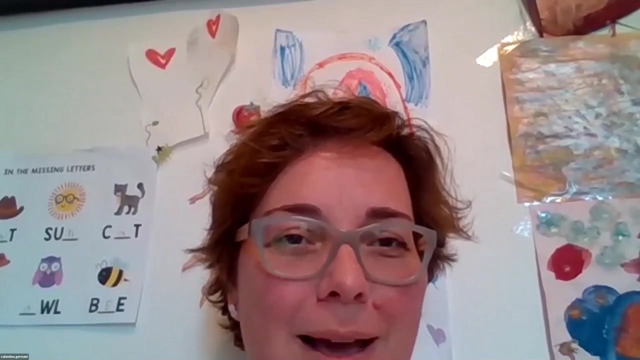 science policy interface. we talk a lot about that in our program and at the un in general, as you can imagine these days, and but it's very interesting to start thinking about additional components, that is, that are not just the natural, physical sciences and policy, but also the human sciences and as humans, we are, or we believe we are, at the center of. 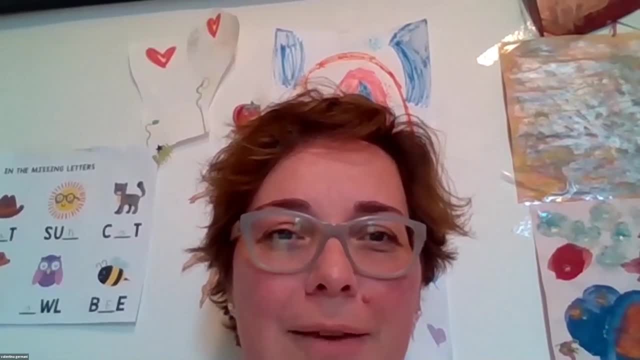 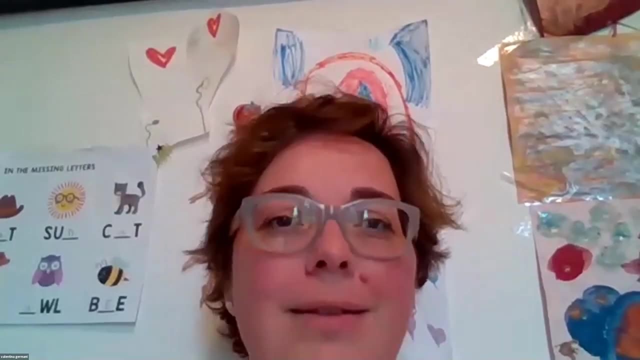 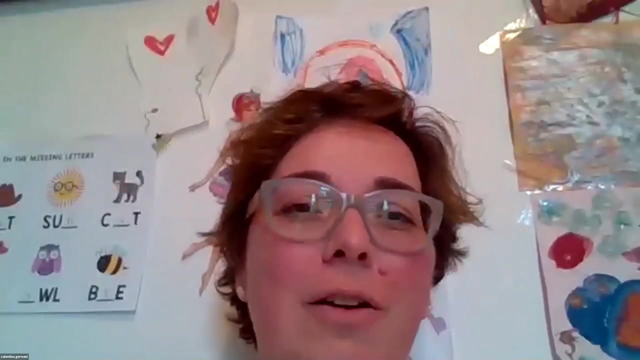 anything and everything, and yet it appears that we never really factor in all these more cultural and spiritual and personal experiences that come from our relationship to the ocean and many other things. so thank you very much for bringing all of us to the, to the forefront. so there wasn't a question there, but a lot of thanks. 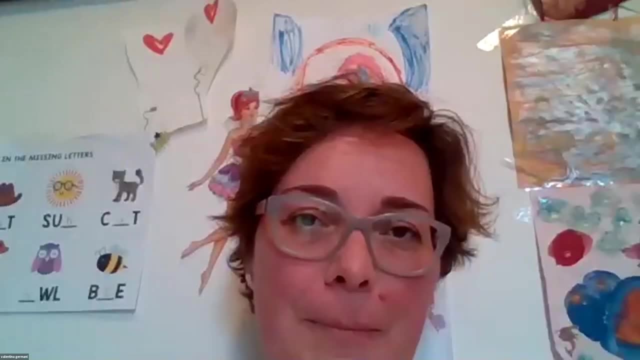 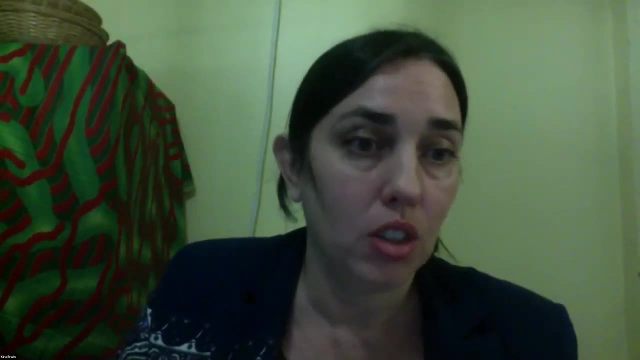 thank you and tina, thank you. that's really lovely to hear. um, yeah, i i have nothing more to add to that except that for me, this has been an incredible journey of research, looking exactly the kind of things you're talking about. um, what are our relationships to the sea? 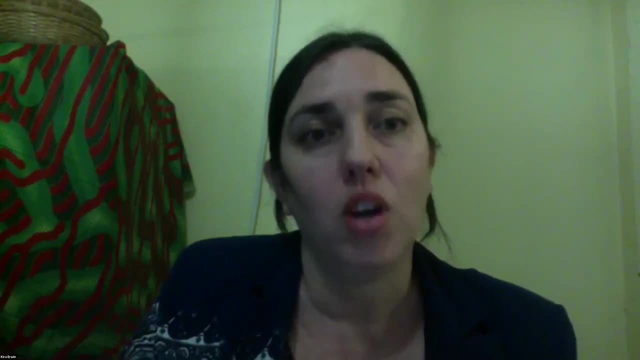 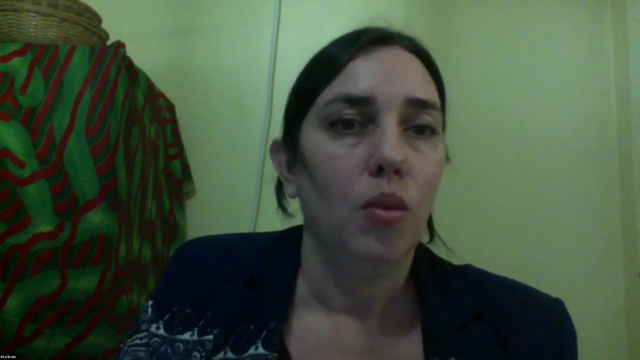 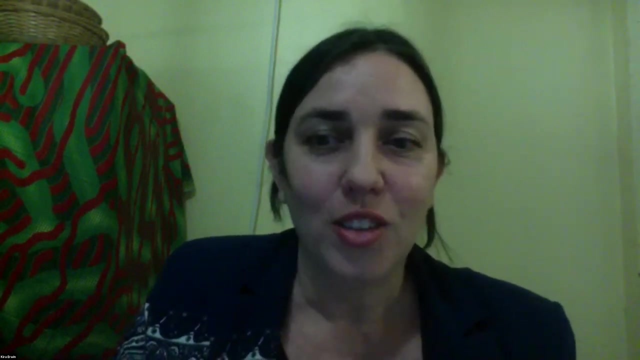 and in fact, in our research project, the question that we asked all participants- it didn't matter who they were, one was actually an ex-minister as well- was: what are your earliest memories of the sea? what are your first memories of the ocean? and it's just incredible how so many people have very moving, uh, memories that kind of have shaped their 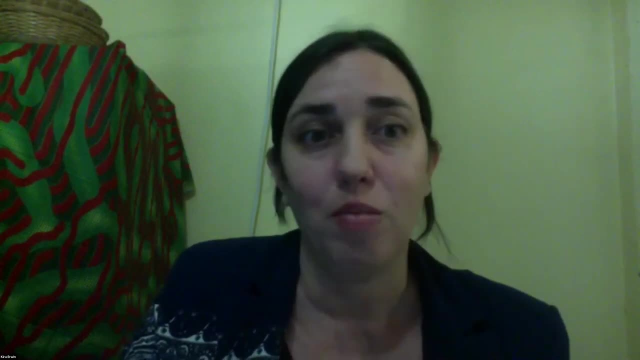 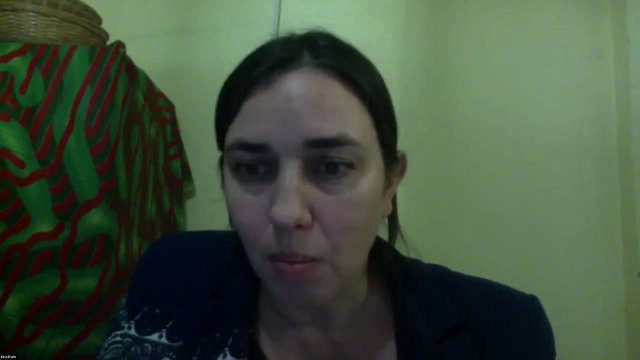 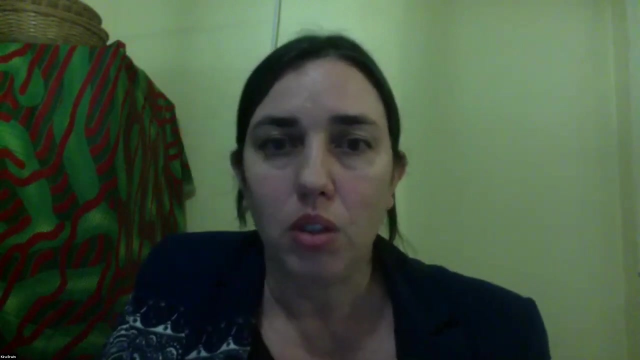 experience and their awe and wonder of the oceans as they've moved into adulthood and all sorts of different fields. i want to just call attention because we have got some more questions in the chat. let me just go back to that and here i think what we could do maybe is, uh, sean dylan, kerry and alisa. 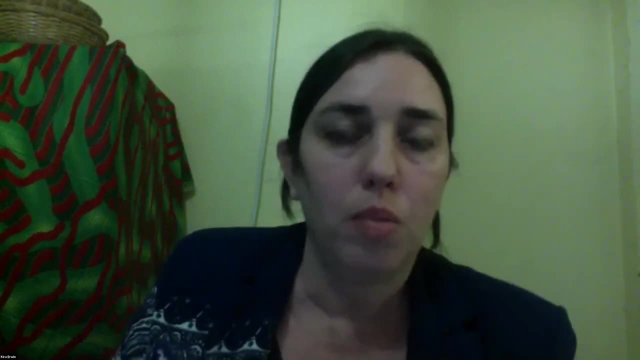 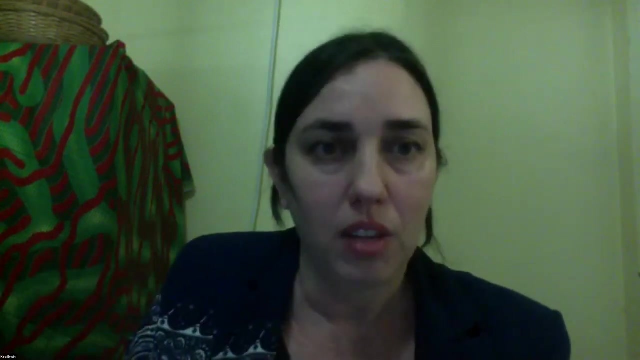 if, very briefly, you'd like to answer this, but it's from andrea, again from brazil, asking and, and he's right, this is the sort of communication challenge that we have here. so what kind of tool have worked really well in your experience? when have you felt like you've, you've got through and 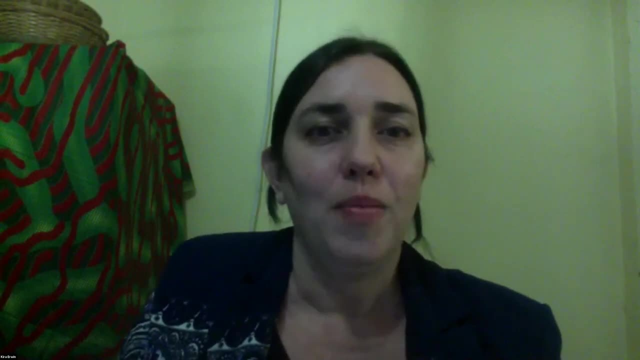 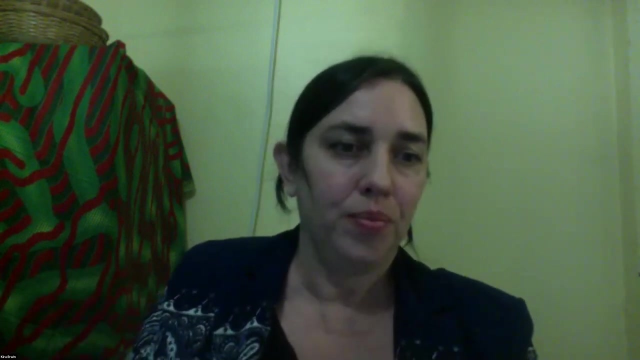 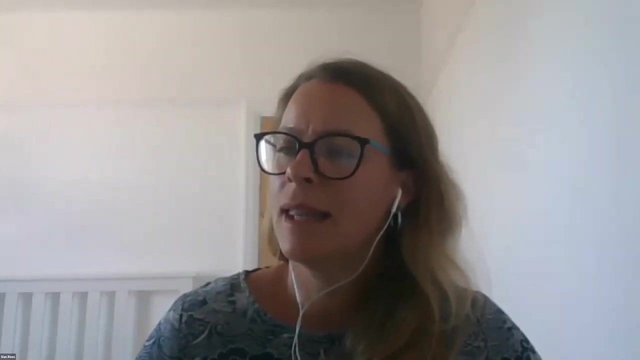 kerry, to some extent, have really said storytelling, um. so maybe sean would you like to talk from your experience, and then dylan and then kerry. so the question is about what tools, what tools in our experience, really work, um, i think, for for me as a, as a social scientist, um economist, what 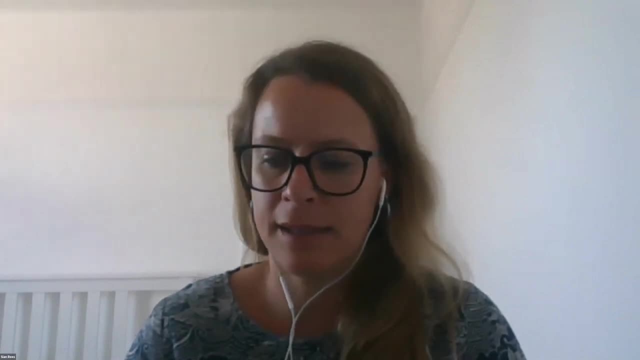 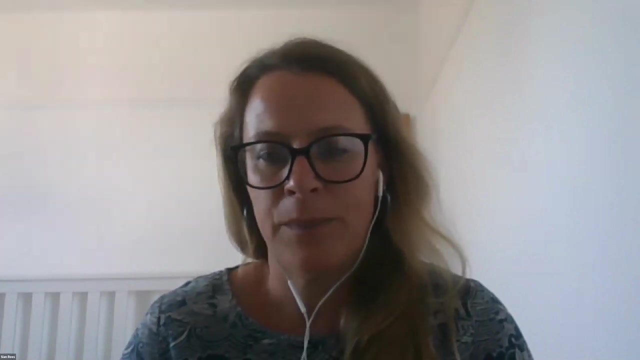 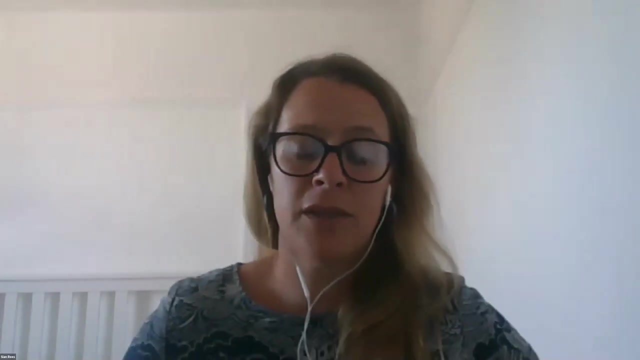 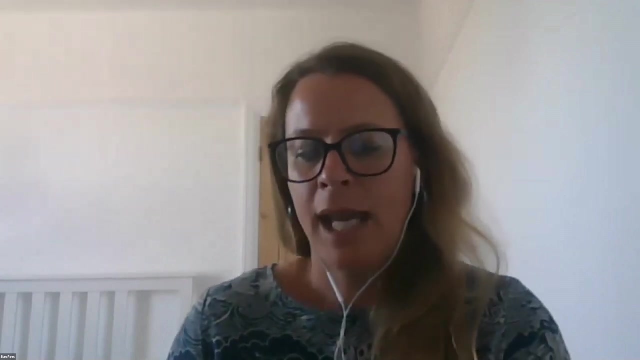 really works is acknowledging that livelihood values and economic values are linked to to ocean systems, and to try and find ways to develop things such as a fishing industry. i'll give an example. we have a small scale fishery in the uk and an area was closed to scallop dredges in order to allow 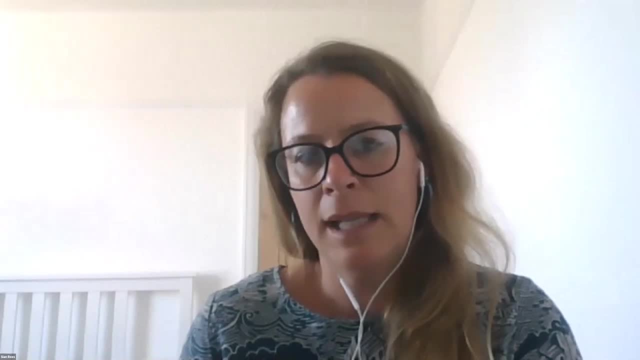 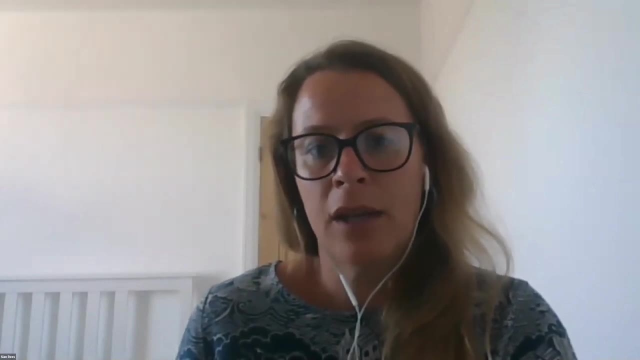 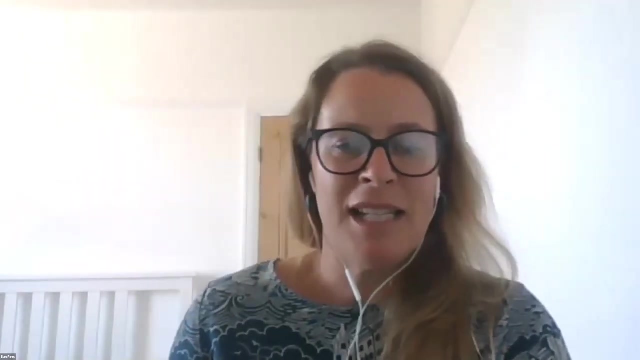 the shell fisheries to benefit from that and it was a huge legal challenge to get the area closed. but that was nearly 12 years ago and in the 12 years since that site has been closed, people who are mortal enemies in the initial stages of the closure have now formed this most wonderful fisher. 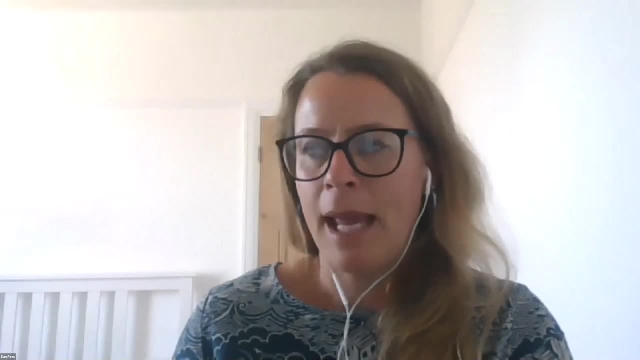 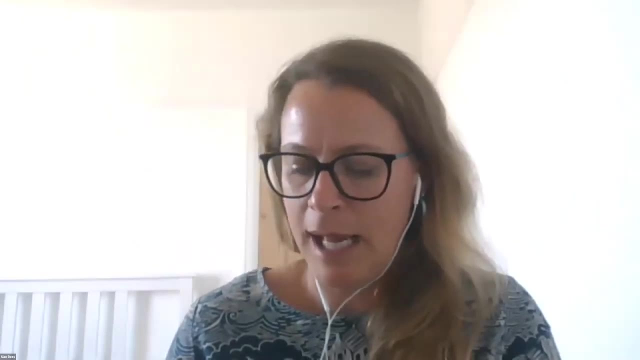 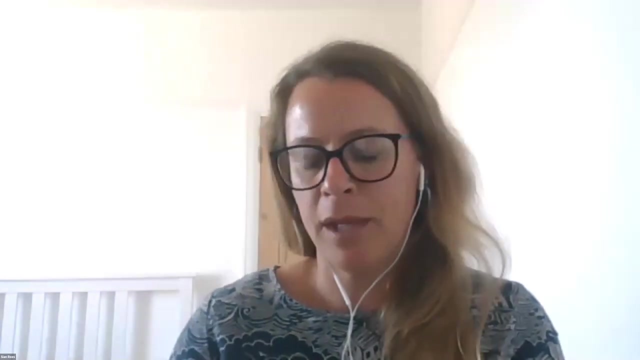 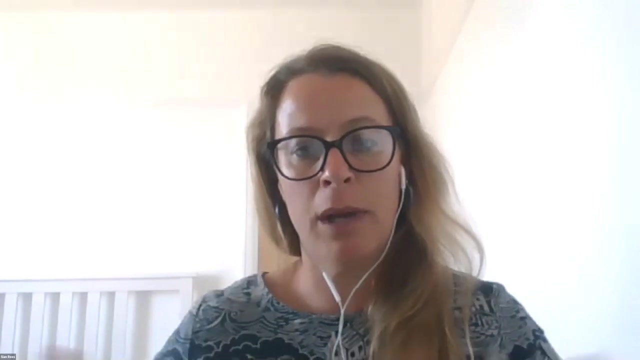 science partnership, which is based around economics, ecology and social sciences. so we ask the question: how are people's well-being influenced, how are people's pockets influenced and how has the environment changed? and through that constant feedback and using the local boats as research vessels as well, we just create this partnership of shared understanding, and it can't just be the 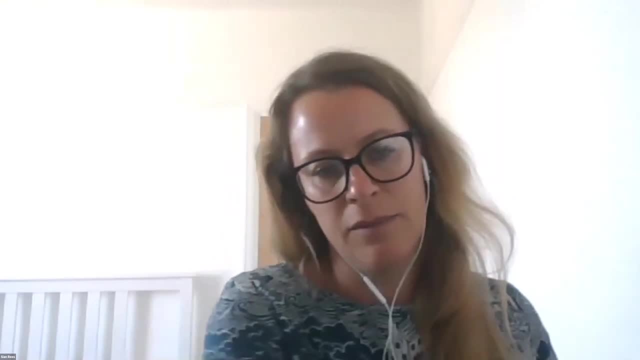 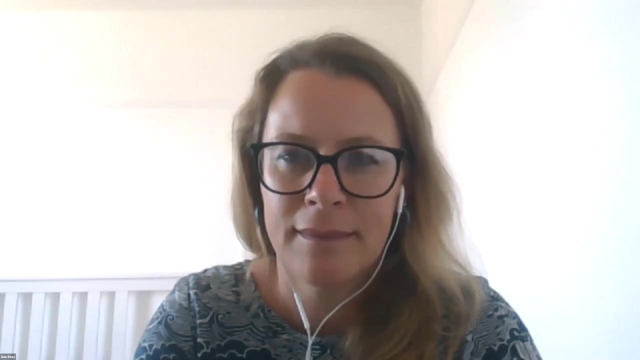 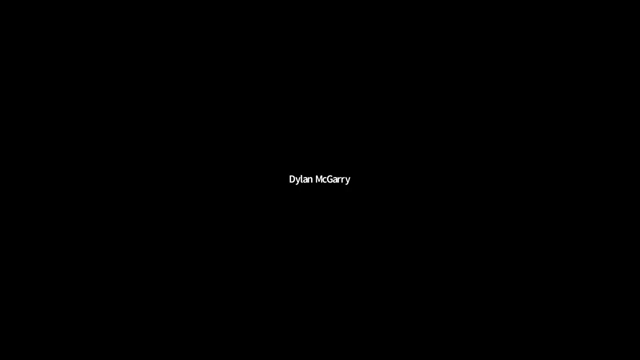 ecology. it has to be the understanding of how that influences change within a community as well. thank you, thanks, sean dylan um. thanks, i mentioned it earlier, but, andrea, the biggest tool i think that we could work with is empathy. i think it's a very powerful um if we see it as a tool in building relationships. 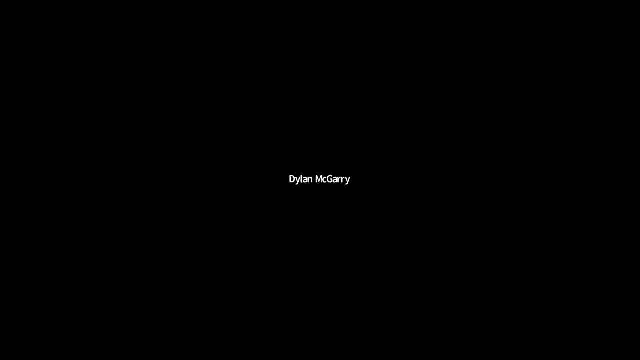 and also friendships. i've noticed that, you know, when we use we? i mainly work in theater, but when we use theater to tell a story about what's actually going on, we get the story at one story, without judgements. they go deep into. the immersive story is that? 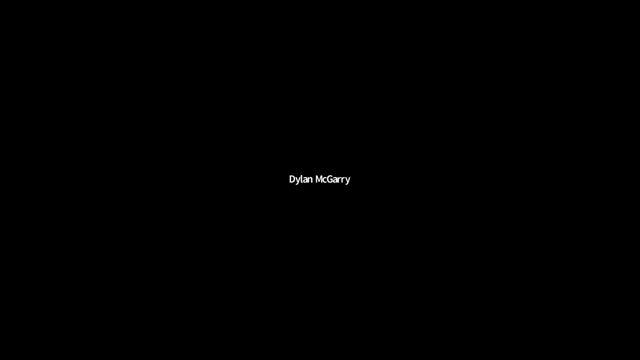 it renders you defenseless. you you can jump into your agenda easily if you're trying to just talk hard facts, but when you talk about the emotional connection to the ocean and long-lived livelihoods and stories and meanings of the ocean, it's much harder to defend certain ways of thinking or being. 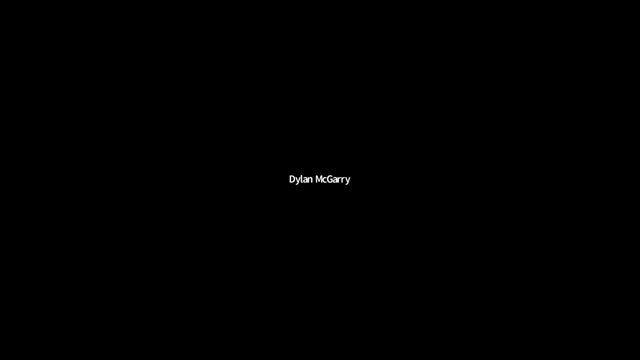 so i found empathy and any practice that can encourage empathy, any tool that can do that, which is usually the arts um, is a very powerful. i've been very powerful in some of our other projects. we've been able to kind of make meaningful changes in very local, practical ways as well as. 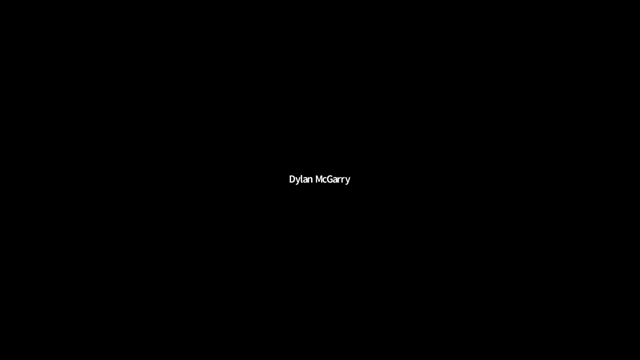 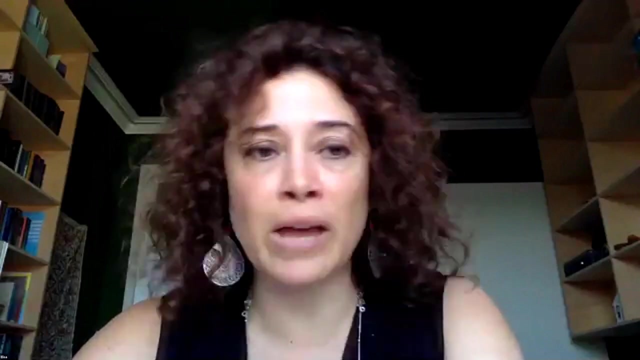 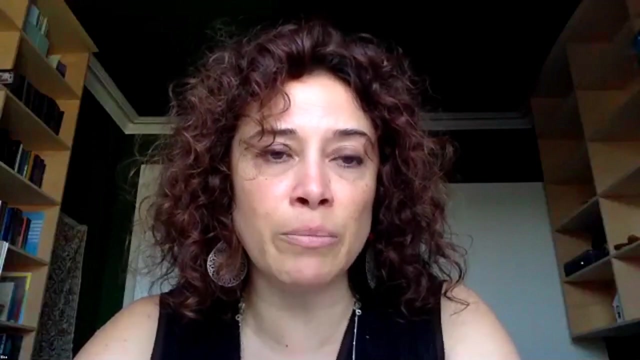 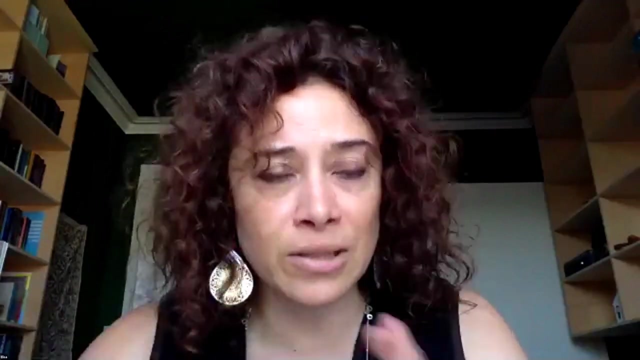 policy, you and, i think, from my end. i think there's also legal tools that we can use to to have stronger communication or potentially more persuasive communication. and going back to the point i was making earlier about different areas of international law that we can bring together in addressing ocean challenges, as well as the, the complex balancing act in understanding, 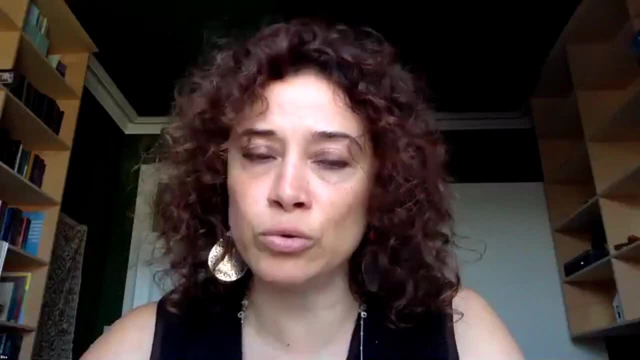 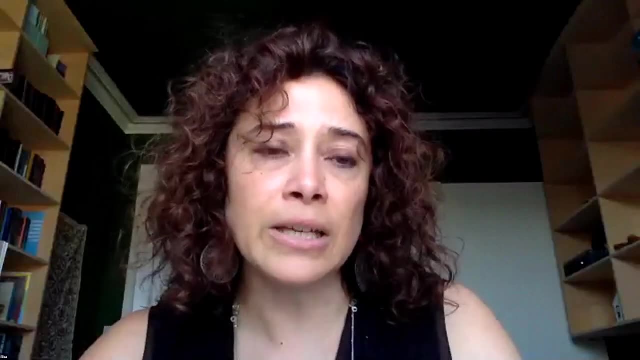 opportunities for ocean conservation and sustainable use. i think one key area of international law that we can all engage more and more in is the question of how can we bring together different areas of international law that we can all engage more and more in, and how can we bring it together, and i think the first area is international human rights law. 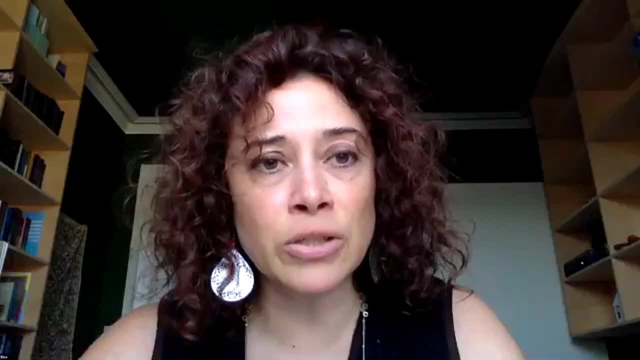 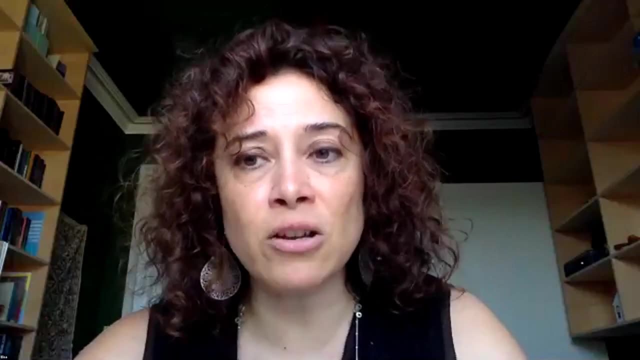 and this is an area where we have recognition of multiple values, including the intangible values, when we have a lot of legal reasoning and tools for balancing. i mean, of course, it's not a silver bullet, but it's also an area where different stakeholders can feel that they are empowered. 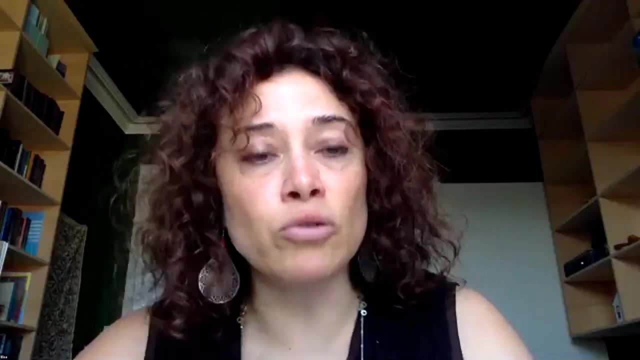 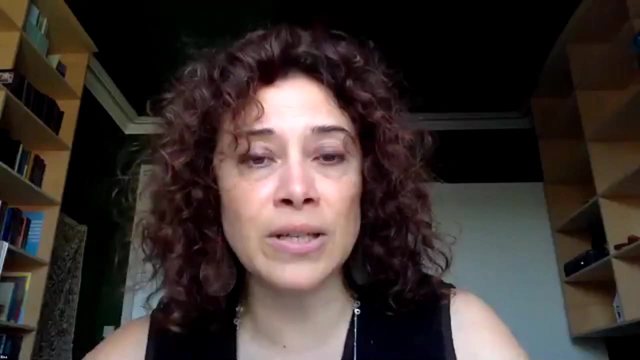 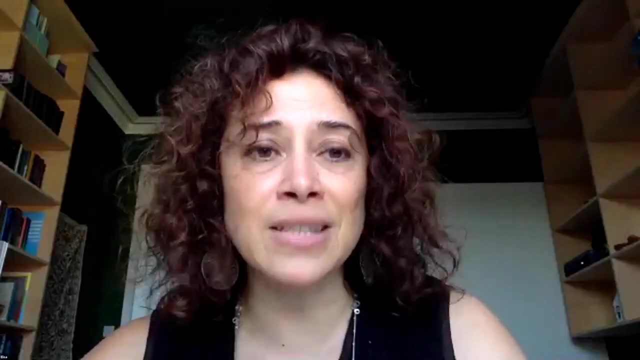 to ask questions or to challenge or or to be heard and where other members of the community, be that you know, judges um, human rights lawyers, etc. human rights advocates and activists, monitoring authorities and others can also understand better their own obligations to listen to different voices and support effective communication. 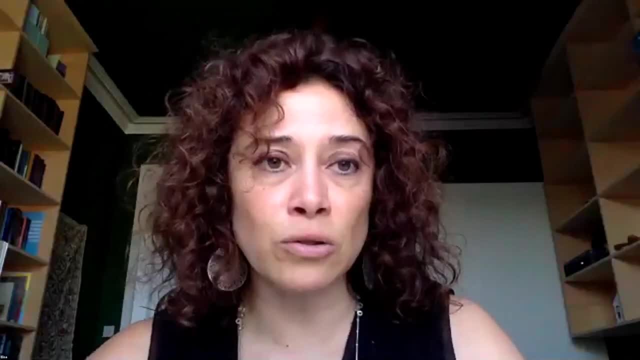 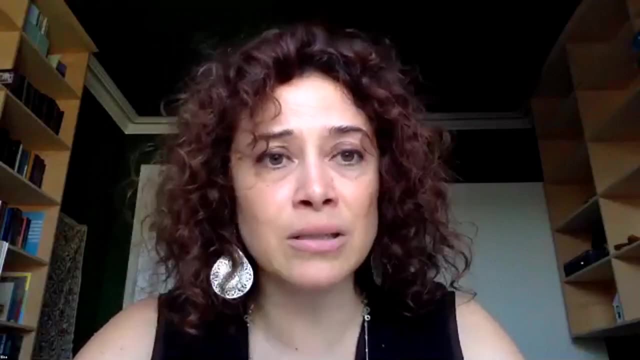 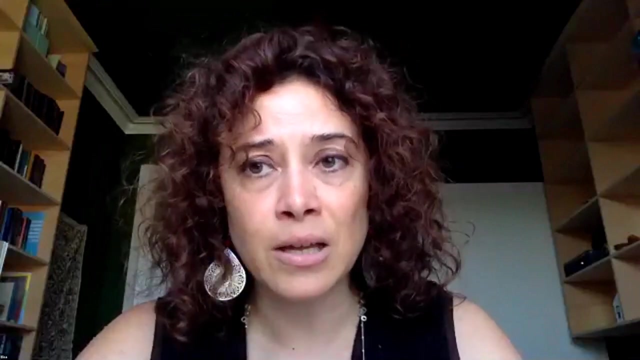 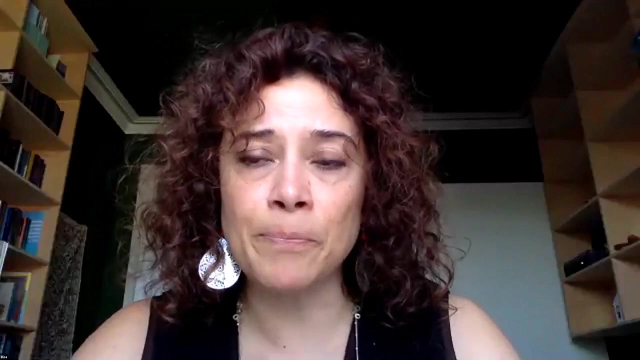 on the different needs and science that we're looking at to take decisions And I saw, Sheku, you had in the chat a few really important reflections about climate change impacts and the approaches to climate mitigation and adaptation and how that may affect negatively particular sectors of ocean constituencies, including communities. 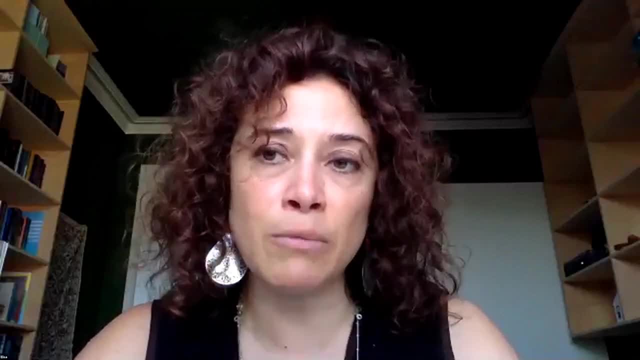 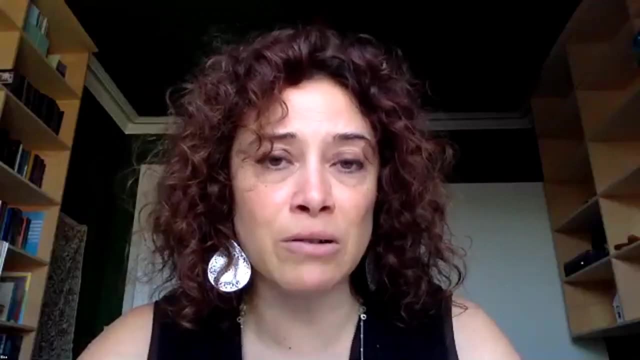 The question of poverty, too, and I think these are all matters that are becoming more and more addressed in human rights terms, in terms of climate justice, poverty, looked in terms of human rights as a way to address these issues, not only as socioeconomic ones, but 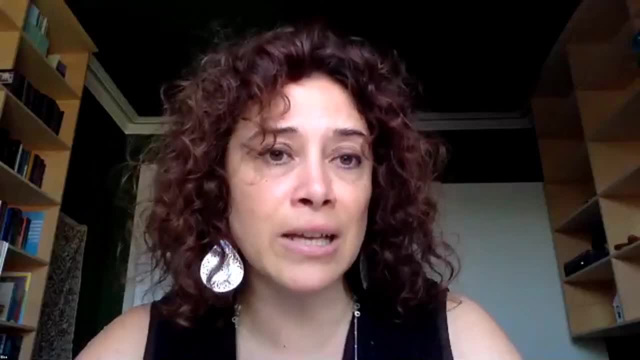 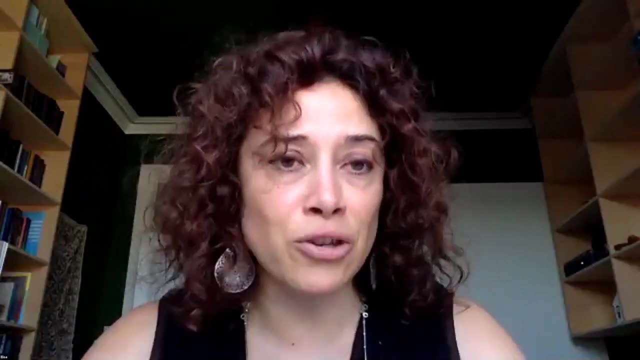 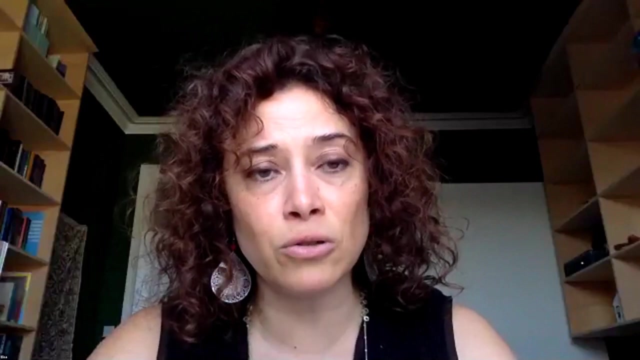 also in legal And, you know, giving a harder legal edge to those issues as governments are balancing with other international and national obligations. So I think there's one thing that we are looking into is to what extent using human rights in those negotiations can help bring a broader group of people to the negotiating table. 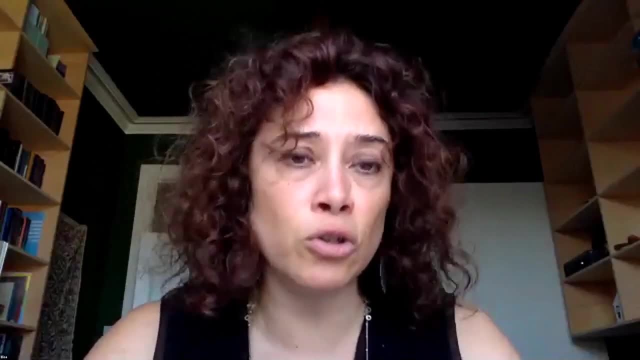 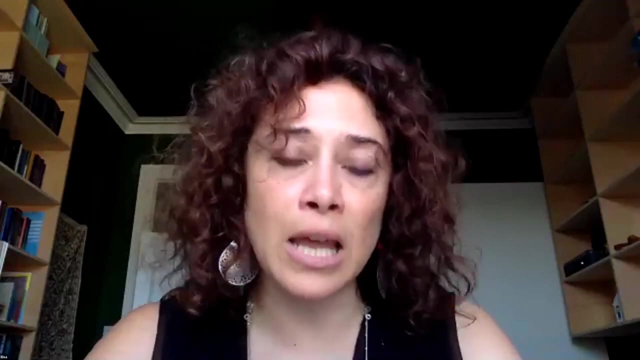 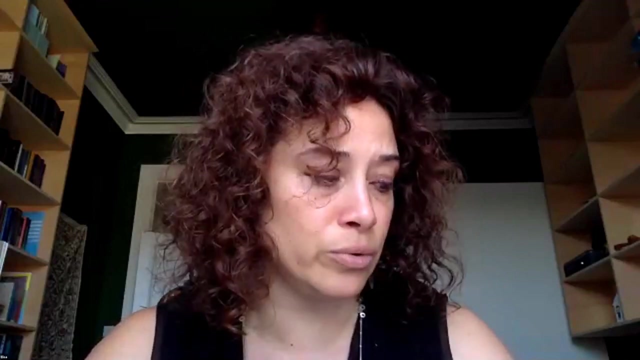 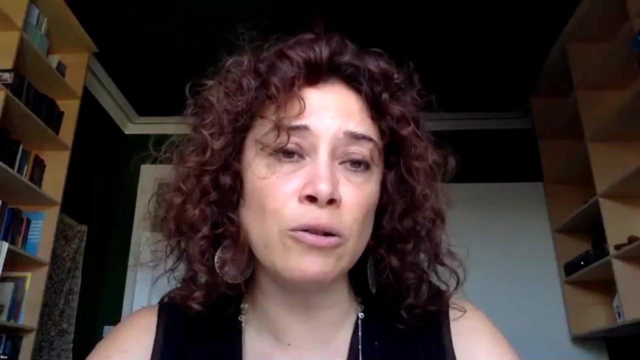 and maybe giving more attention to those voices that are not usually heard as much, And particularly the voices of those that are most vulnerable to climate change impacts and to the negative impacts of our own decisions on ocean conservation and sustainable use. And, in fact, human rights law also has a very strong branch related to the rights of children. 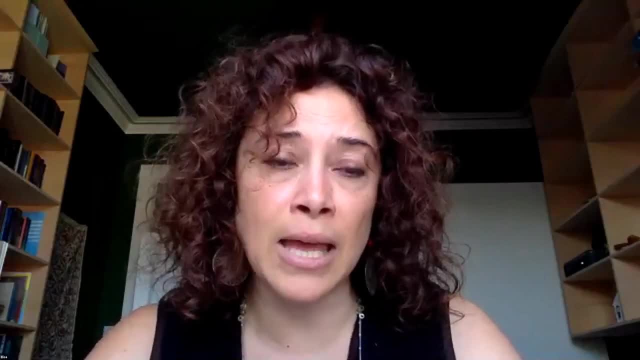 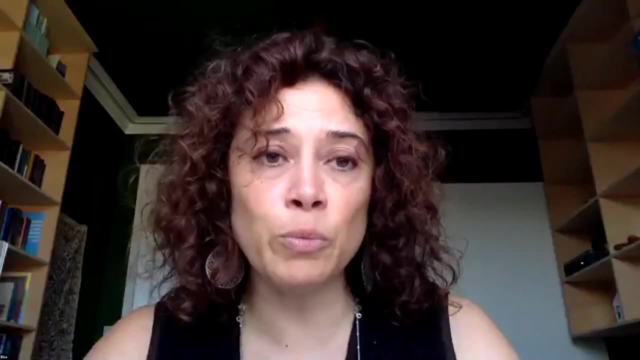 and how children are the most affected by any mistake we make, I think, in environmental management and conservation, and particularly marine. Both because right now, because of climate change, we have a lot of issues that we need to address, But also because of the things that we are going to be doing now because of the early 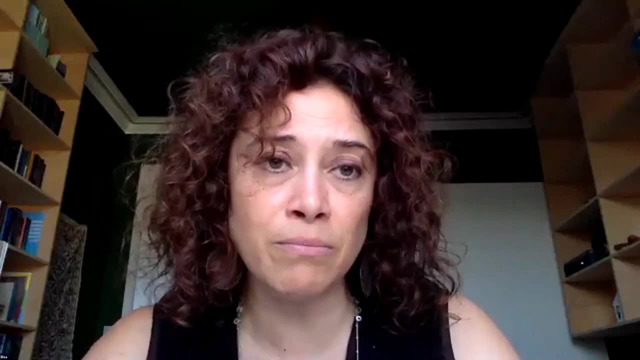 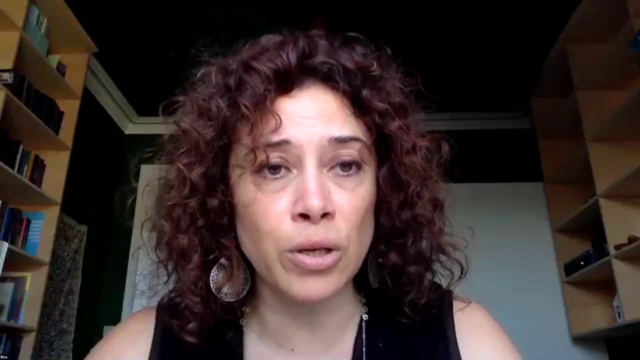 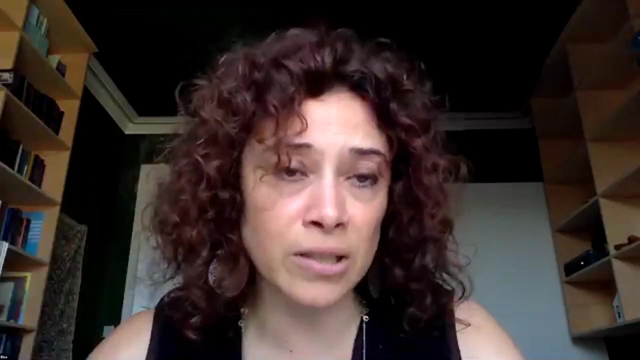 phase of physical and mental development, the impacts are stronger on them. They have less resilience than grownups do, But also because they'll have a longer time in which they will be affected by those negative impacts as their development continues, And their timeframe is 50 years down the line, 70 years down the line, which is actually 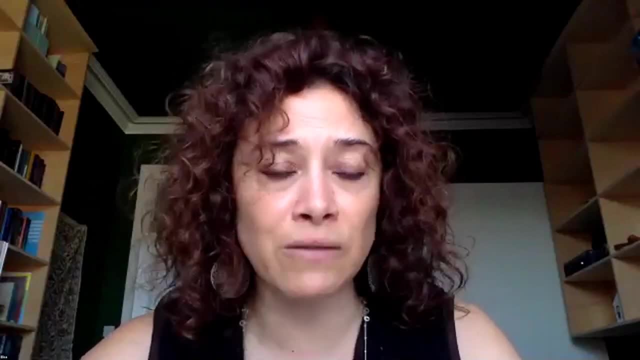 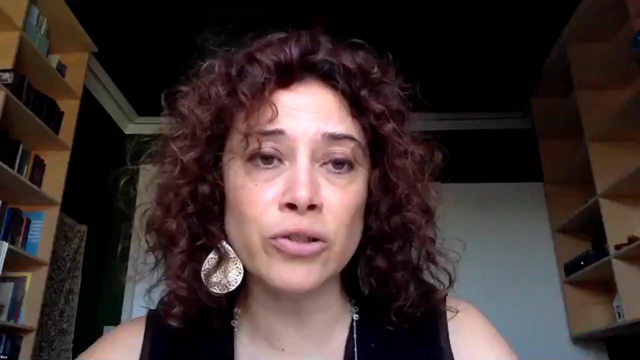 a timeframe that is more aligned with that of nature and biodiversity and ecosystems, And so human rights law really both. It gives children a voice just now, not just as future decision-makers or stakeholders, but right now, governments who are party to the Convention on the Human Rights of the. 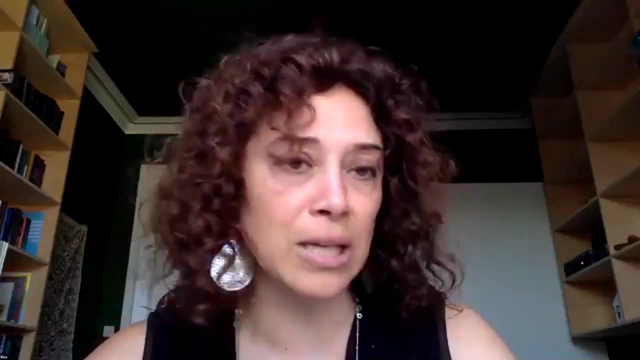 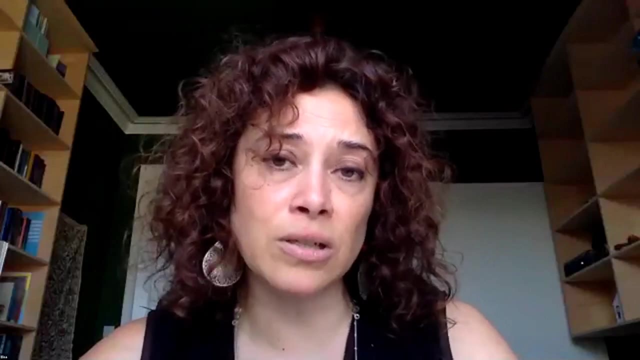 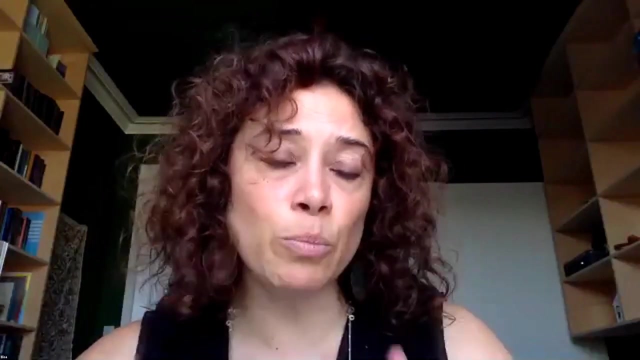 Child are expected to involve children in decision-making, And this can be very powerful voices and very important- but also critically, to make sure that their own concerns and vulnerabilities are taken into account in environmental impact assessments and decision-making. So I think there's an opportunity there for scientists and lawyers. 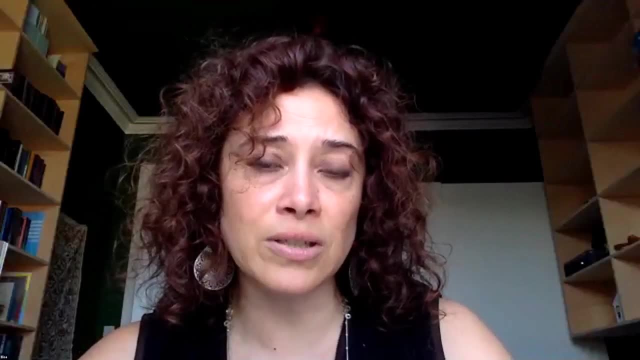 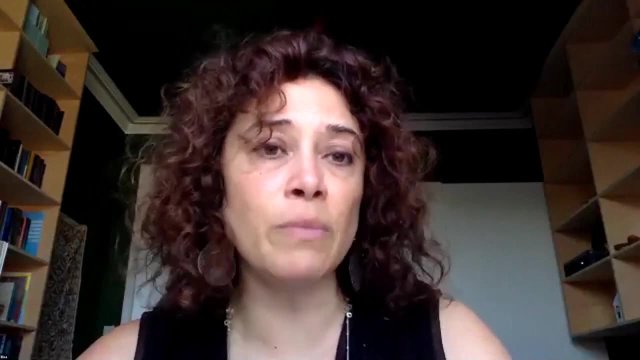 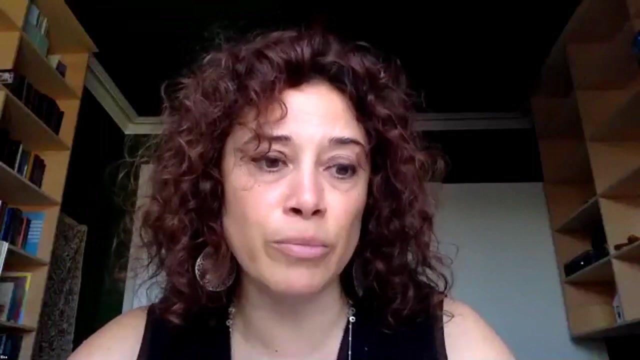 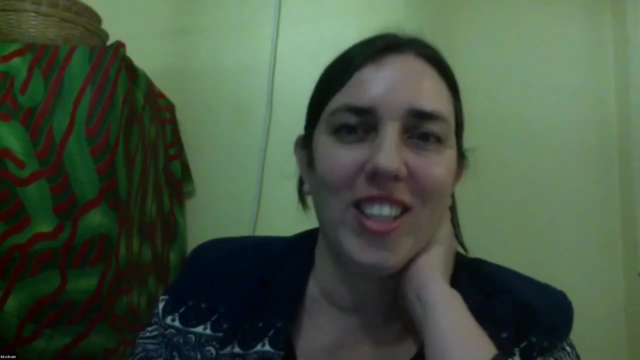 And social scientists who work around ocean conservation and sustainable use, to use for communication purposes, but also for building alliances, human rights, to give those voices the attention they need and for us to learn from them and be better at our own job. Go for it, Kiri. 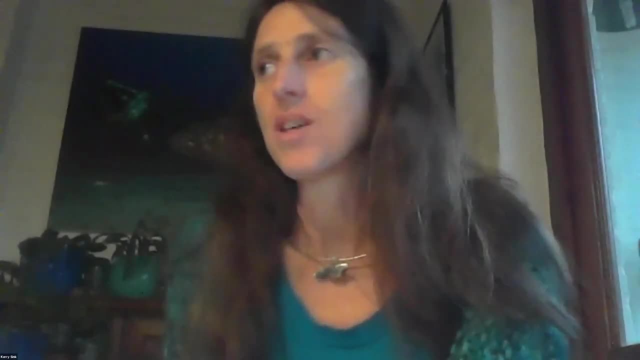 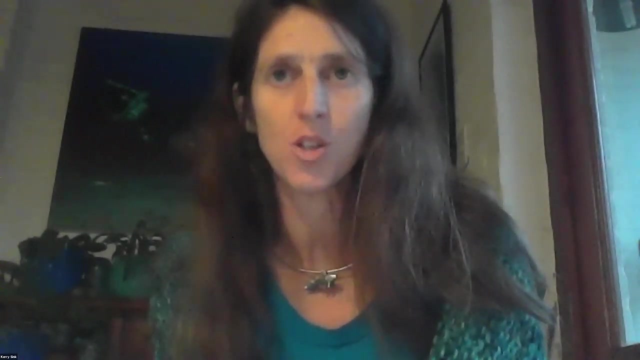 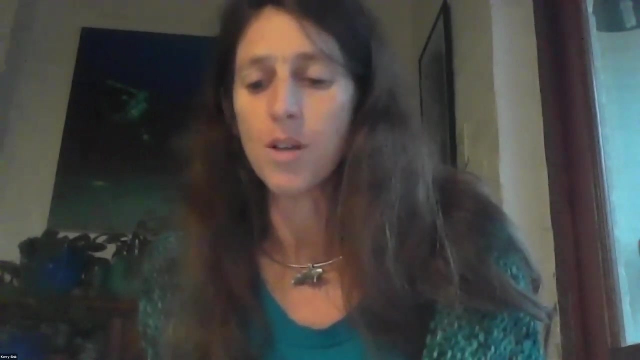 Thanks. I think that's. There's a really important link there to the rights of the child and the decisions that get made in government And in fact one of my most important communication lessons is to bring future generations into the room. So just to reflect on Andrea's question about our communication strategy, I'm trying to 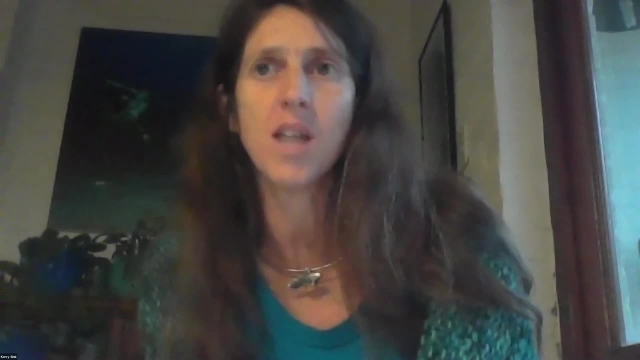 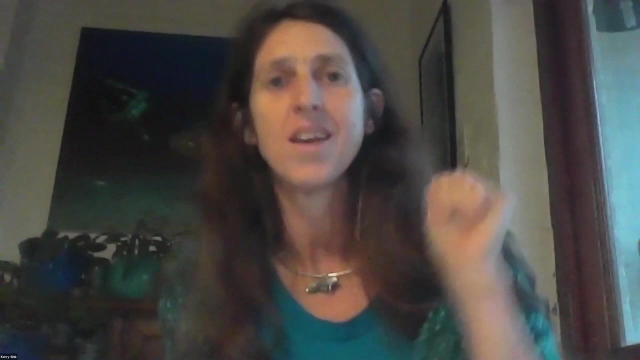 write up my lessons. We invested a lot in understanding the audience, Which was cabinets, South Africa's cabinets- and the factors that had previously influenced decision-making, And one of those that emerged very strongly is the impacts on future generations, And so we put a lot of imagery of children into our websites, into our communication. 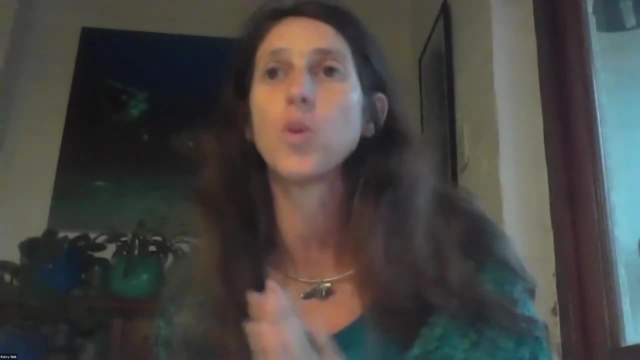 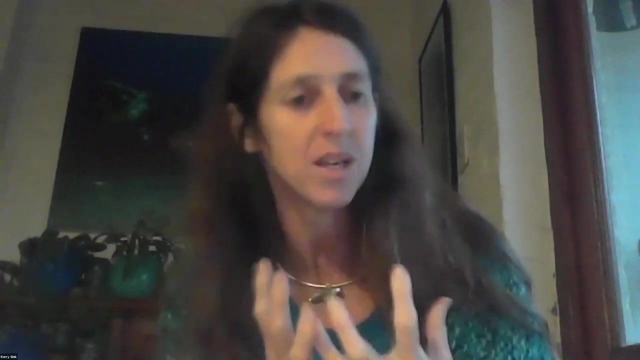 products, into our brochures, that we took into cabinets and into a film And the film. The film had a lot of. The film had a lot of images, It had a lot of emotion in it, It had empathy in it. 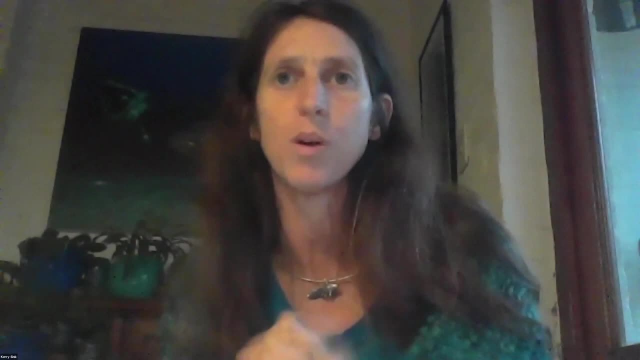 It had national pride in it. So those were all also important elements in that work. But, Jo, like all good communication efforts, you do need to understand your audience in preparing what you're doing, And we studied that to look at our cases. 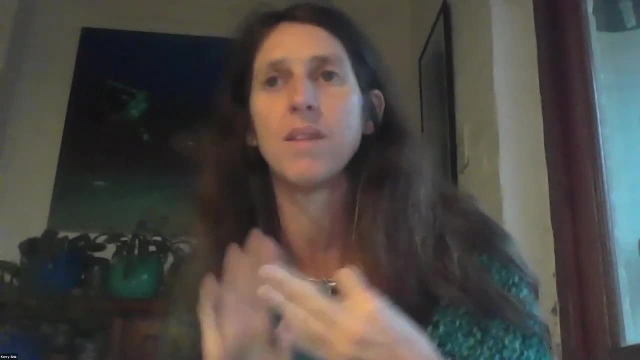 And future generations' economic sense and then framing the work as practical solutions were, And then framing the work as practical solutions were actually key messages that we distilled out through research. Perhaps I can just add to that, because there's a lot of really interesting both statements. 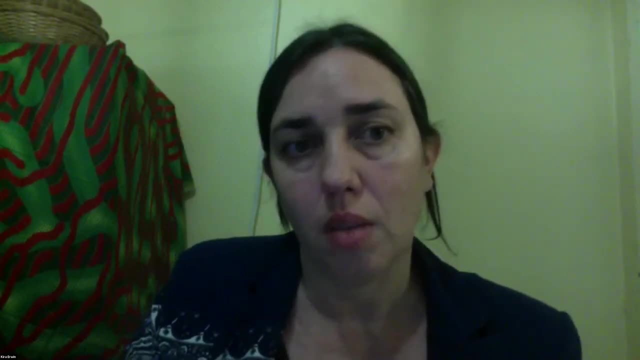 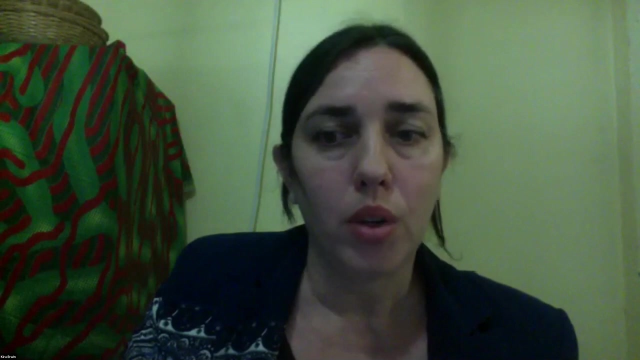 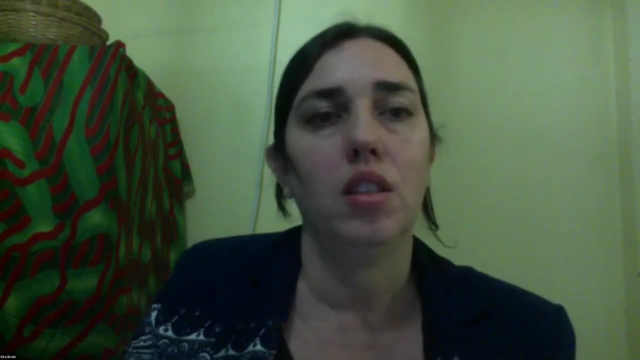 and questions coming up in the chat and we're starting to run out of time, But EIA processes, legal processes, research, scientific papers that are really showing evidence in which change needs to happen. I think one of the most important things that we're trying to do, and I think that's what 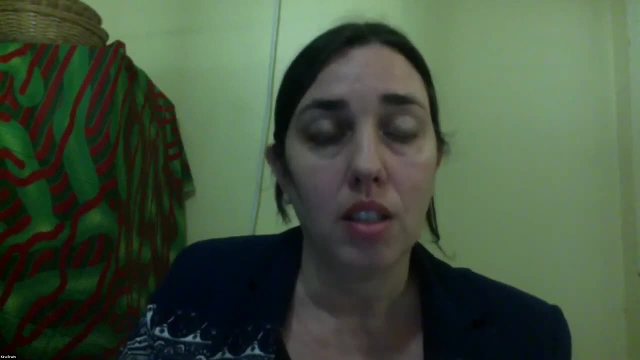 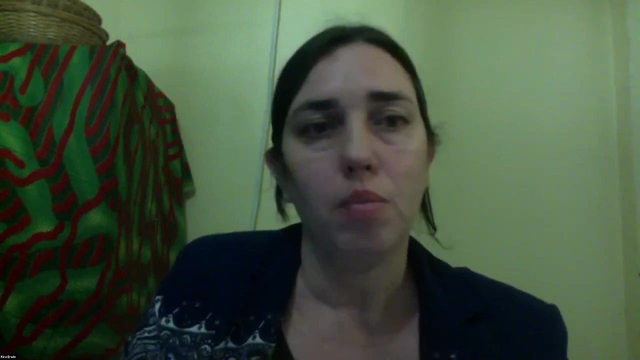 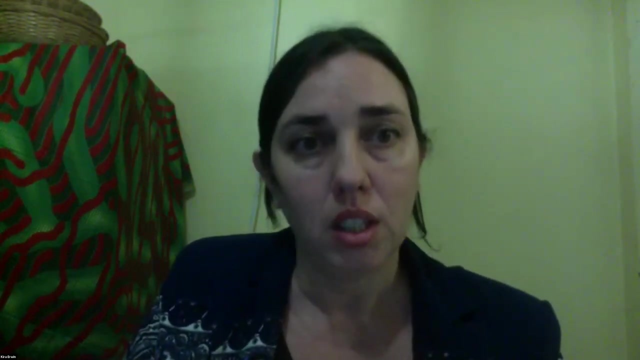 we're trying to do. I think one of the most important things to recognize, if you're trying to both communicate but attempt to change policy nationally and internationally, is that it's impossible for any one of those fields to do it alone. So one of the most useful strategies that we found is thinking very carefully and carefully. 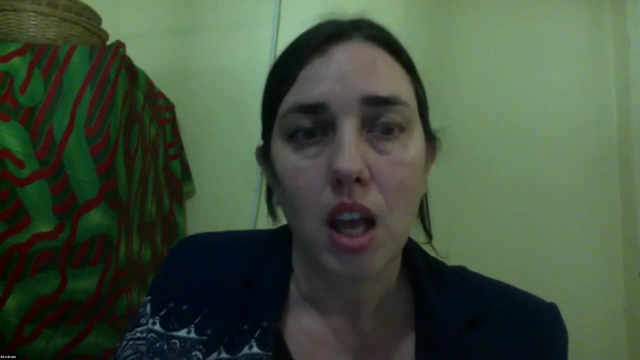 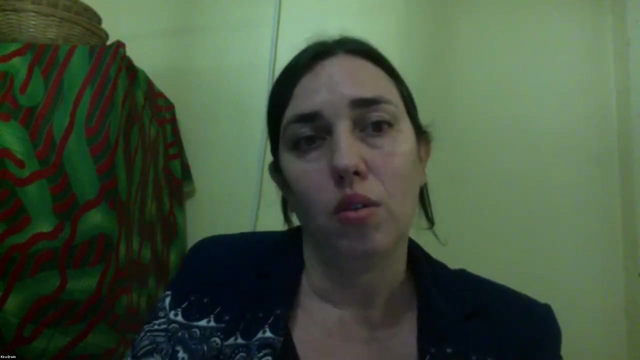 crafting and building your network of allies, And those allies can be unusual bedfellows sometimes. So allies can be scientists, Allies can be politicians, Allies can be activists. So I think that it's not just in the sort of form in which you want to communicate. 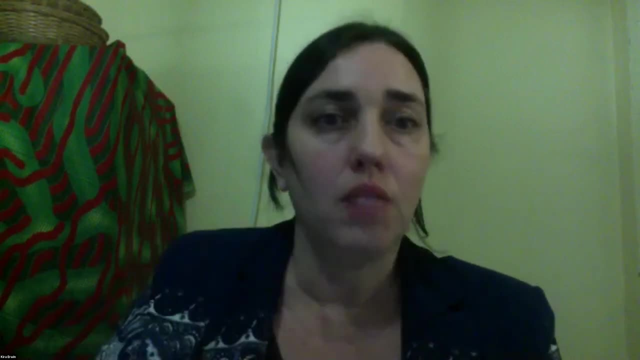 whether it's film, music, theater, scientific papers. More importantly, who's the network, who's the person that's going to get you the in? Actually, Kerry is one of our people that gets us the in sometimes when we know that she. 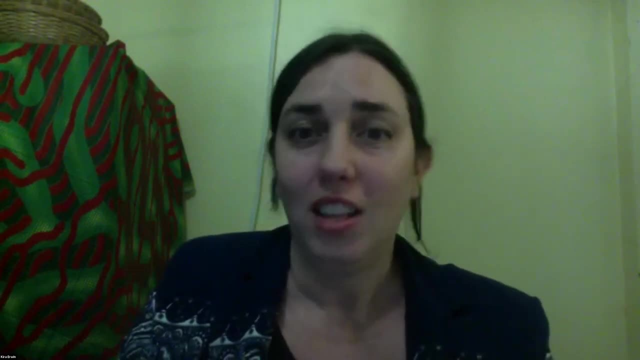 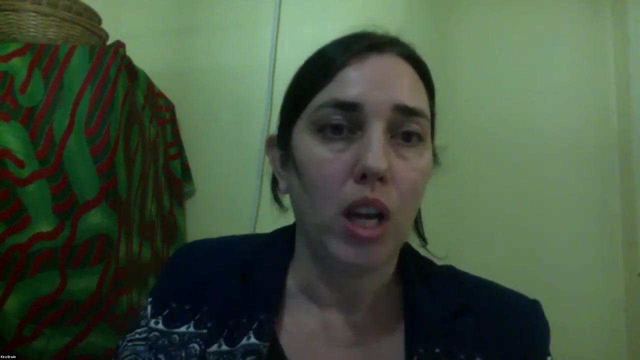 sits on the marine spatial planet And she's a very interesting body, then Kerry's an ally And we hope sometimes that we can be her ally in getting her message across in different ways. So for me, one of the important things is thinking through your network. 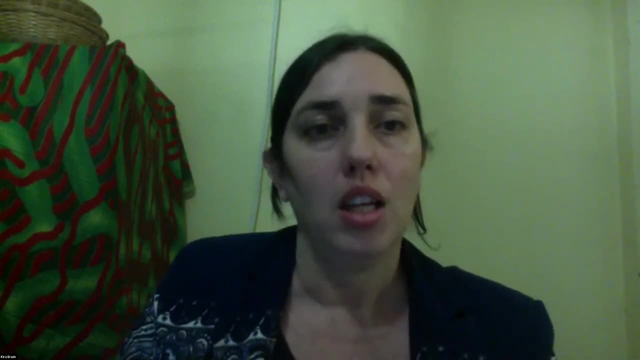 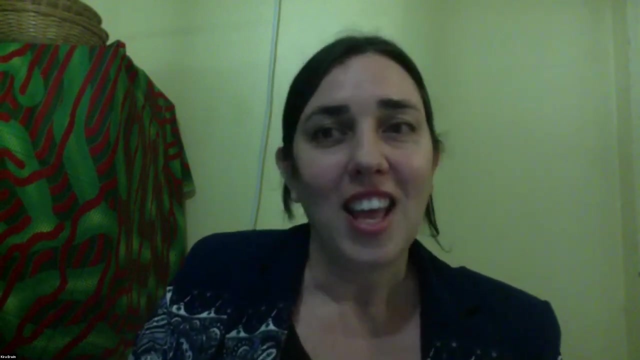 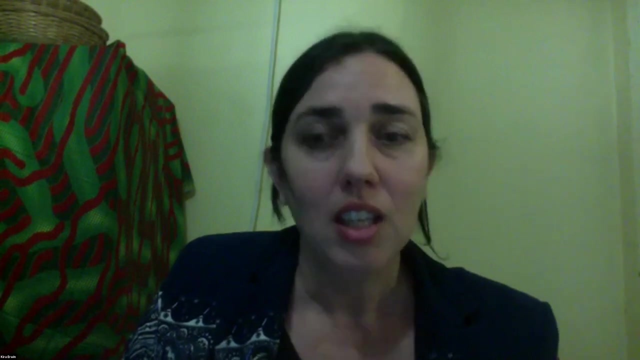 What is your strategy? How is your network working in solidarity, even if you're working in different ways, towards an end? I think that we may have to wrap up, and I'm really sorry about that, Because I think we could probably go on for much longer. 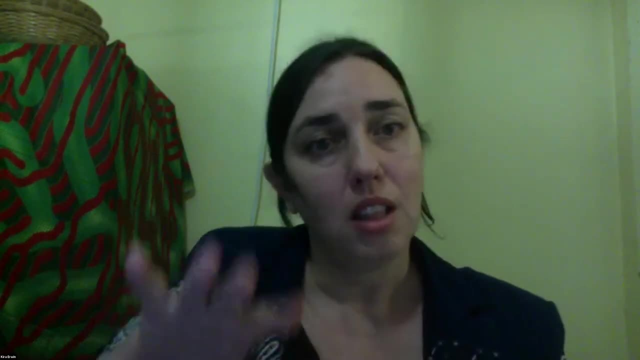 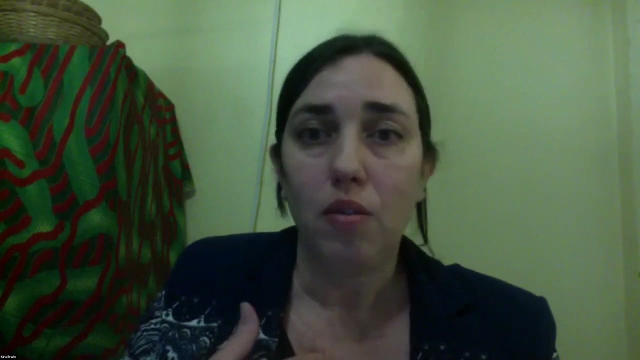 What we will do, and Jo's just reminded me, is that the video of this will be available. It can get emailed if you're interested in it, And I know certainly myself and, I'm sure, some of the other panelists, if you would. 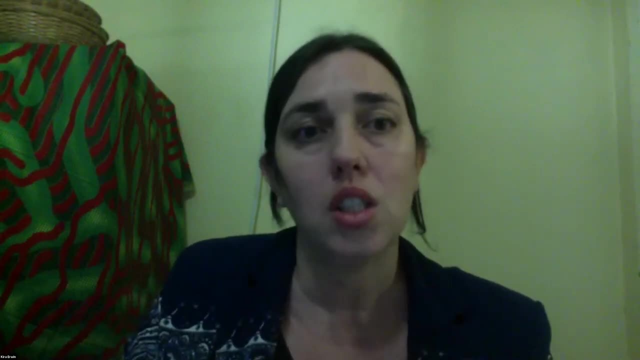 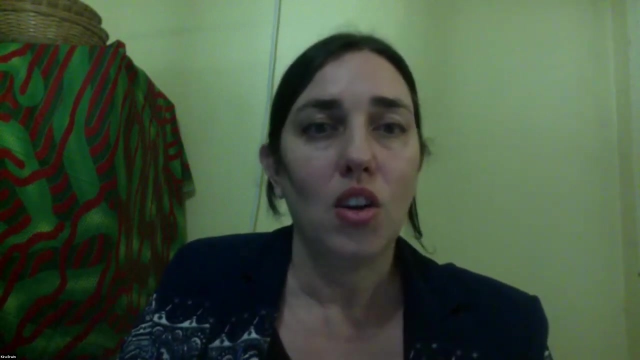 like to email us directly. if you have further questions or you want more information on some of the specific points that we raised, we'd be happy to take those. So just to say thank you so much for myself, What a fantastic day. Thank you. 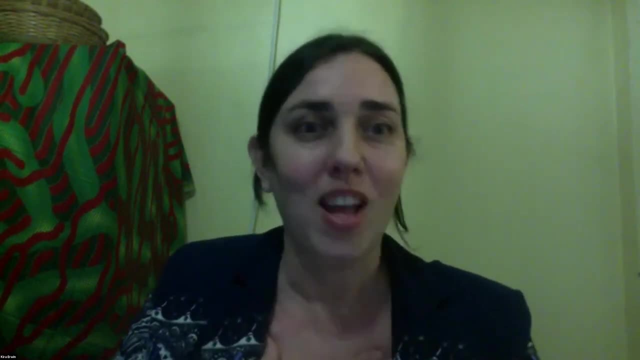 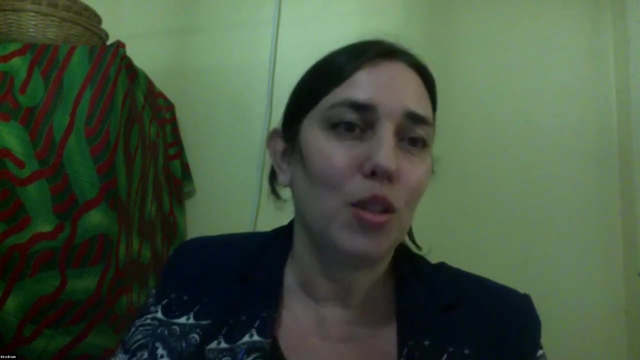 It was a fantastic event. I stayed awake the whole time. I've been on Zooms where that can be hard, but this has been really exciting. So I'd like to just say thanks once more and hand over to Elisa to do the close. 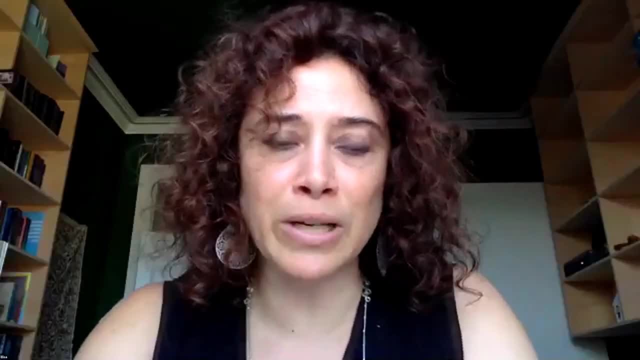 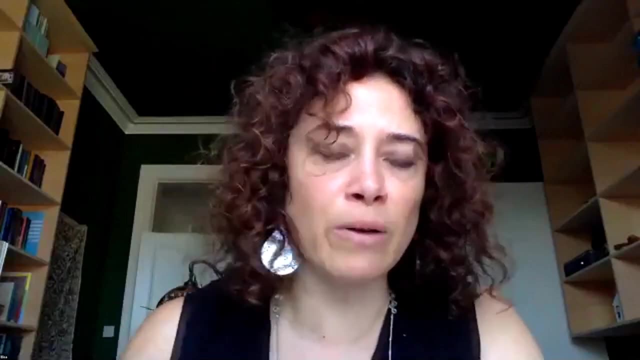 Yes, no, thank you so much. I also really enjoyed myself and learned a lot. I can see that the discussion has really picked up in the chat and I'm sure other colleagues who haven't had a chance to speak have benefited, and I would very much encourage them to stay. 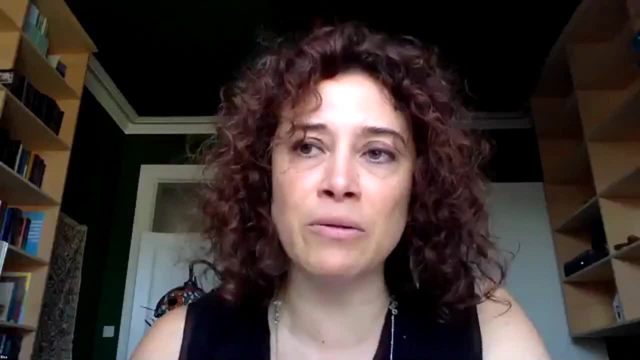 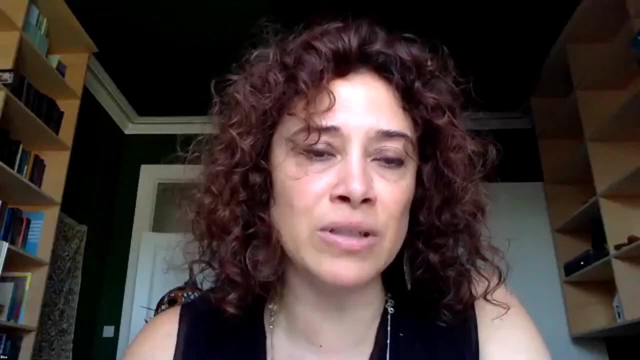 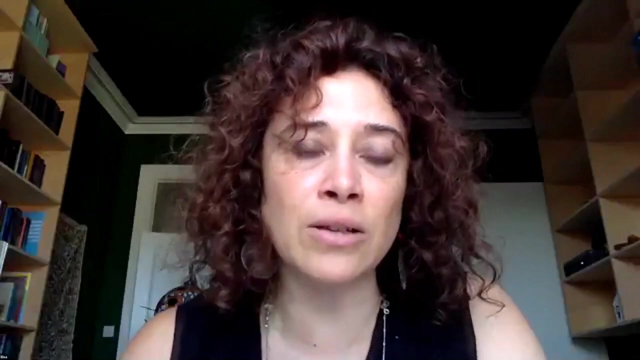 in touch with us. If they have any specific questions or interest in our own research, please reach out. I know as you subscribe for this event, you'll have now received One Ocean Hub newsletters, So don't be strangers. We really, I think a lot of our work and for us to make sure that our research is relevant. 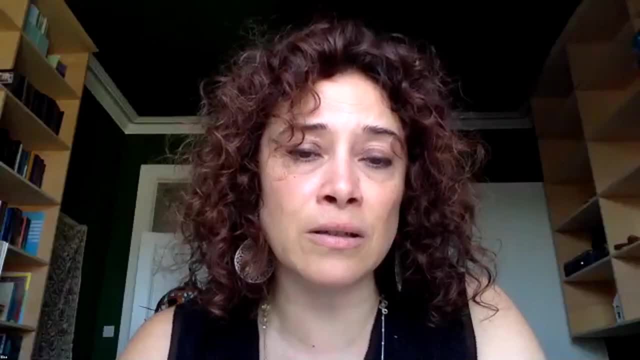 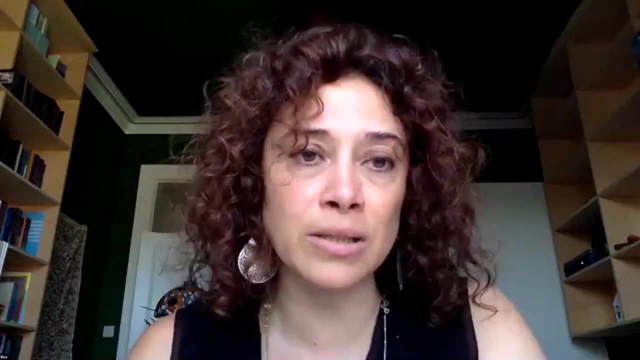 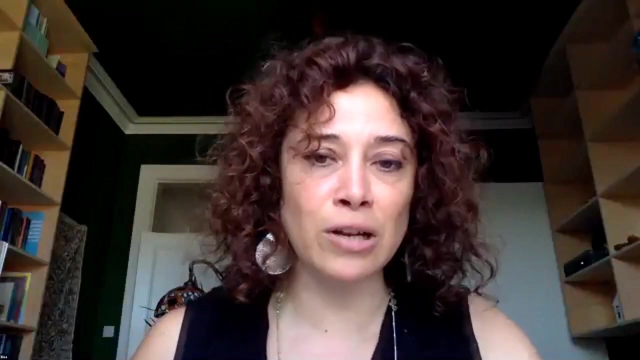 is very much keeping a dialogue with you and understanding the research you are doing or the challenges you're facing, and bringing them back into our own research to make sure we complement And address questions that are shared across different countries. I think as an international lawyer, and just to bring in a few other points that have been 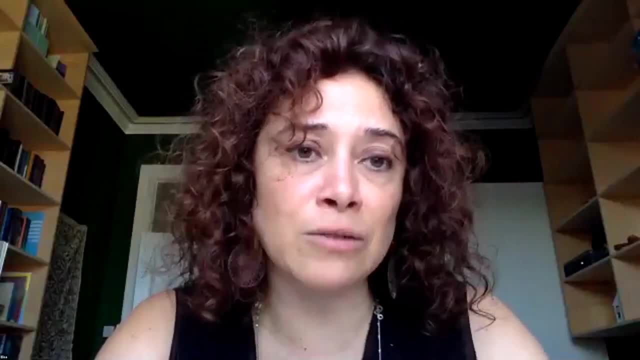 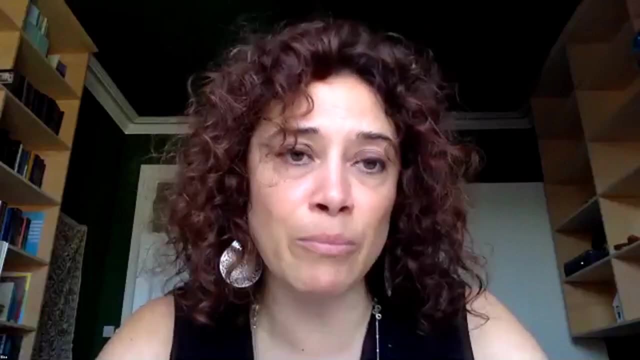 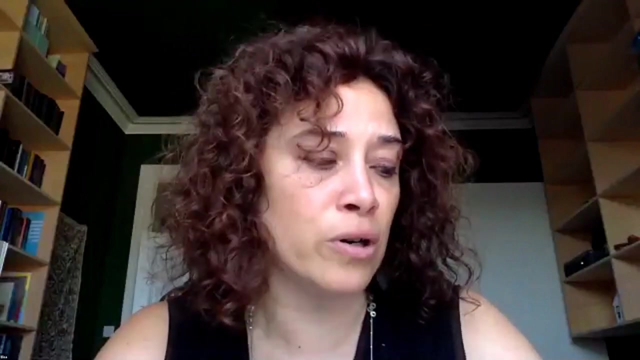 made and thinking also about the role that Strathclyde and the One Ocean Hub hope to play vis-a-vis the Nippon Fellowship Program and our collaboration with Yuen Doallos is really thinking, as a lawyer, what I have learned from these exchanges for my own work. 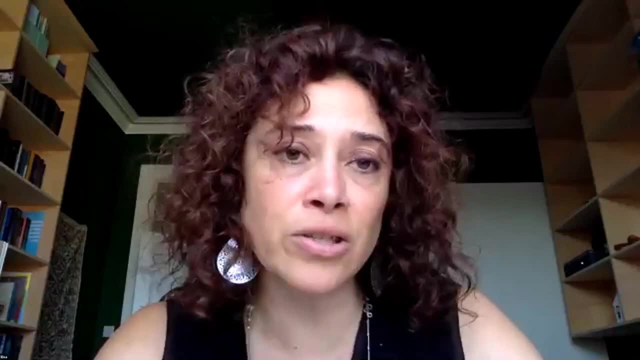 And, on the one hand, it's really understanding. Thank you, Thank you. Thank you so much, Thank you, Thank you, And also I know that you are just explaining the real world challenges in implementing international law and the law of the sea, particularly those bits that you think wouldn't. 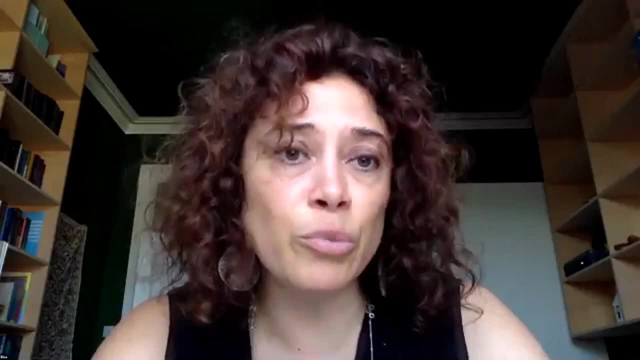 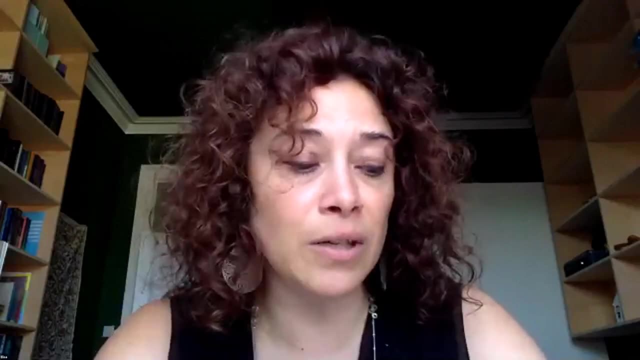 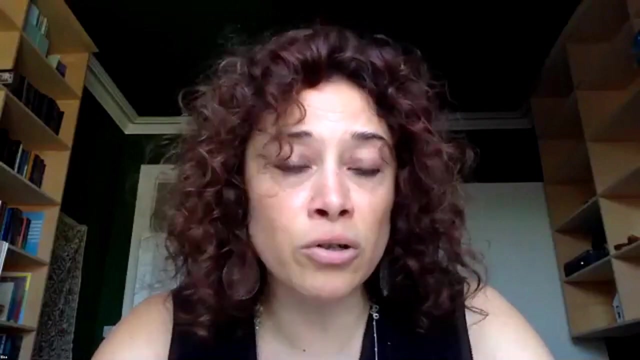 necessarily be very controversial. I mean we have very clear, beautiful provisions in the UN Convention on the law of the sea, on the importance of marine science, of sharing scientific information, and obligations related to scientific cooperation. I mean all of these obligations are, should be, non-controversial. they're very clear. 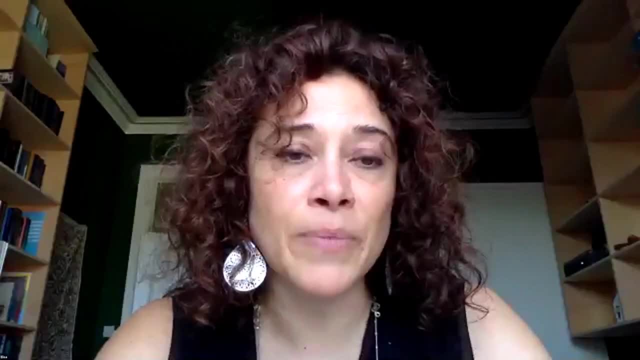 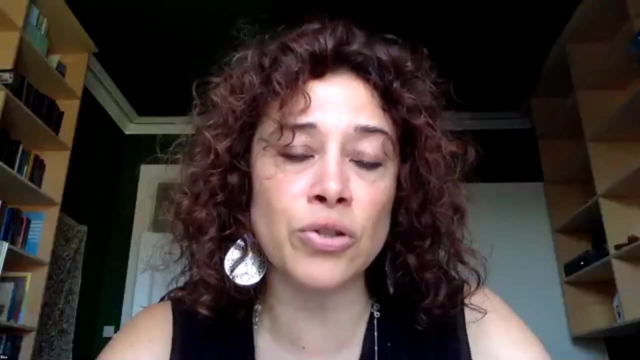 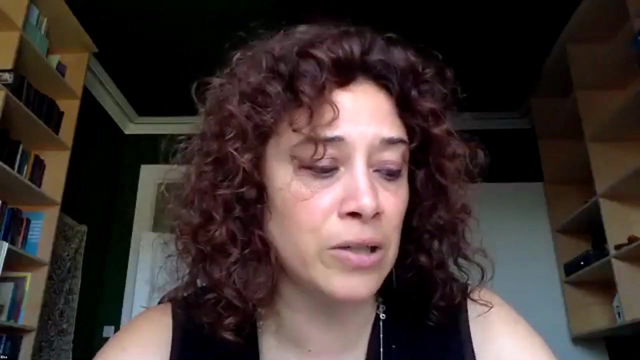 they make perfect sense. yet when you understand the the challenges of ocean research, how much we don't know and, as Kerry said, how much having access to technologies or not, how much building real relationships and actually friendships among researchers from different countries is crucial for us to advance, 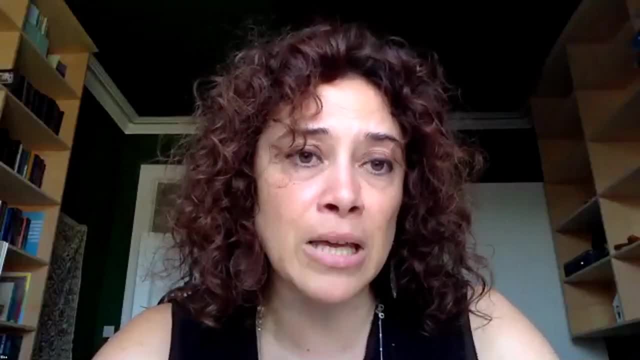 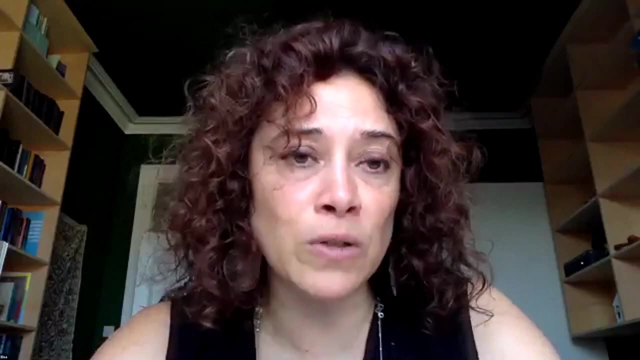 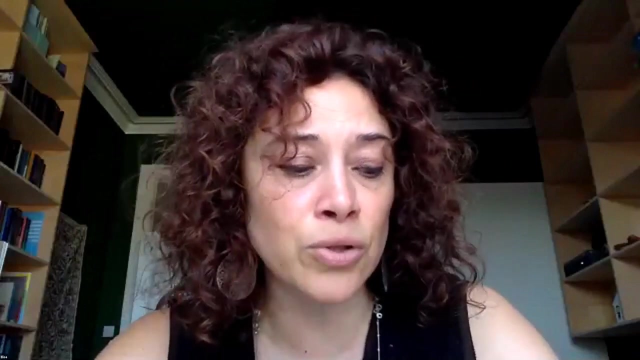 on, you know, building that knowledge base that can allow us to then take decisions on the ocean. it's it's a lot more than you know what those provisions in the convention on the law of the sea can convey. a question of costs: who has the budget? how these budgets are used, how many. 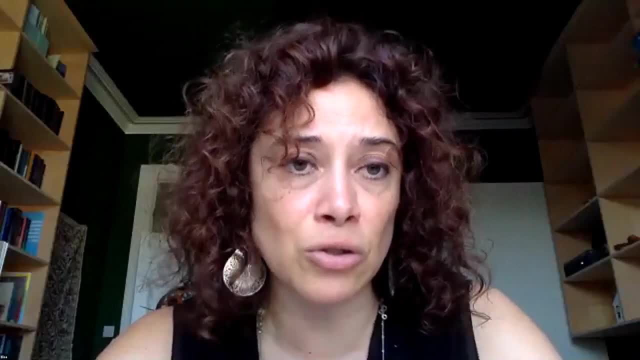 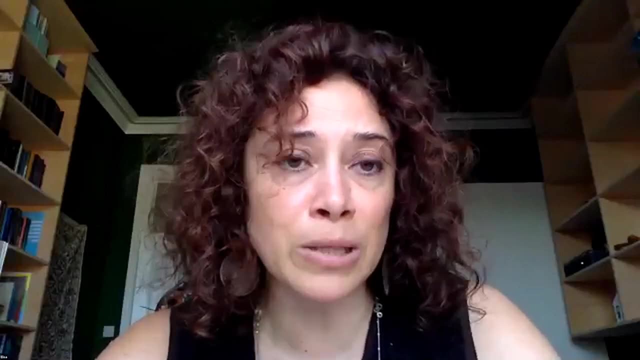 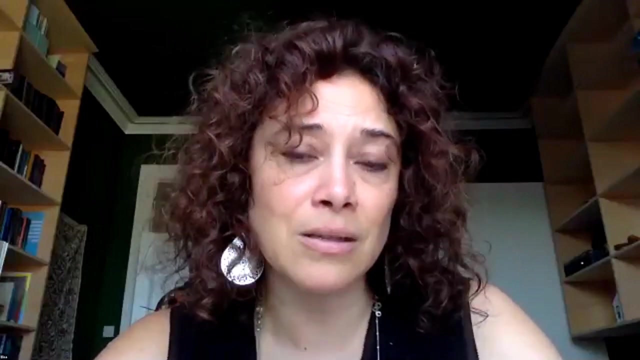 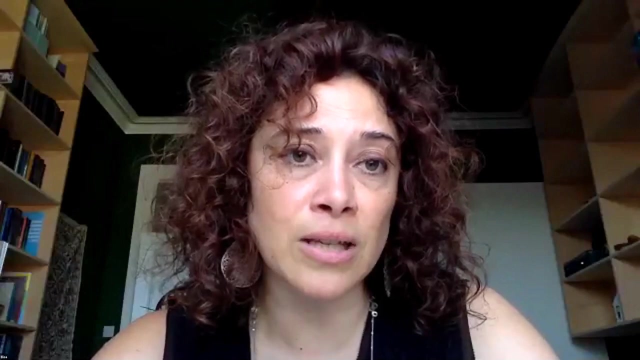 colleagues from across the world can benefit from the financing that is going into ocean research, particularly deep sea research, and how the capacity and technologies are built is really important, and there are processes like the BB&J negotiations where we hear from scientists and where the policy makers are, of course, in contact with researchers in their own countries to try and make sure that. 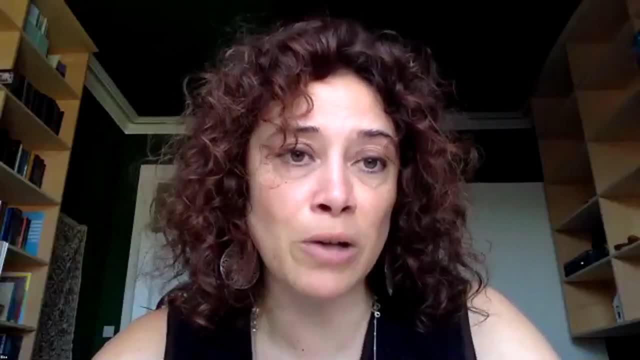 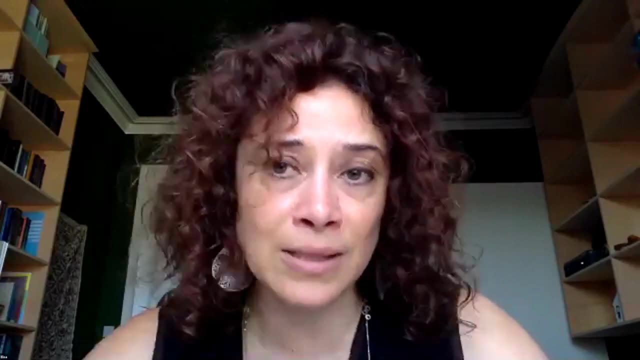 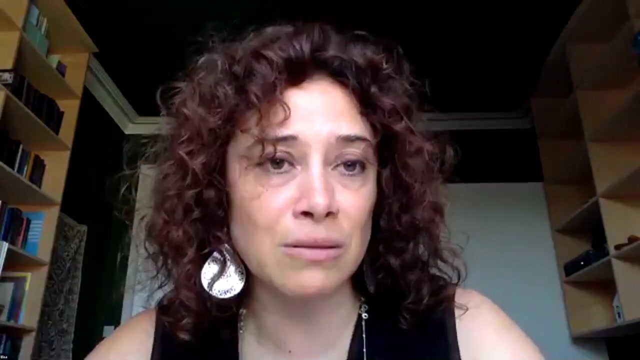 the new international law of the sea we're developing is responsive, but I think much more dialogue and and documentation of lessons learned needs to happen, and the more, as researchers and practitioners, we can exchange ideas and learn from each other- like, I think, the exchange with Andre about the experience in Brazil- I think the more we can all think more realistically and 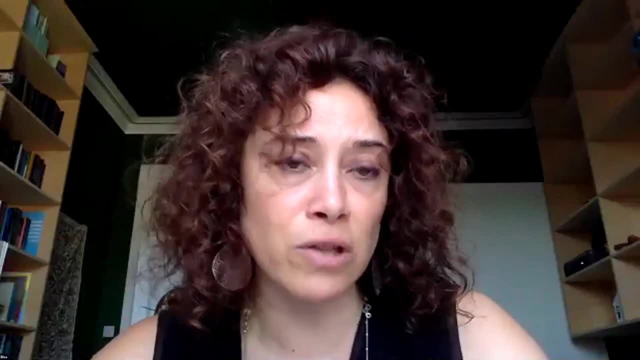 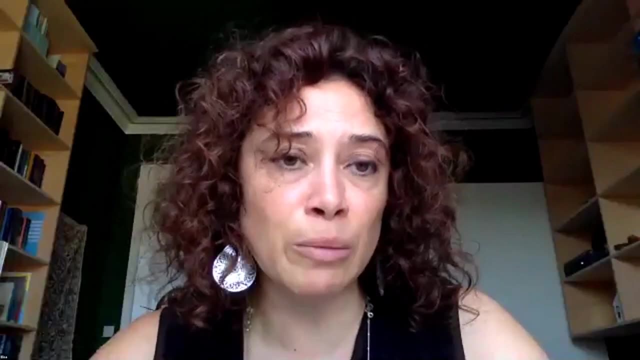 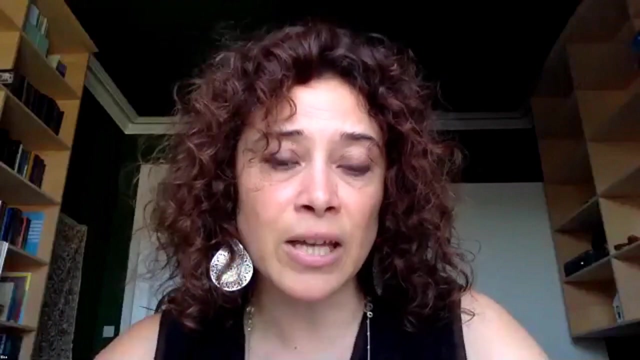 creatively about what it takes to realize those obligations of the law of the sea on science. equally, I think we made some good points here and there about the importance of general principles of international environmental law and the law of the sea. precaution has been mentioned a few times and, of course, understanding 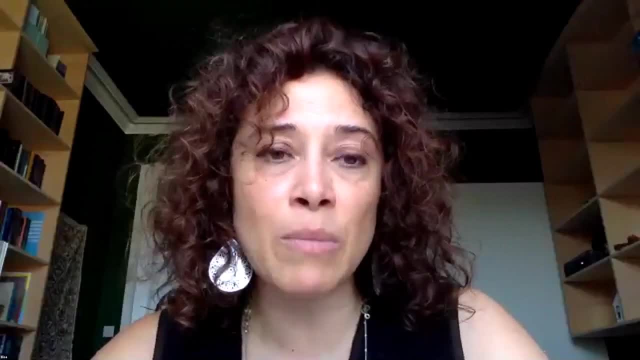 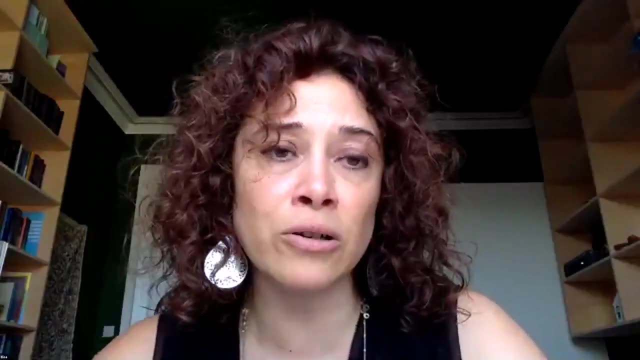 from Kerry how much we don't know about the oceans and how much the fact that we don't know means that we need to protect and develop more knowledge. and, how Sean said, how they're both the wonders- unique features, but there's a lot of the things that we don't know about the oceans and 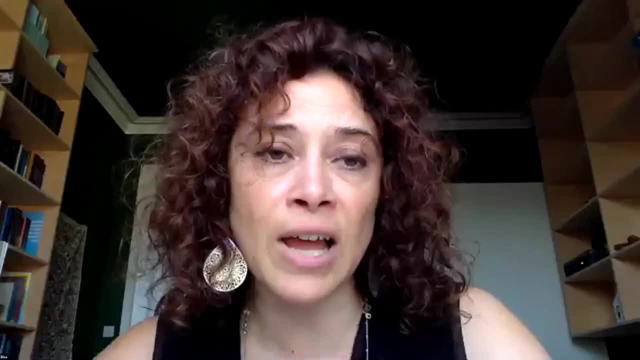 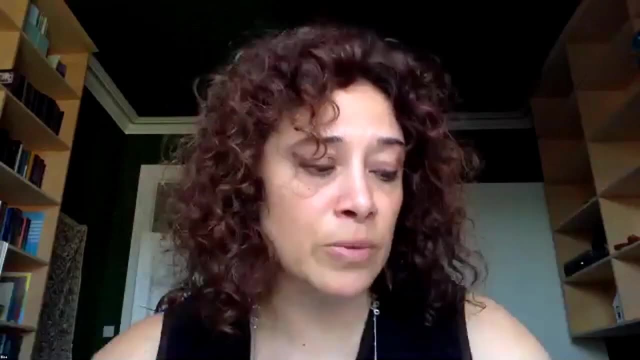 the fact that we don't know about the oceans and how much the fact that we don't know about the is also the commonplace features in the oceans and of ocean life that are critical for our continued well-being on earth. all of that just shows how how much, as as policy makers, we need to. 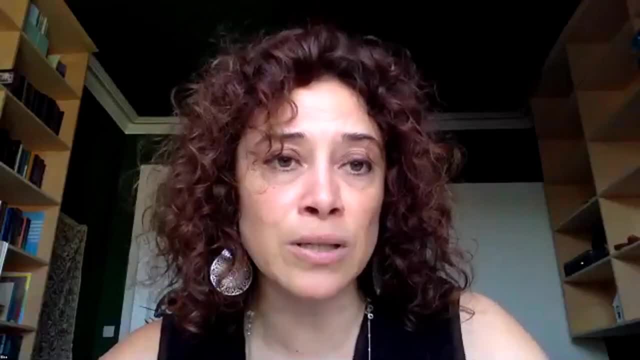 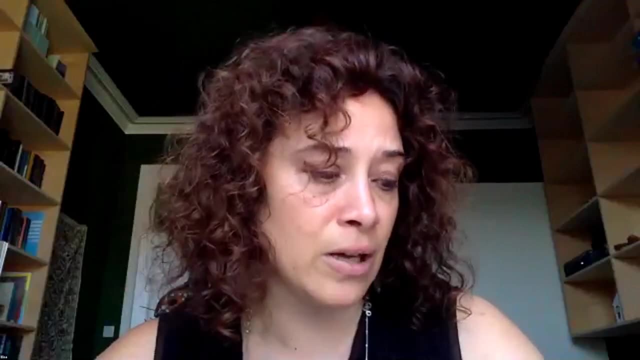 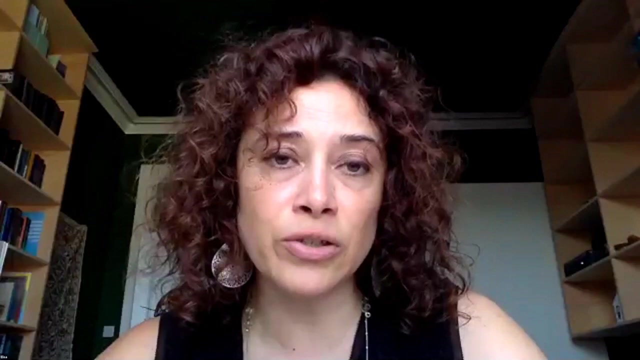 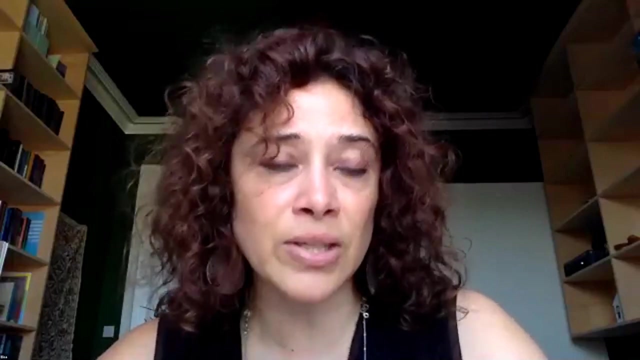 seriously engage with the idea of precaution and working with and ever evolving but still significantly limited scientific understanding of all the mysteries in the ocean. um, maybe another point, both around precaution and scientific cooperation, i think, is the role of uh reaching out to non-public bodies and the private sector that have more means and information. that is. 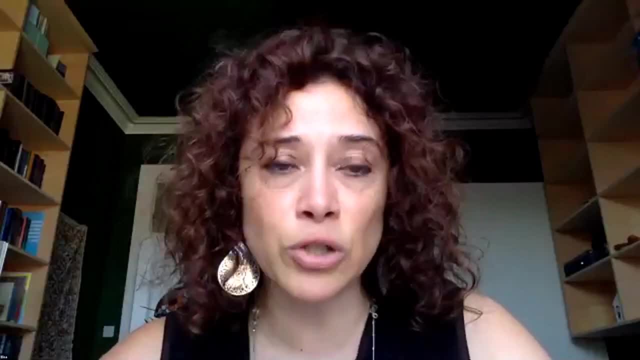 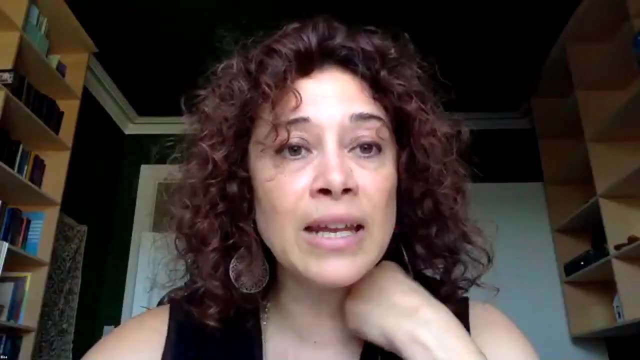 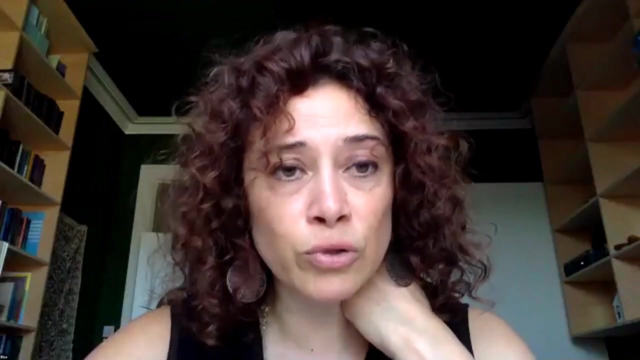 crucial for our shared purposes and the ways in which we do that, be that through communication, but also those individual relationships that we can build. and again, how, then, what we learn from that to share that more for other um colleagues around the world to to, you know, to increase. 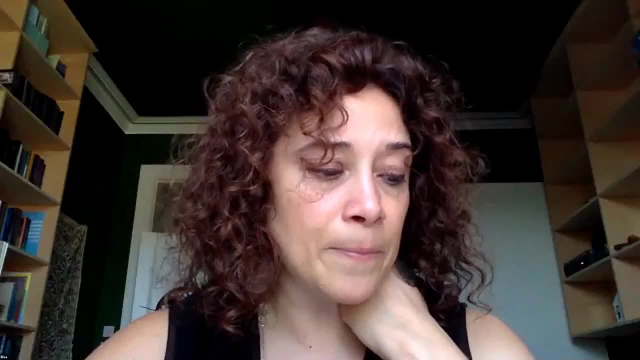 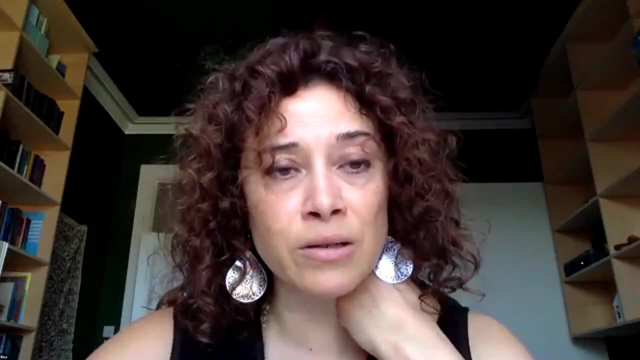 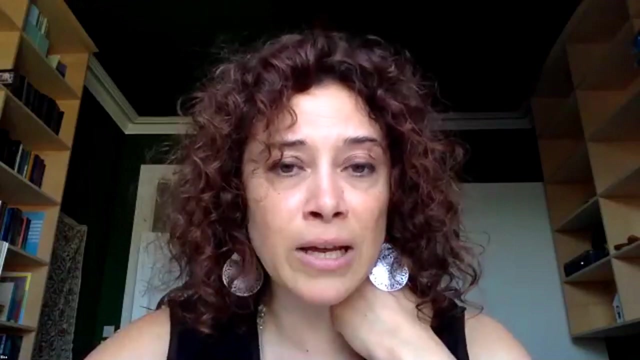 their success in creating those collaborations. um, and the final point is exactly that: that legal thinking that we still need to do and the practice around how we can bring together the love they see with international biodiversity law, international human rights law, international long cultural heritage, and finding the not only the challenges to those areas, but also solutions, how, as lawyers, 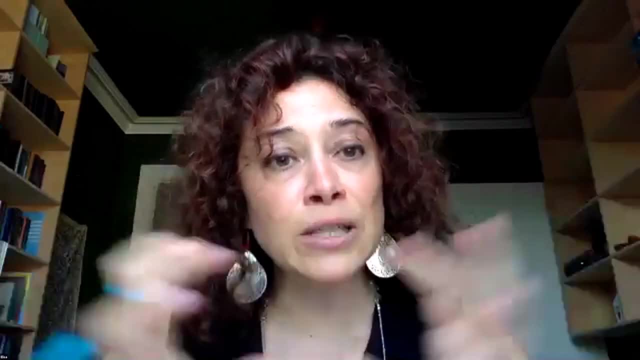 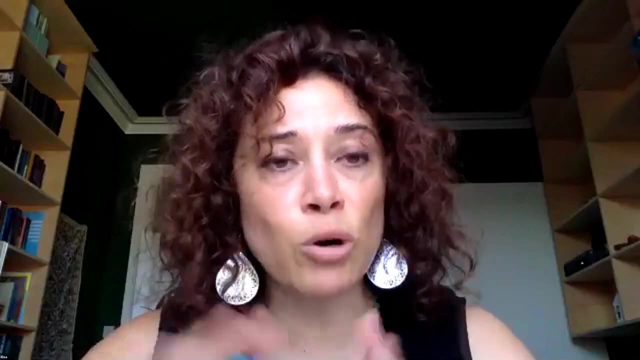 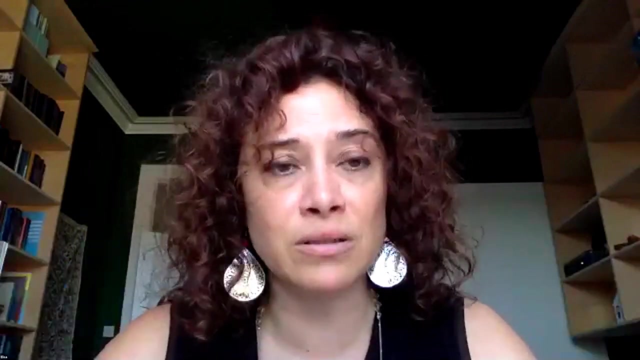 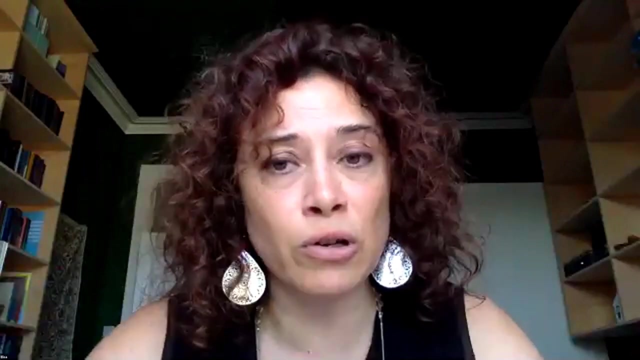 we can be more creative and involved in in reading together these areas of law and find solutions and showing to governments how this work is not made more complex by multiple sources of obligations, but in fact comes together. we have opportunities for policy coherence and for- um, i think- integrated approaches if we think about all these areas of law together. 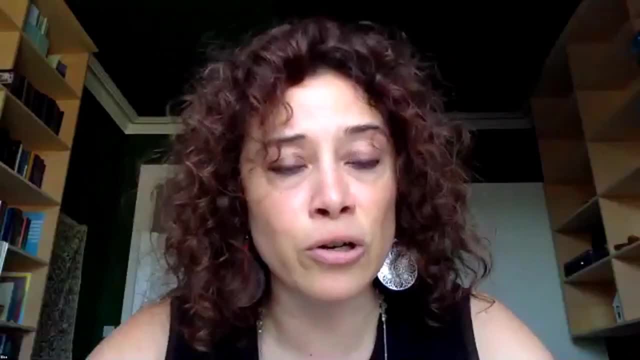 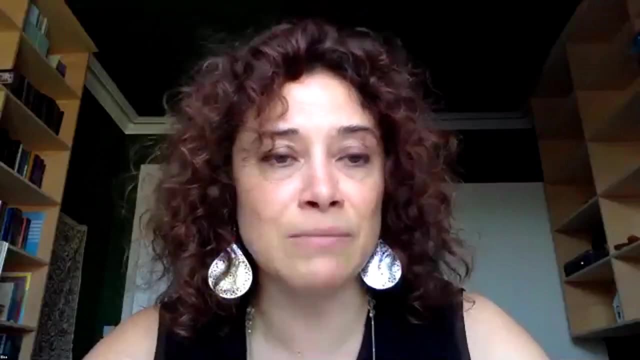 and we try and learn from the innovations that each area of law may have come up with, so ideas that human rights lawyers may have come up with. biodiversity lawyers and love this lawyer, so to say so. i think exchanges like today are one way to do it, and for lawyers, of course not. 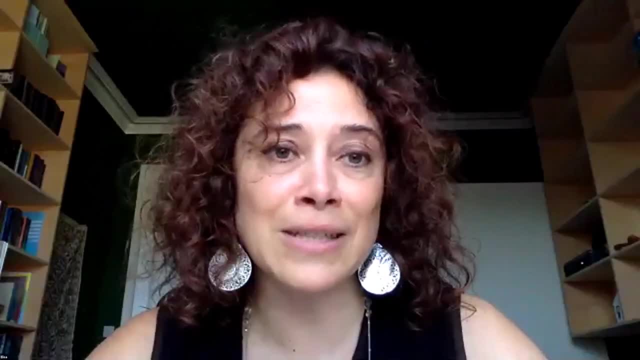 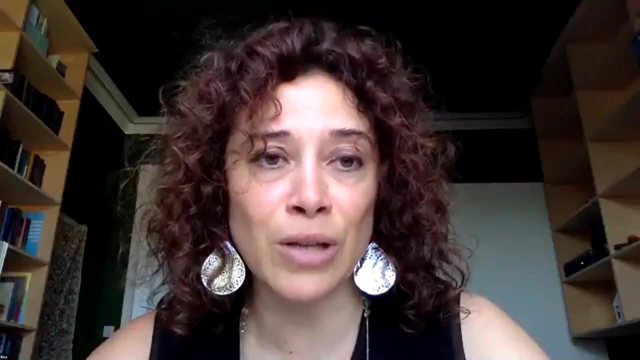 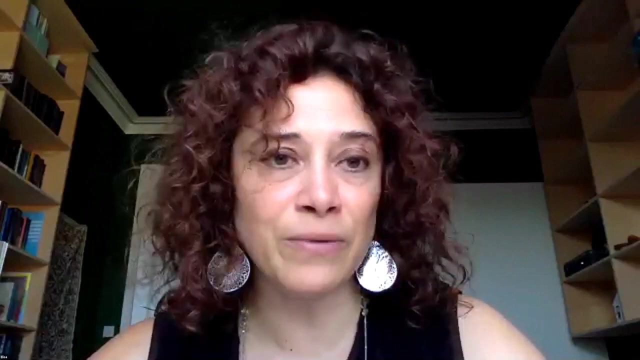 to speak just among themselves, but with colleagues in the marine sciences and social scientists and artists is um, i think, has been really already very transformational for me and we hope to learn more and more how we can do that through the one ocean hub and interactions with you. so i think we've 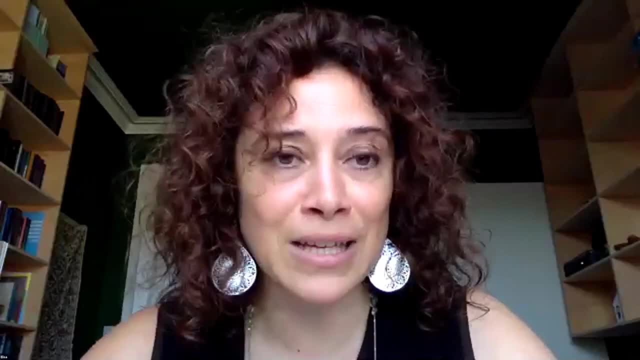 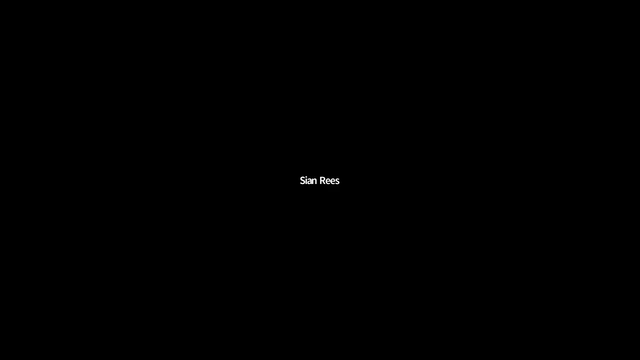 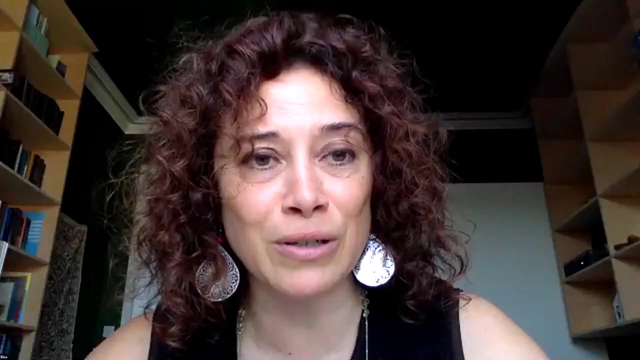 reached the very end of our session for today. i hope that we will stay in touch and hopefully see many of you at the sister section session we will organize on social sciences and the ocean science and policy interface in a few weeks. um. so do keep in touch and and we hope to see you very. soon and thank you so much for participating today.